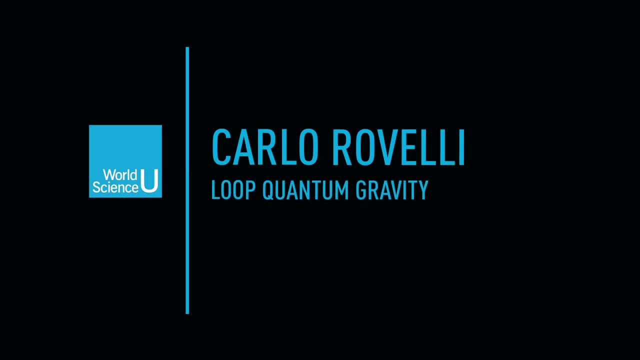 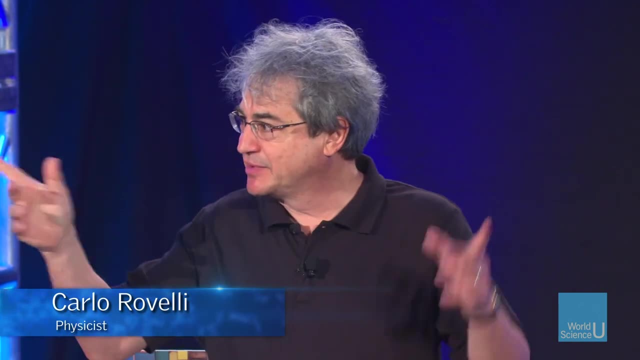 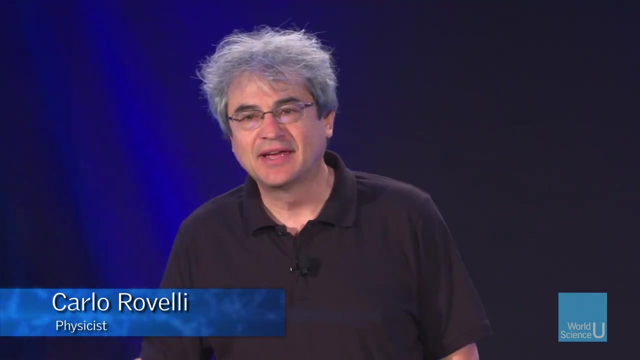 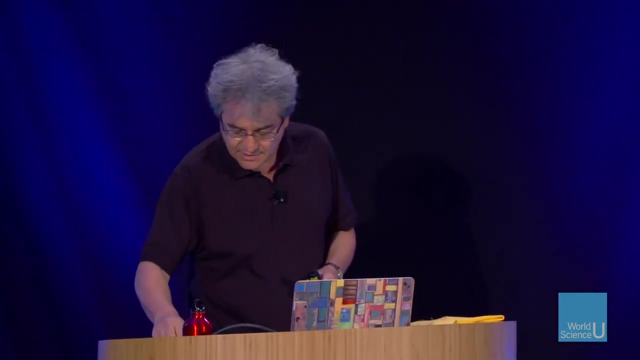 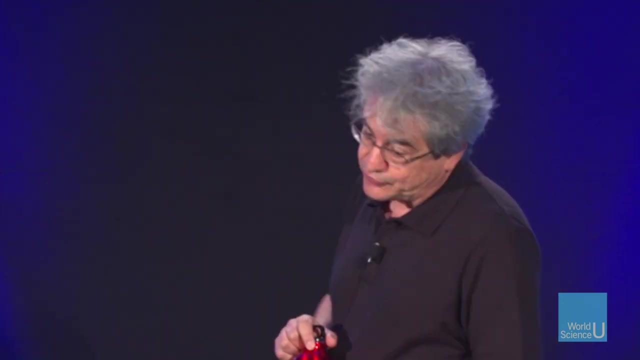 Well, thank you. Welcome all of you. Hello to the people who are here, Hello to the people who will be watching that online, Hello to the cameraman. I am going to talk about quantum gravity. And to talk about quantum gravity, I will break this in four parts. The first, 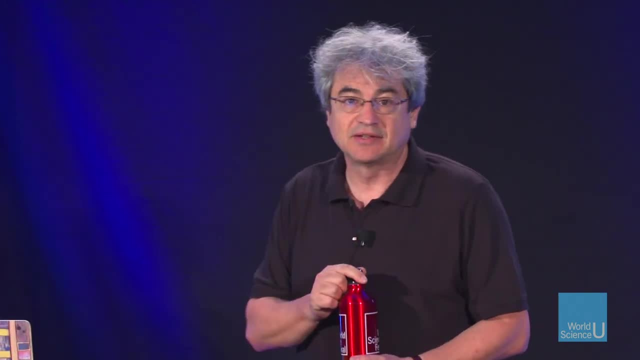 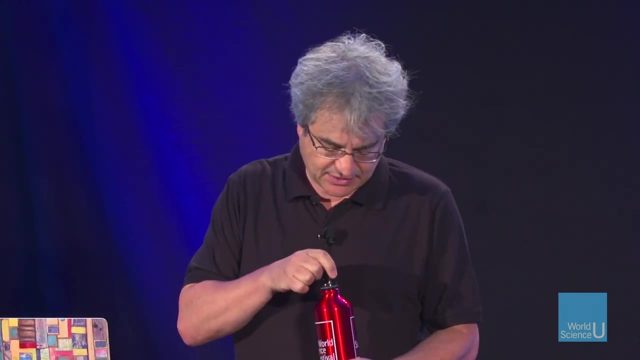 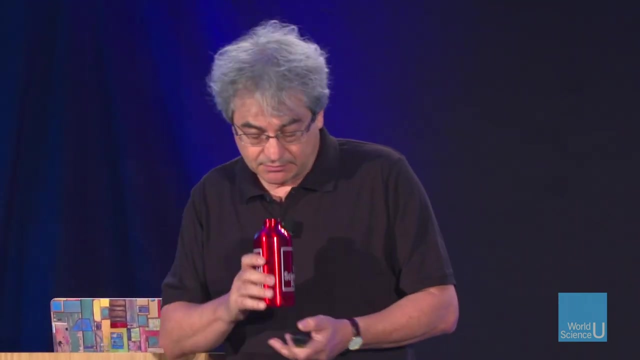 I will talk about gravity, The second about quantum And the third about quantum gravity. In the first and the second, I will just very rapidly review what we know about gravity and about quantum in a way which I think is Sorry. 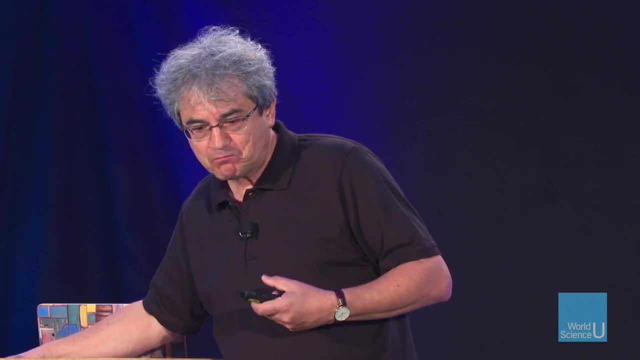 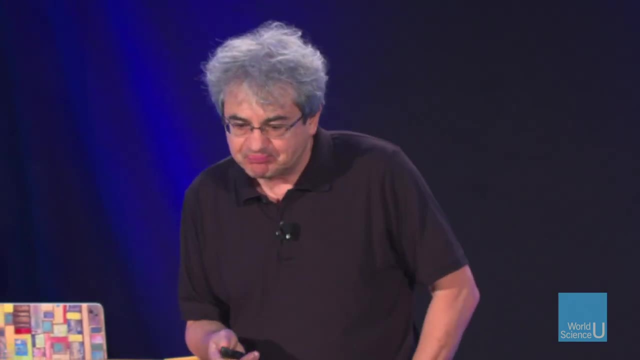 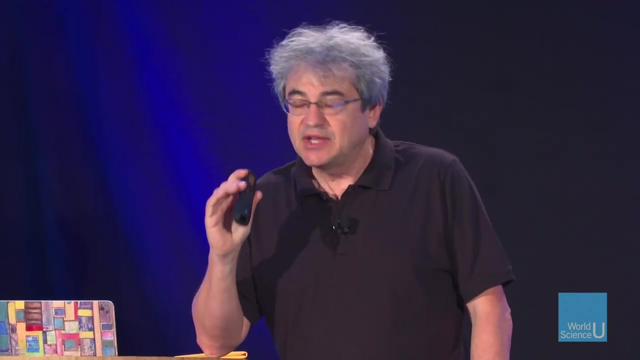 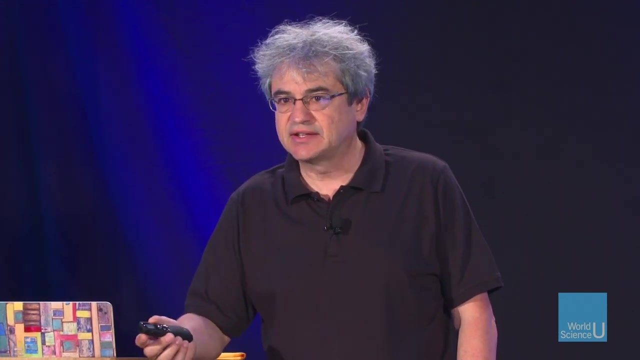 I need drugs to work. It's caffeine In a way which is adapted to put them together. And then in the fourth part, which is white holes, I will address the key problem of quantum gravity, which is to find experimental evidence that what we do is correct or not correct. 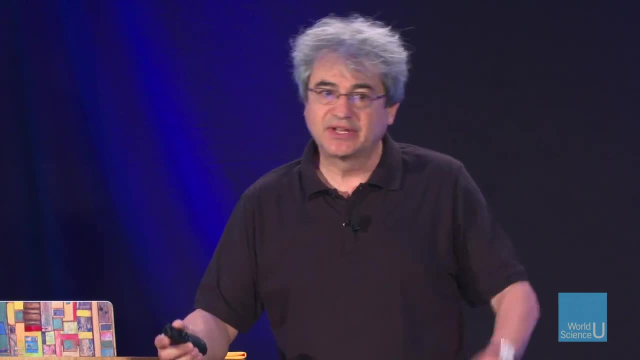 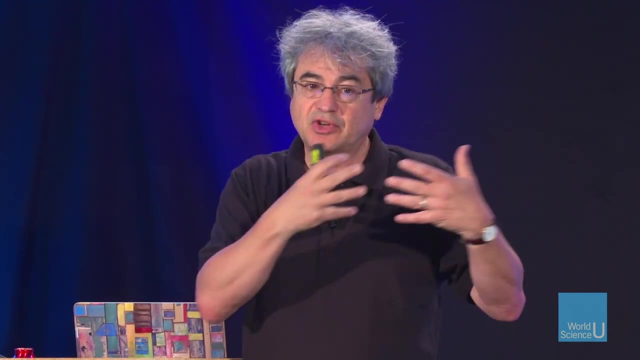 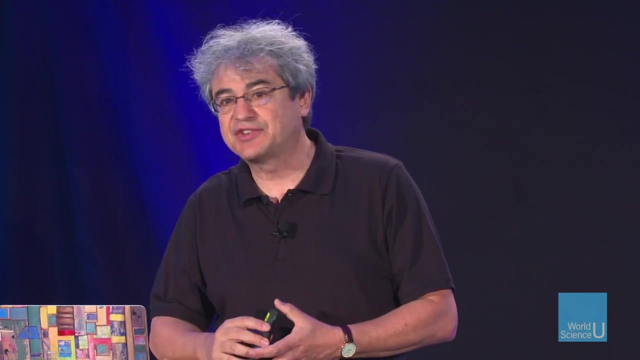 We in quantum gravity have a problem which is bringing What we know about space-time, what we know about quantum theory together. so do the quantum theory of space-time. We know that space-time has quantum properties. We strongly believe that space-time has quantum properties. We have tentative theories for describing quantum. 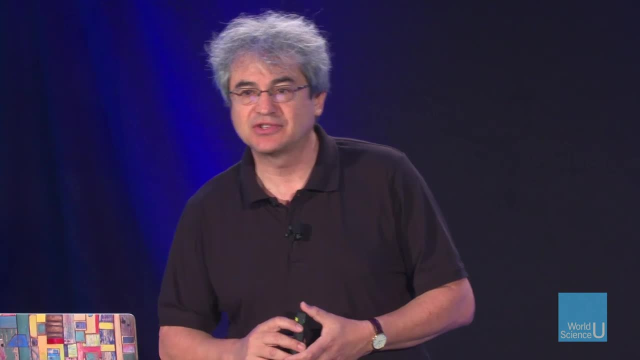 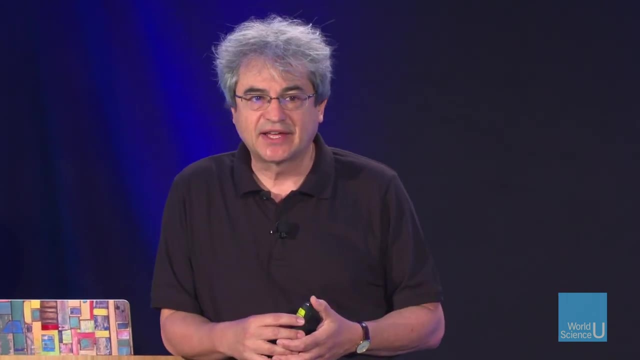 space-time. It's a nice, a beautiful. Some of us are passionate for one theory. Some of us are passionate for another theory. The problem is to know whether these theories are correct or not. The problem is to know whether these theories are correct or not. 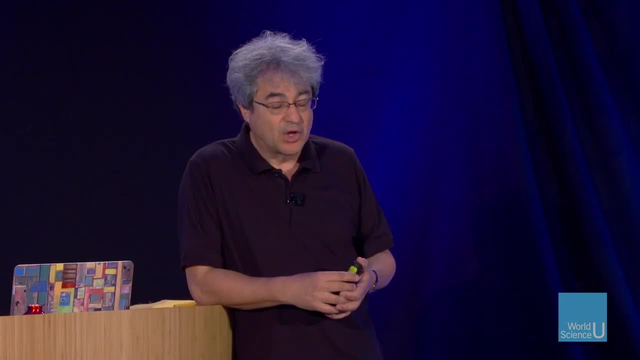 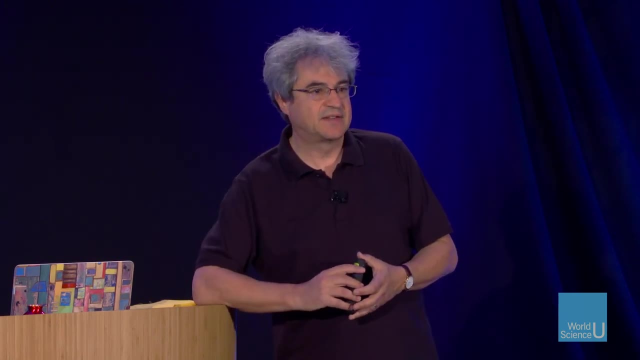 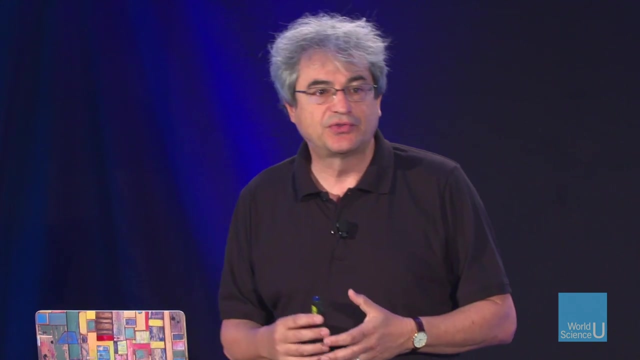 And to know that we have to make measurements and confirm or disconfirm, support or find evidence for or against the theory. And that's the most interesting part of the game, I think, Because after all the conceptual work of figuring out what is quantum space-time, we have to. 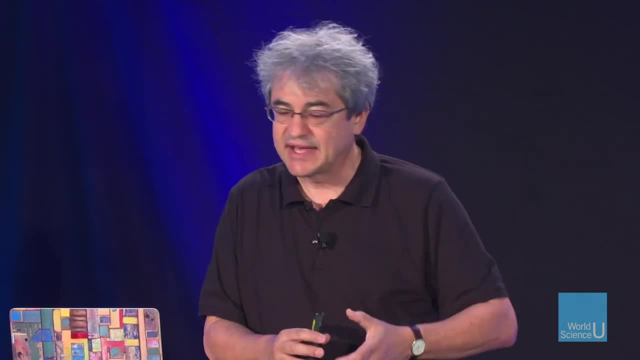 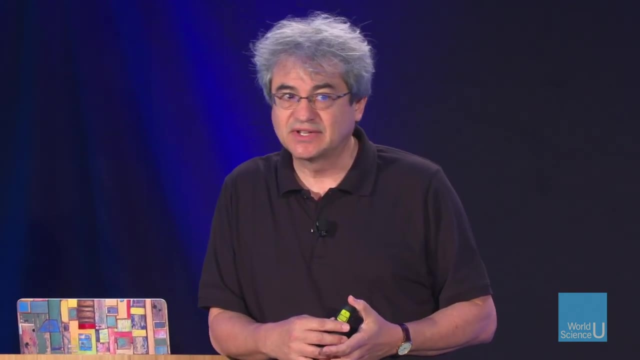 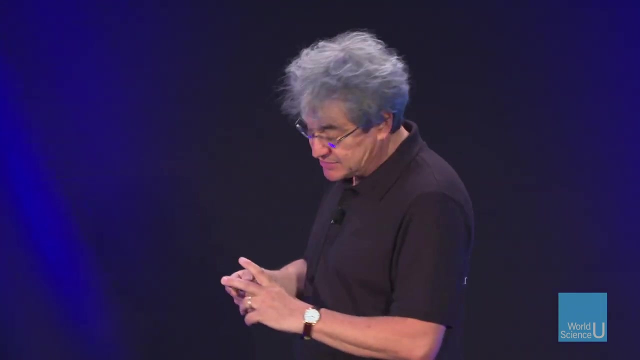 come back to reality and check these ideas against reality. And I will talk in the last part about one recent idea of how to check Our understanding of quantum gravity using White-Holtz. So four chapters. First chapter: gravity. Gravity, of course, is what makes things fall. 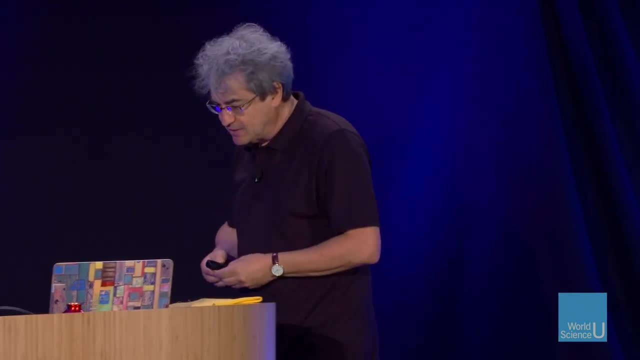 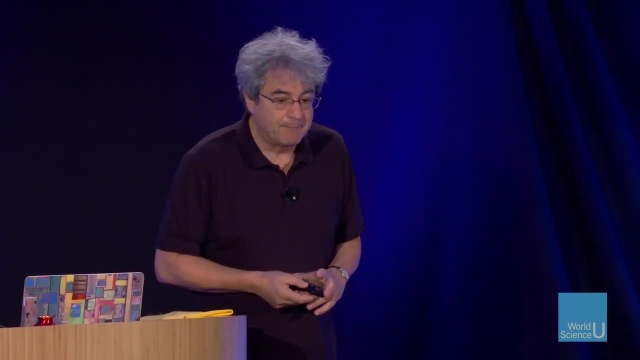 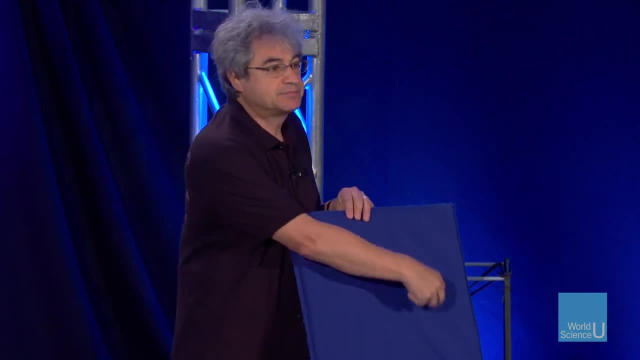 theory. is Newton had the idea of understanding gravity And Newton theory. is Newton theory? is Newton had the idea of understanding gravity And Newton theory? is Newton theory? is Newton had the idea of understanding gravity And Newton theory? is Newton had the idea of understanding gravity And Newton? 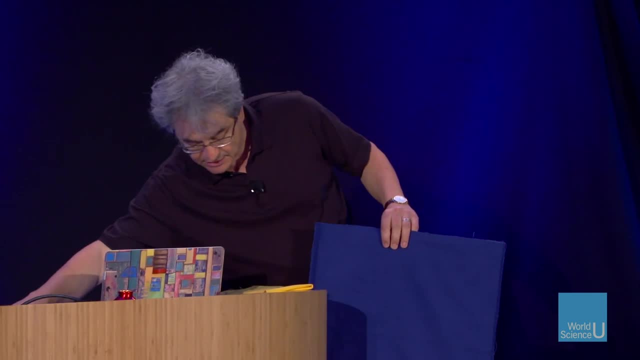 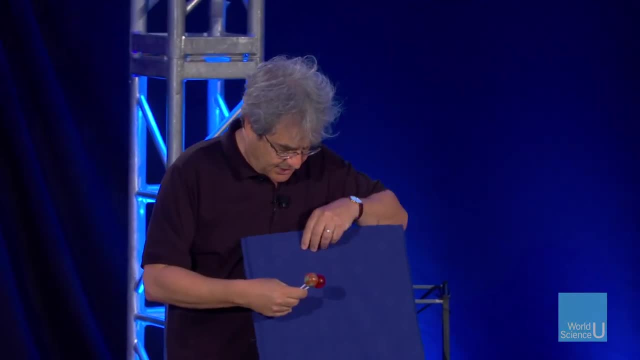 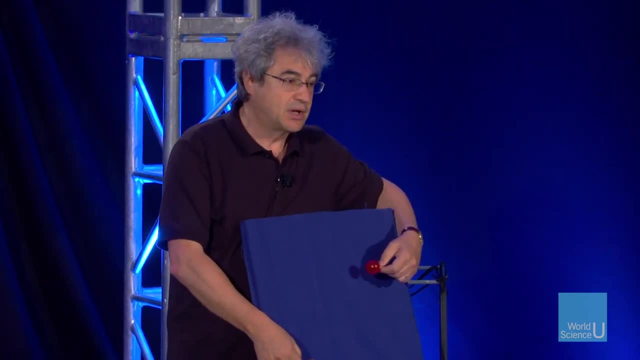 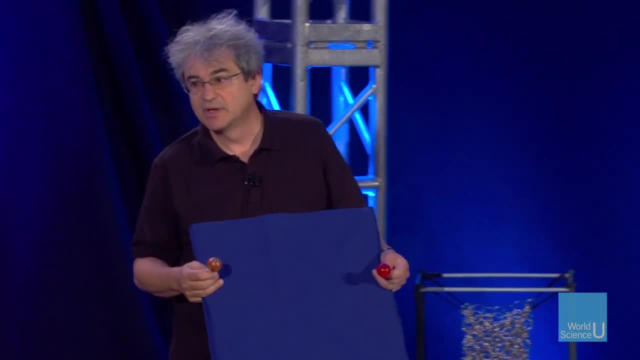 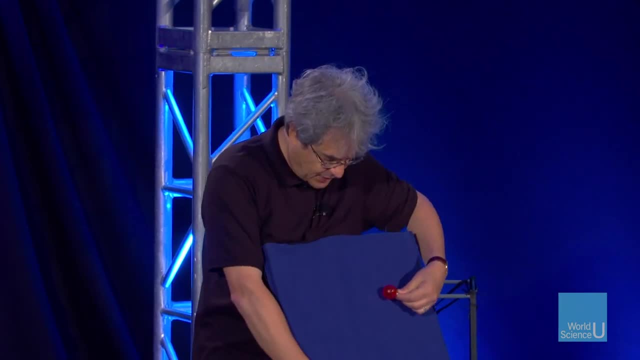 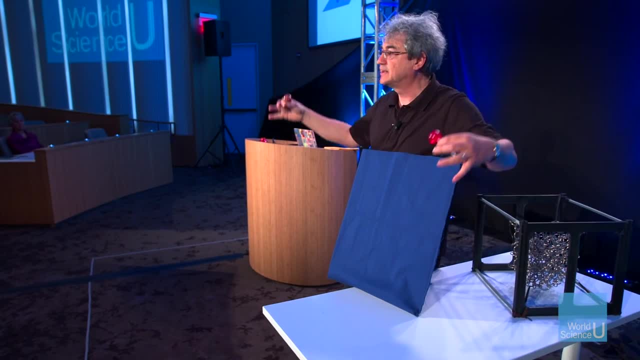 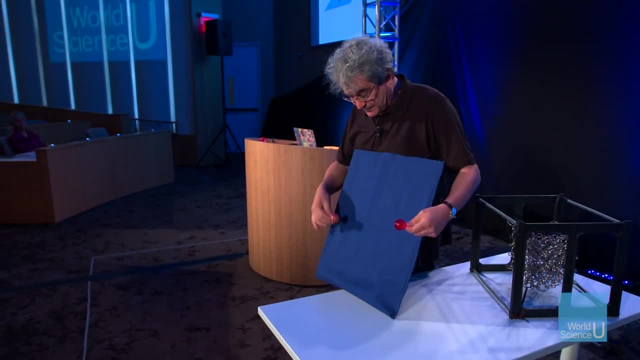 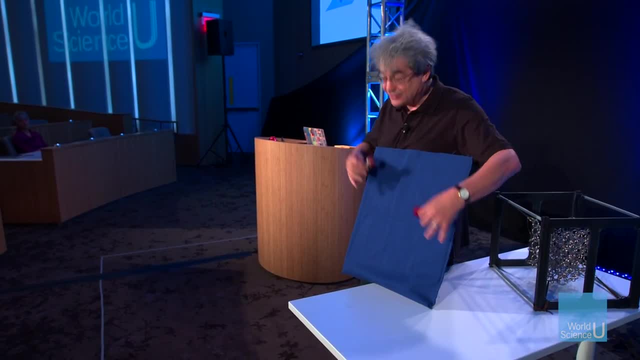 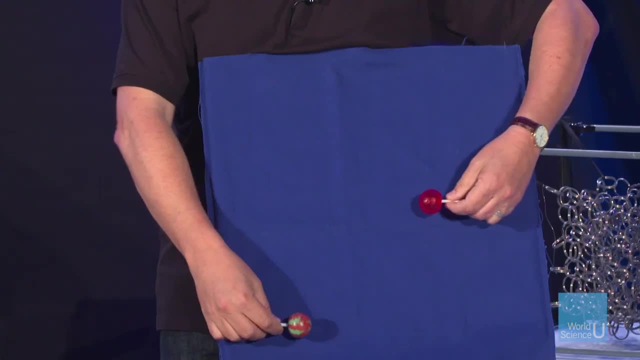 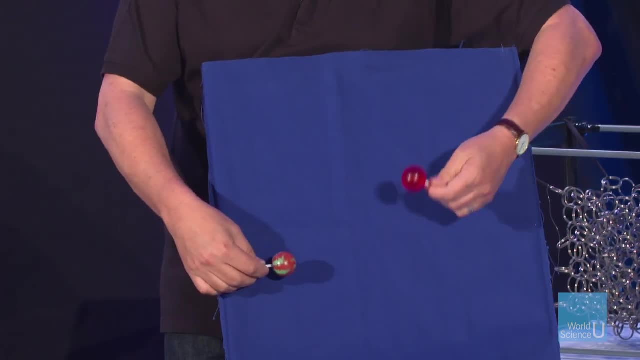 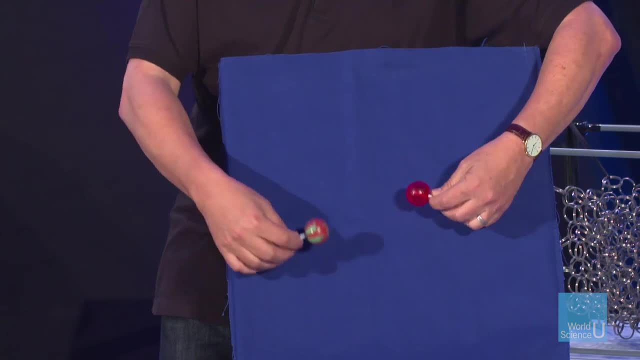 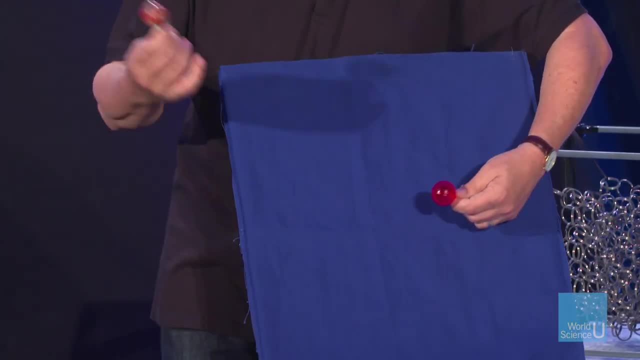 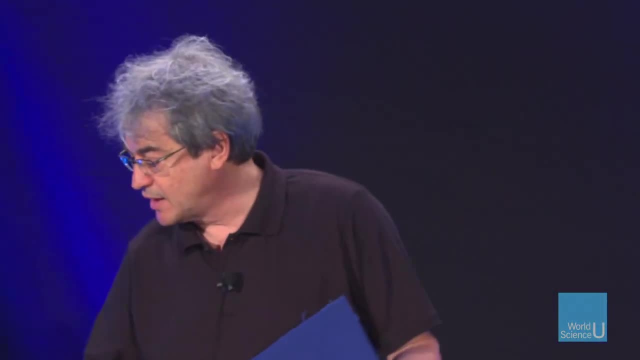 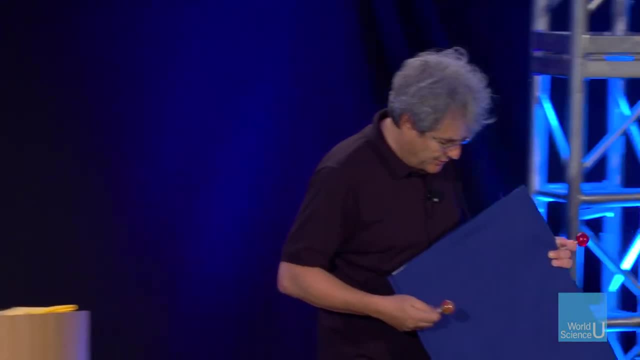 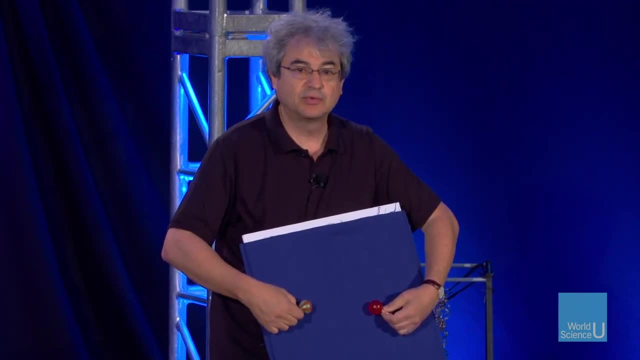 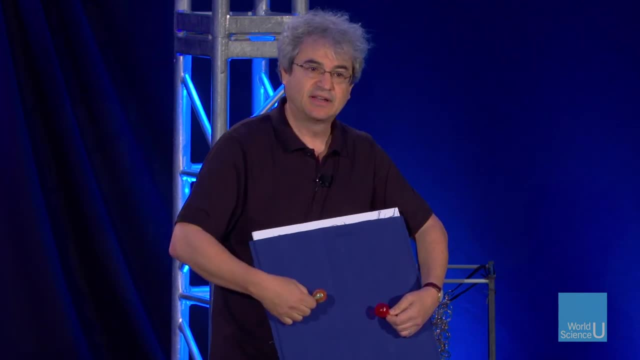 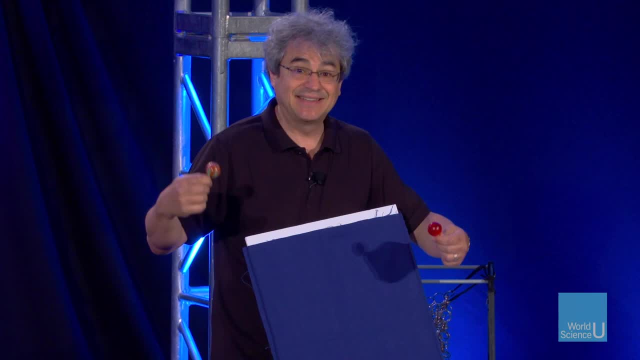 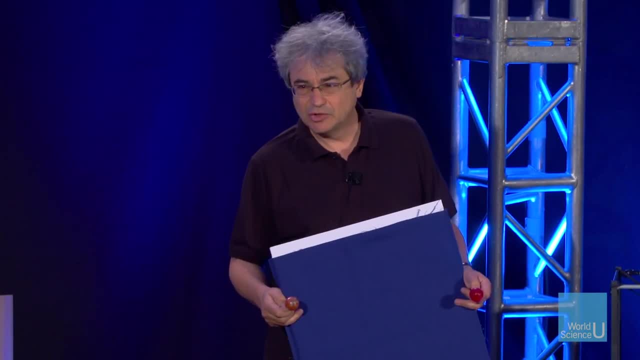 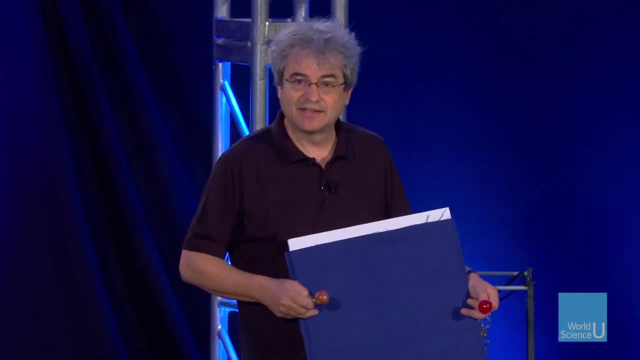 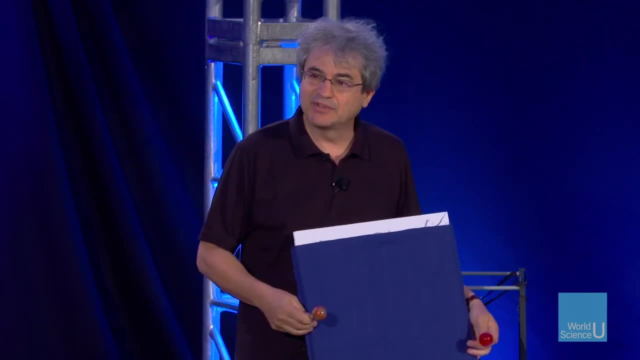 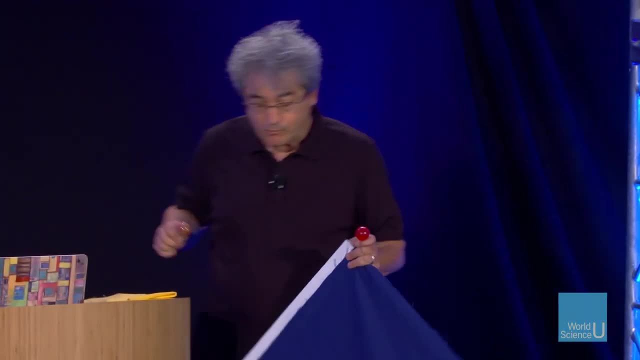 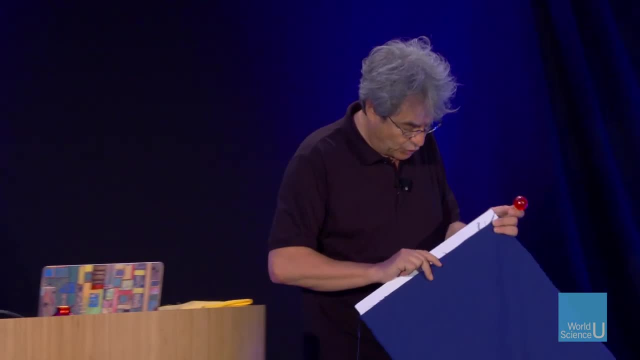 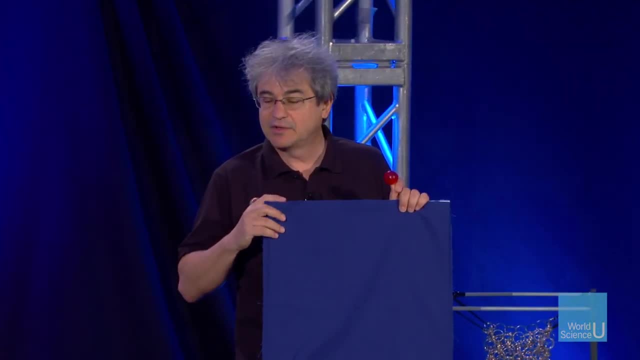 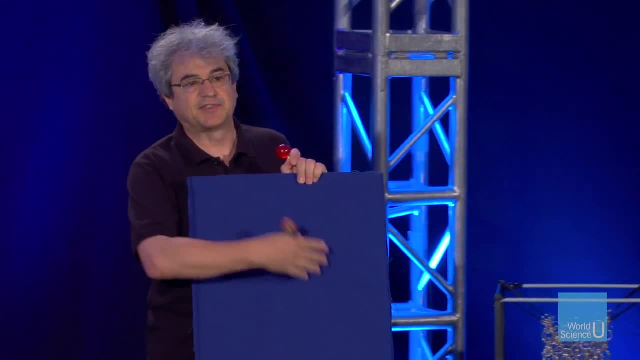 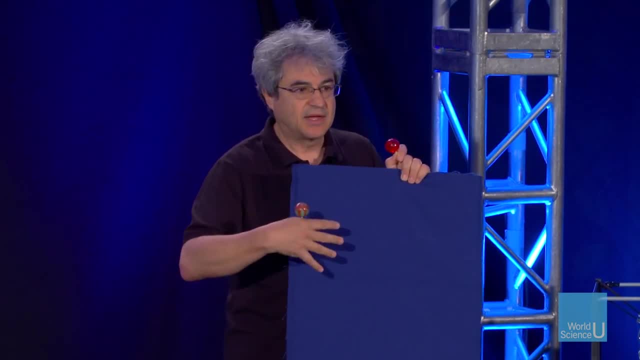 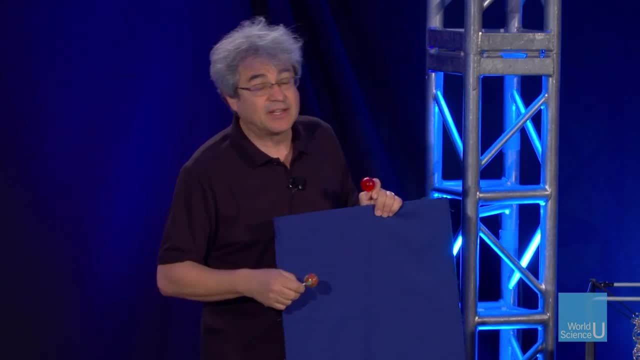 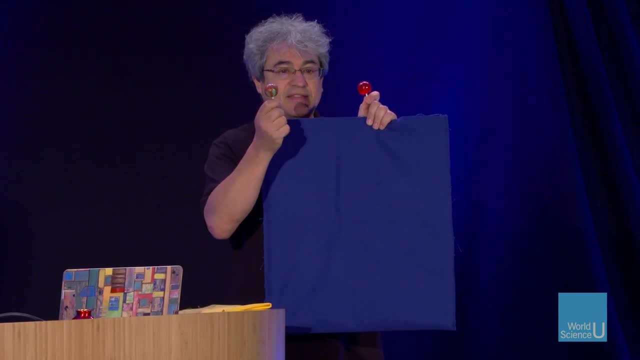 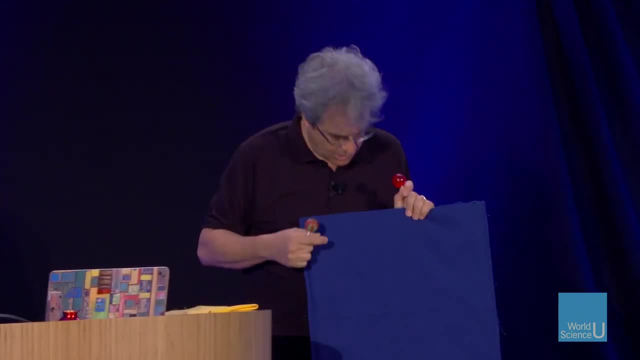 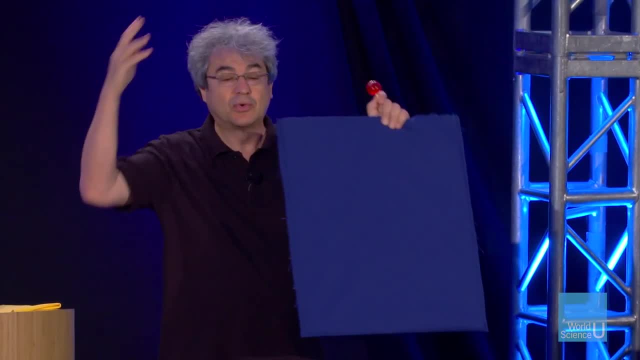 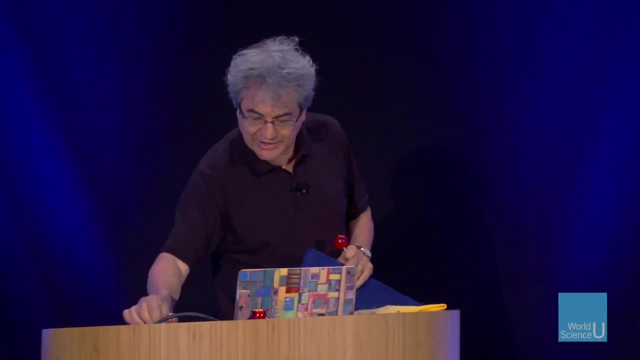 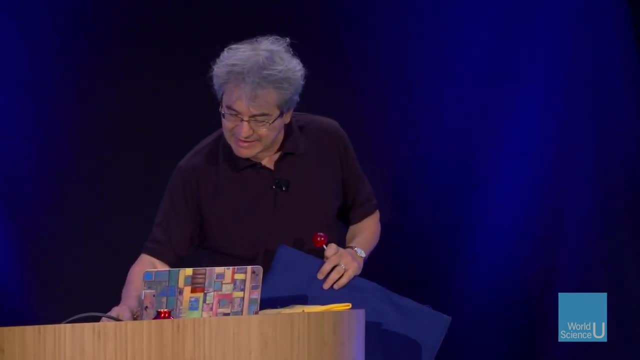 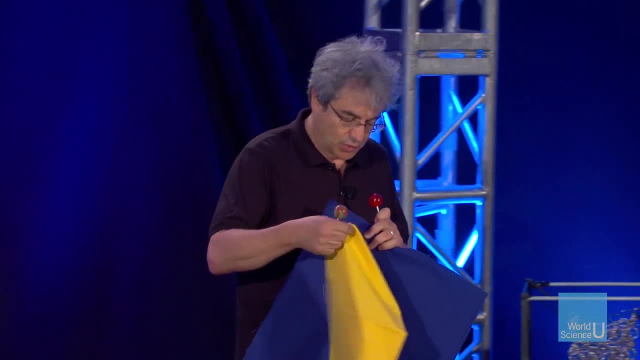 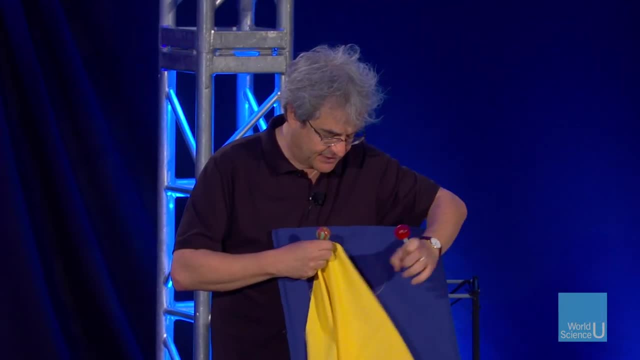 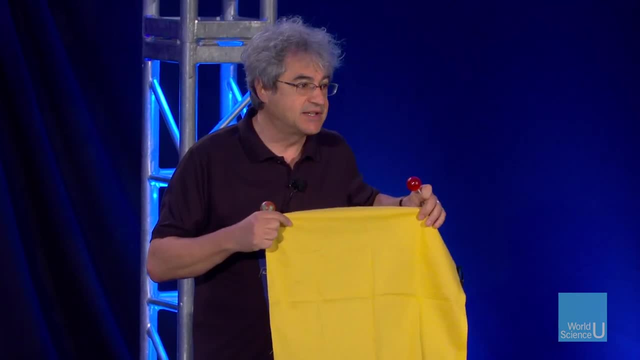 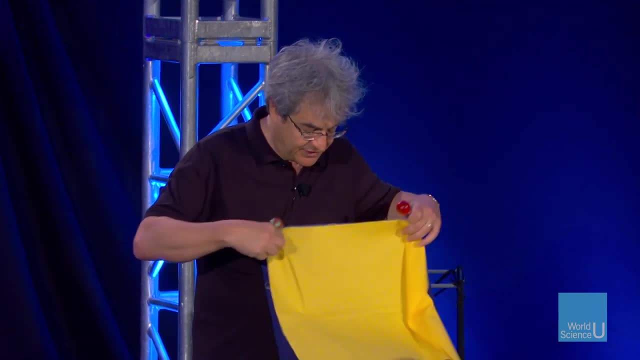 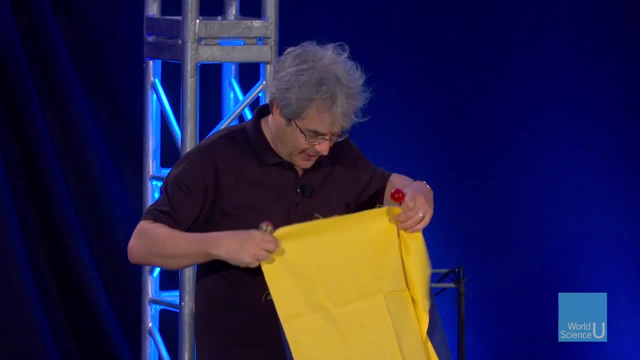 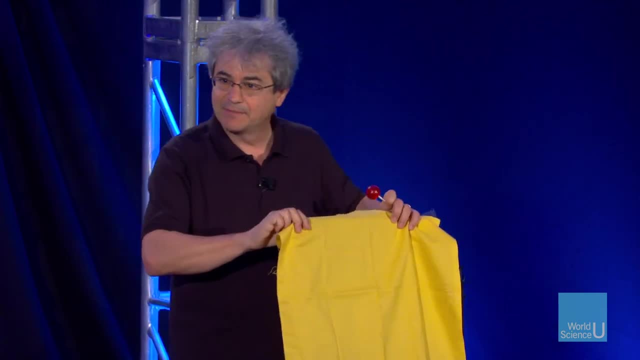 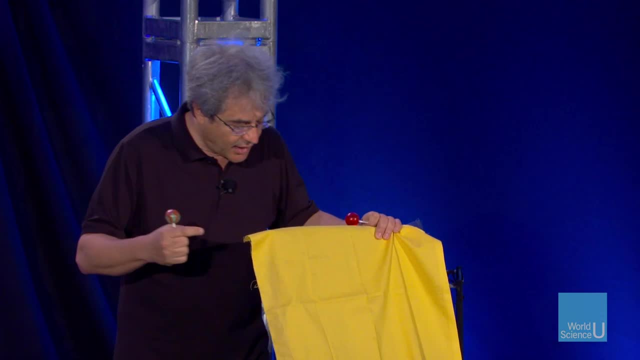 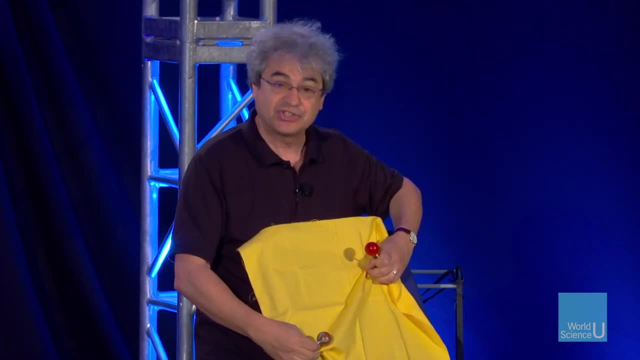 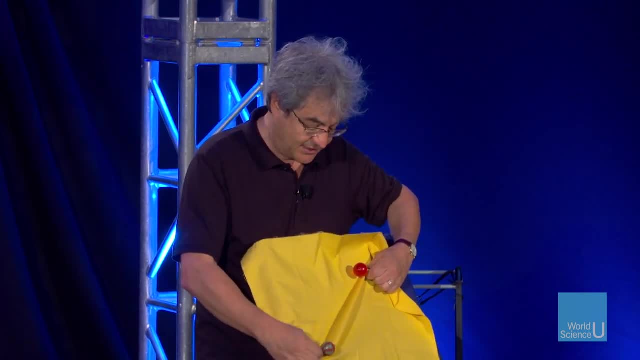 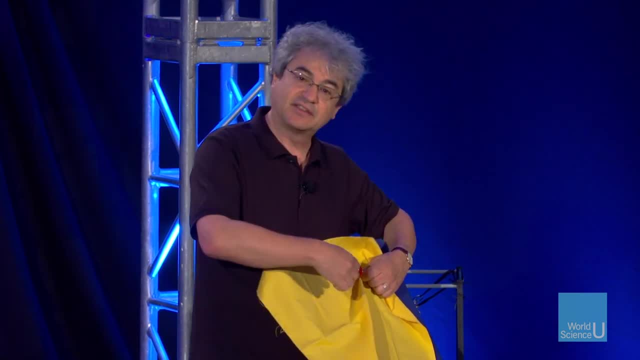 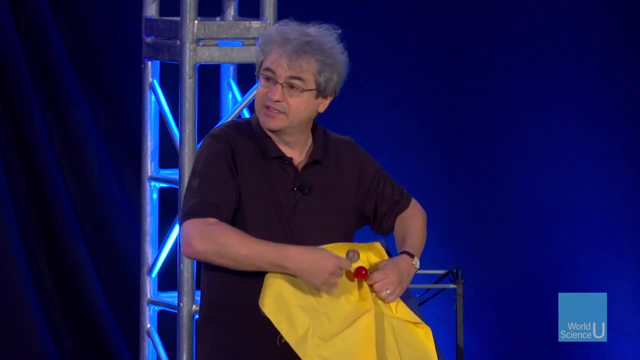 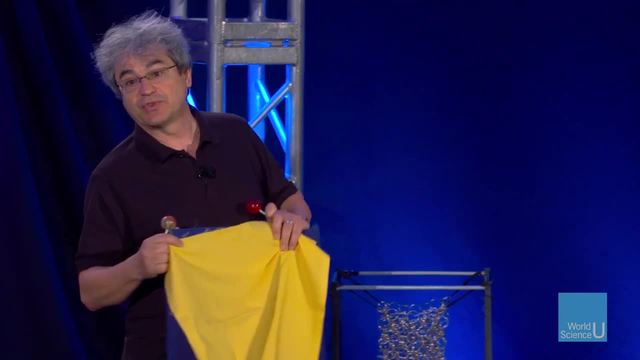 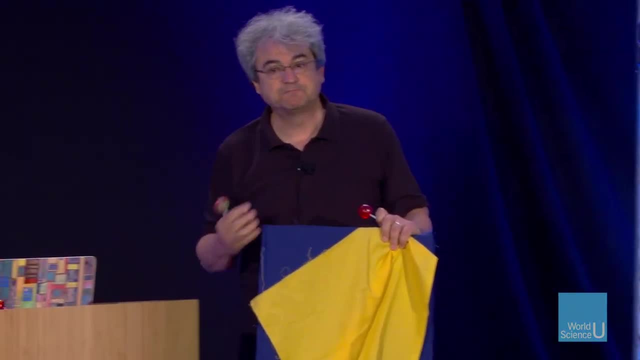 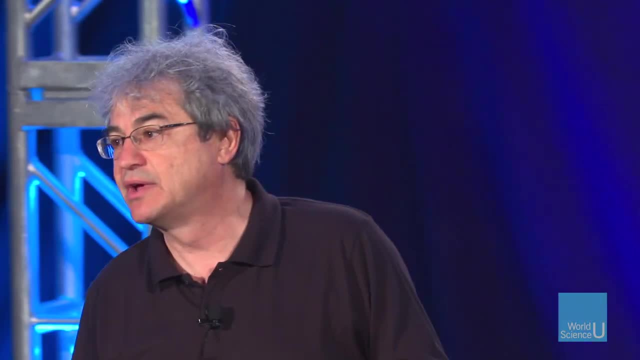 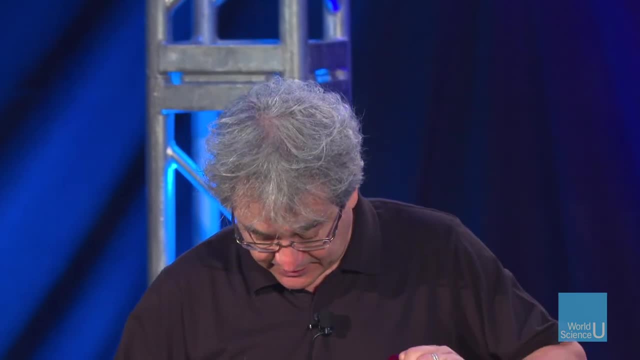 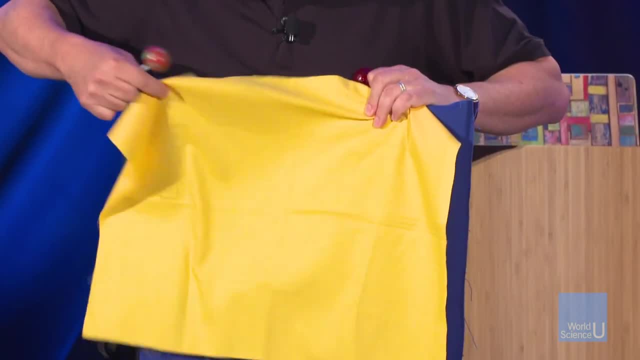 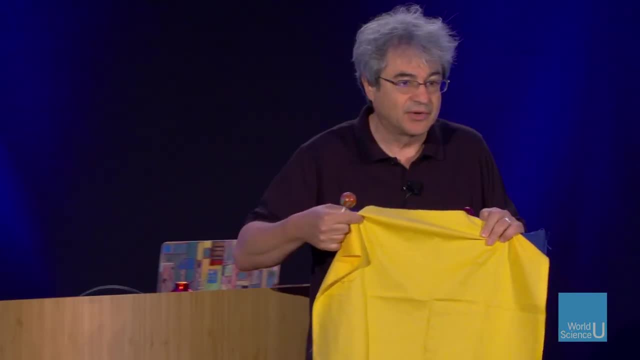 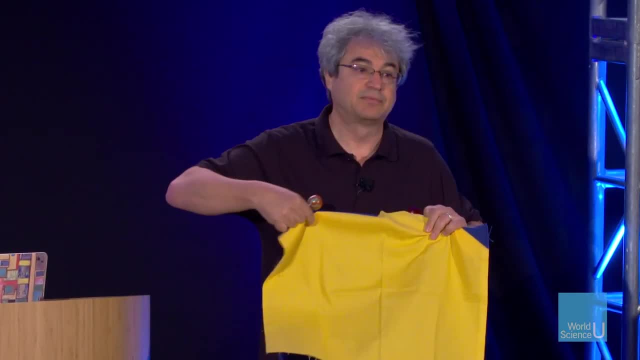 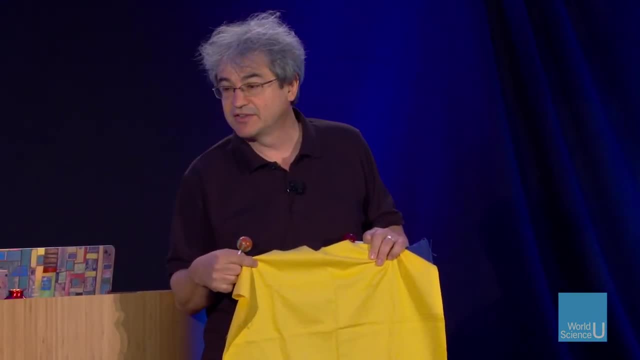 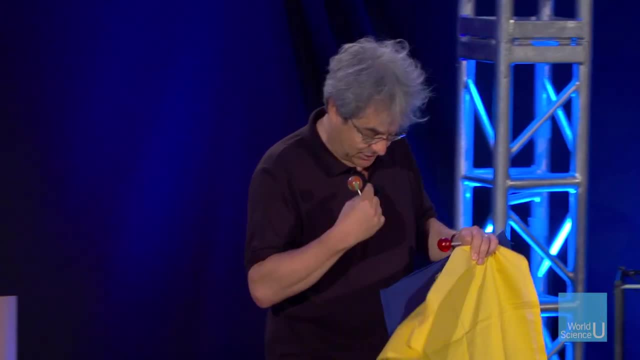 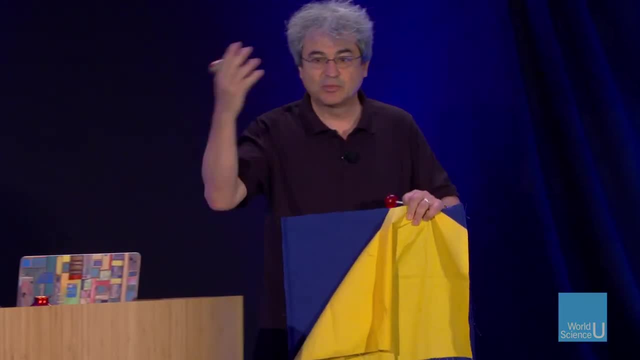 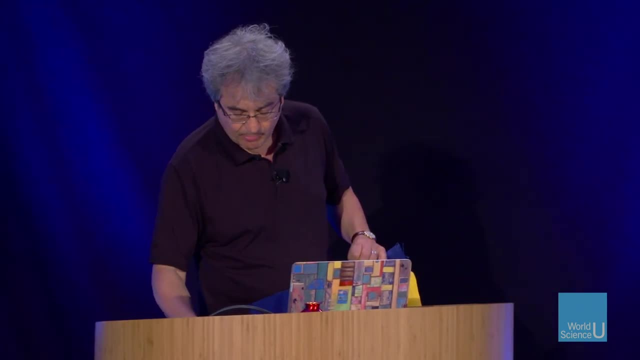 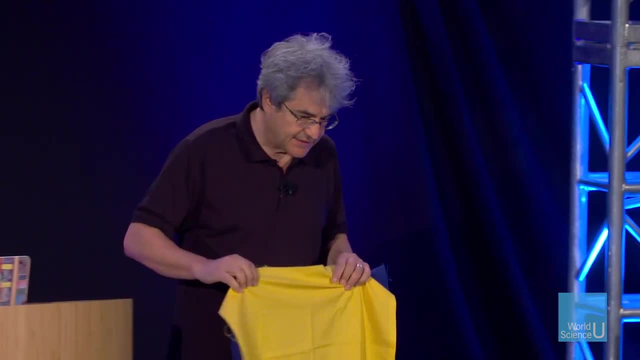 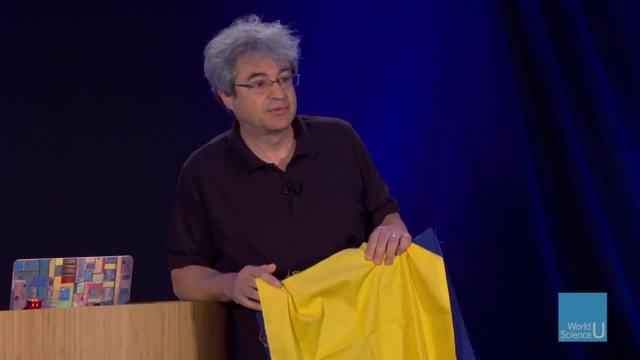 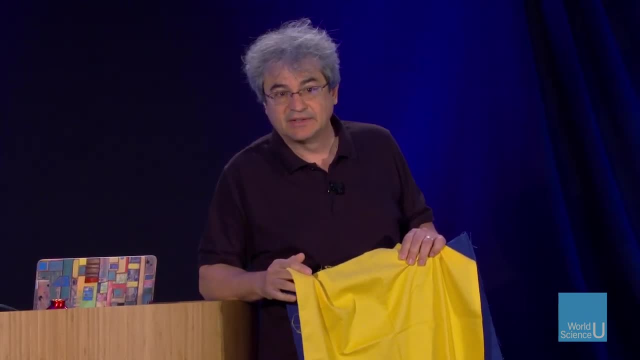 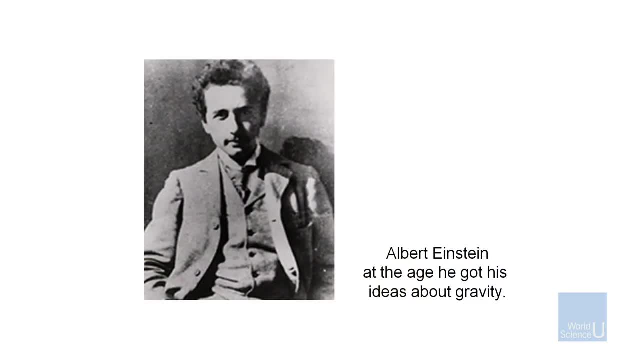 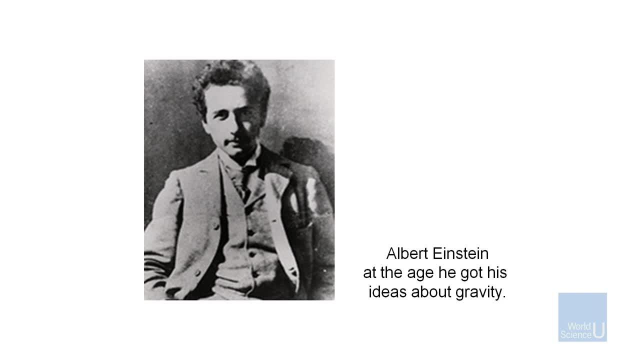 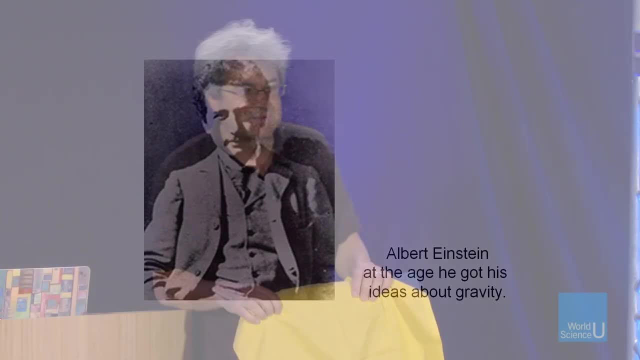 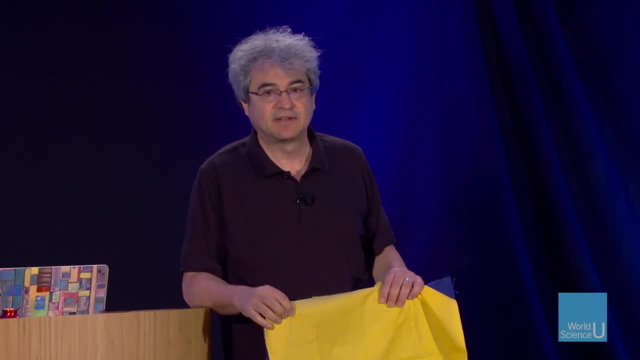 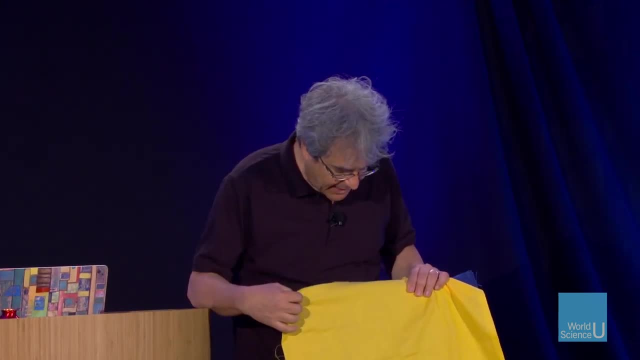 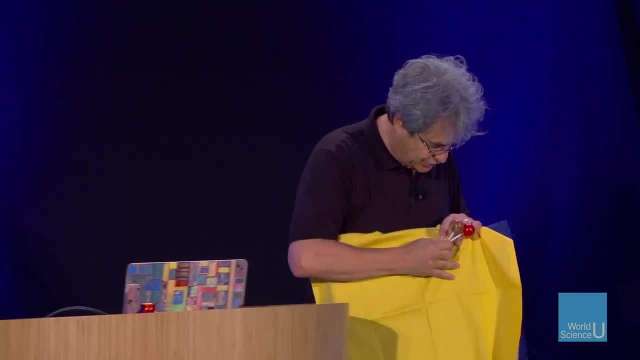 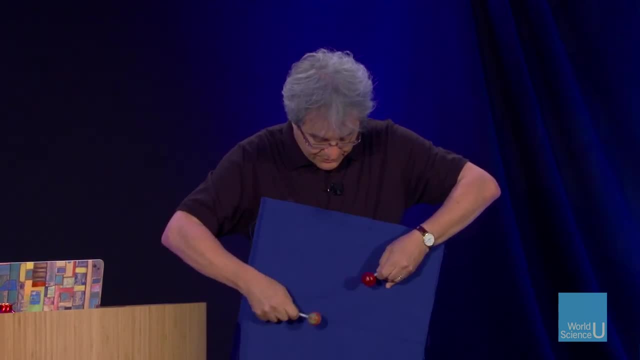 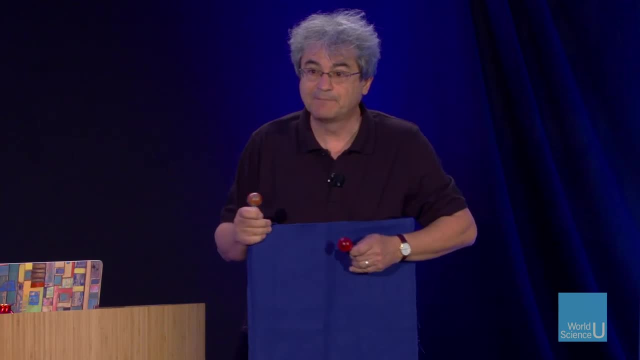 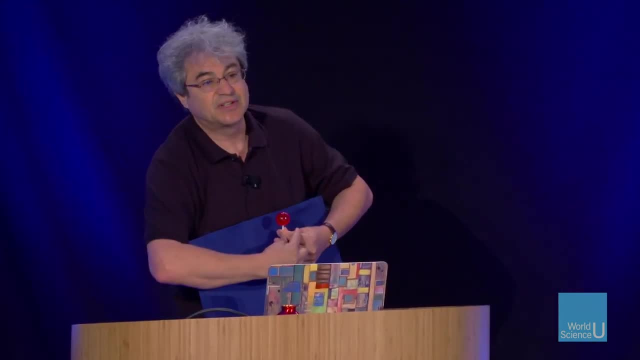 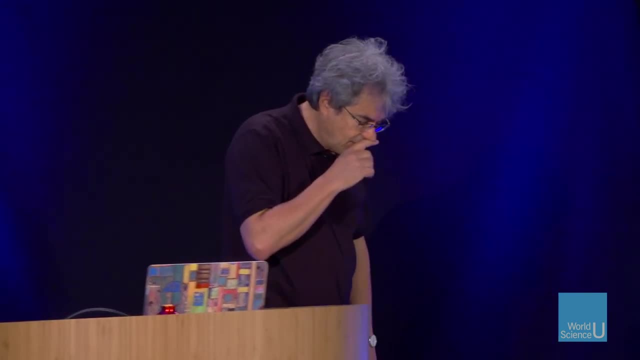 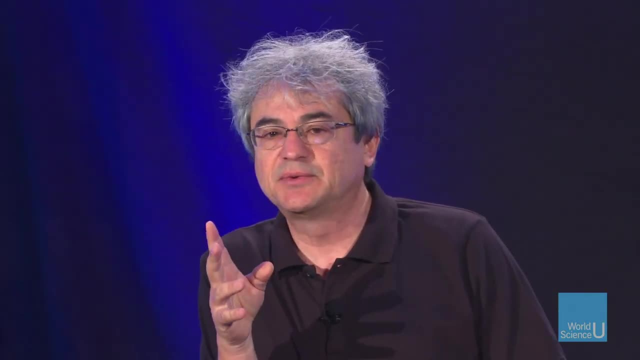 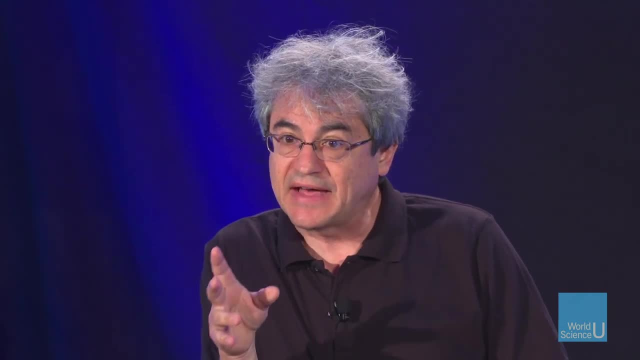 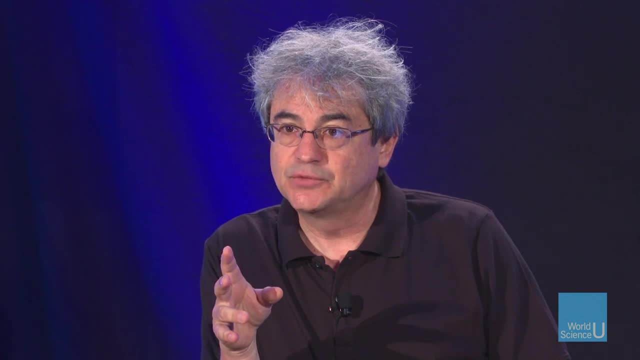 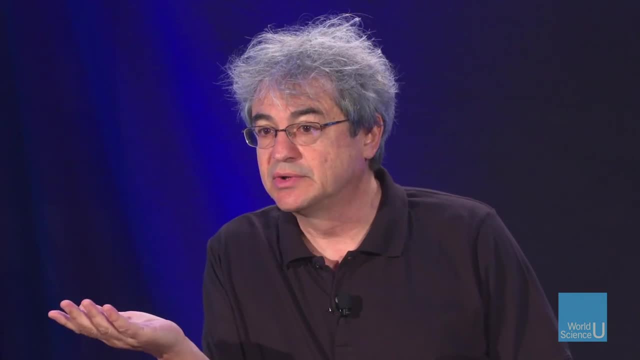 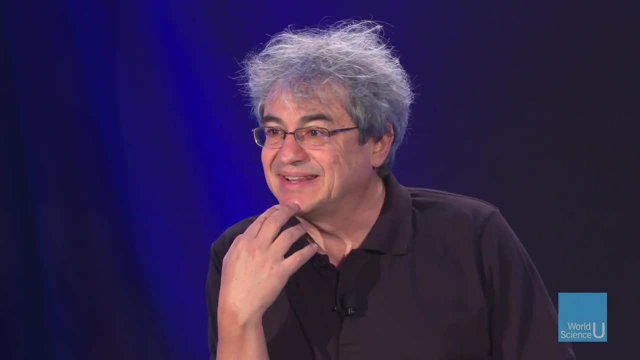 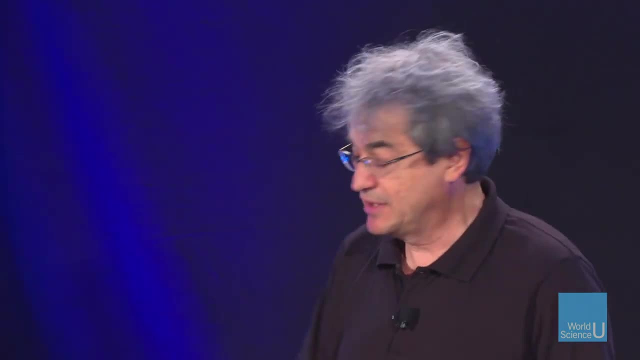 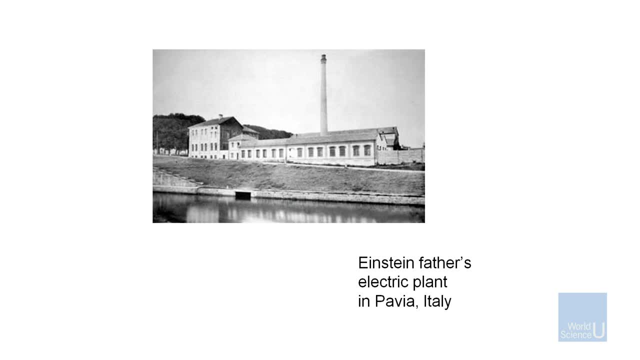 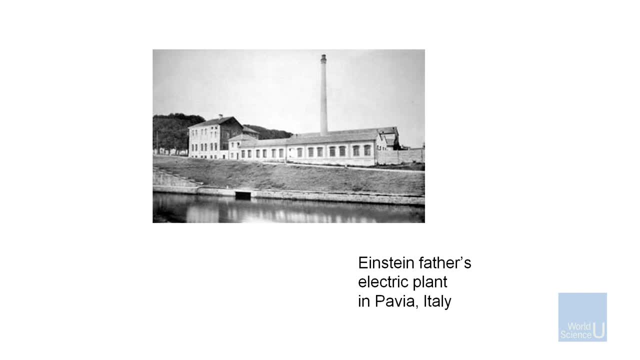 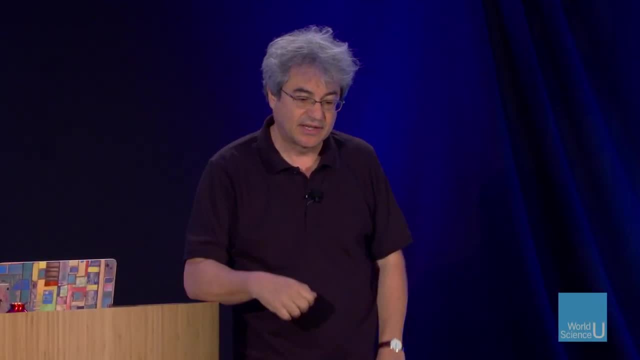 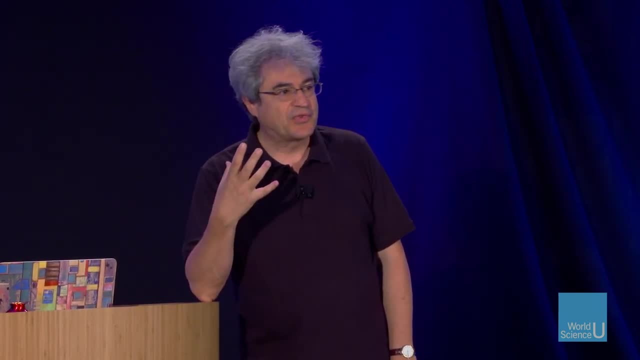 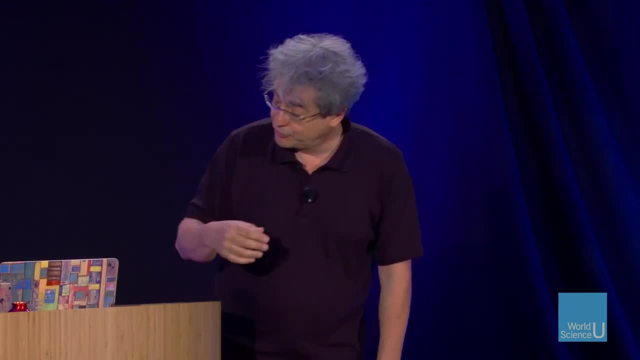 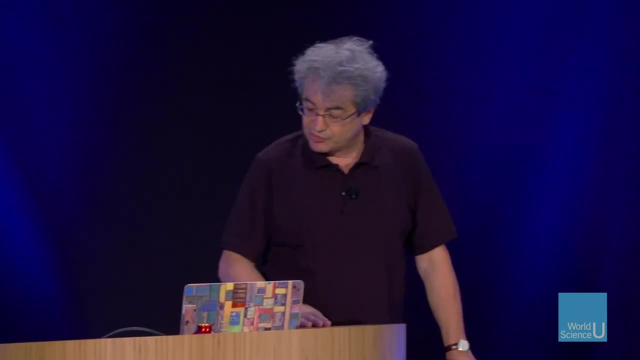 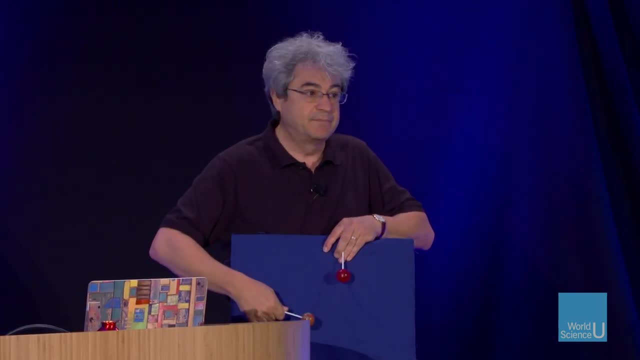 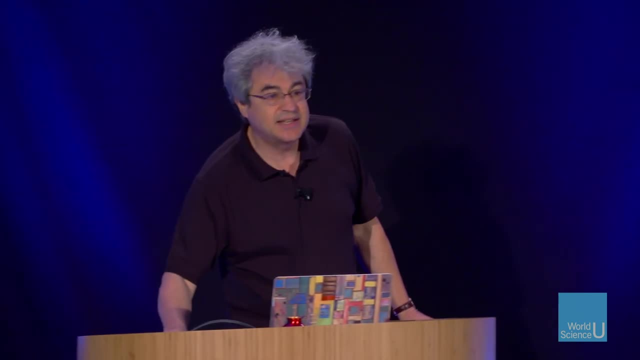 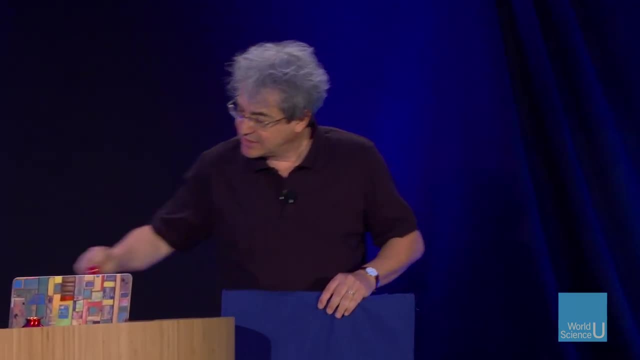 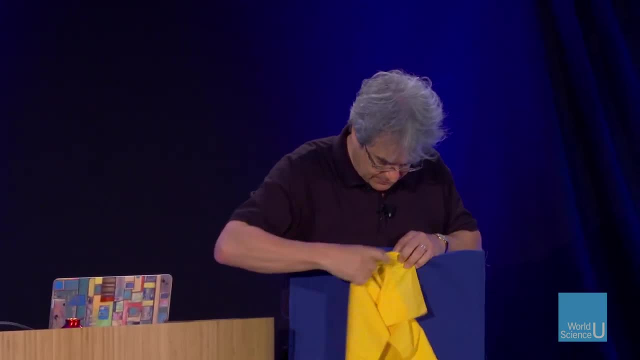 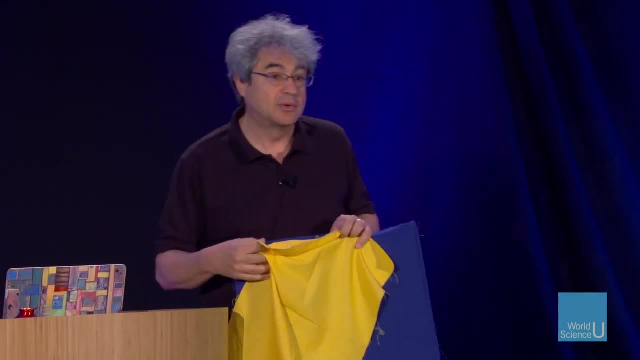 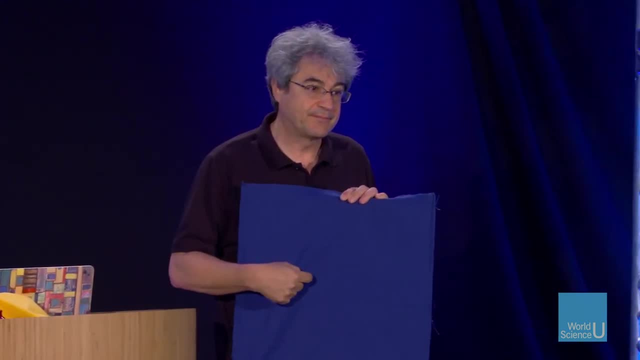 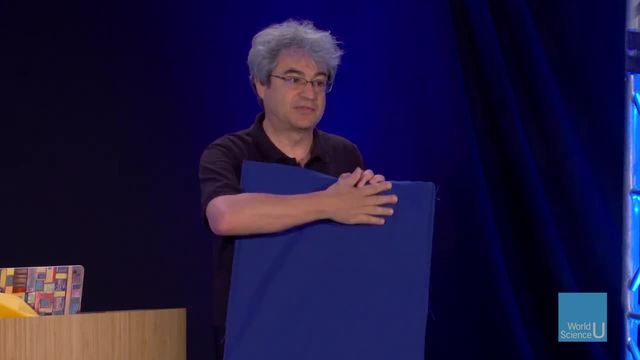 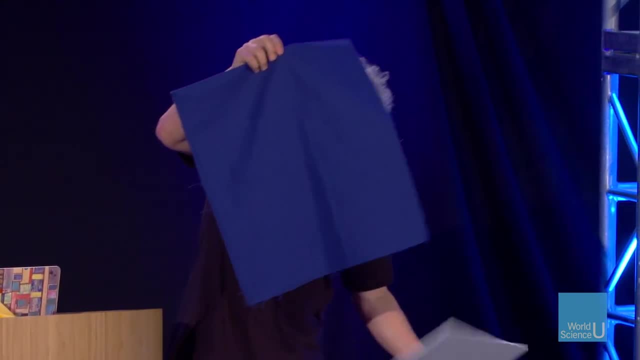 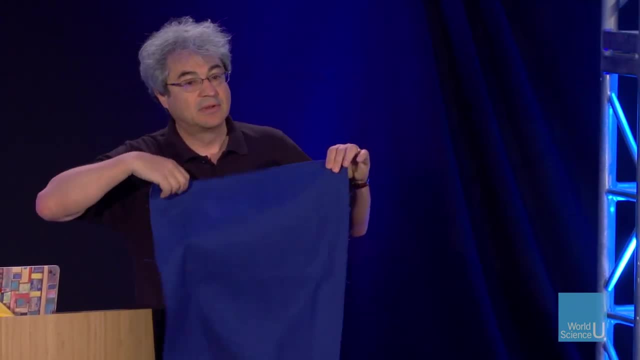 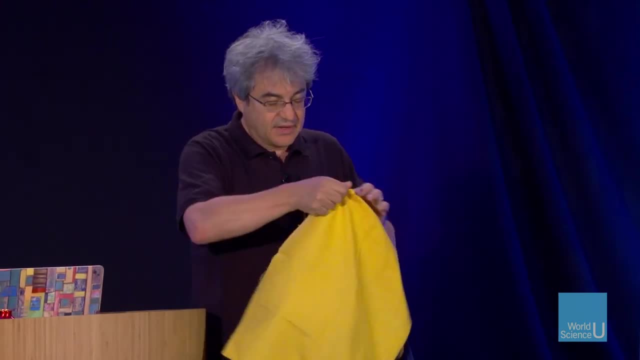 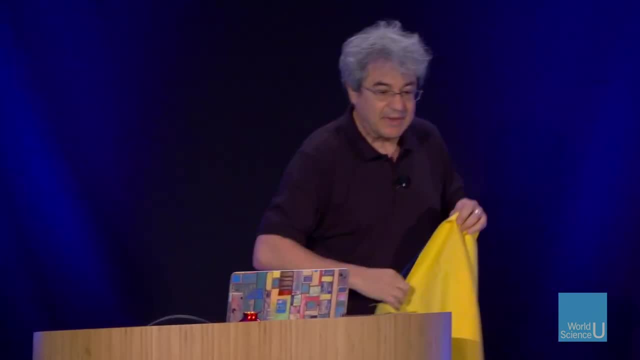 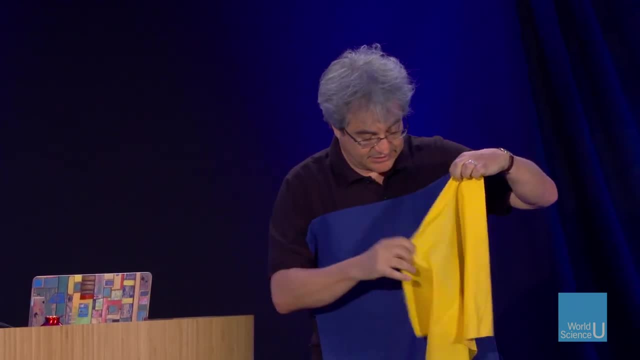 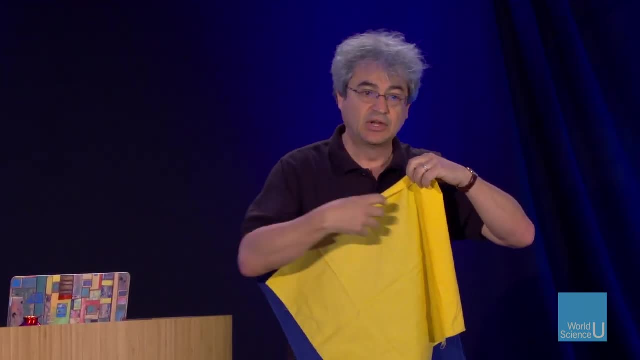 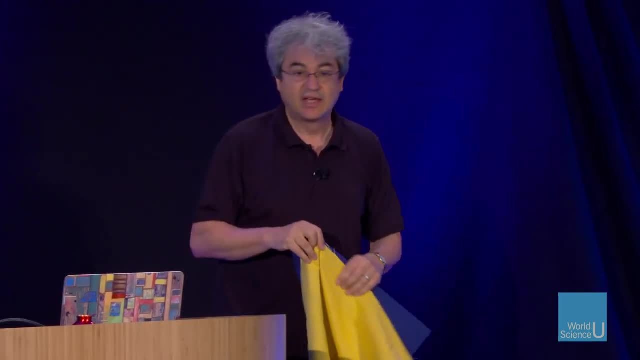 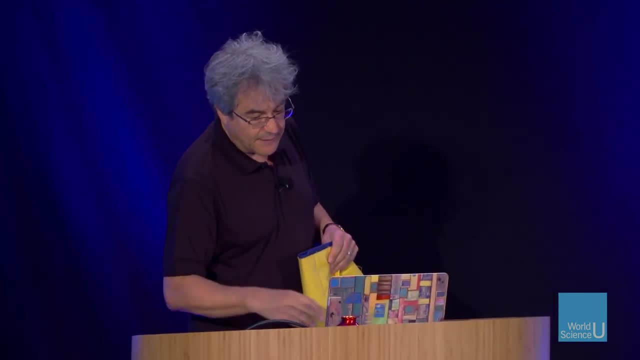 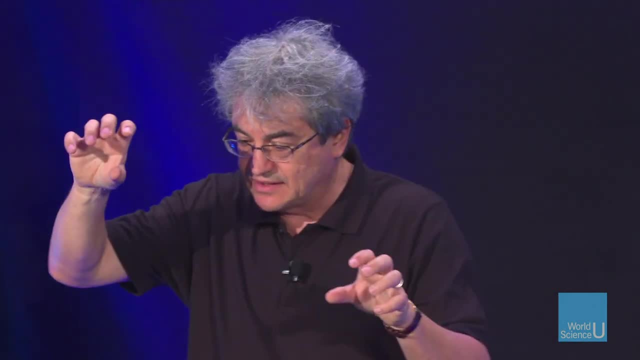 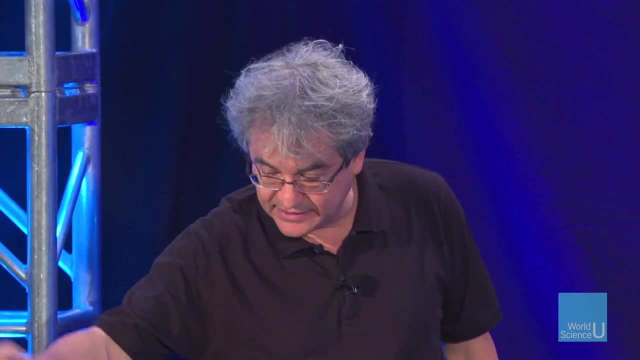 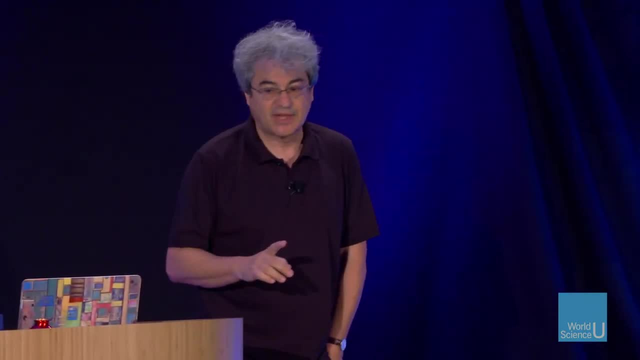 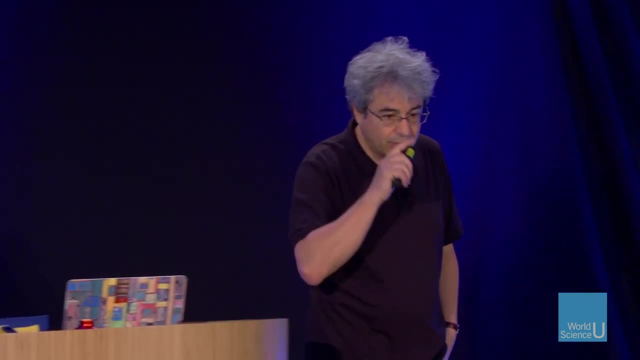 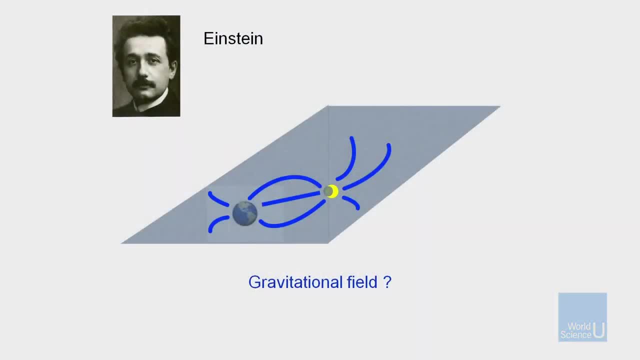 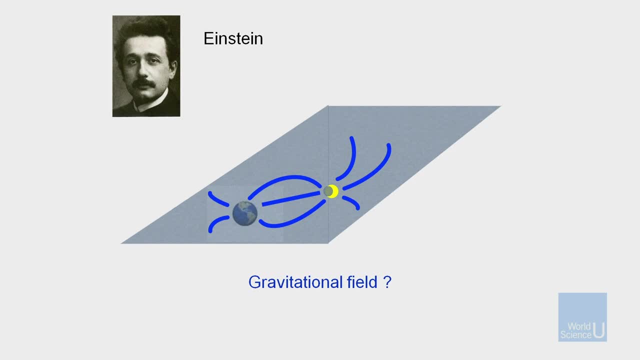 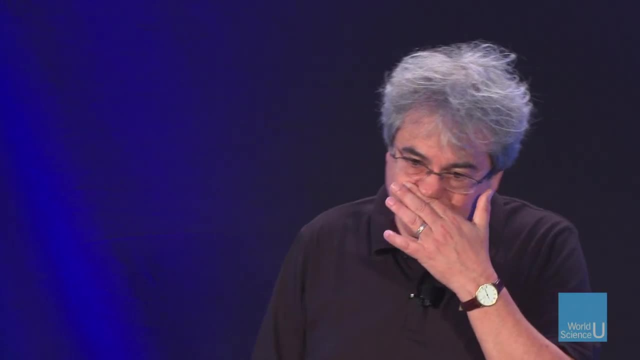 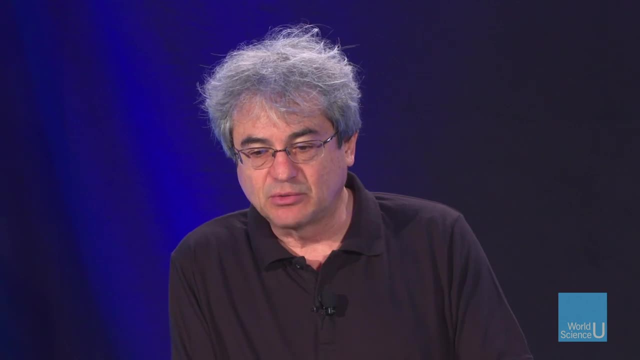 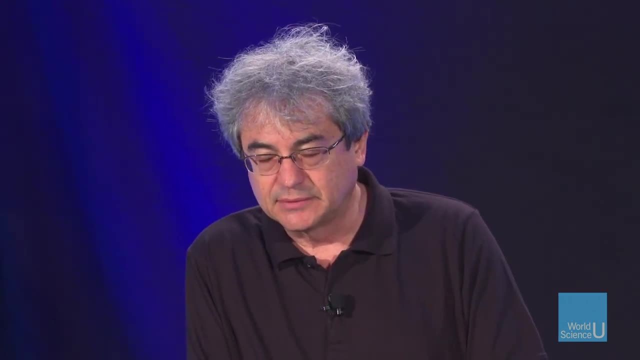 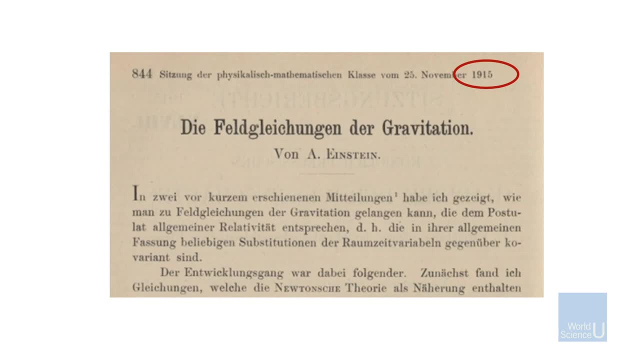 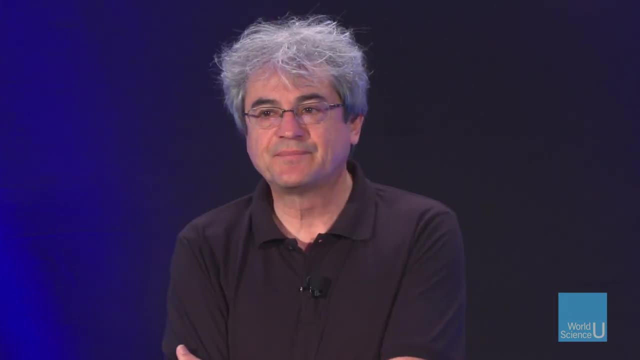 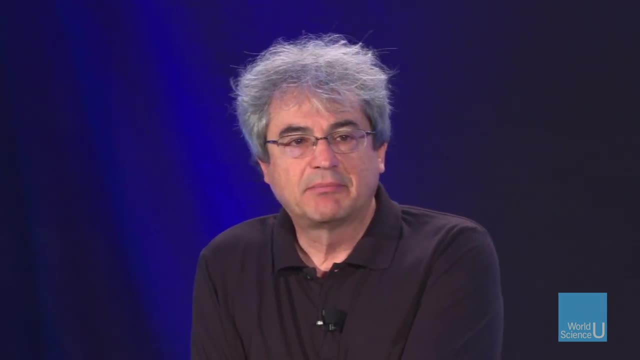 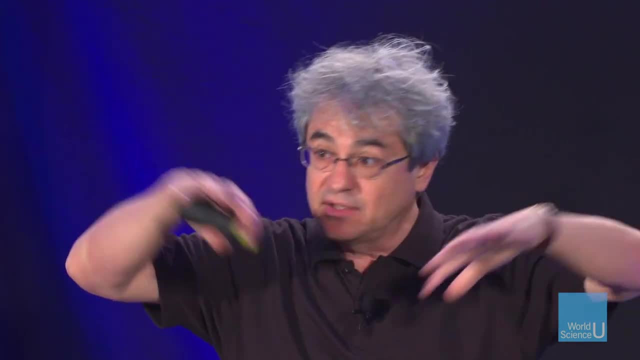 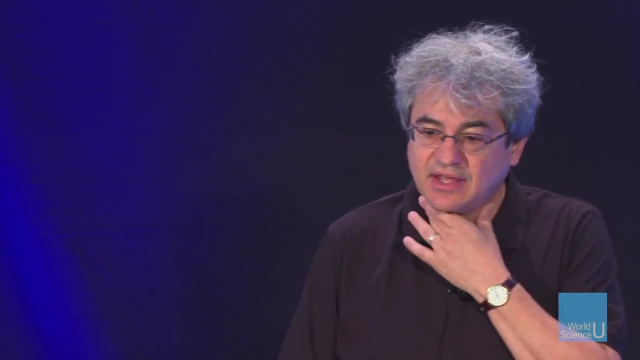 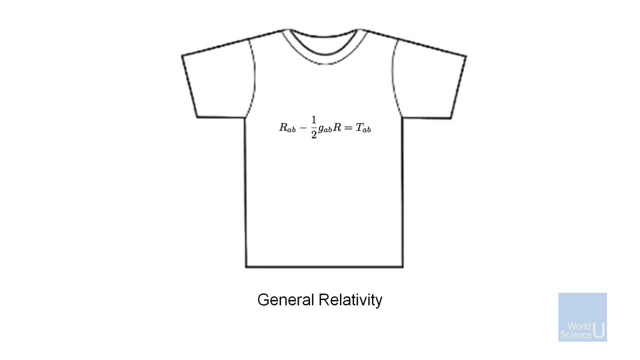 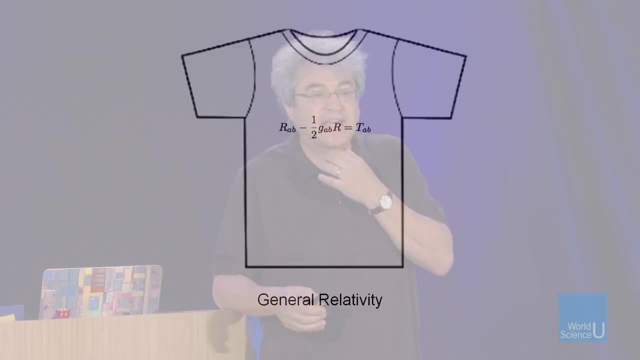 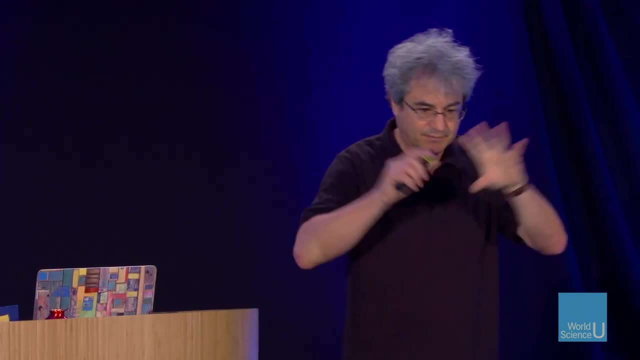 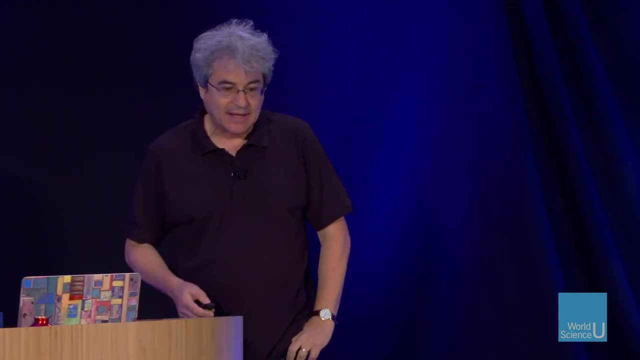 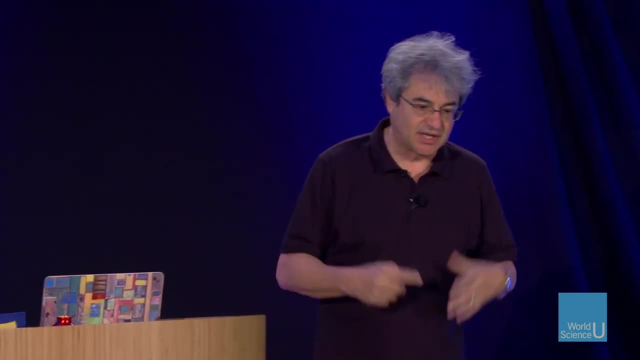 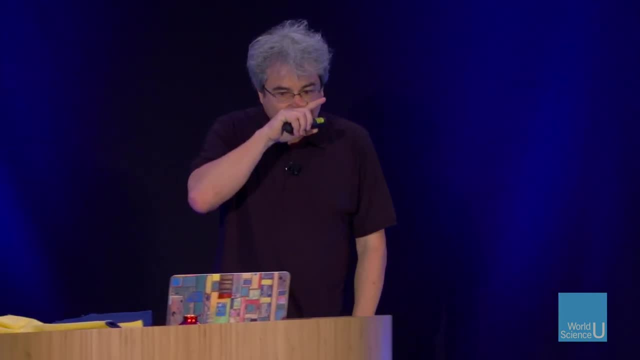 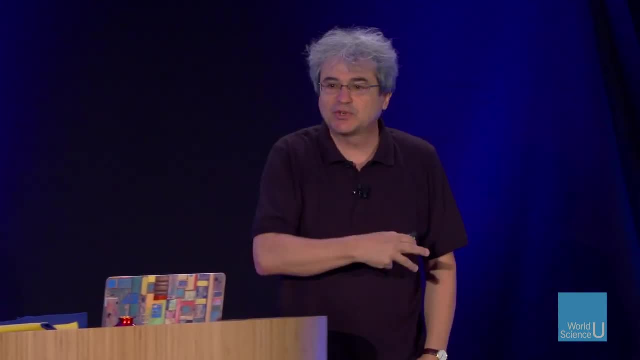 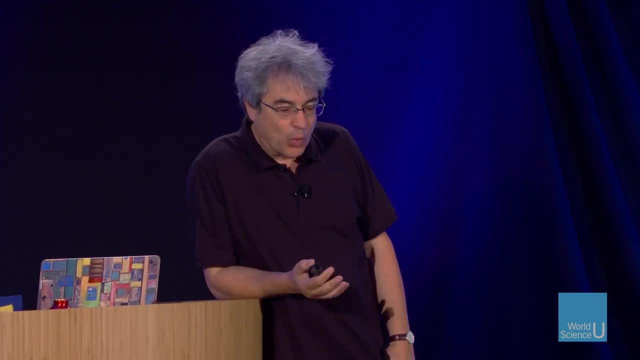 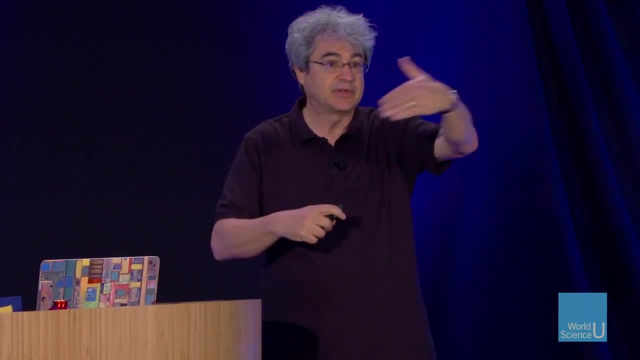 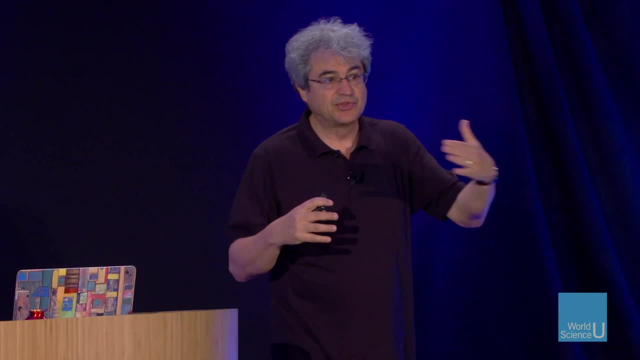 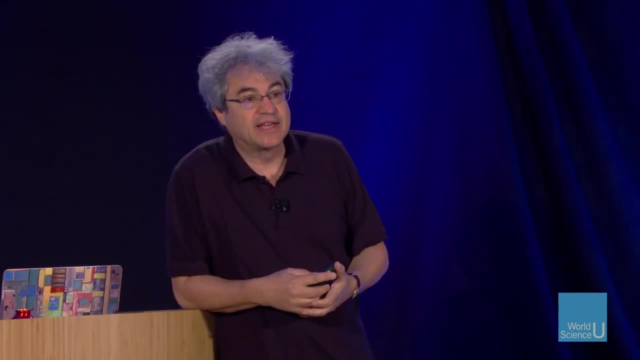 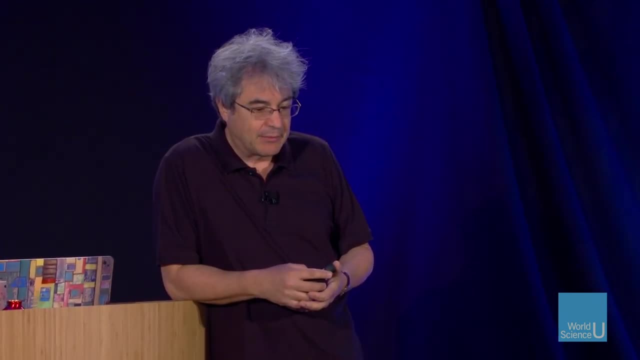 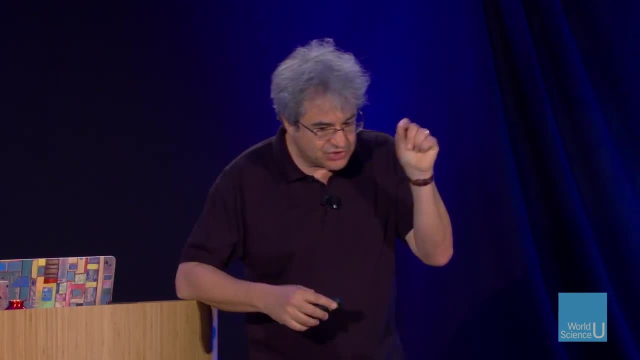 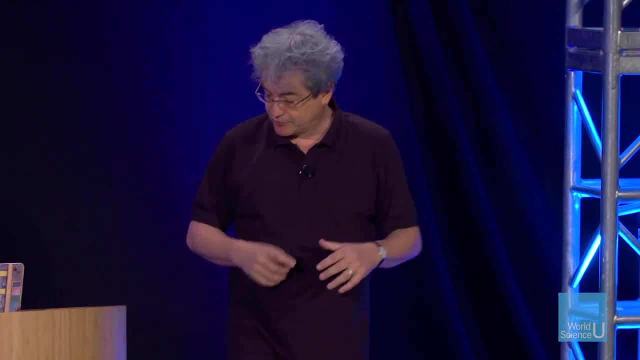 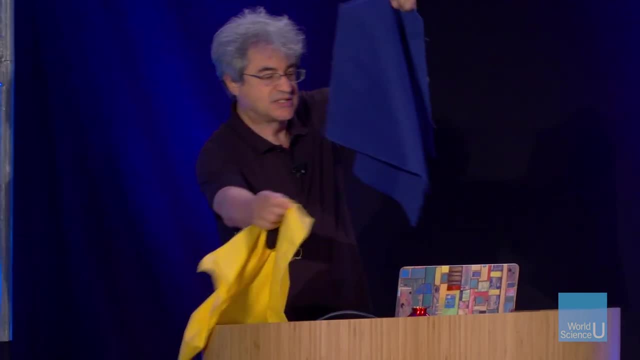 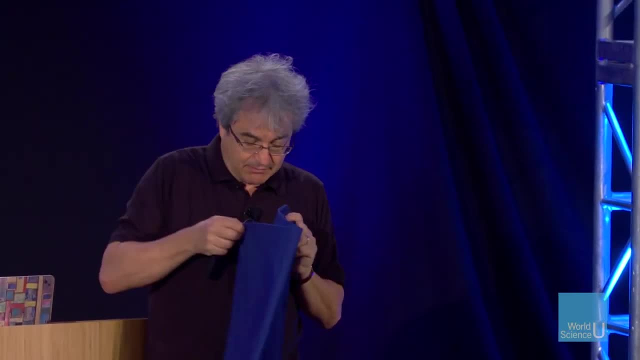 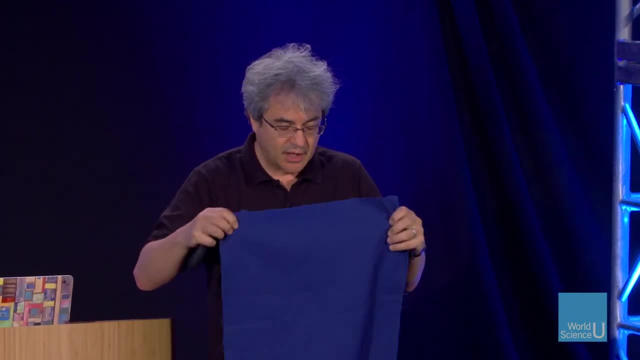 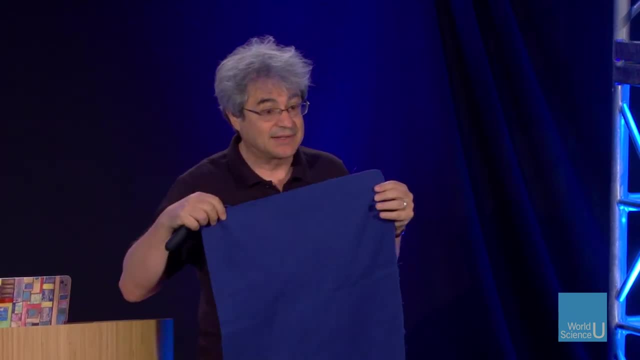 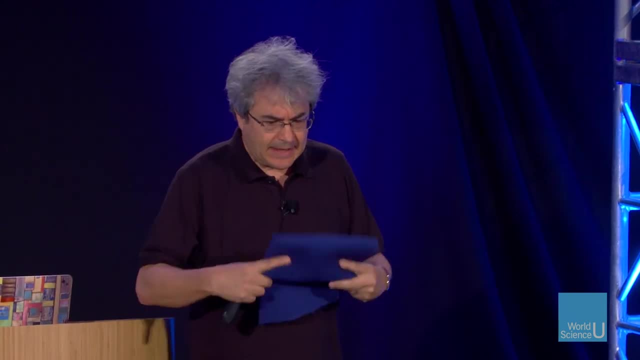 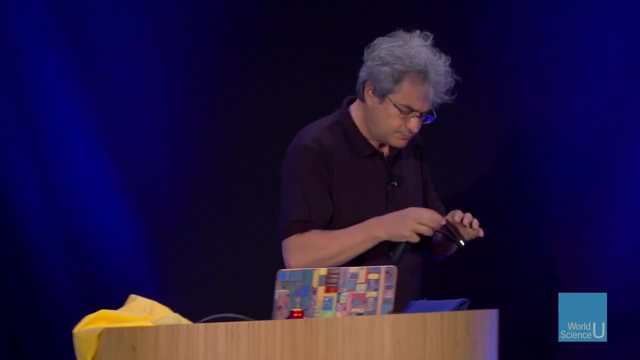 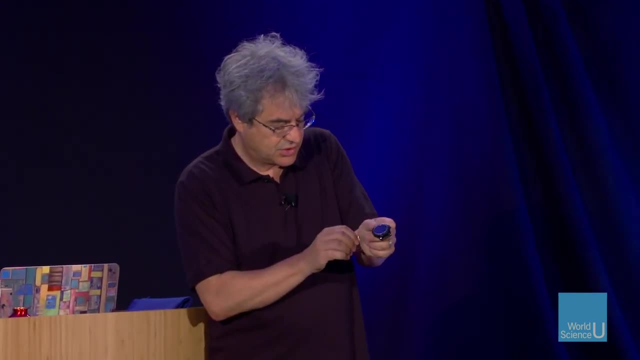 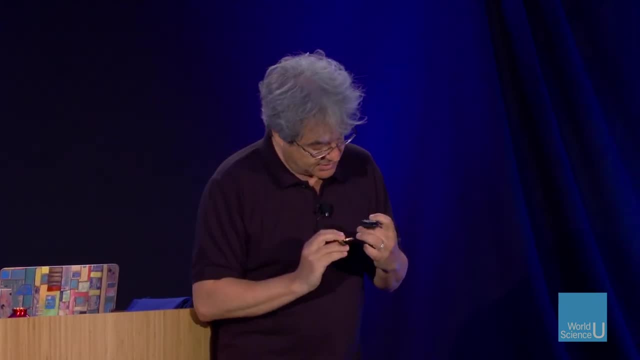 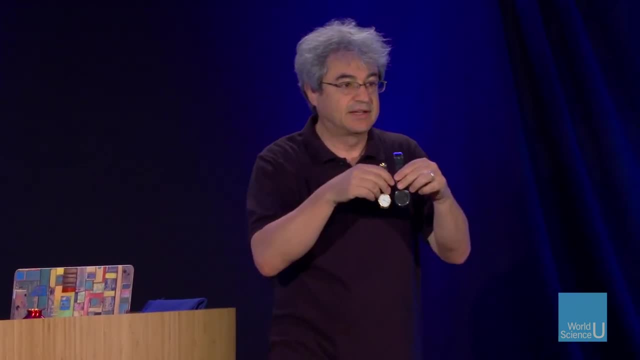 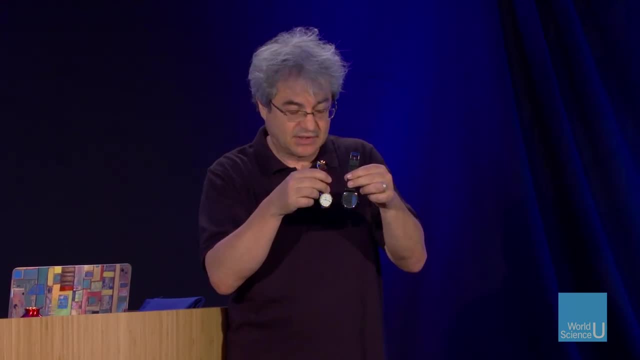 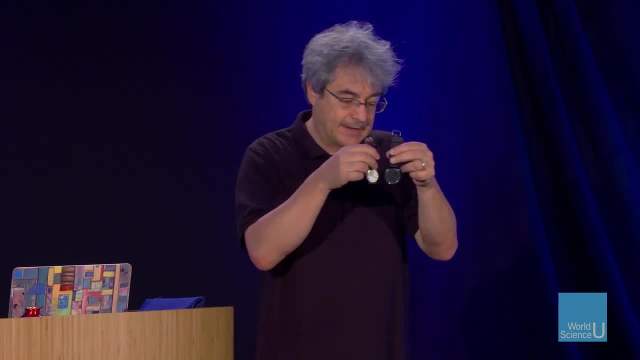 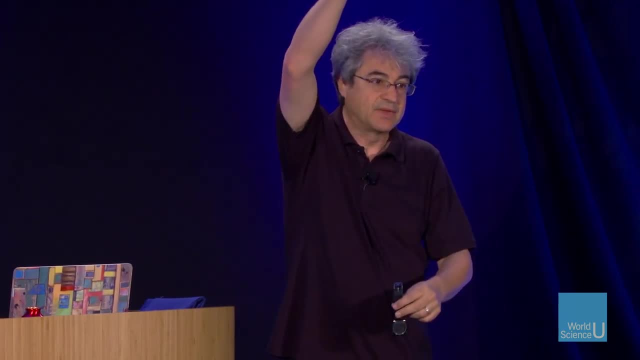 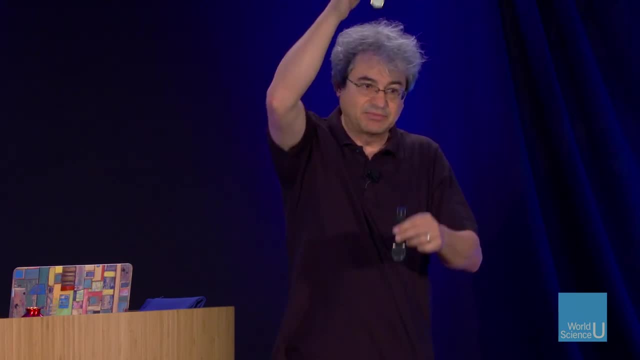 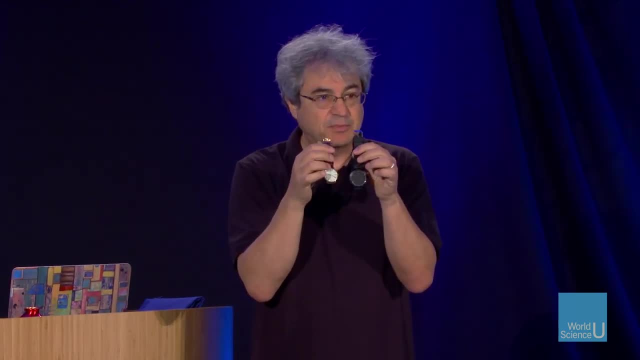 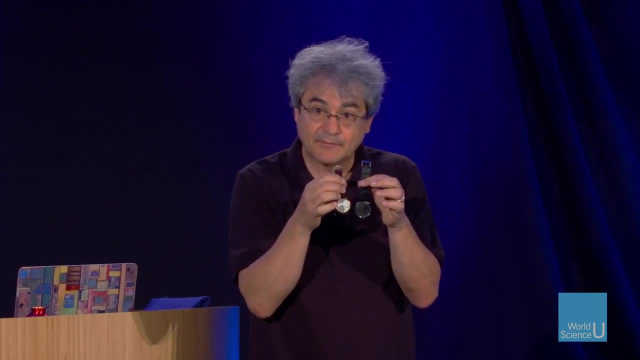 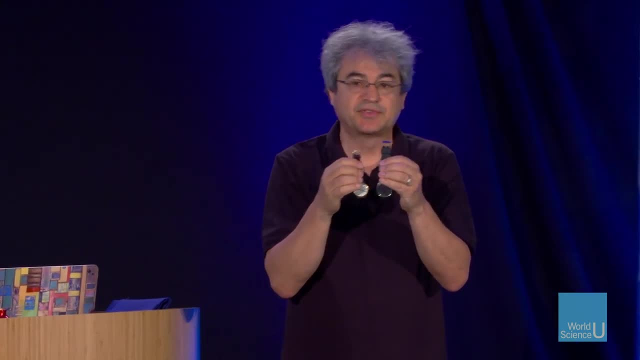 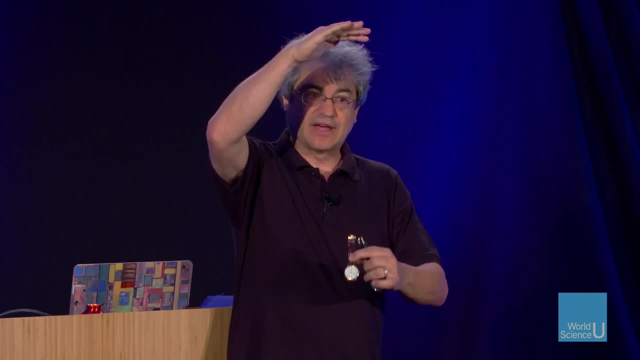 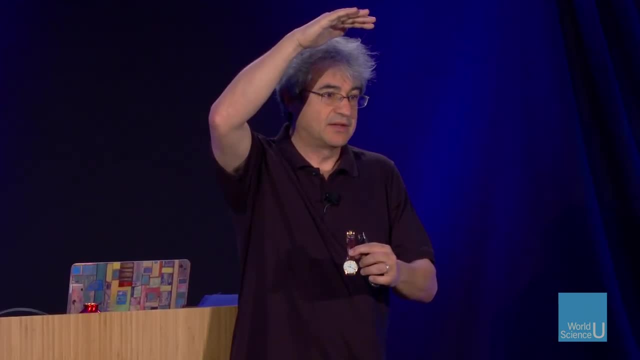 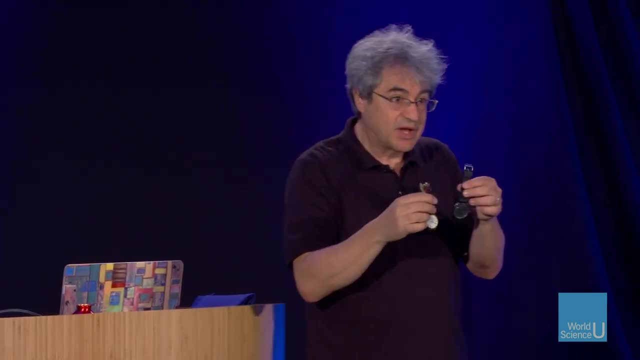 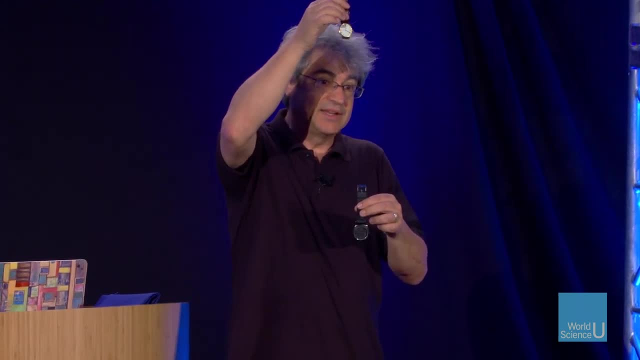 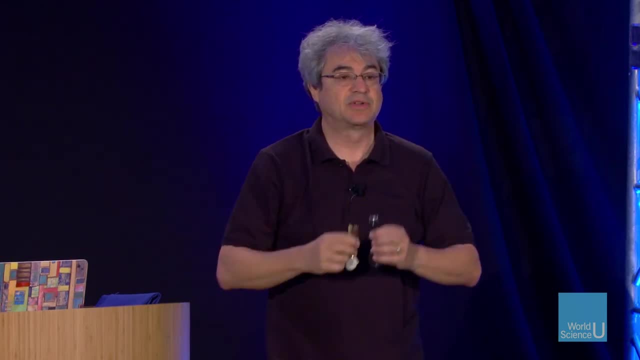 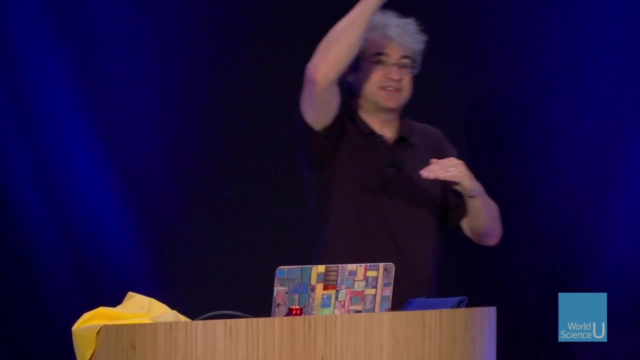 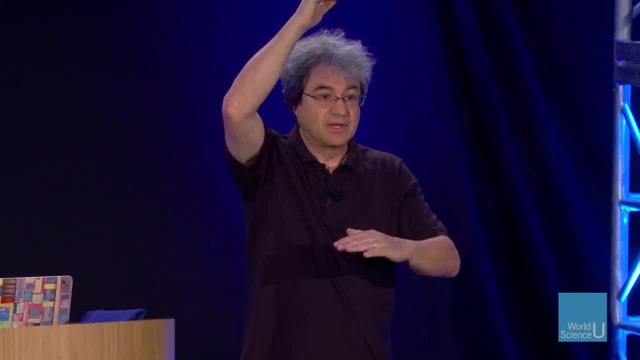 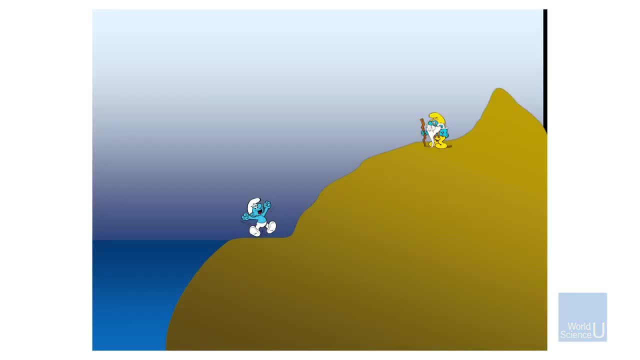 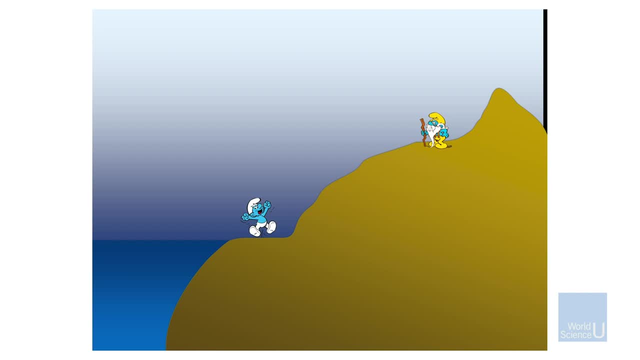 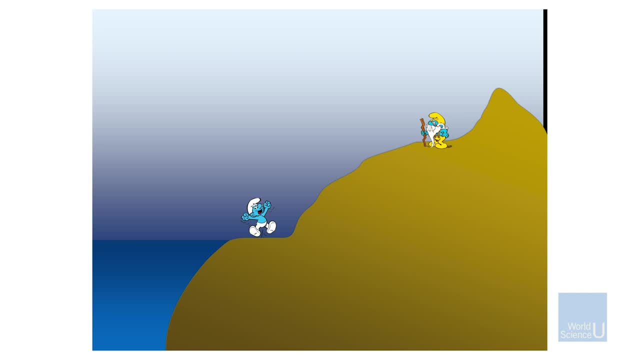 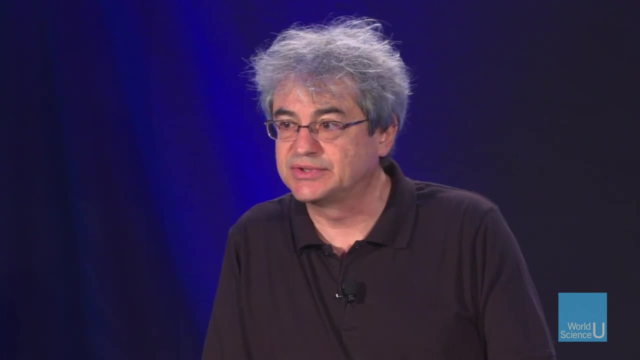 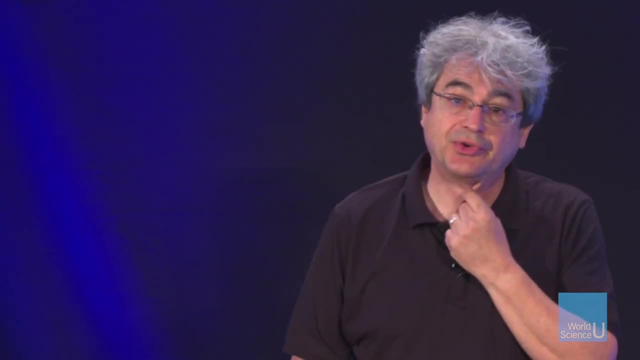 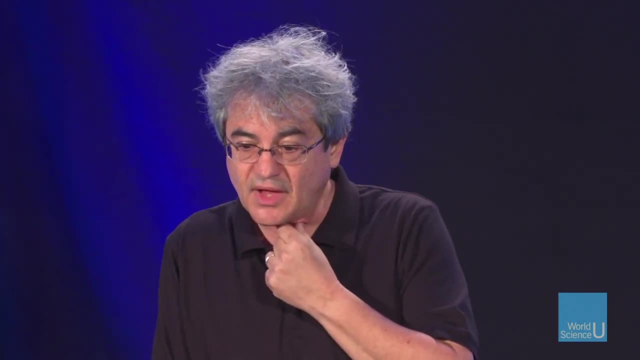 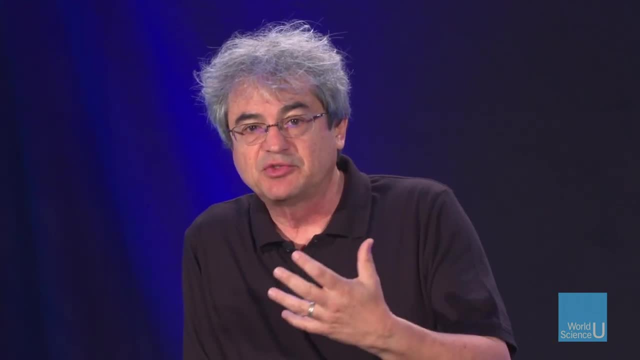 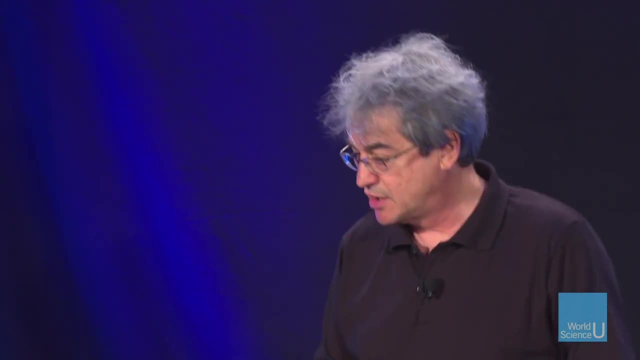 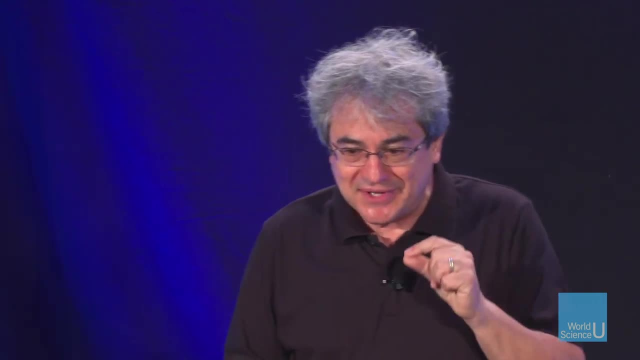 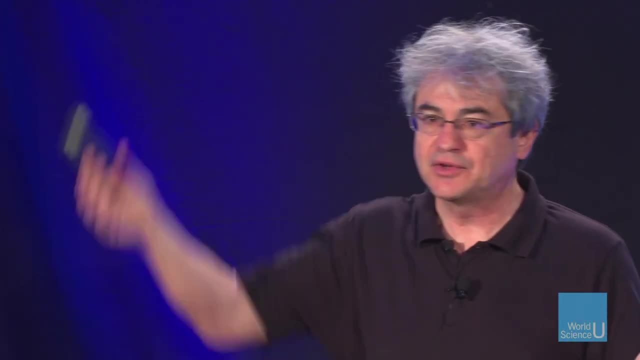 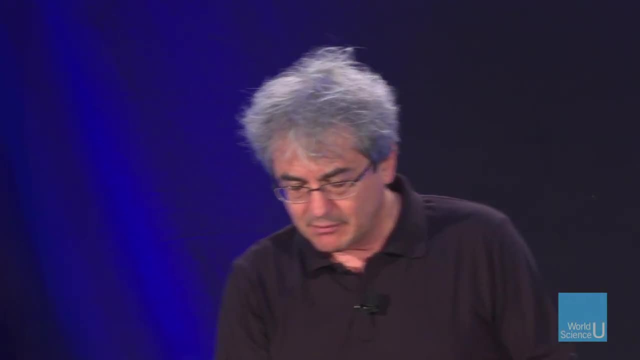 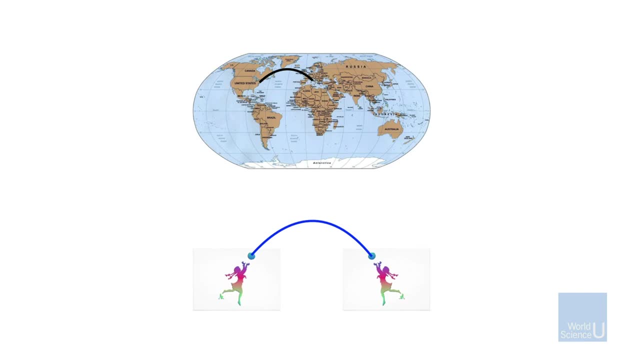 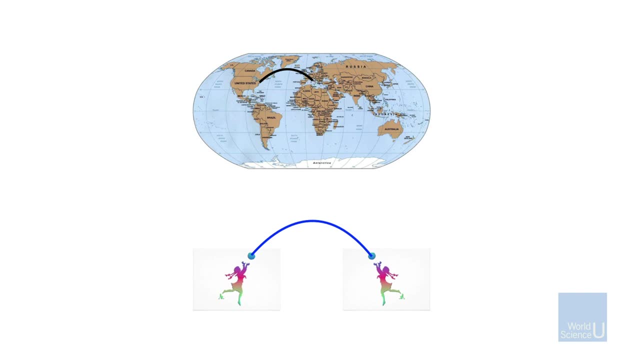 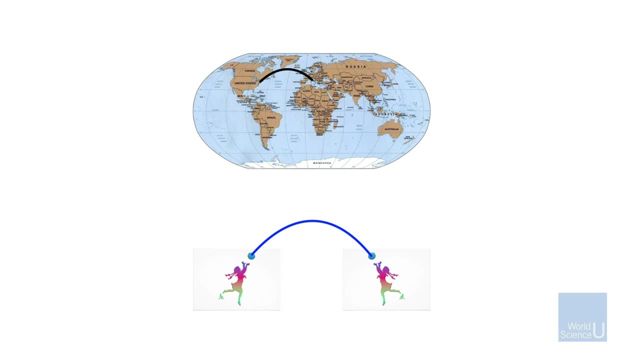 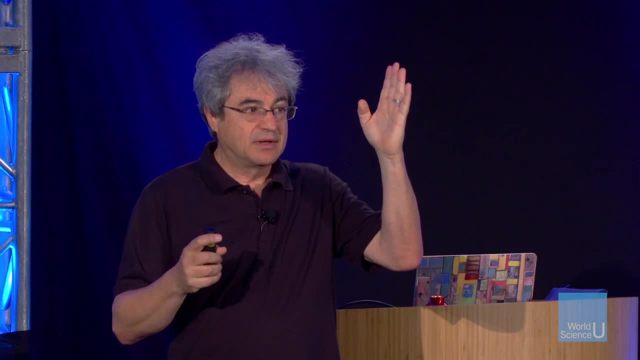 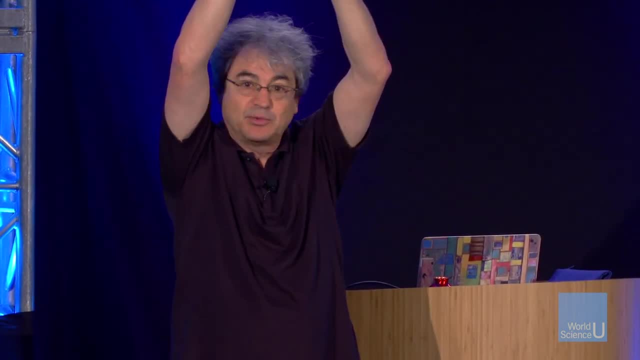 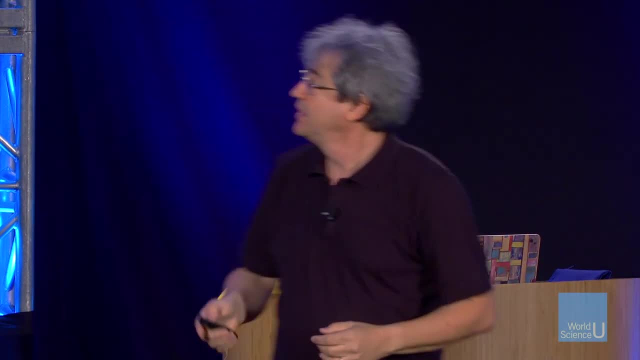 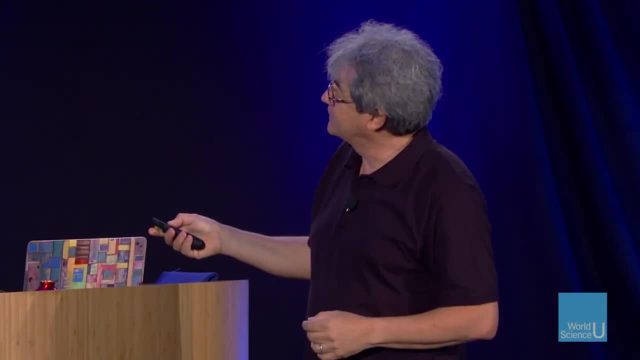 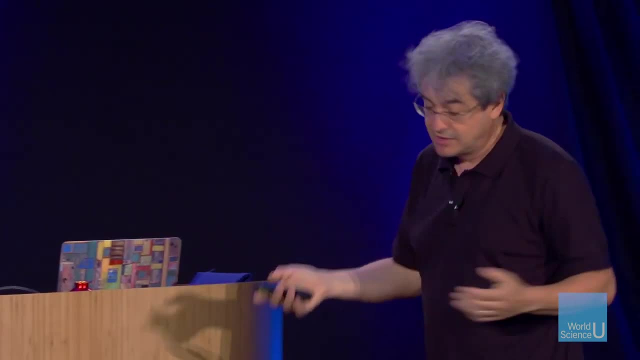 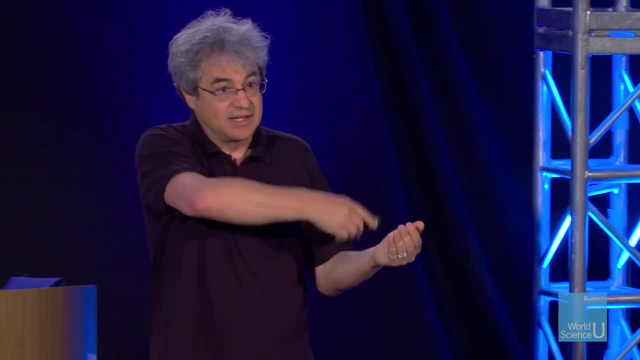 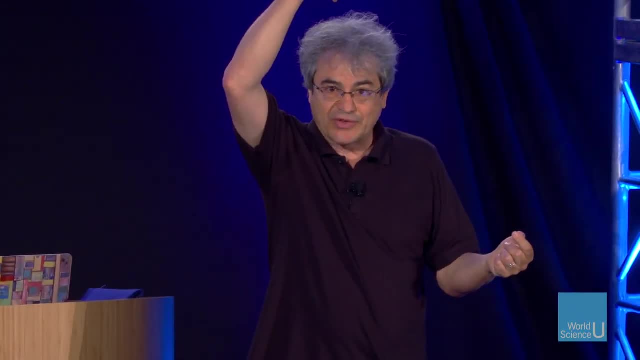 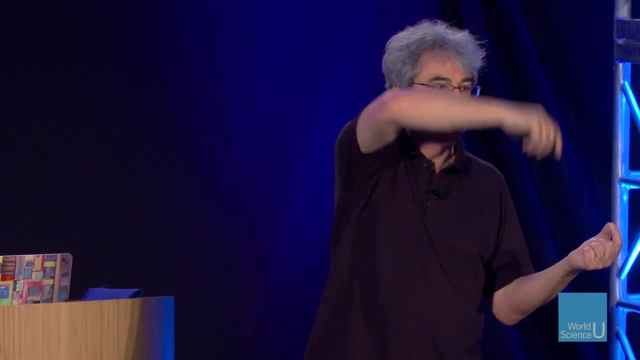 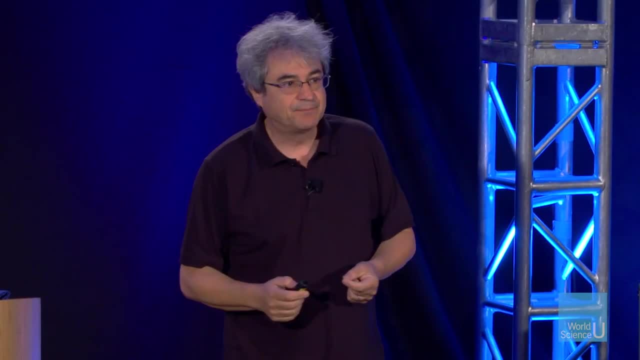 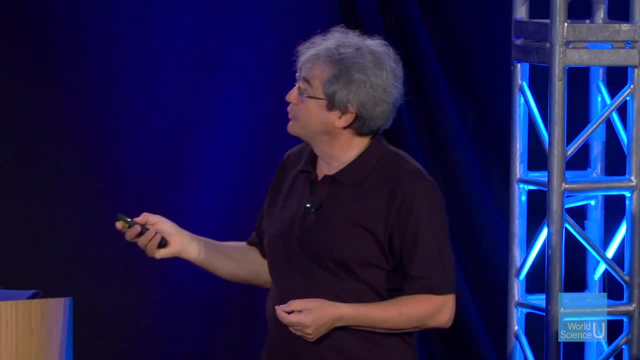 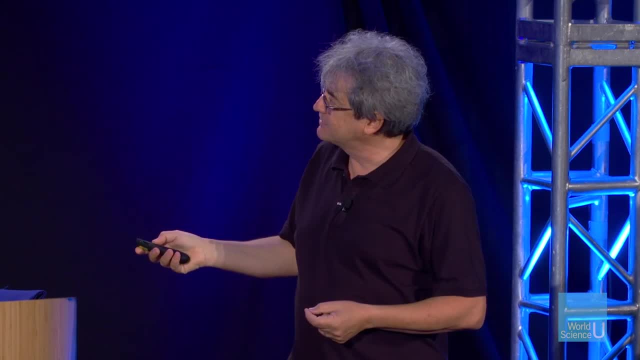 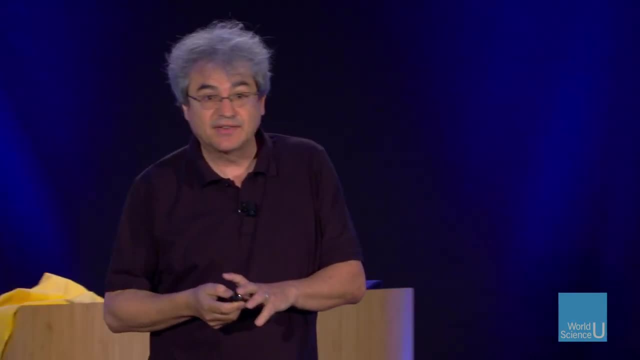 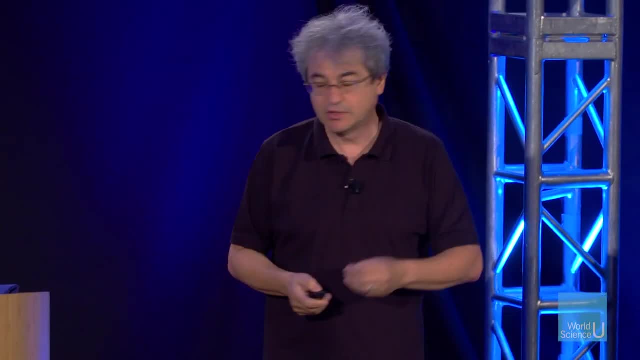 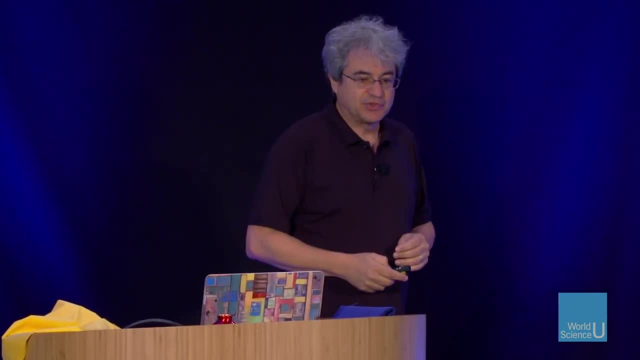 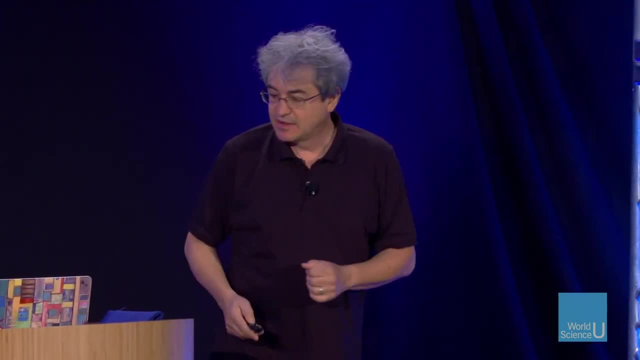 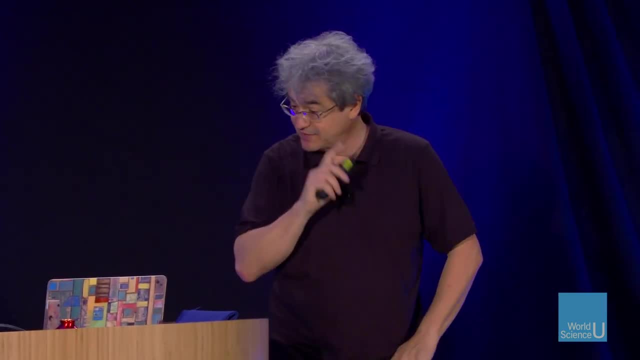 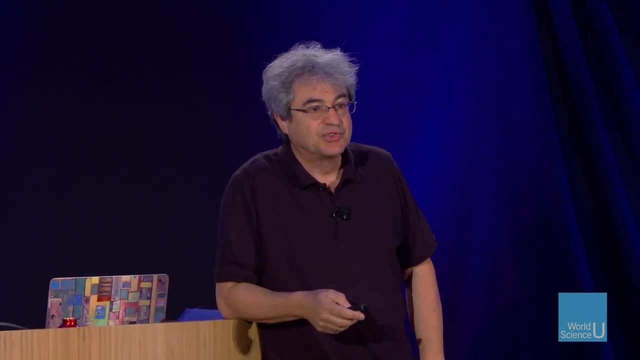 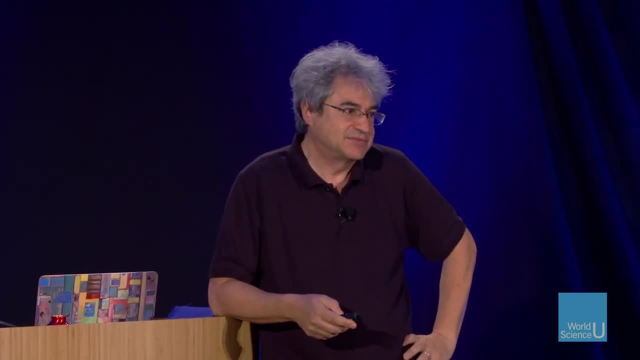 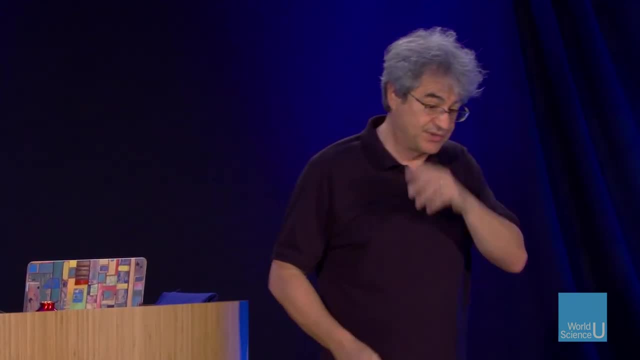 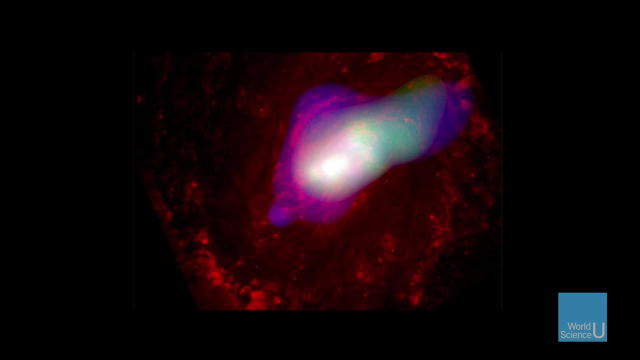 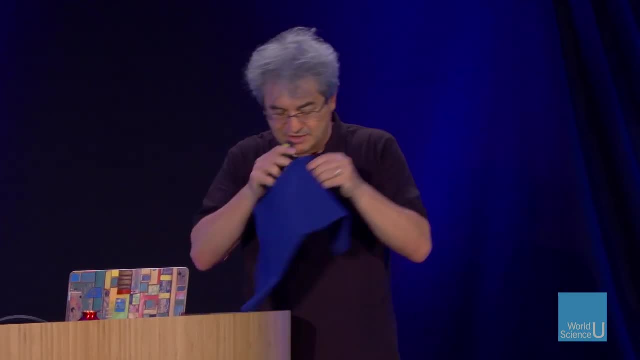 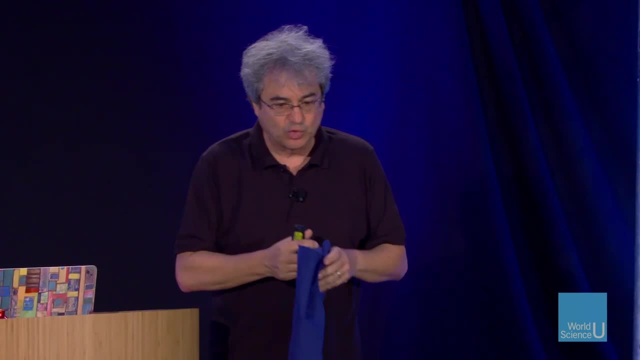 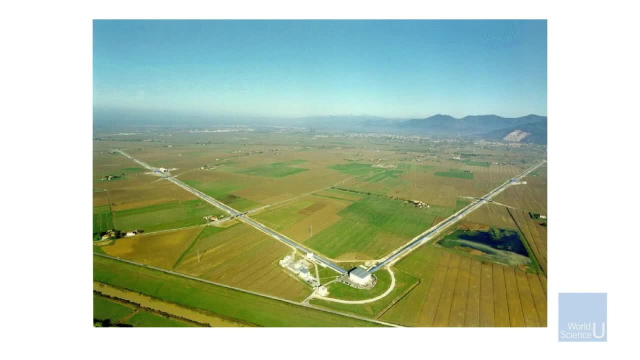 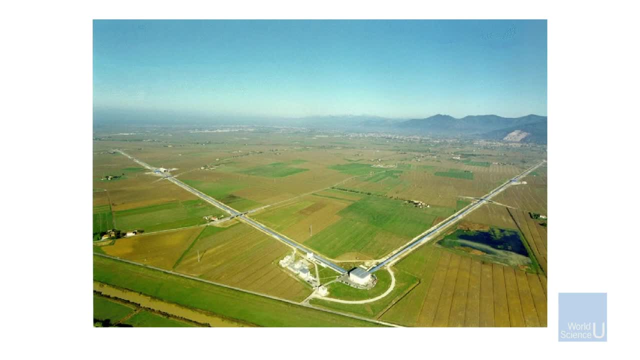 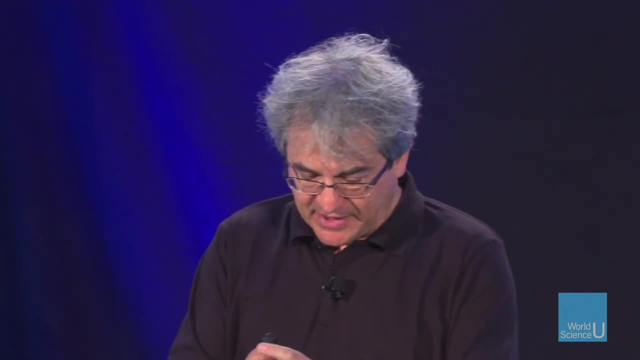 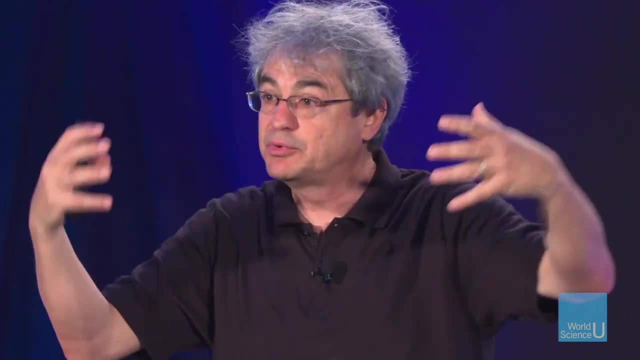 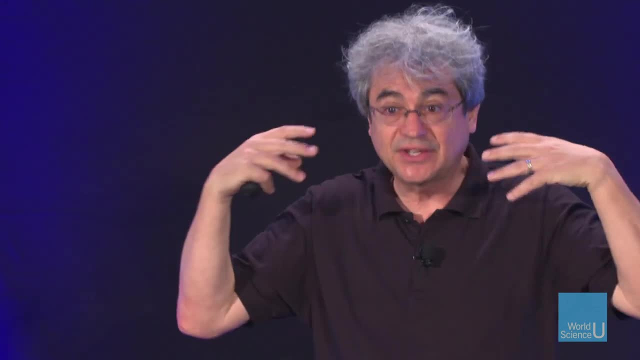 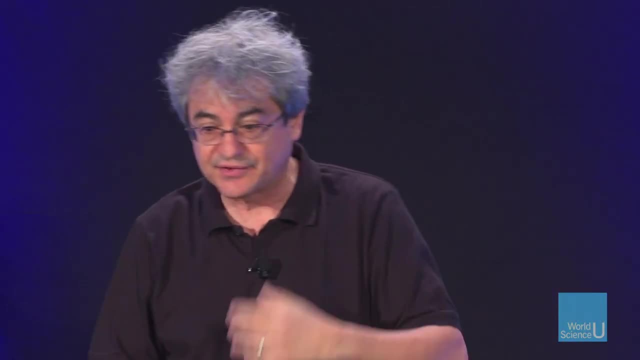 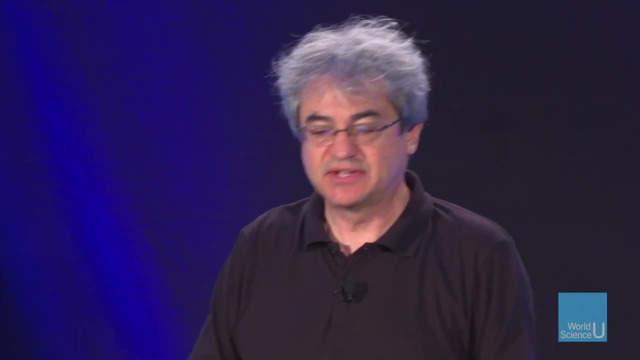 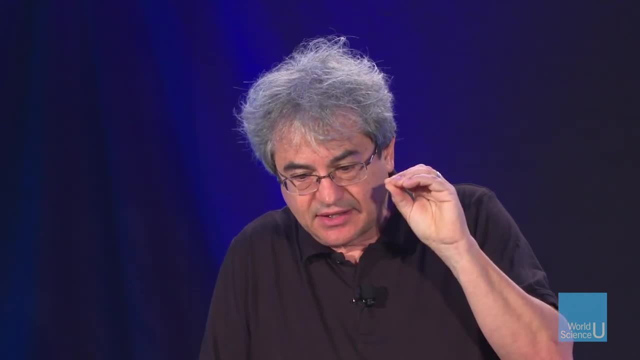 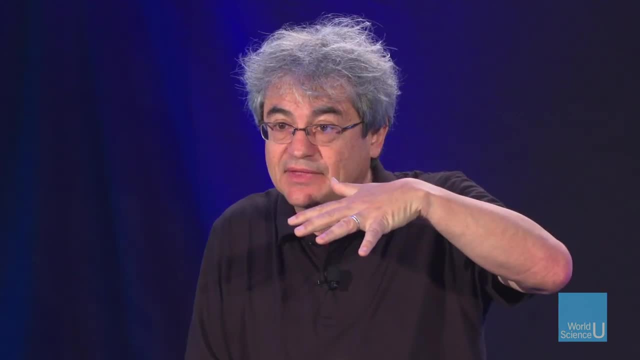 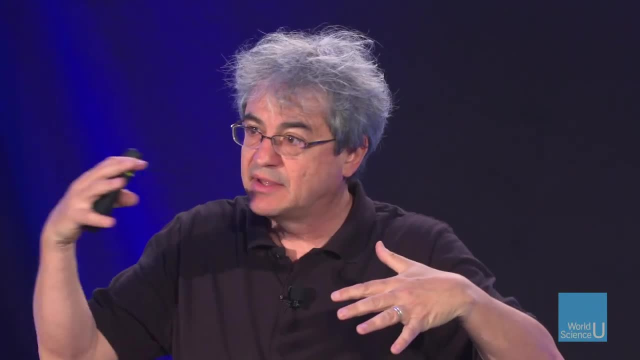 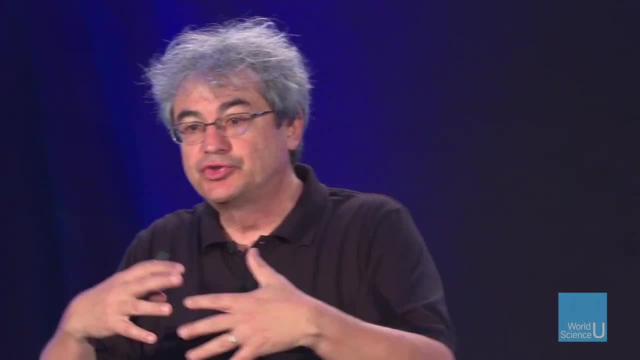 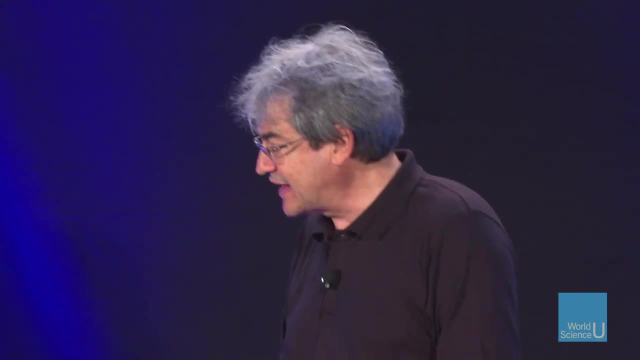 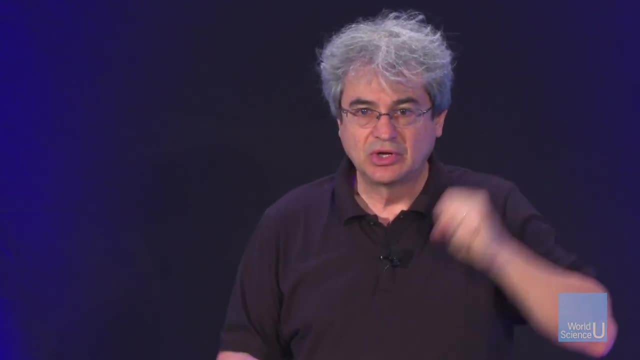 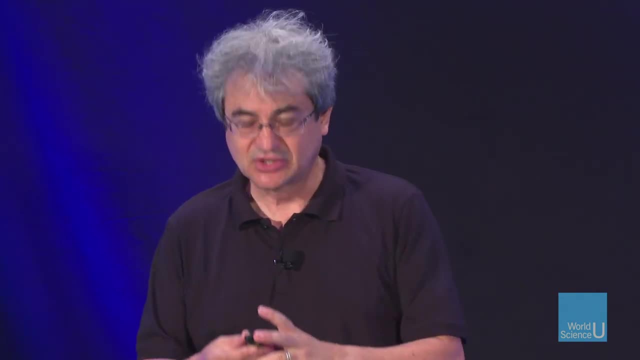 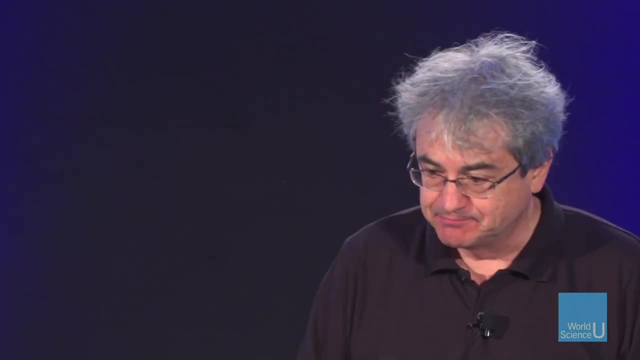 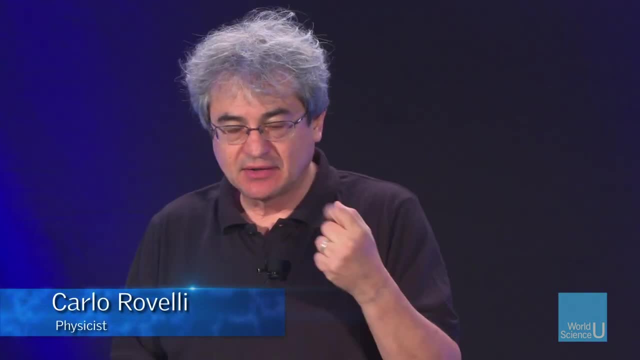 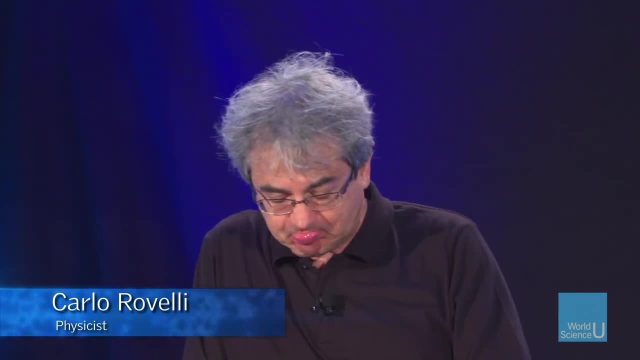 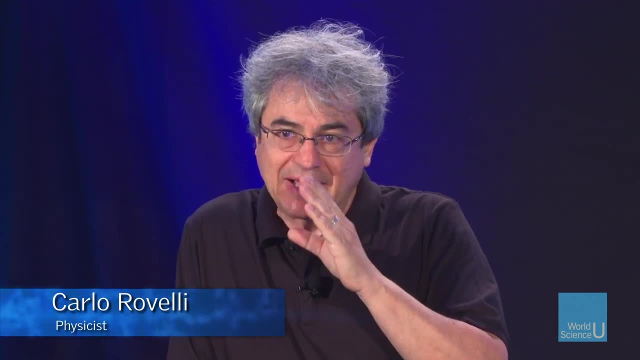 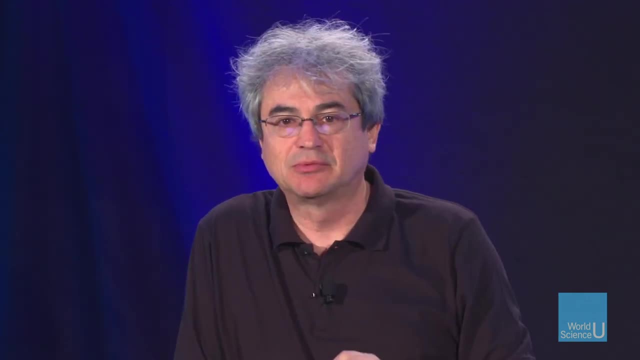 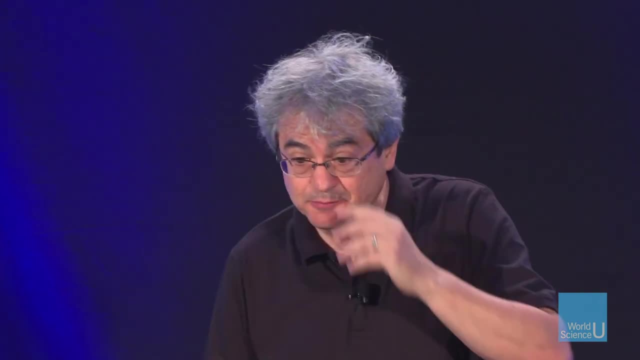 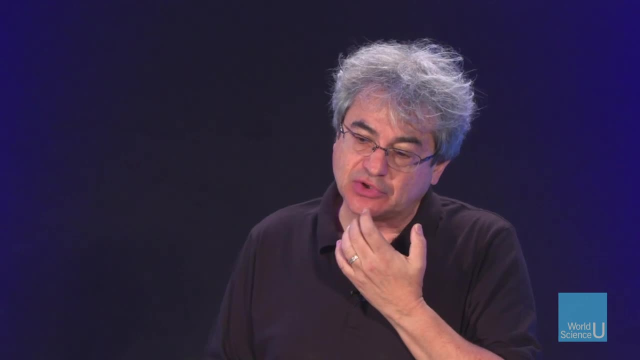 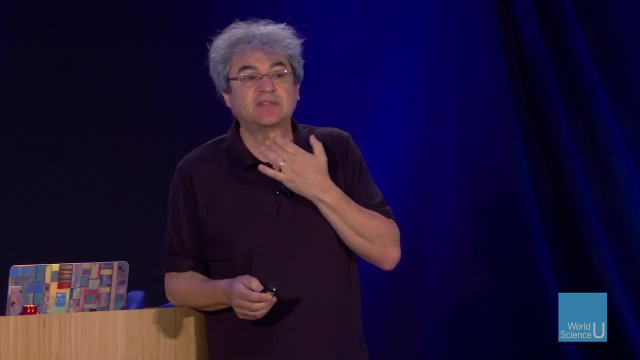 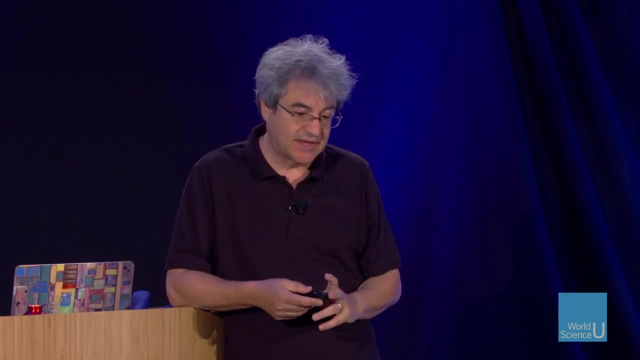 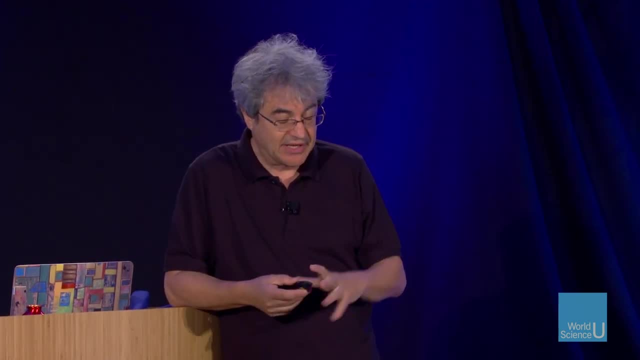 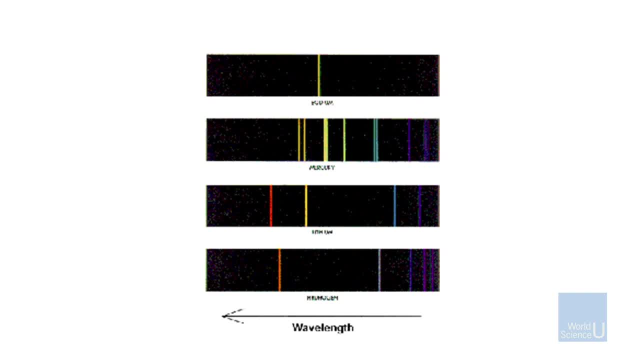 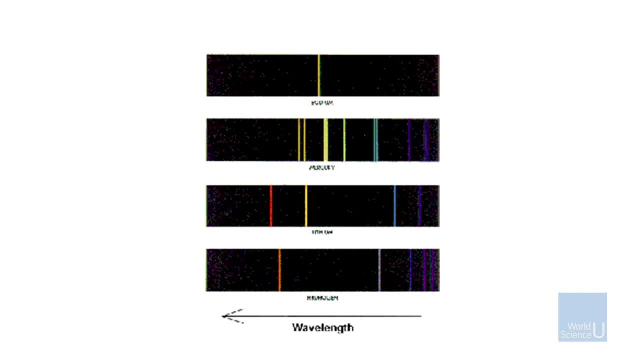 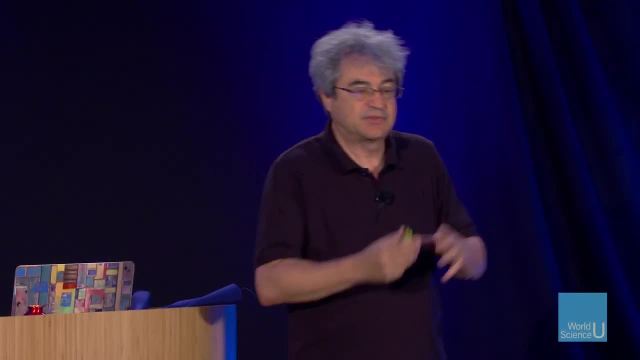 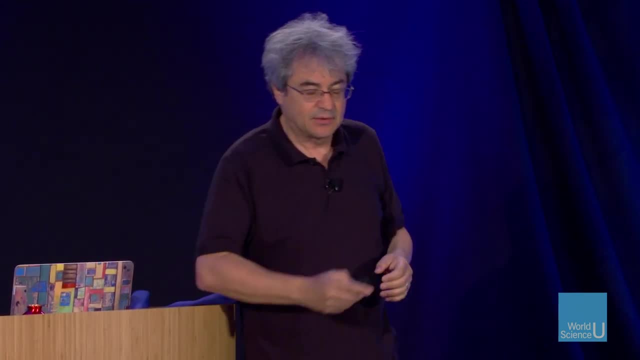 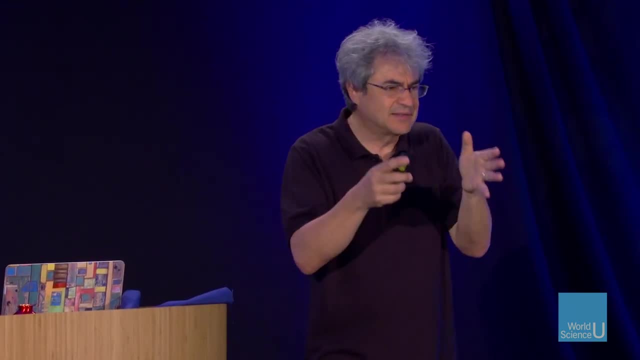 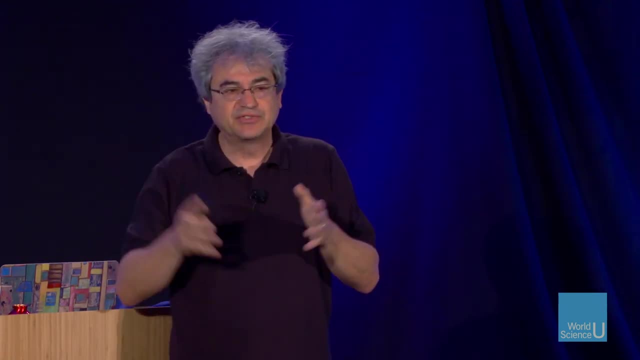 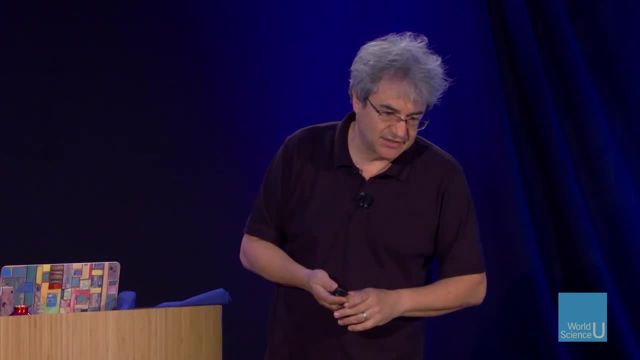 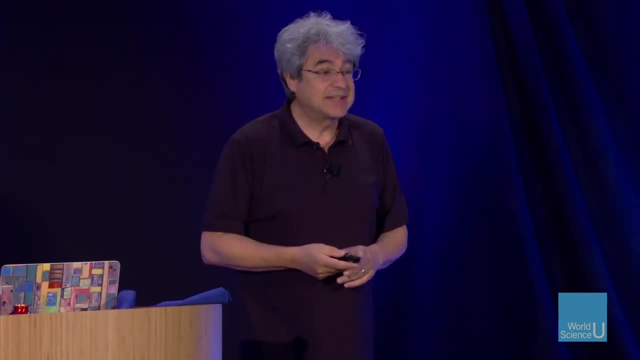 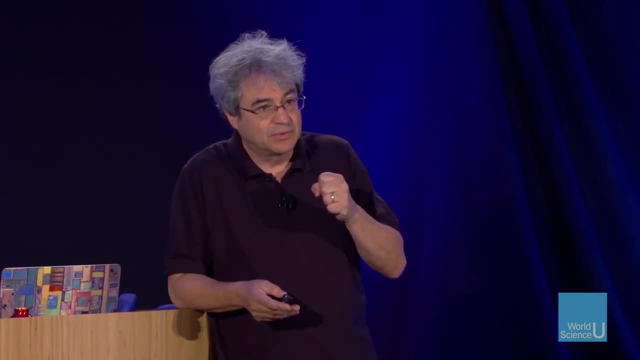 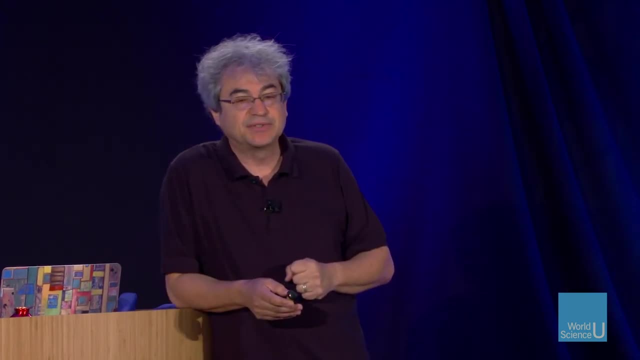 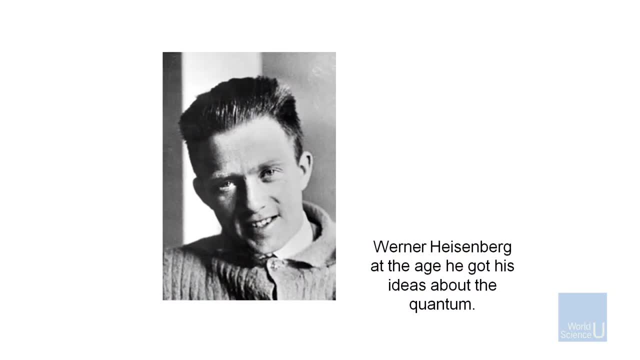 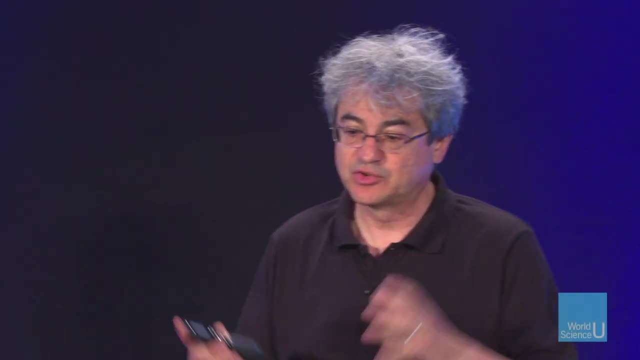 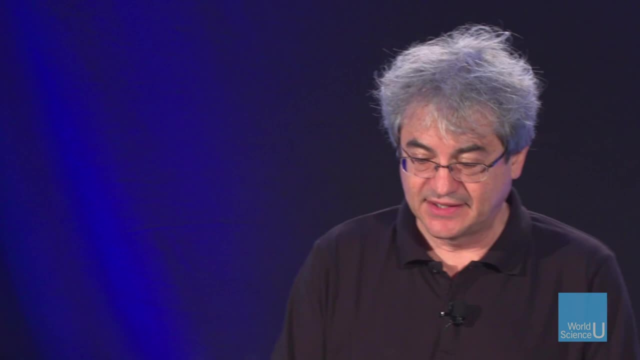 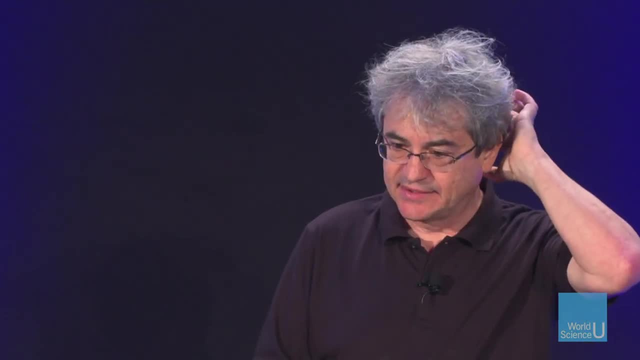 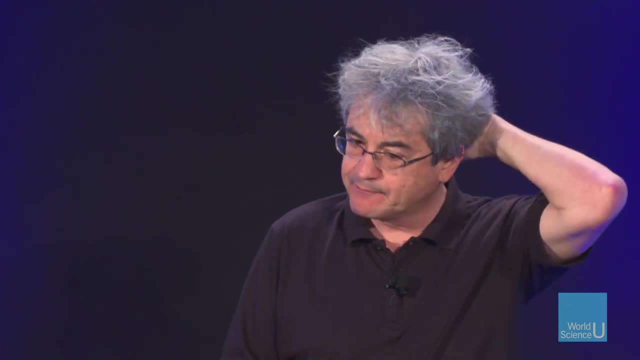 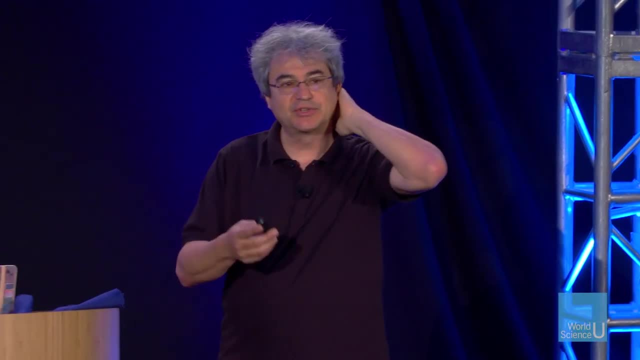 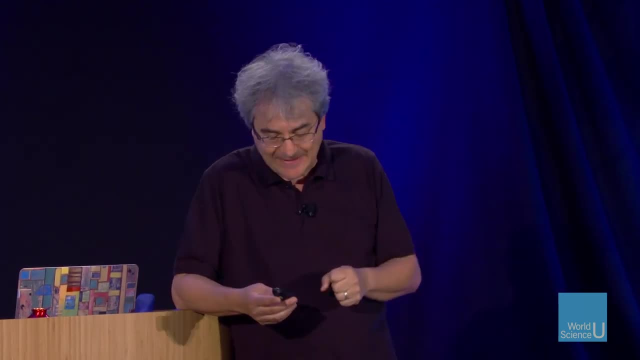 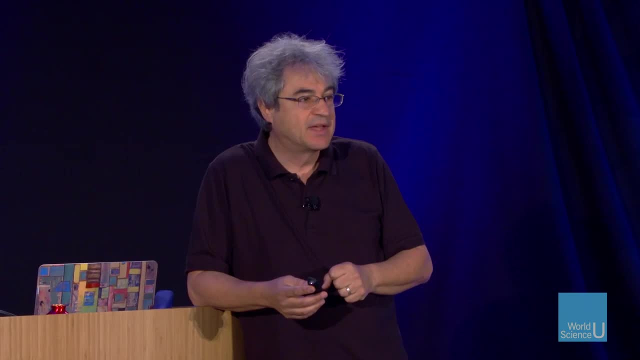 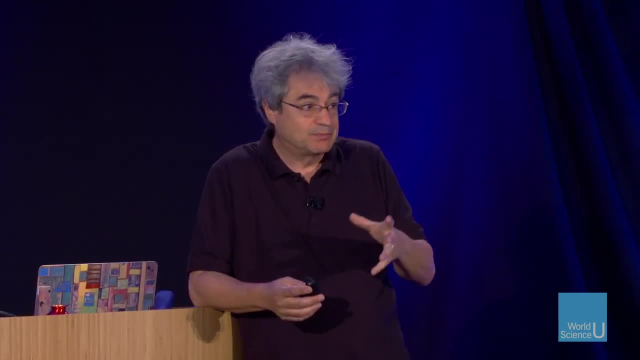 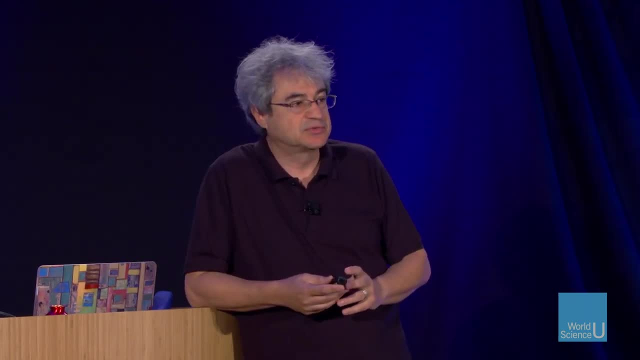 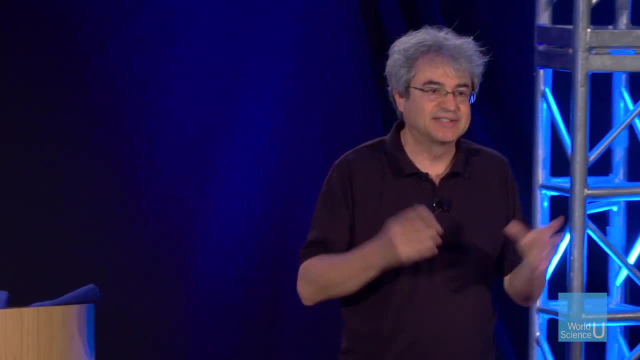 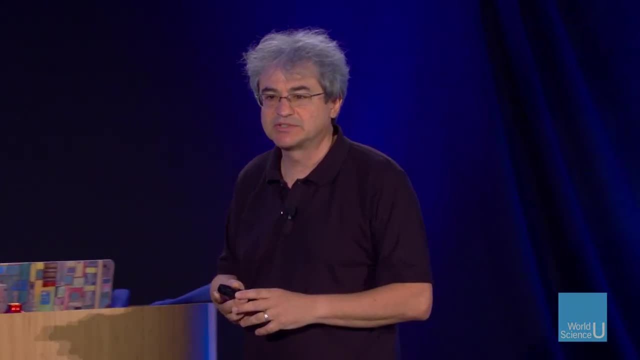 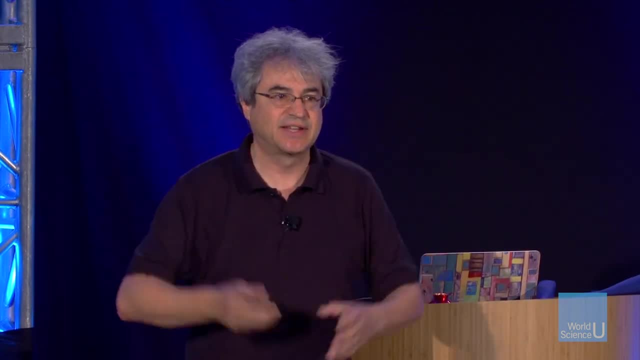 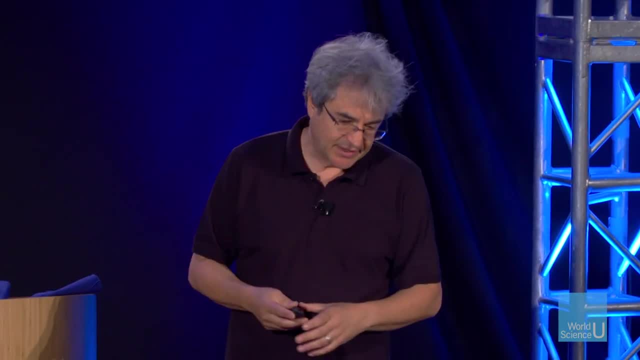 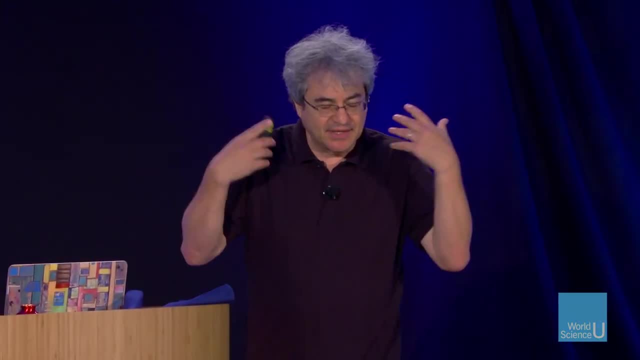 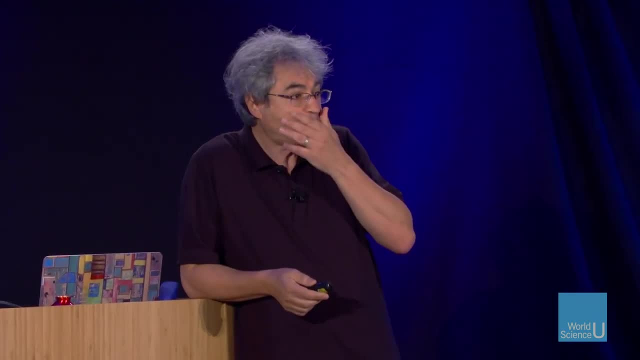 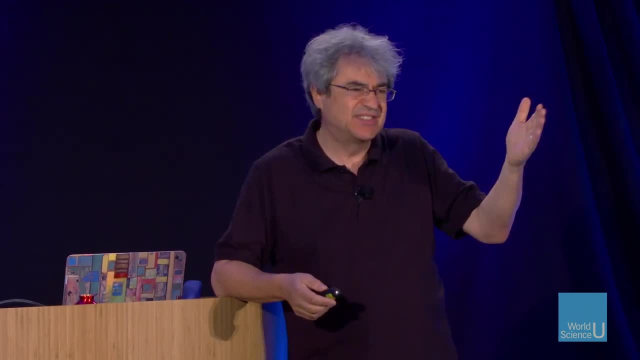 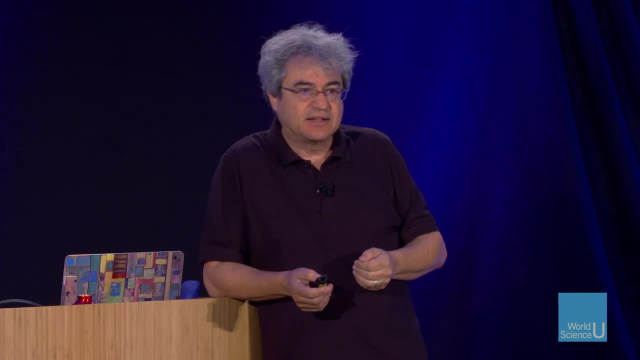 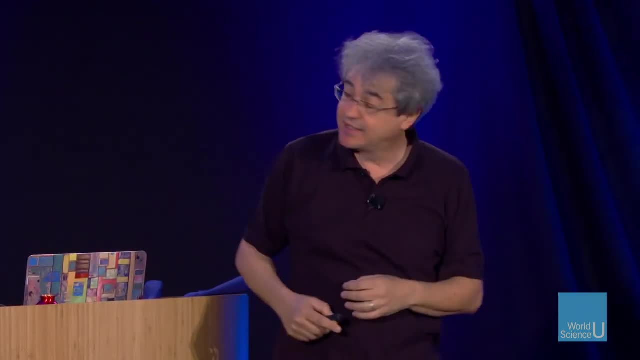 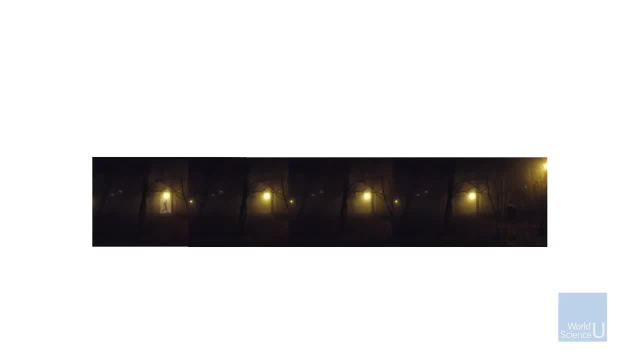 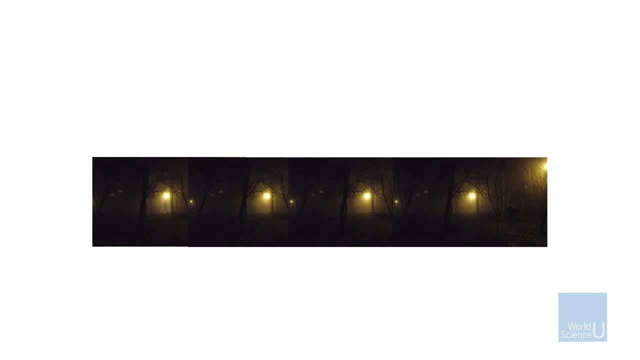 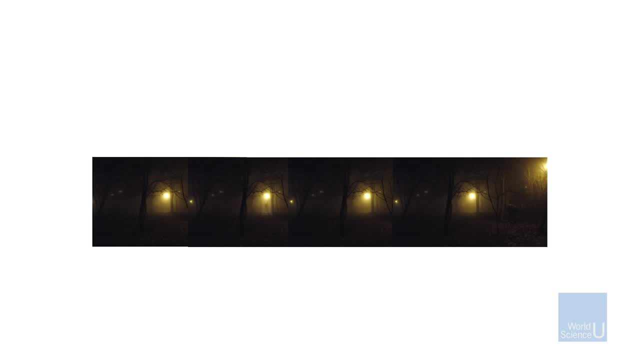 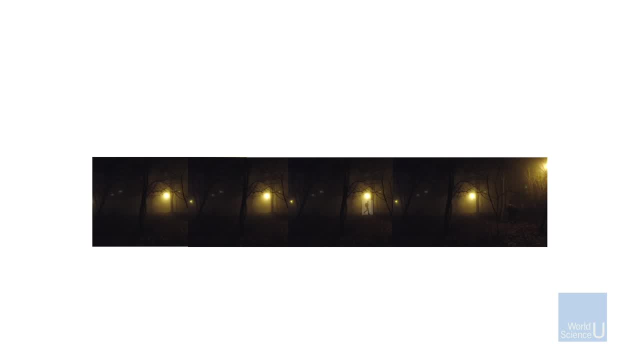 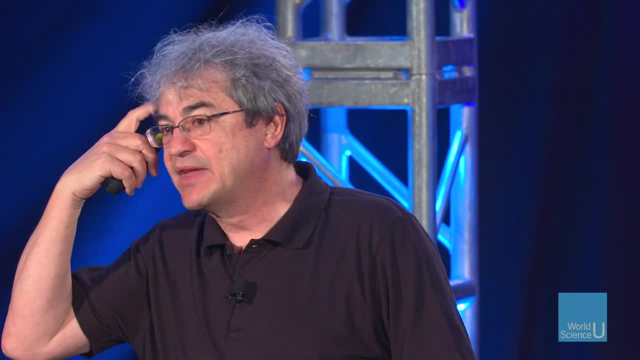 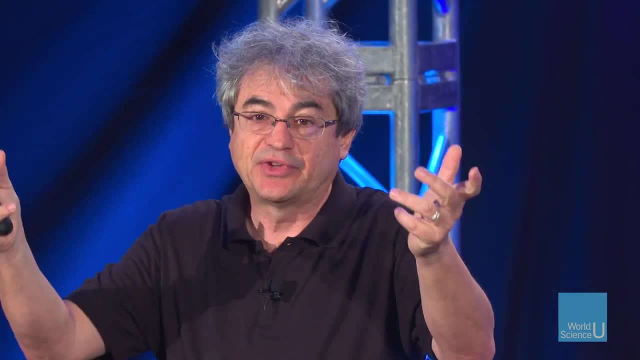 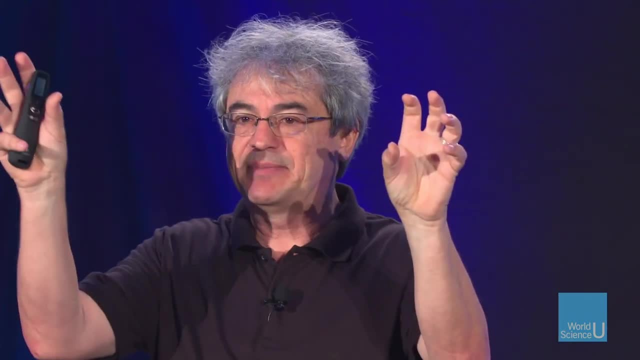 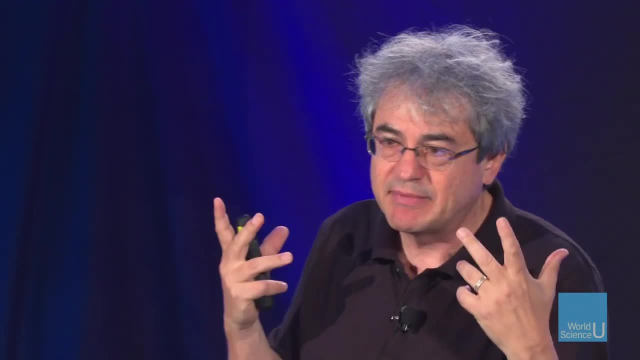 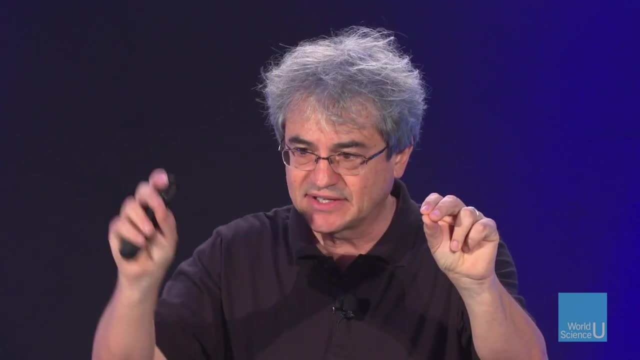 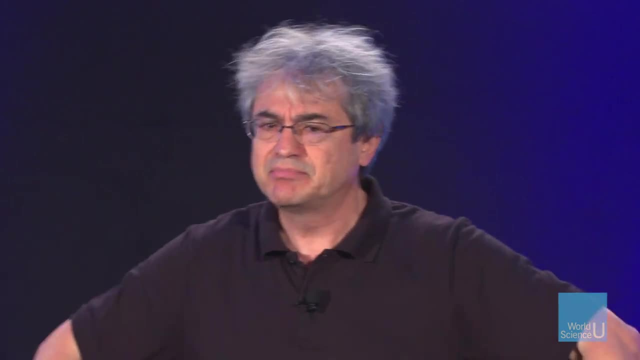 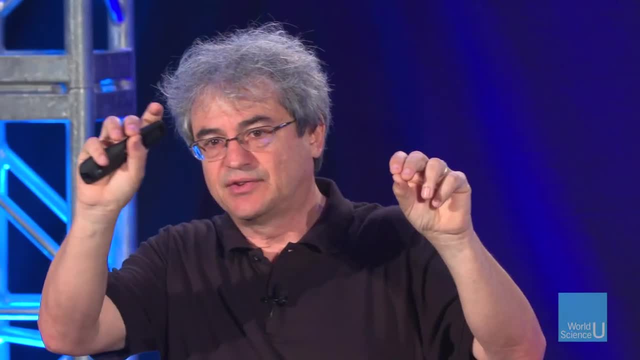 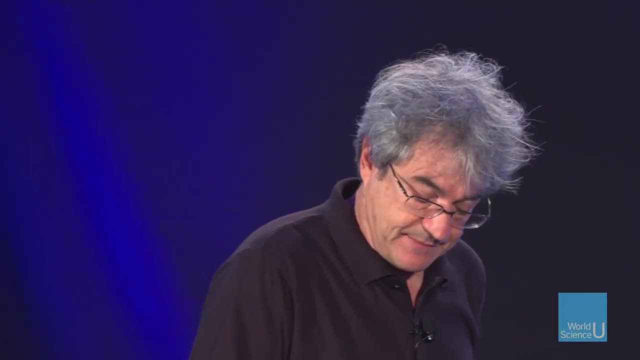 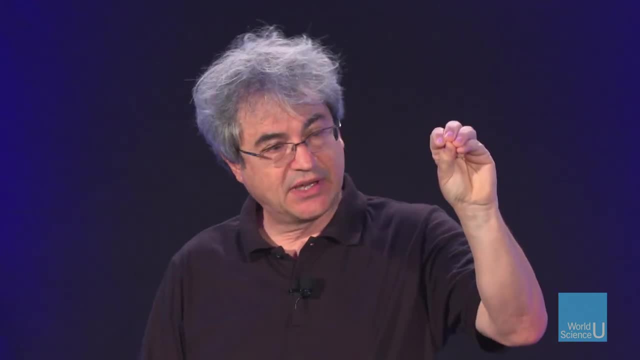 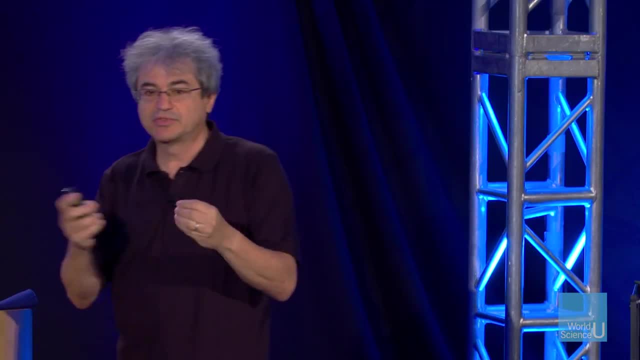 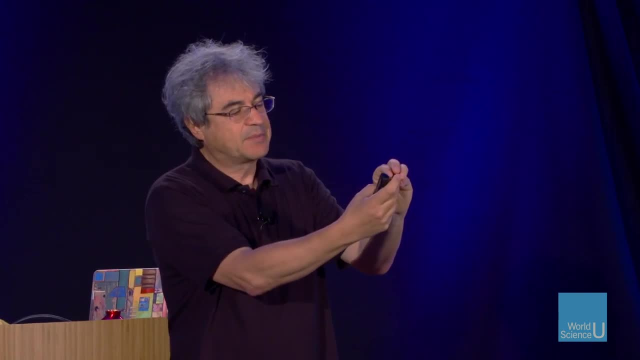 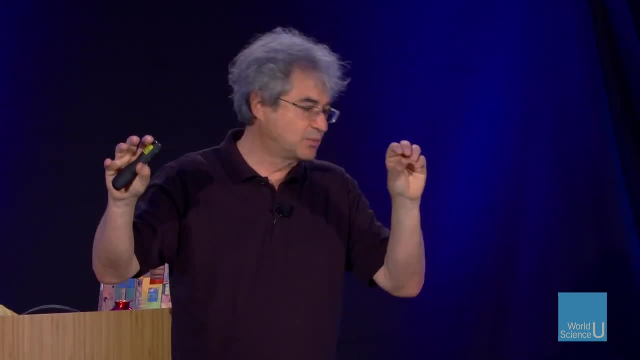 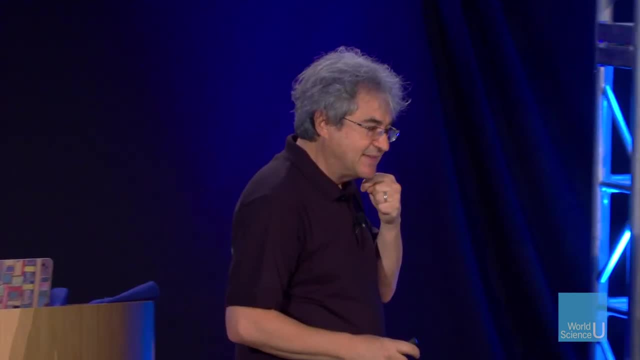 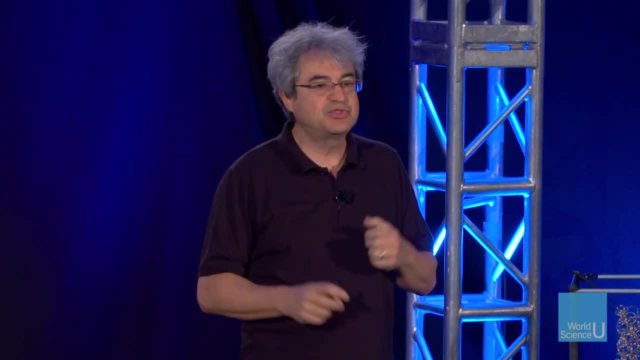 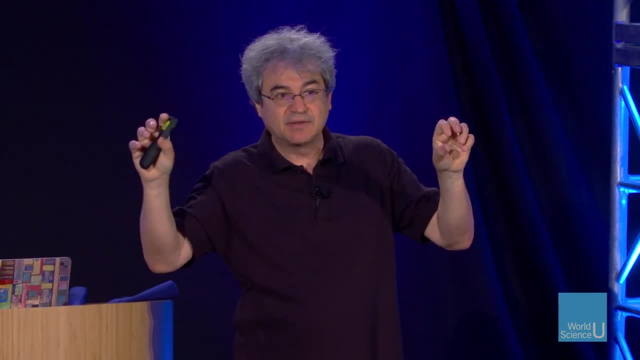 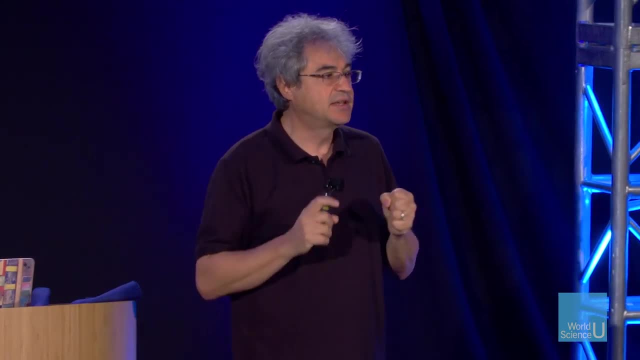 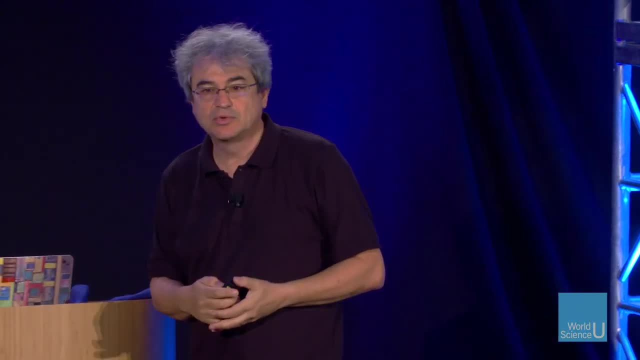 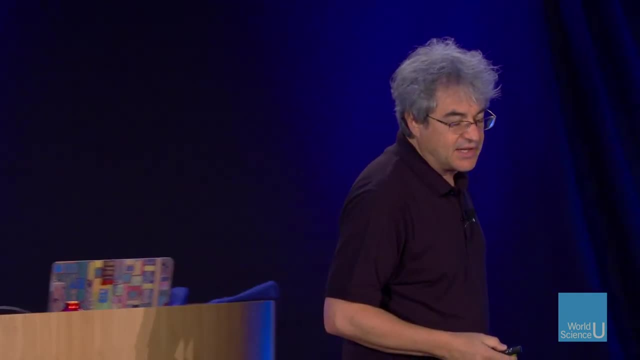 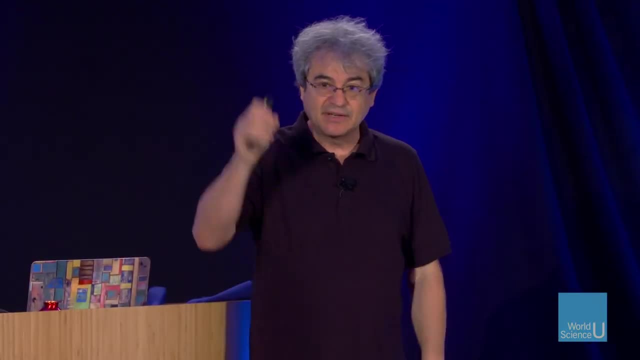 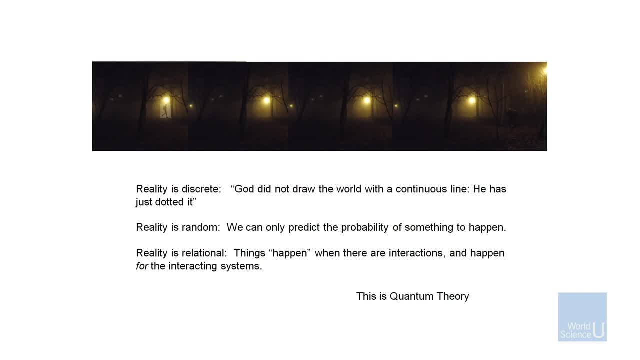 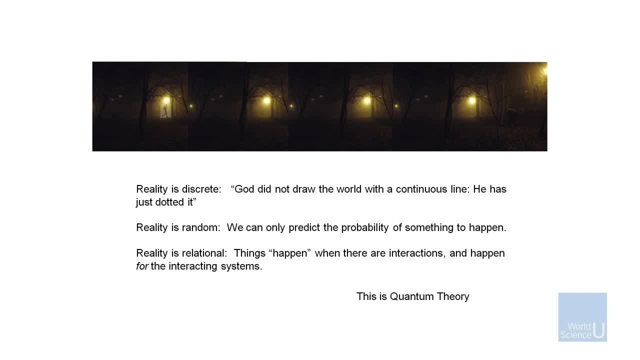 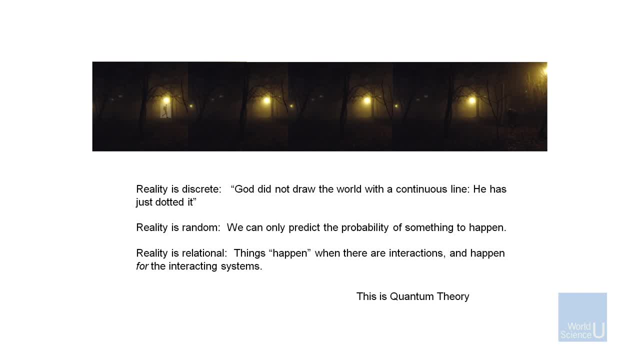 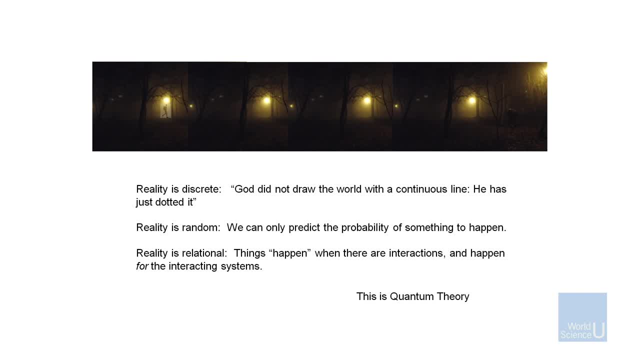 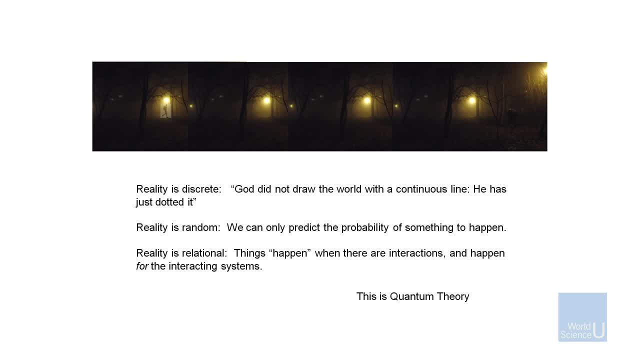 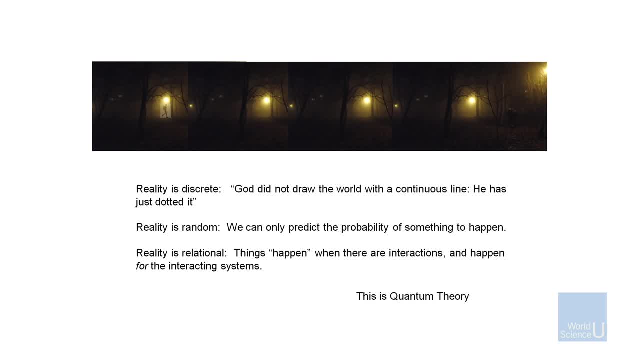 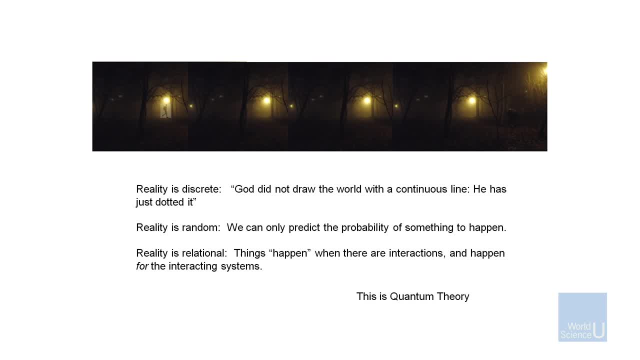 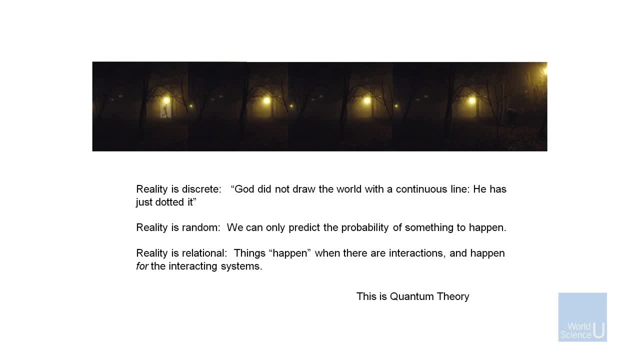 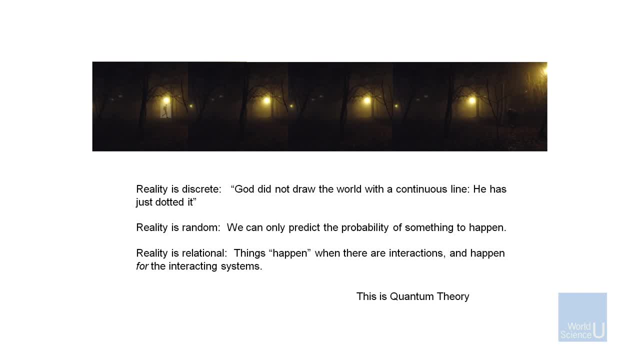 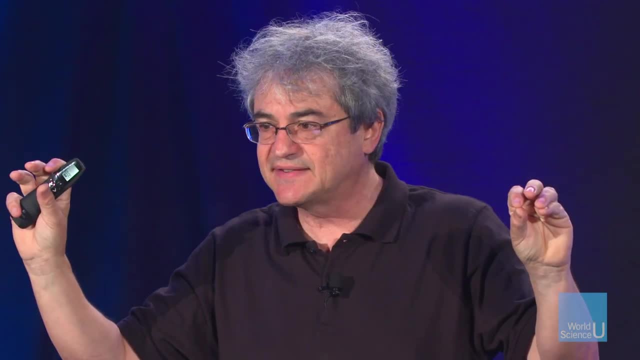 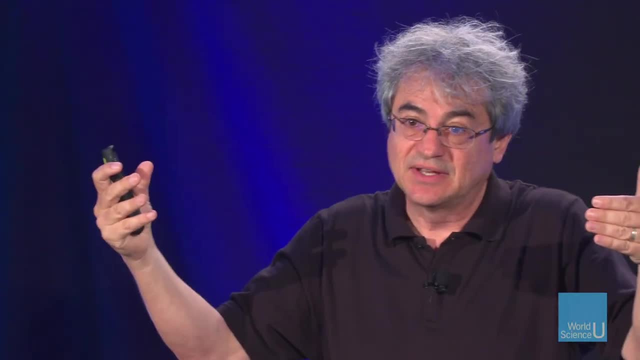 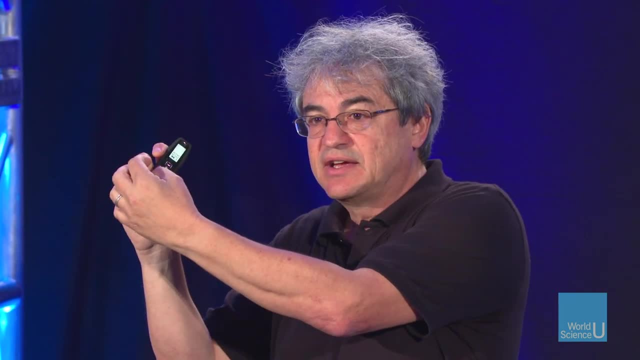 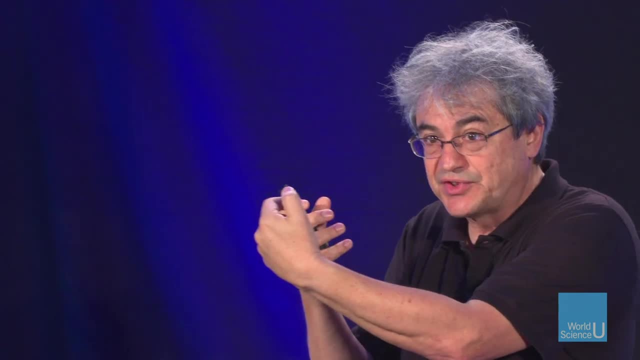 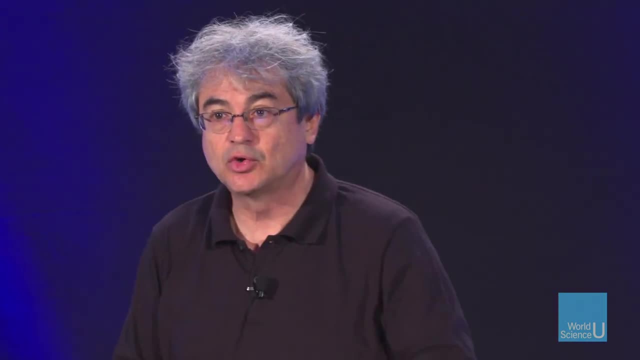 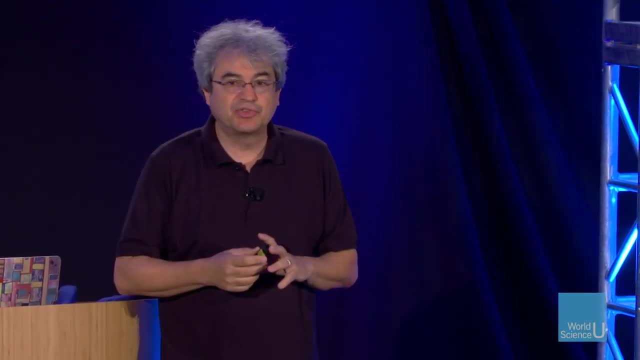 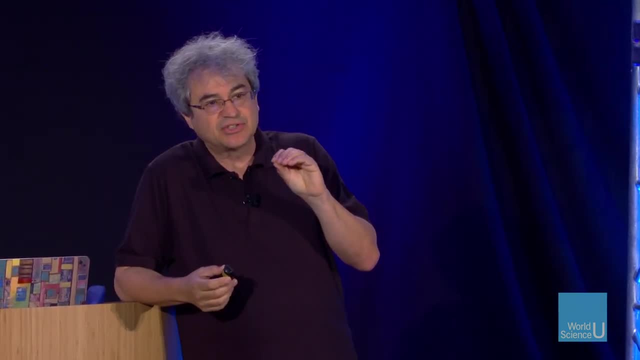 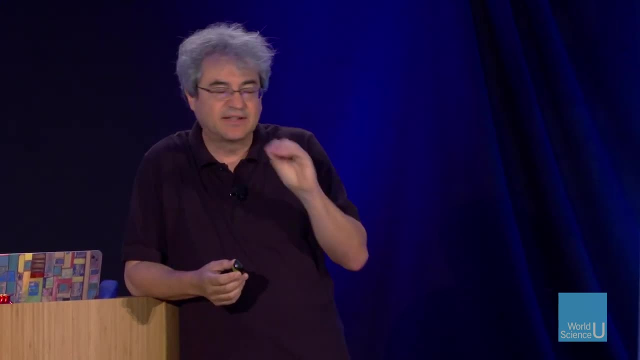 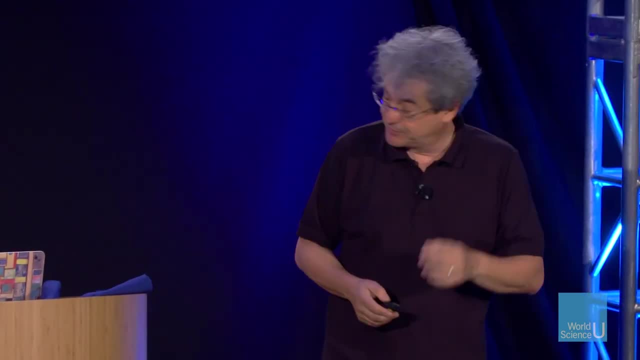 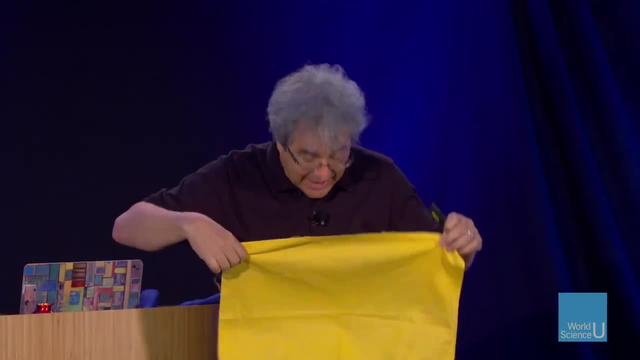 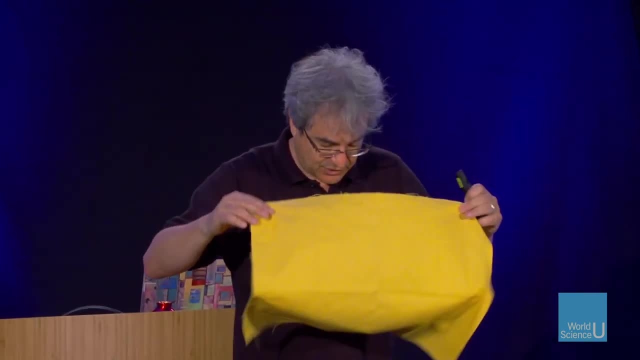 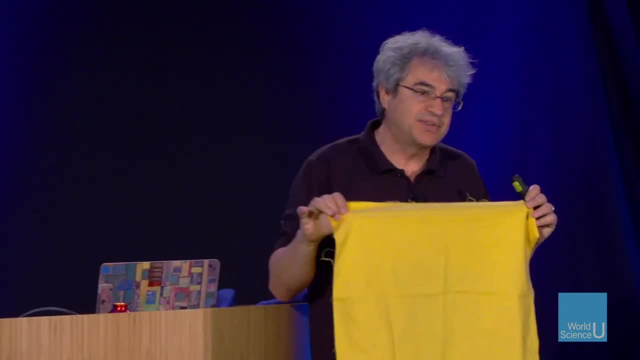 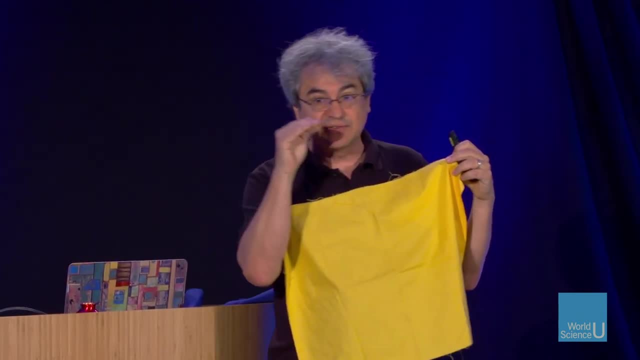 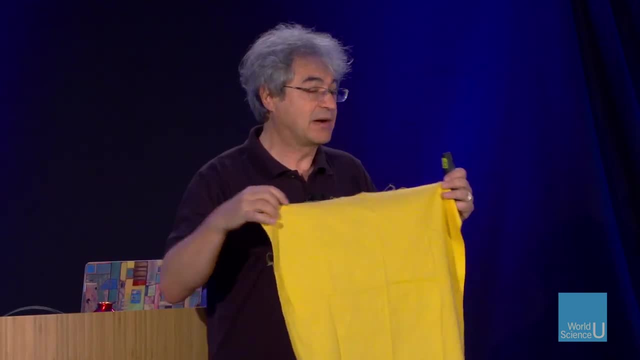 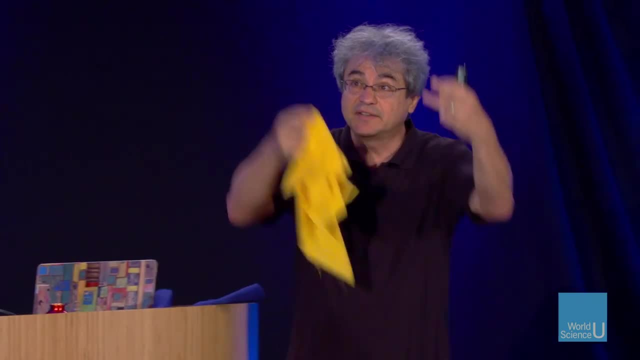 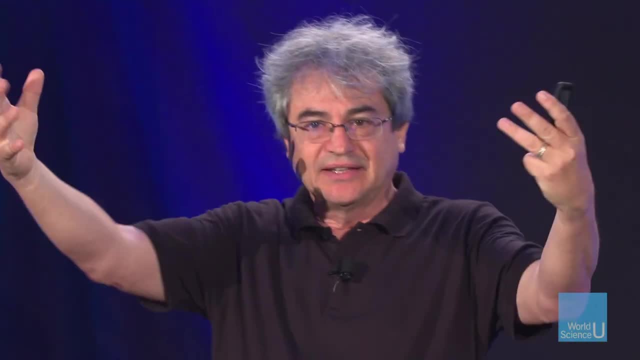 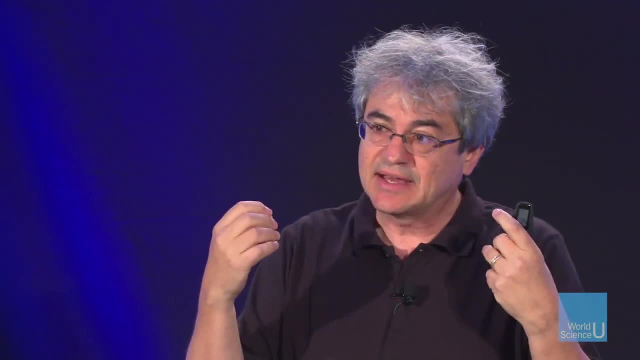 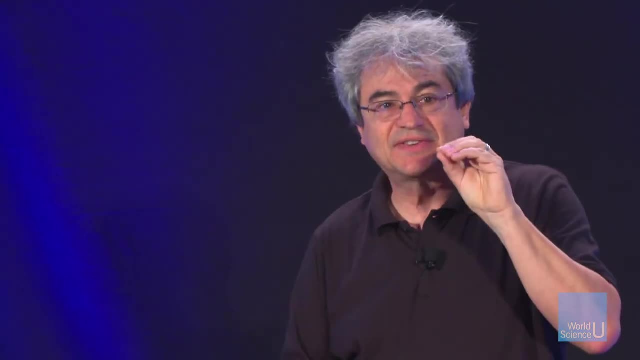 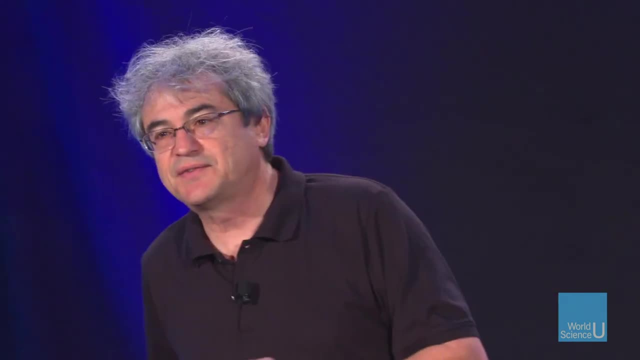 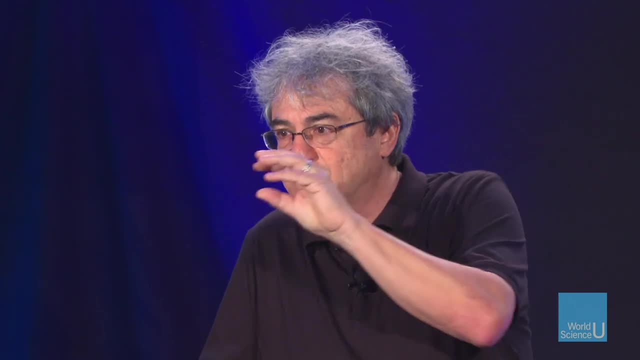 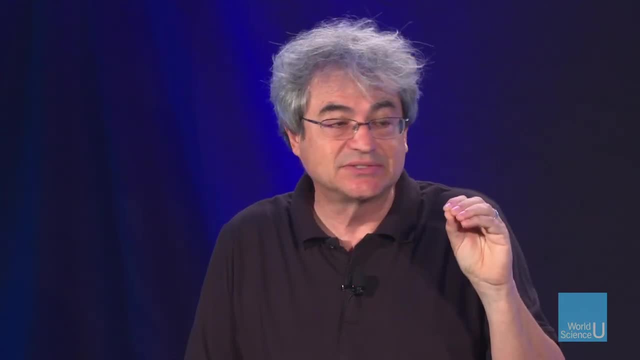 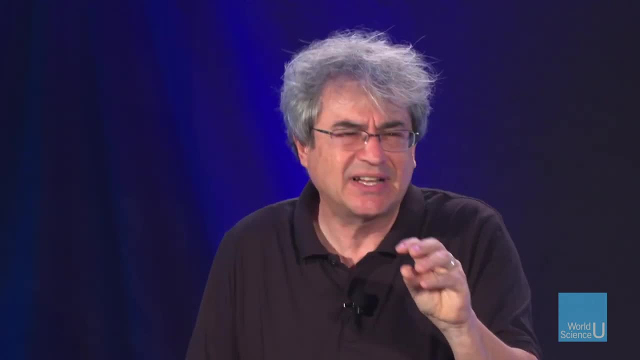 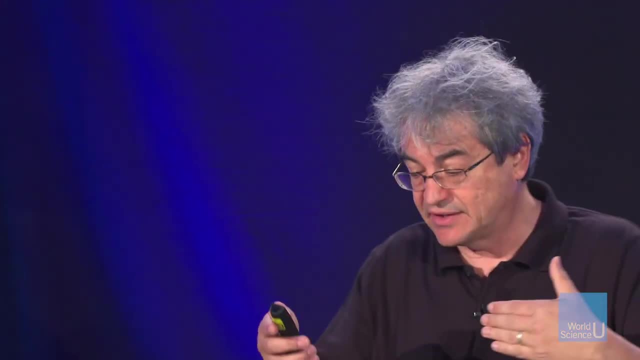 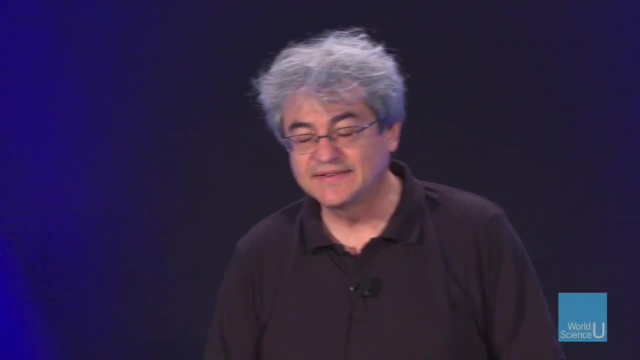 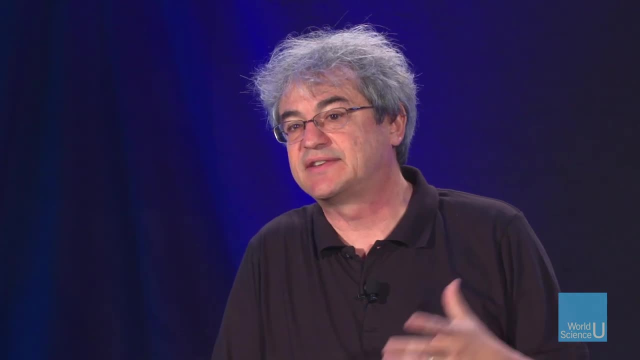 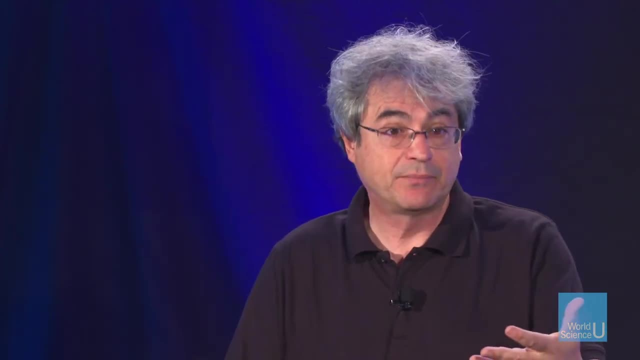 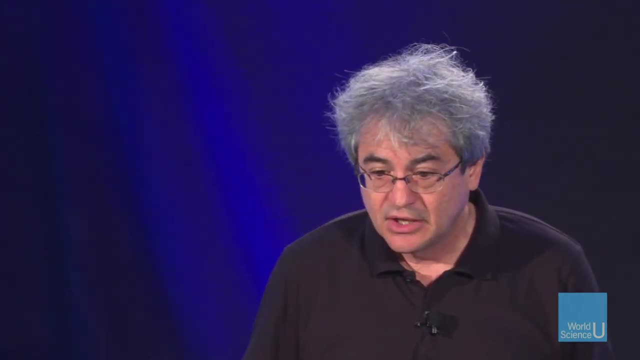 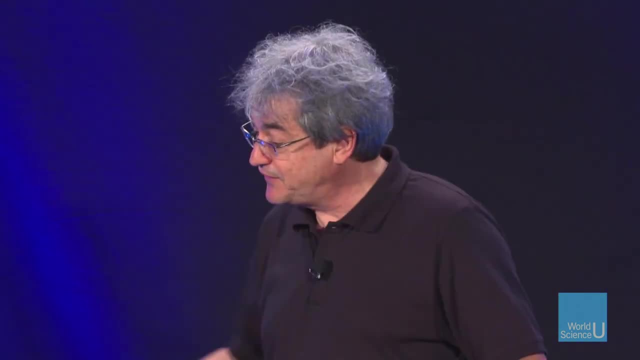 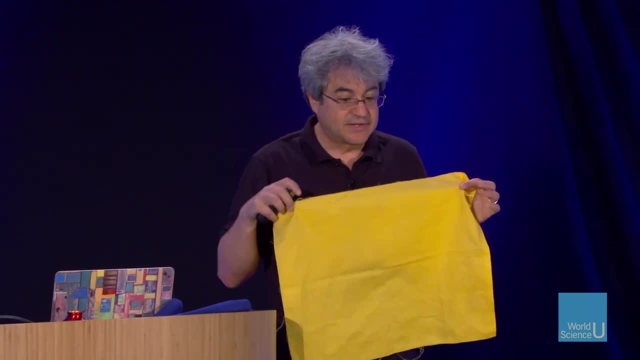 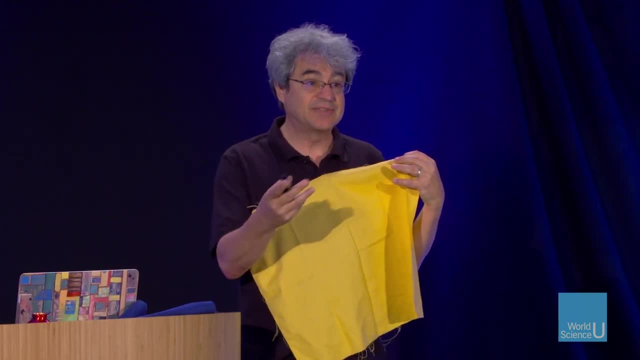 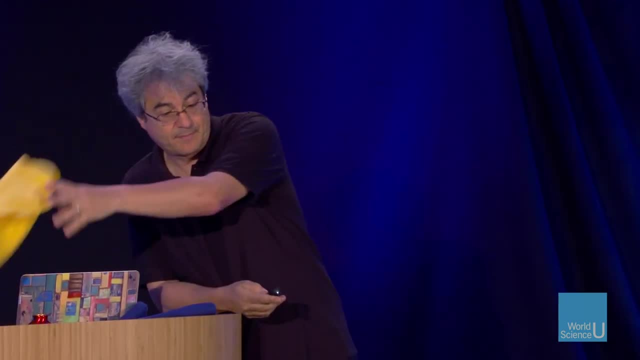 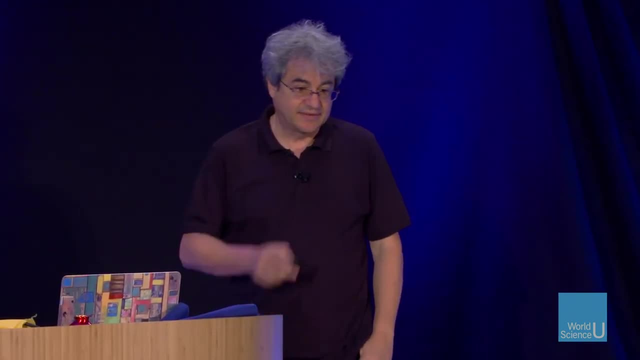 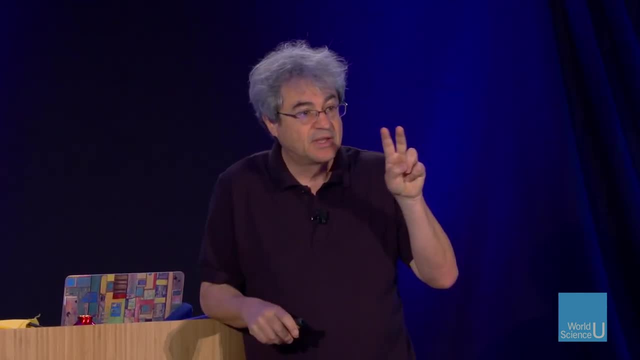 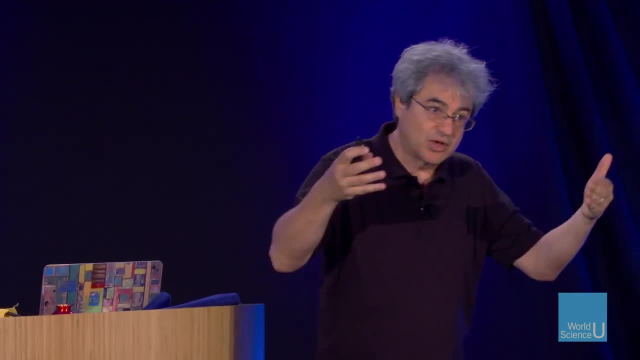 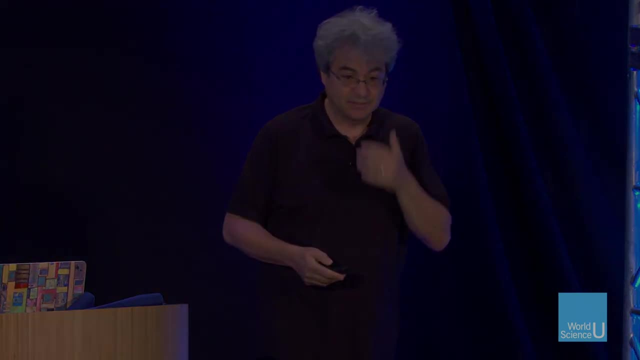 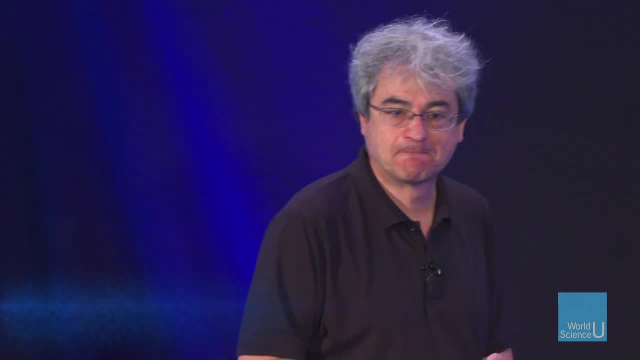 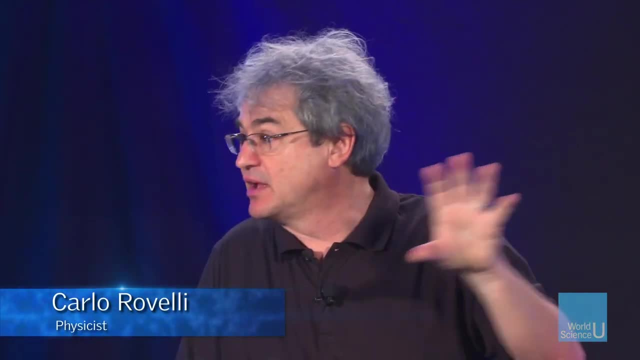 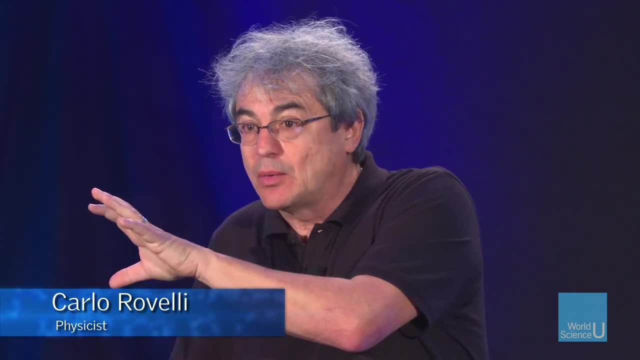 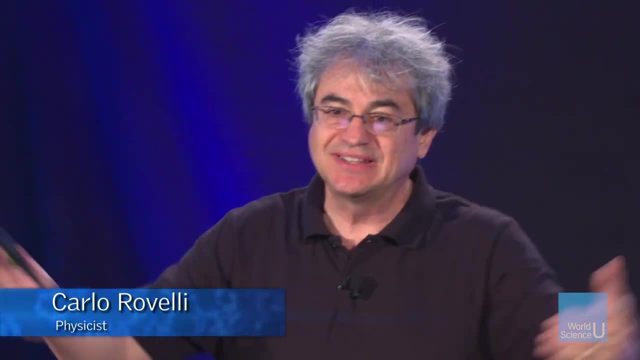 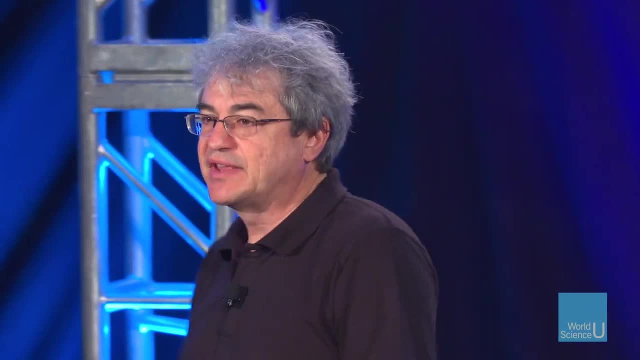 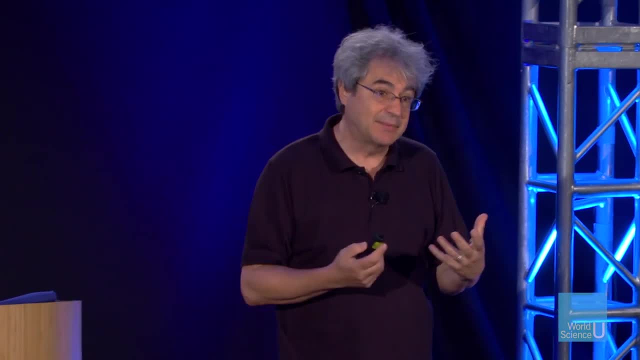 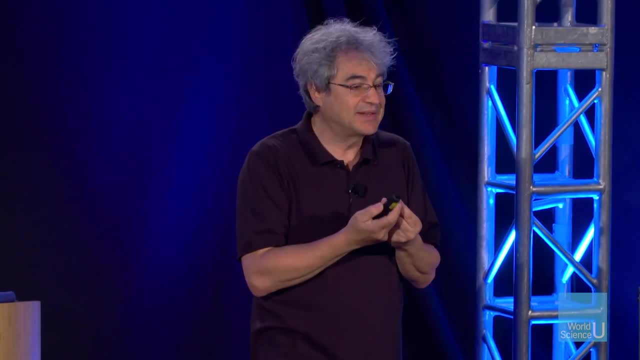 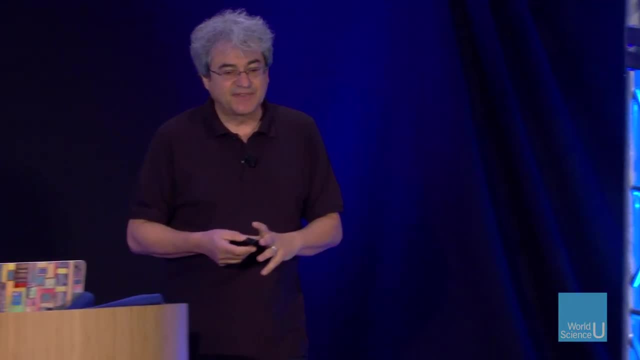 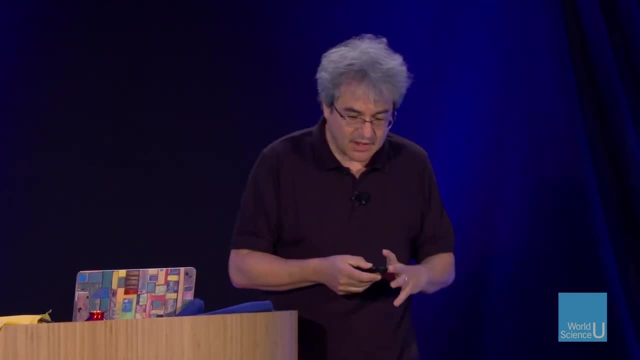 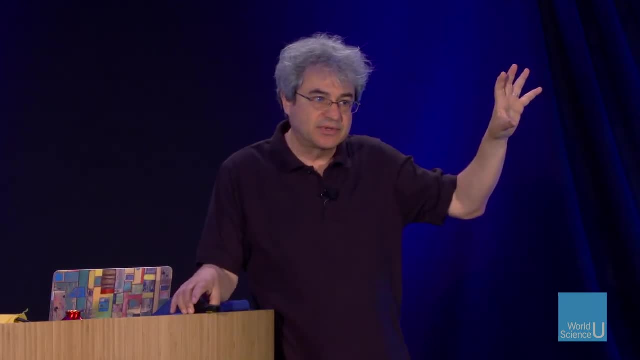 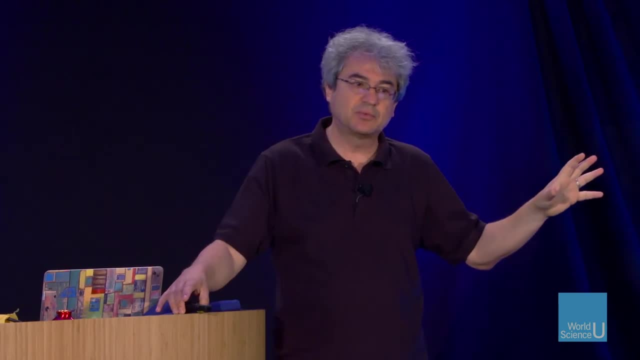 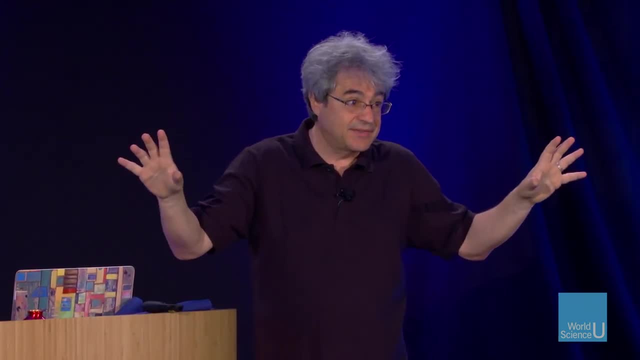 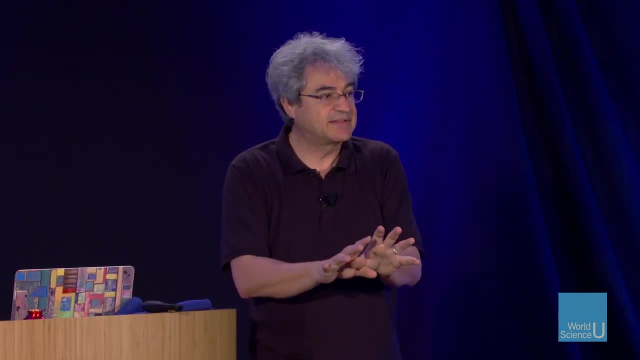 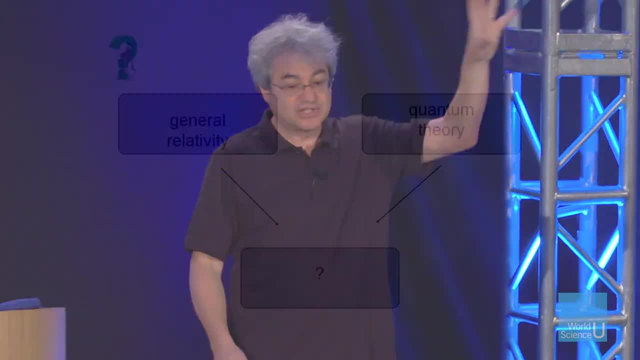 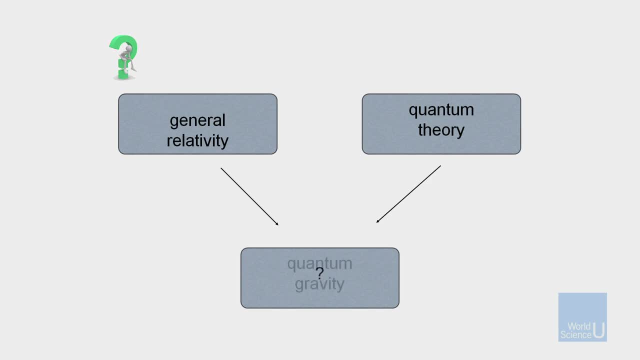 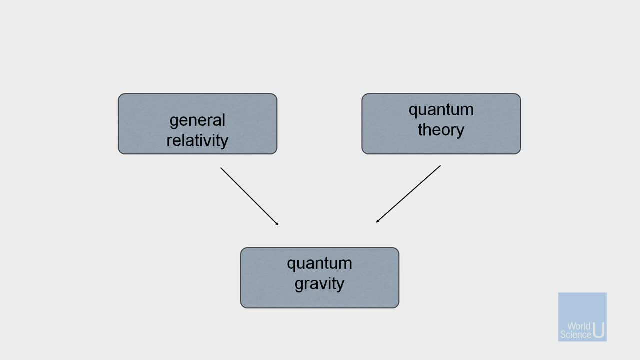 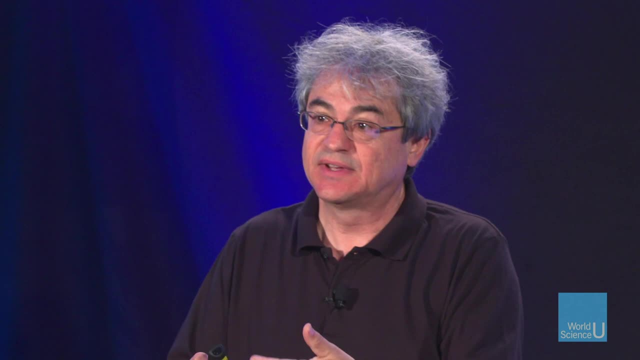 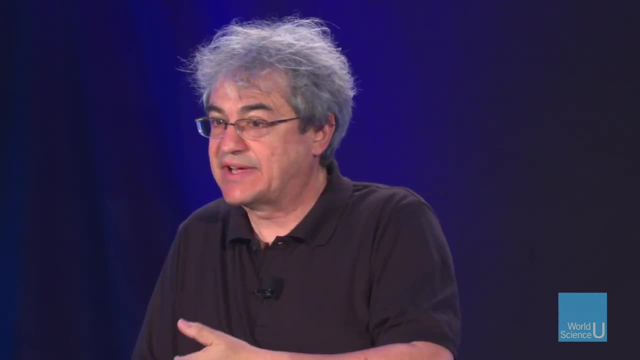 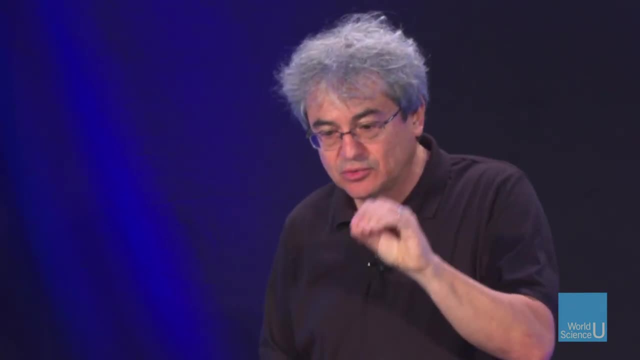 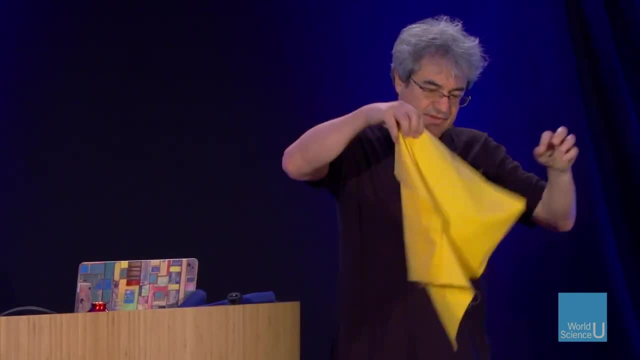 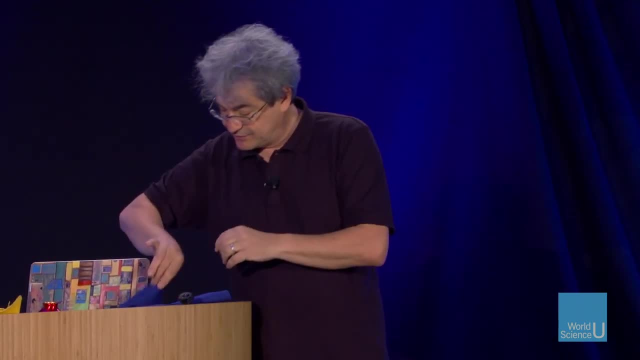 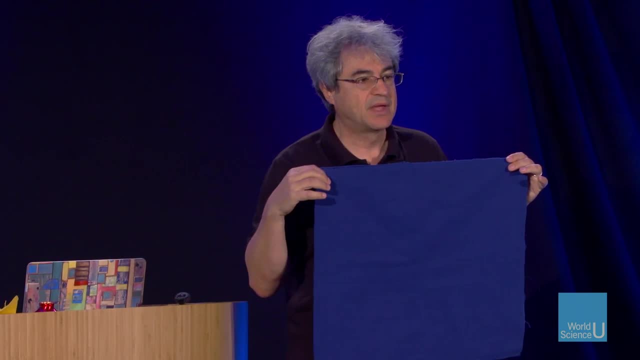 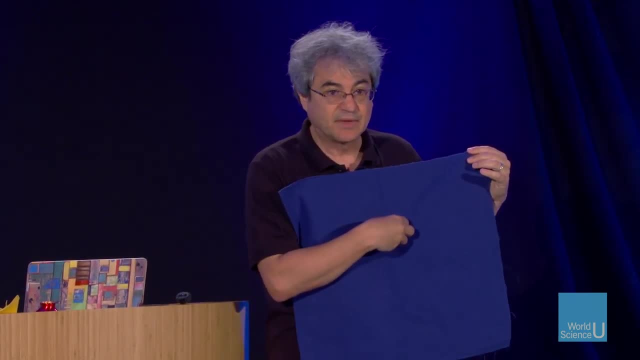 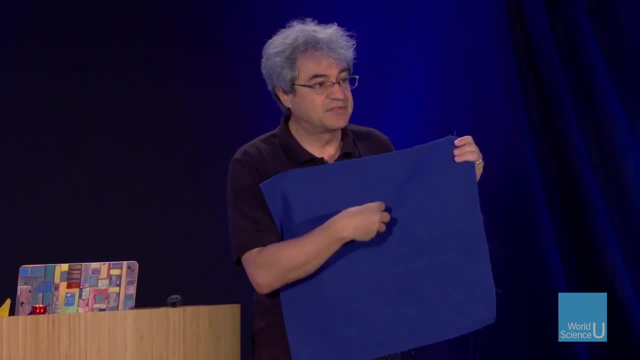 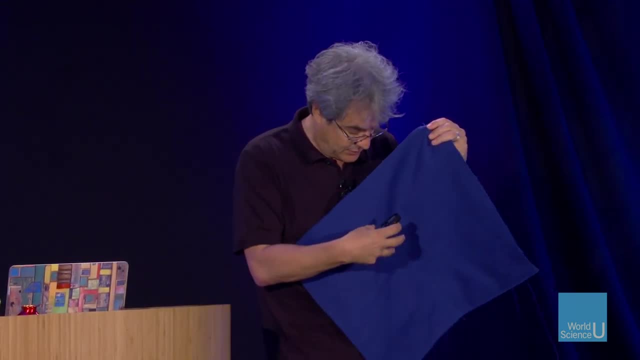 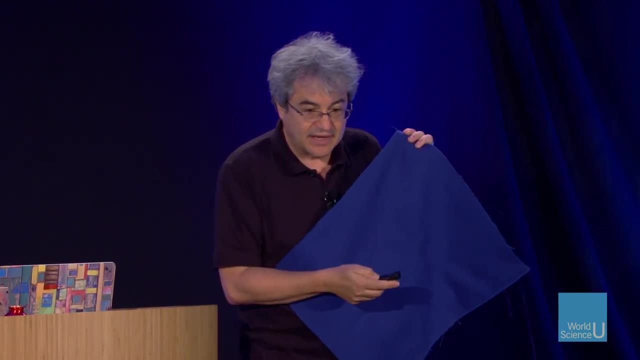 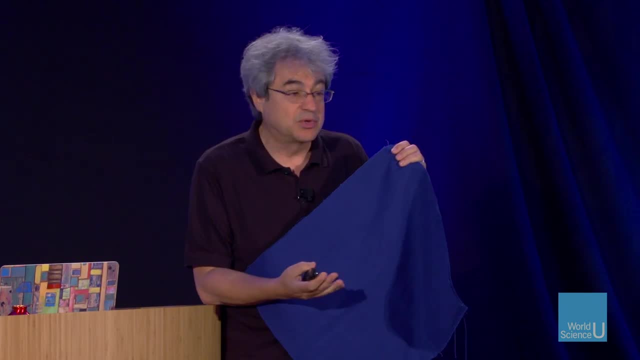 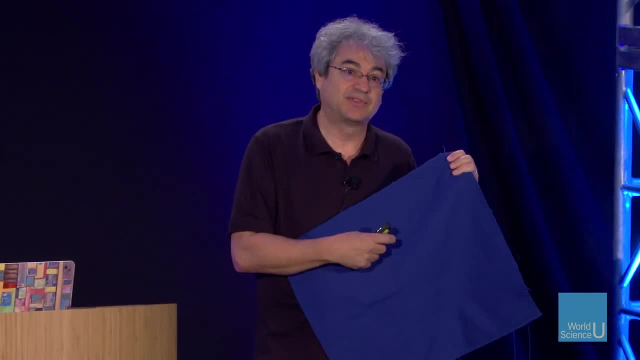 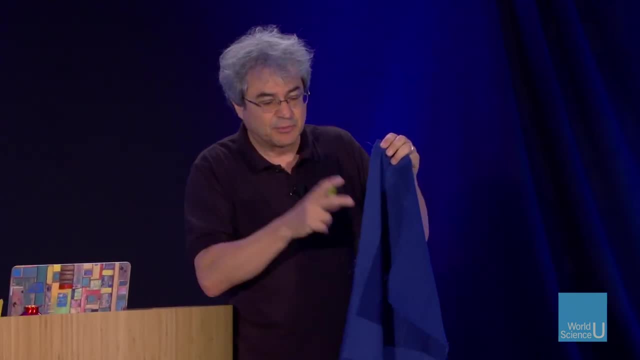 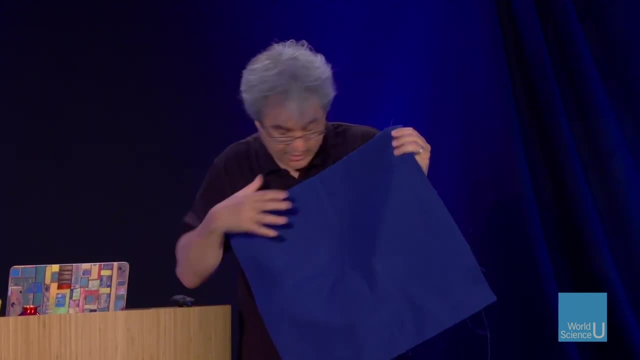 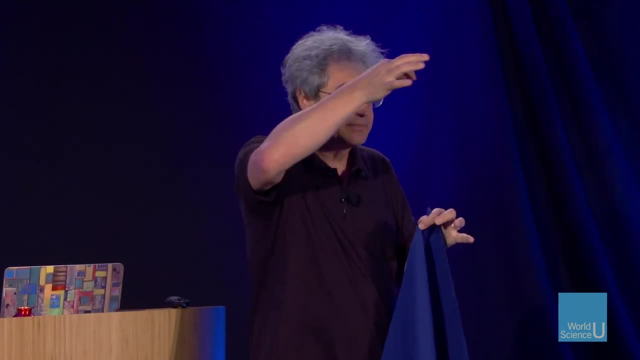 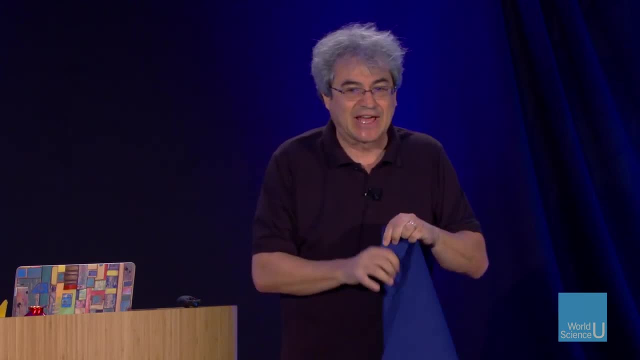 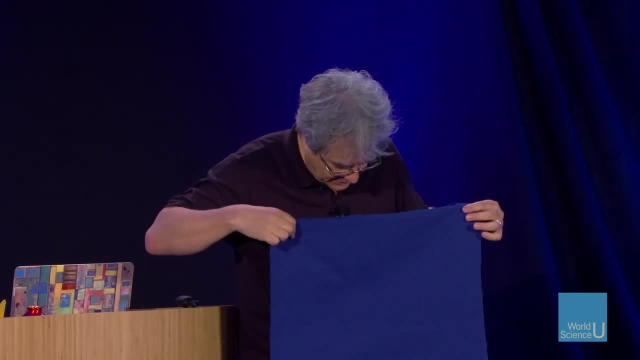 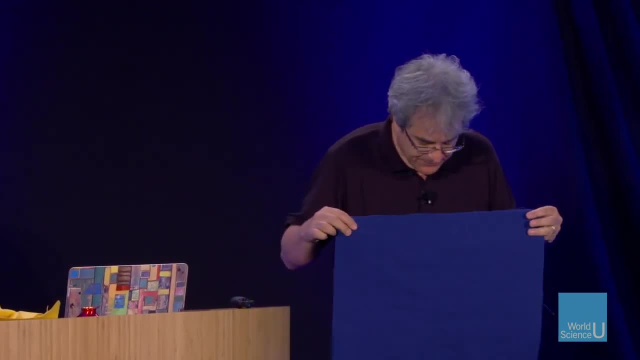 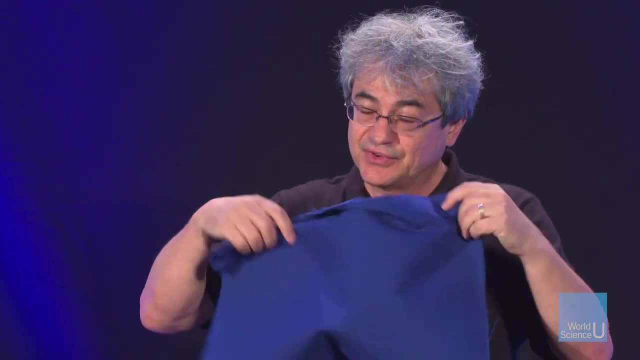 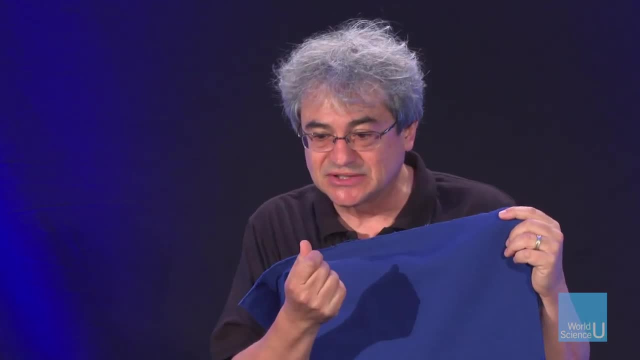 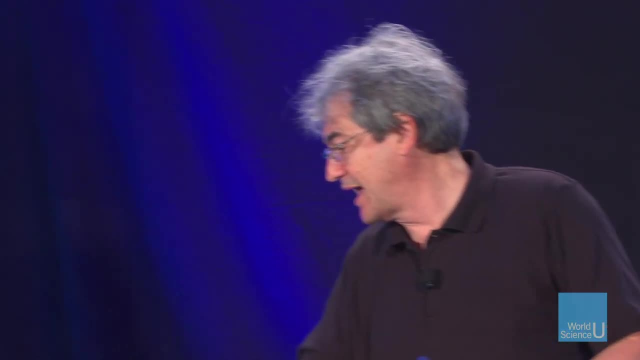 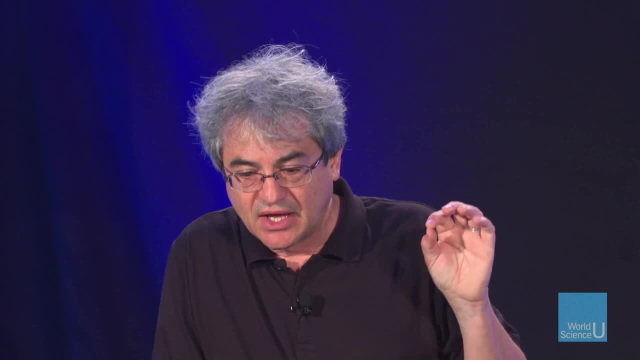 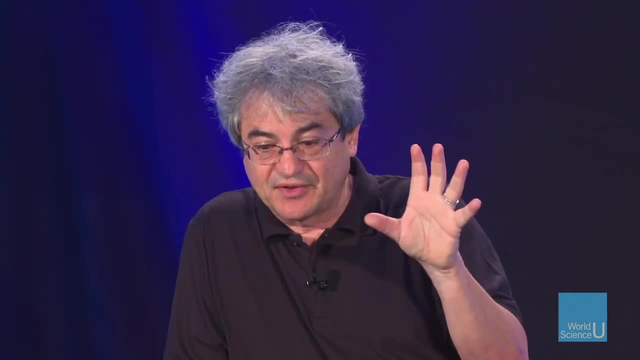 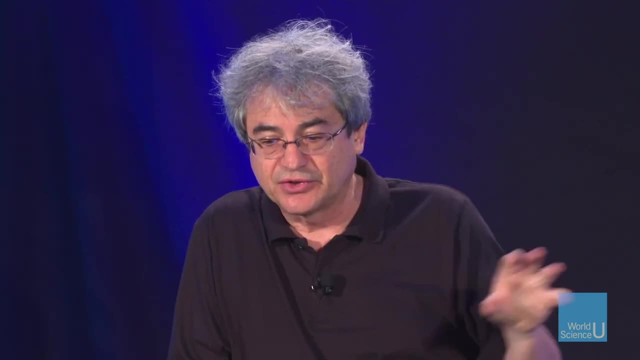 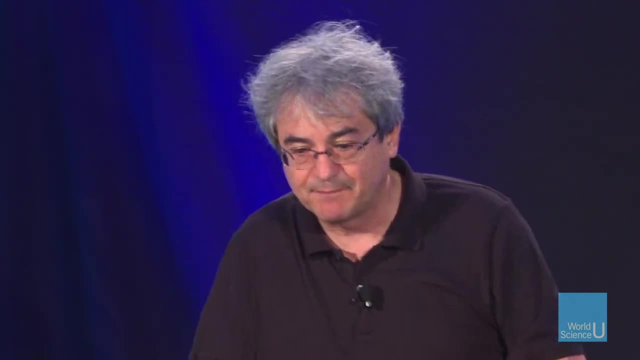 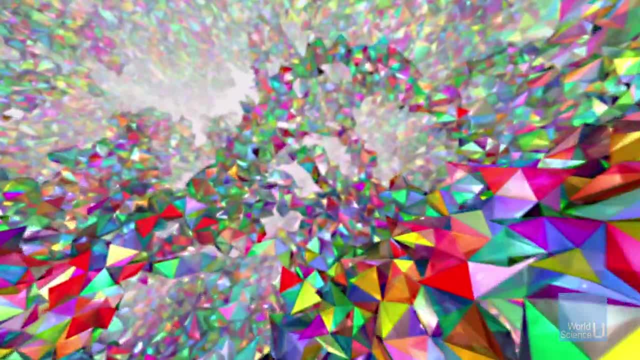 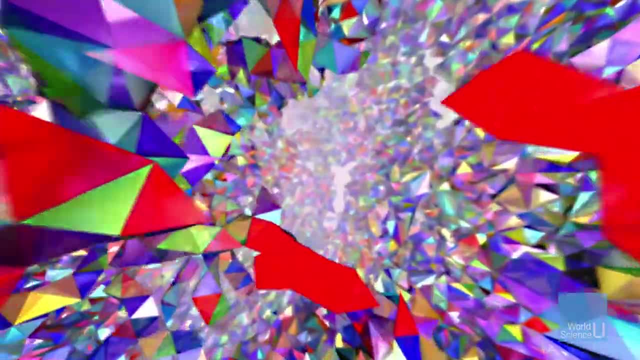 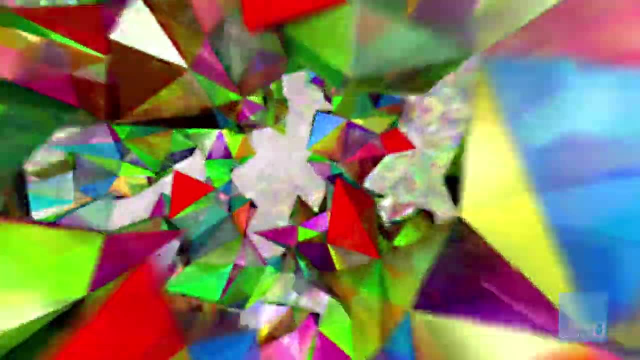 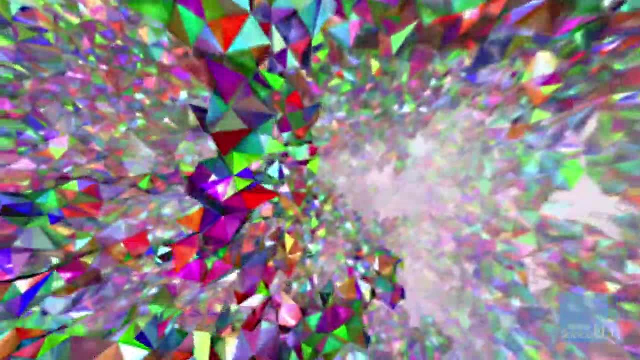 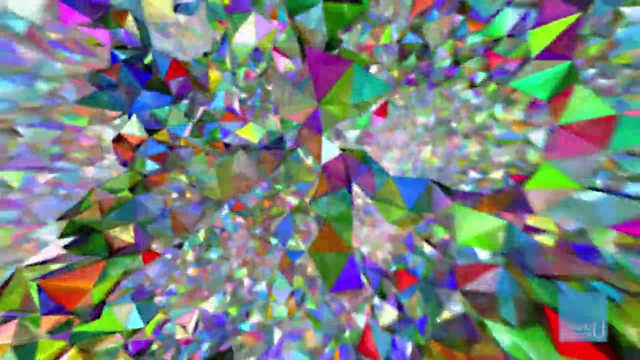 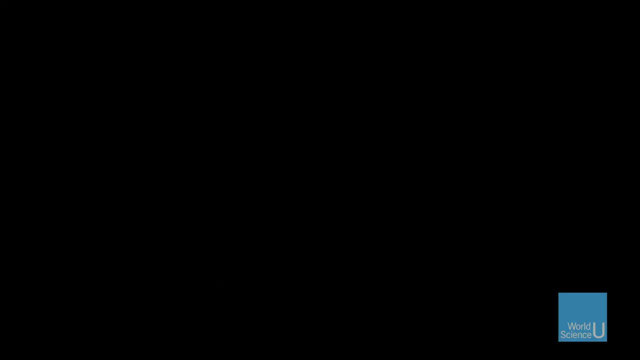 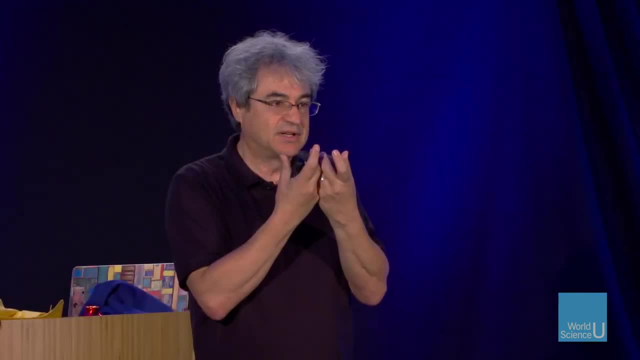 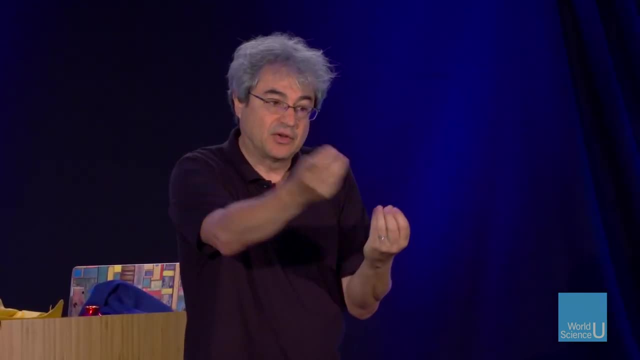 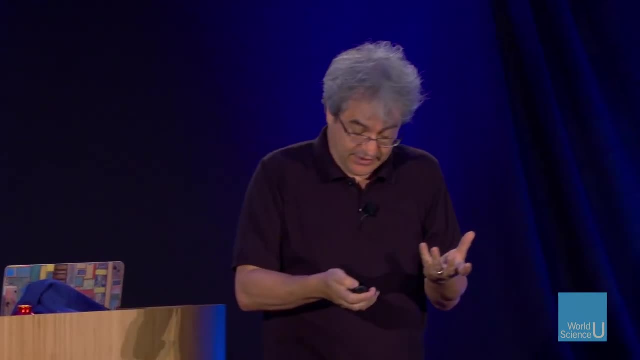 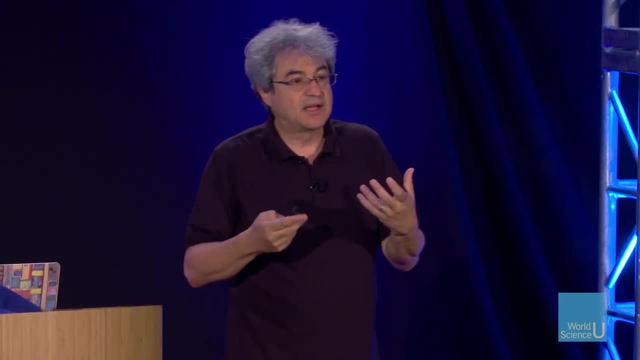 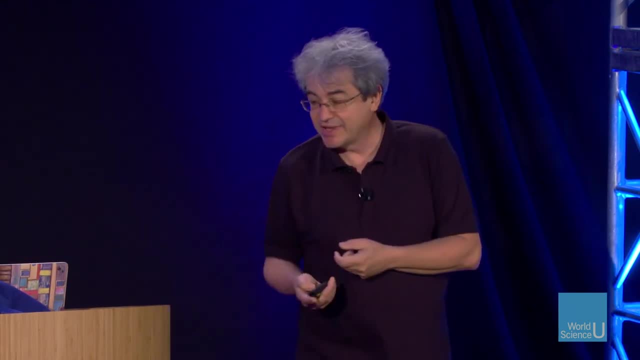 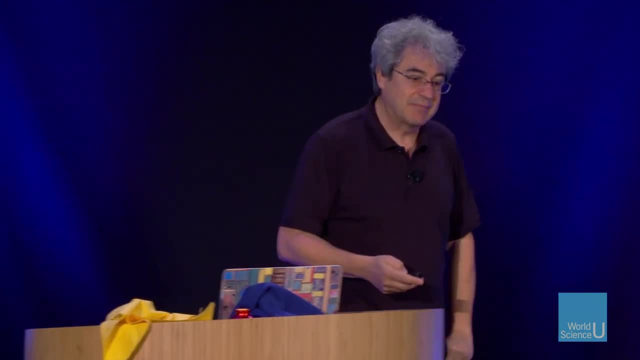 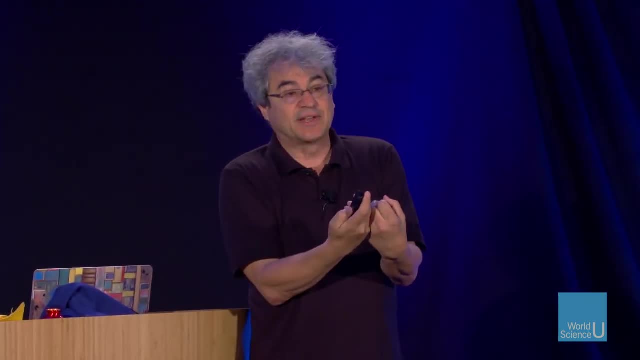 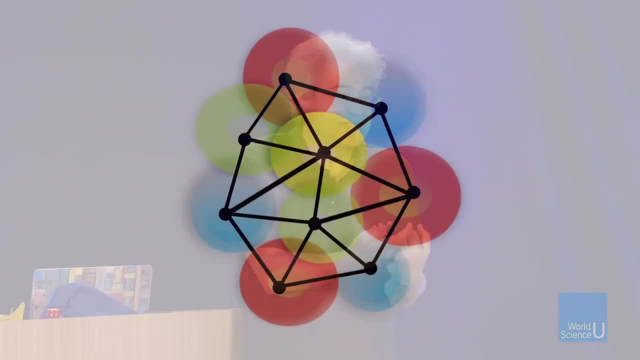 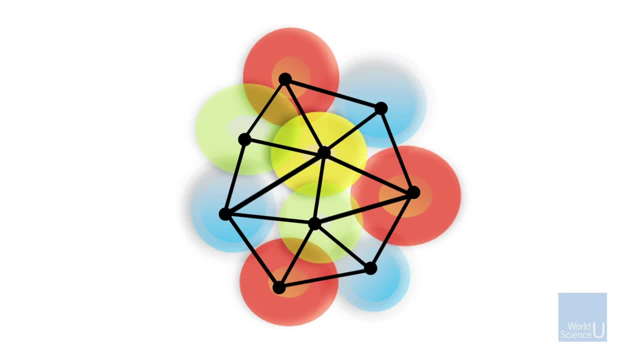 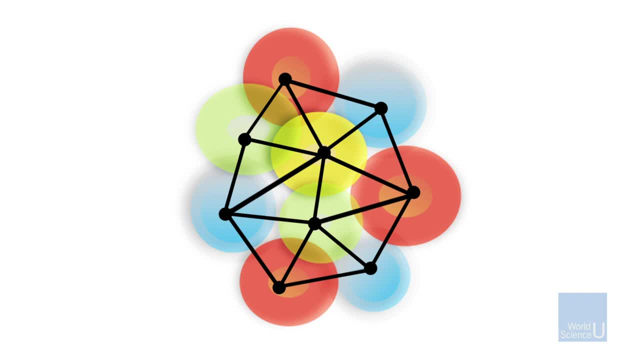 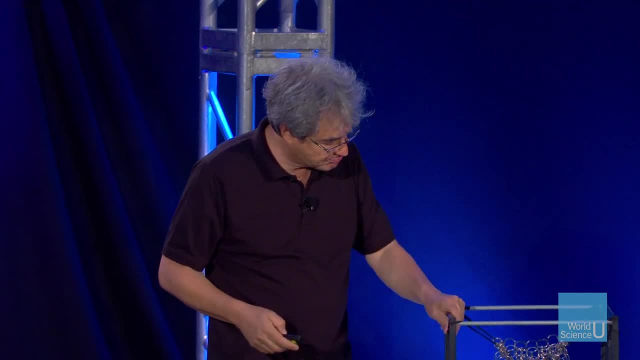 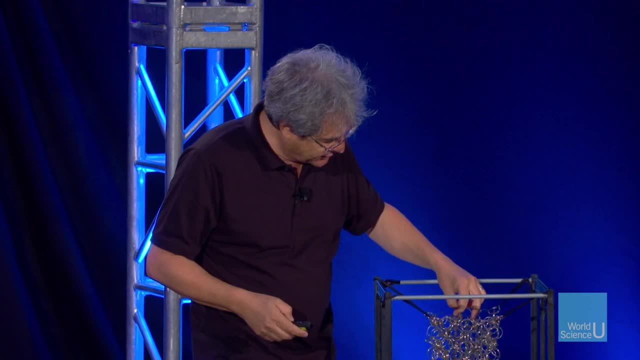 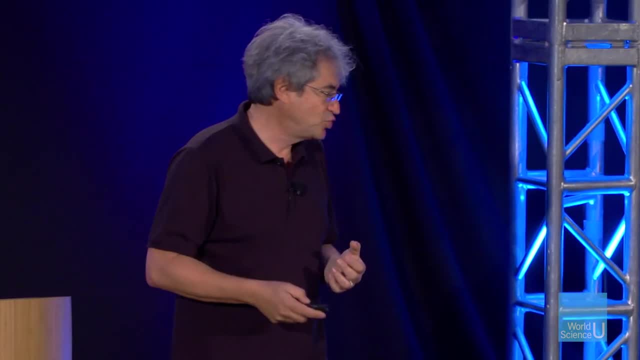 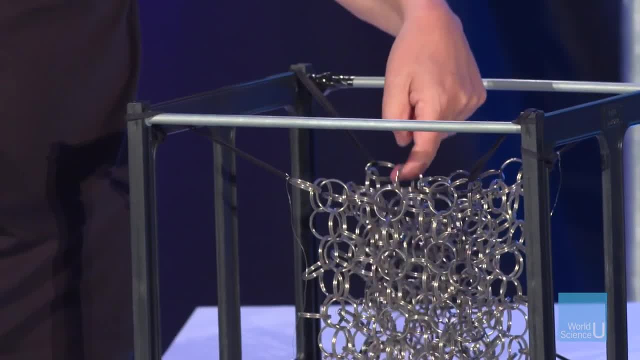 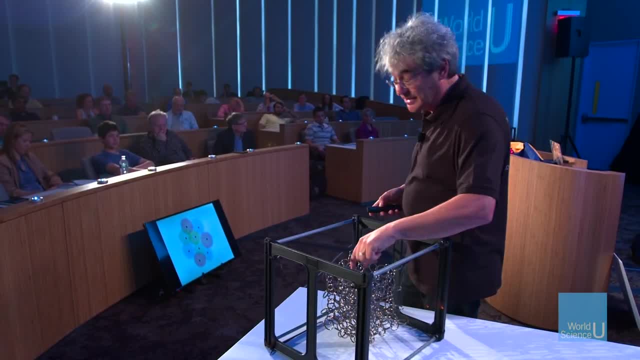 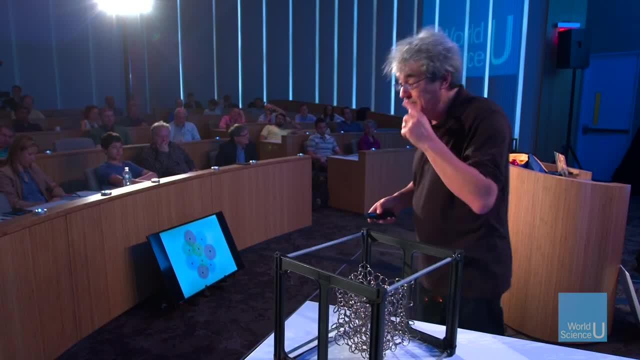 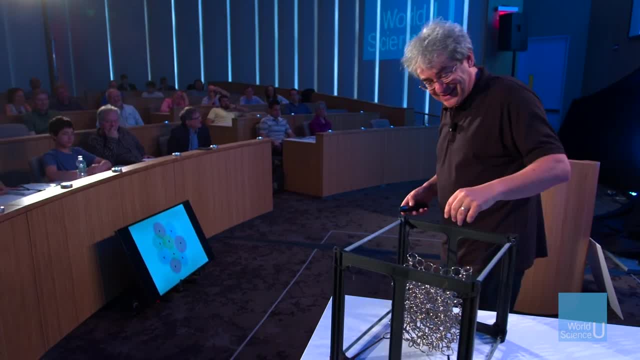 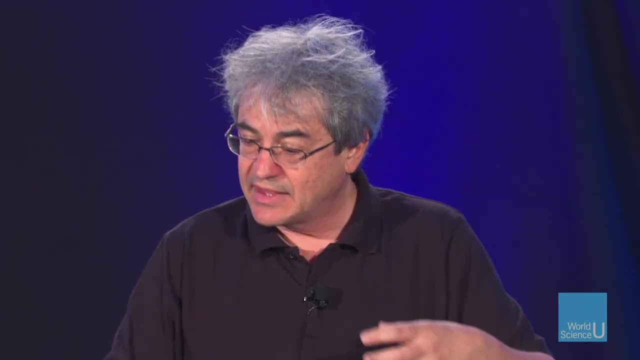 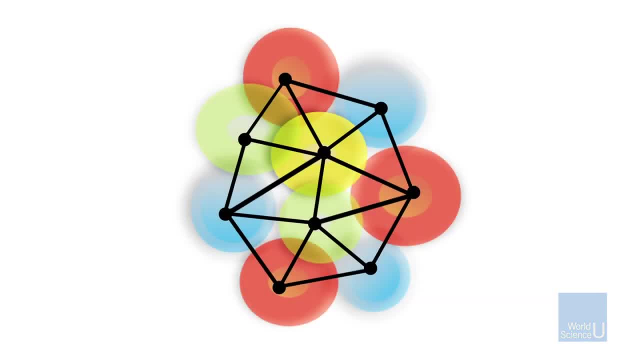 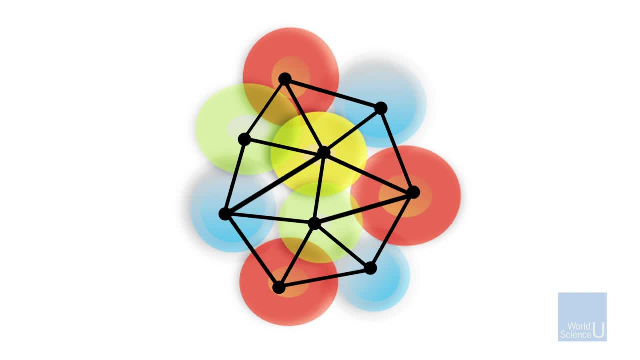 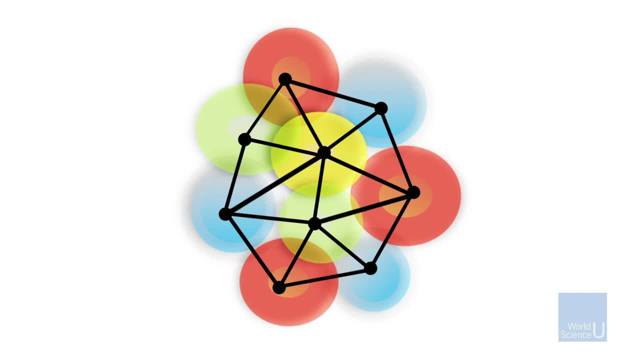 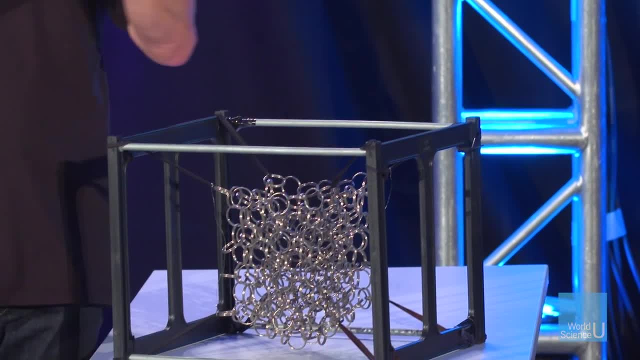 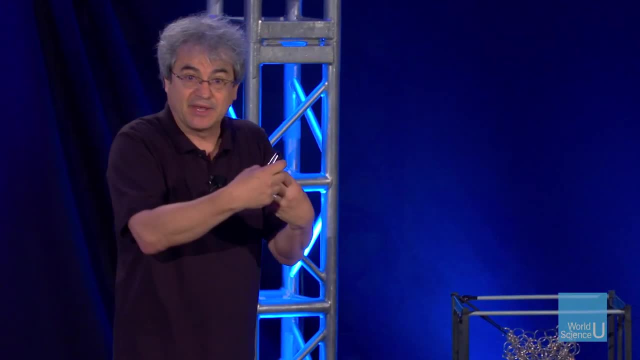 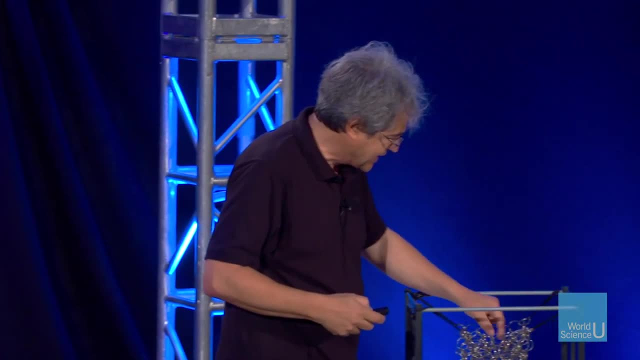 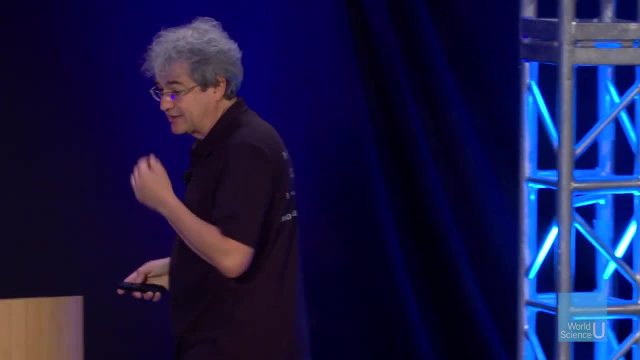 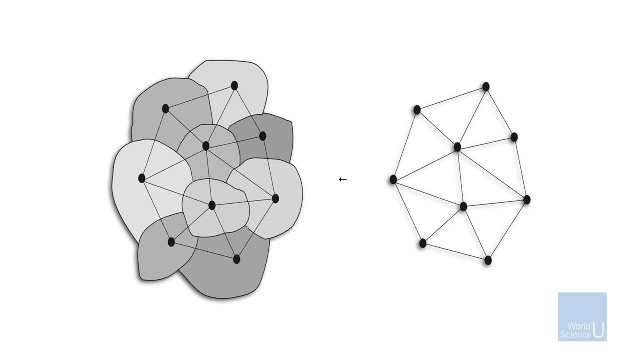 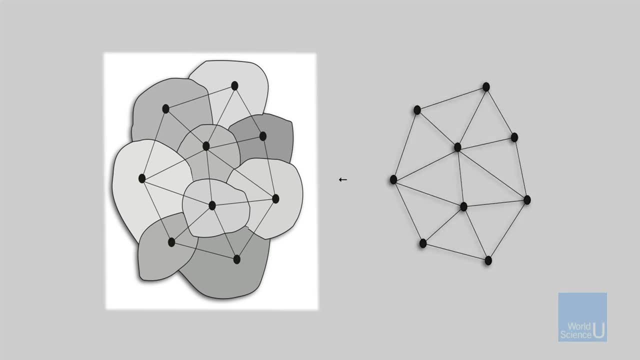 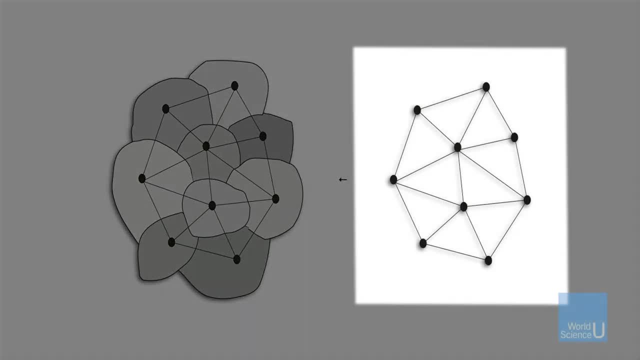 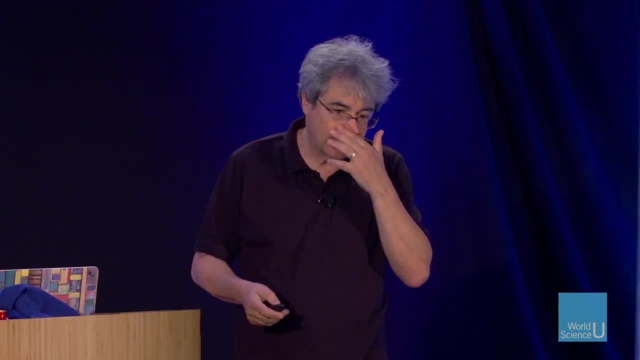 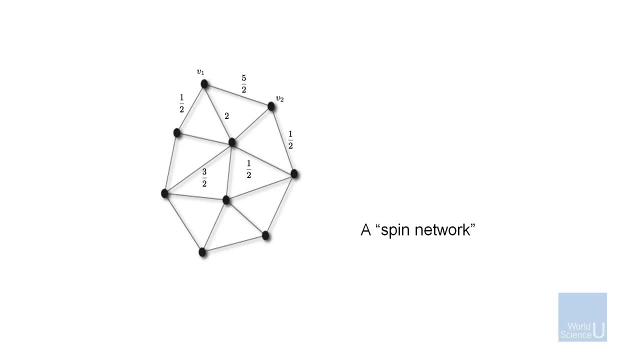 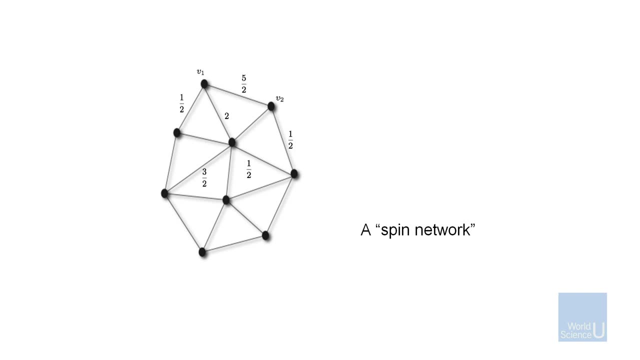 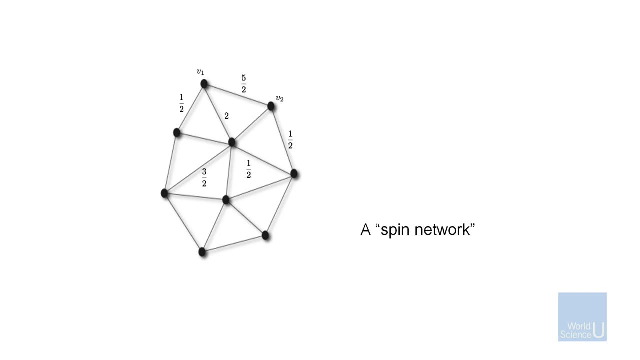 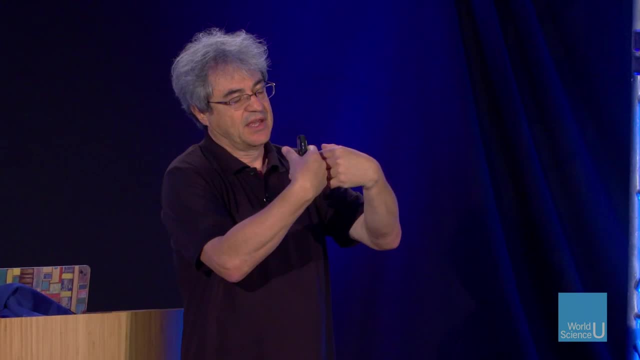 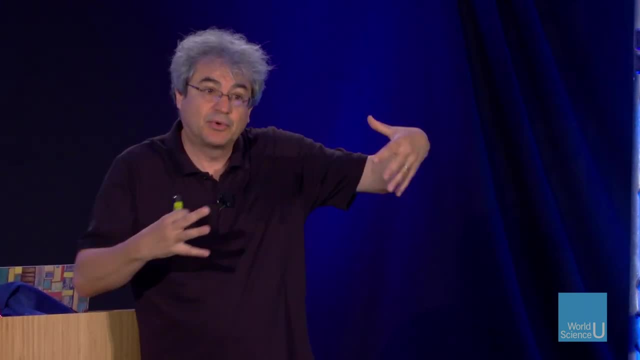 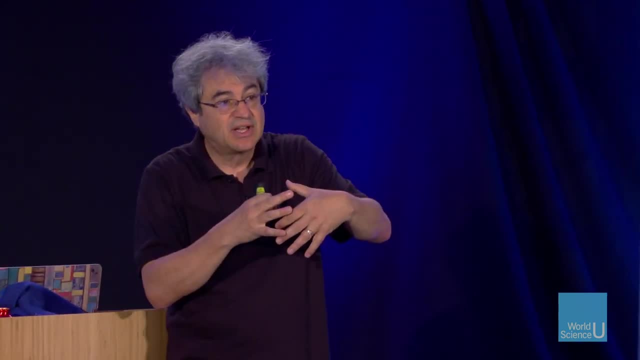 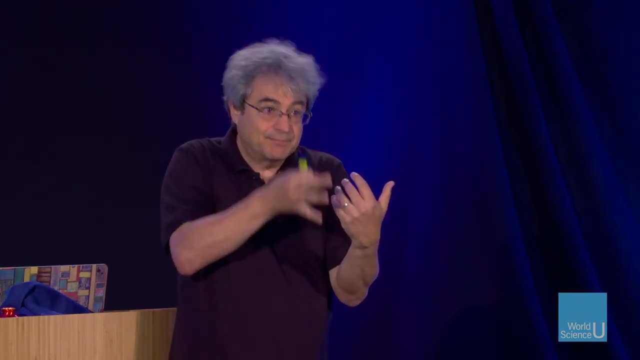 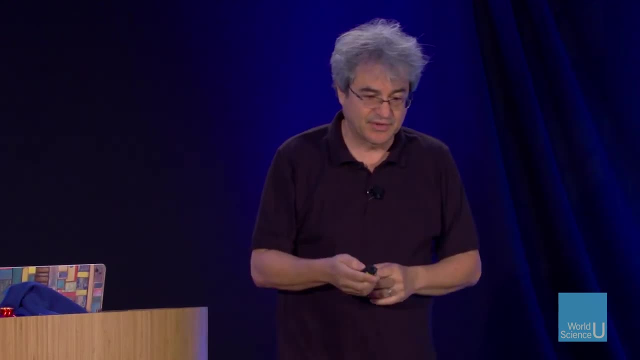 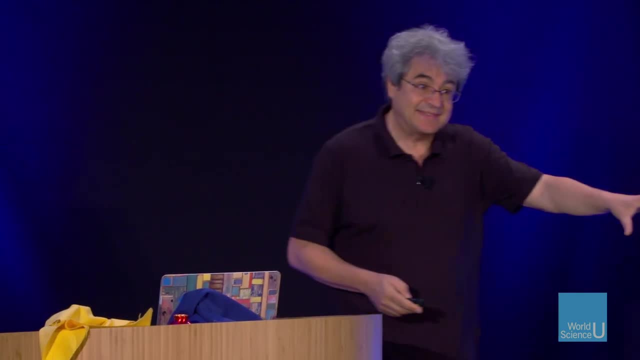 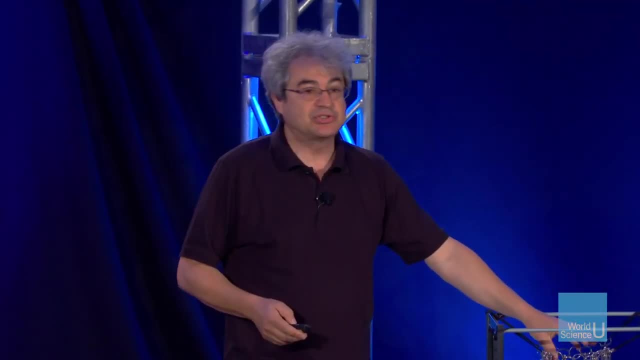 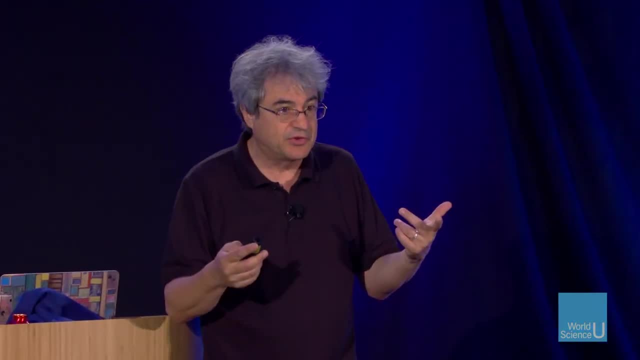 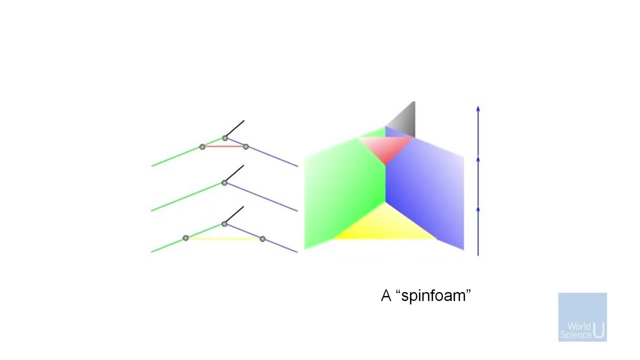 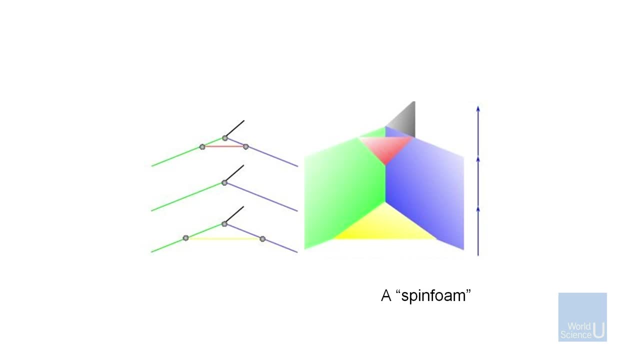 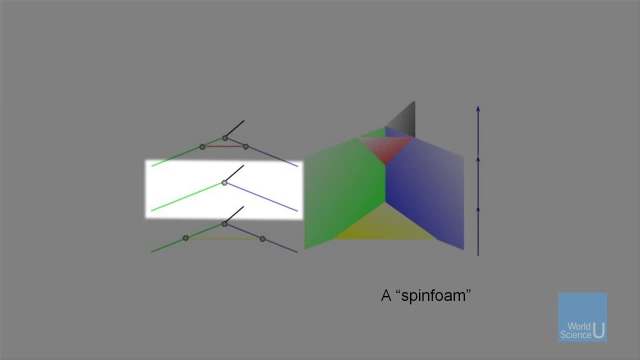 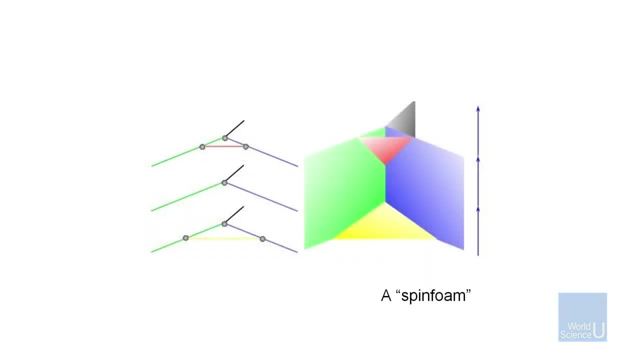 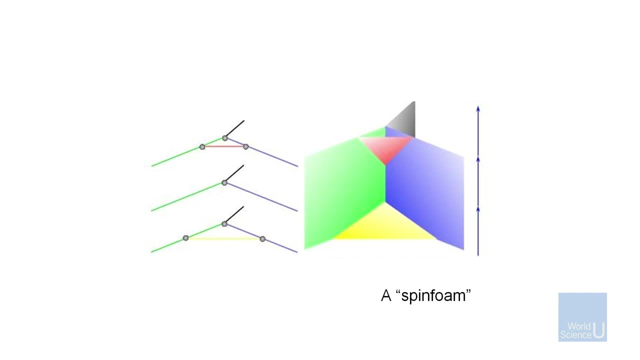 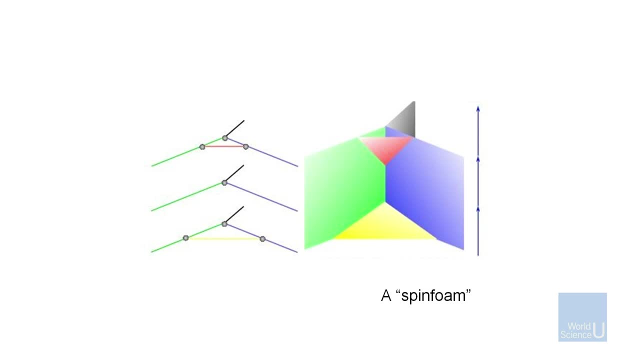 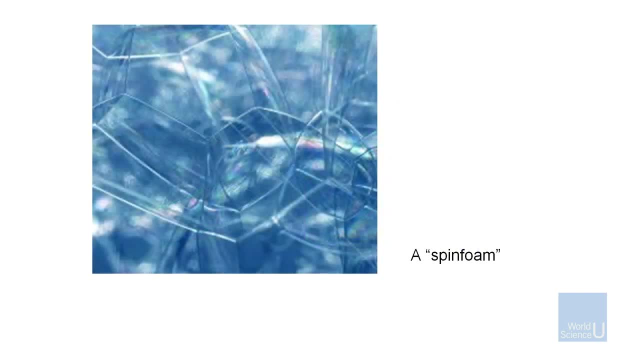 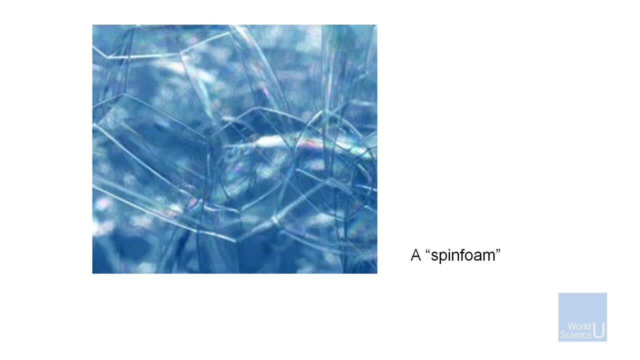 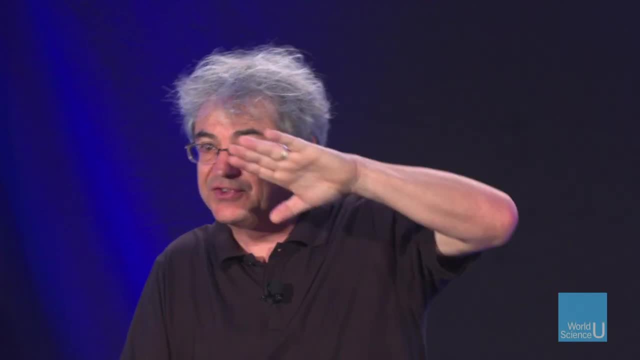 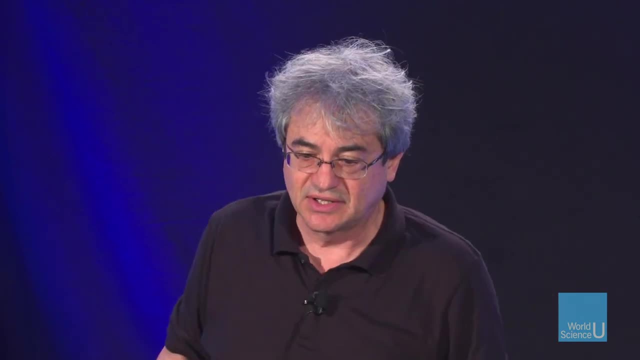 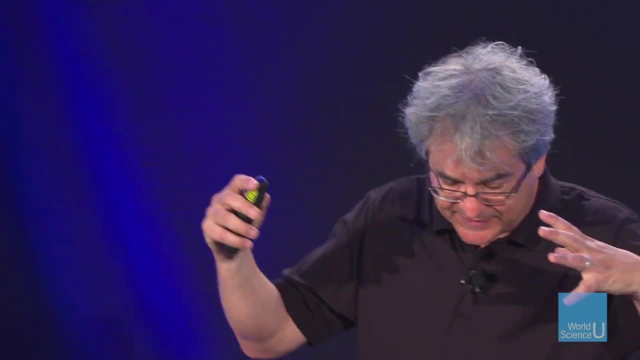 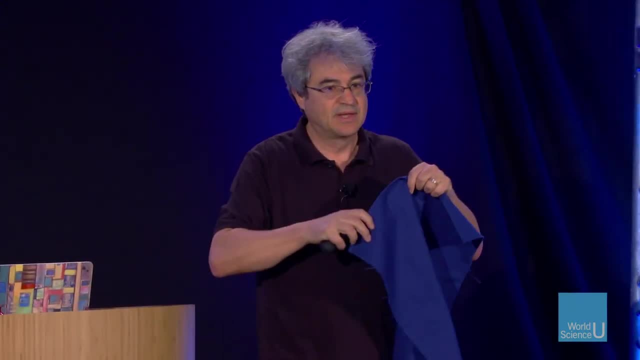 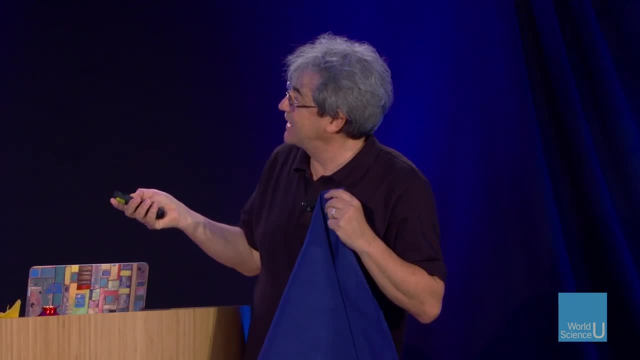 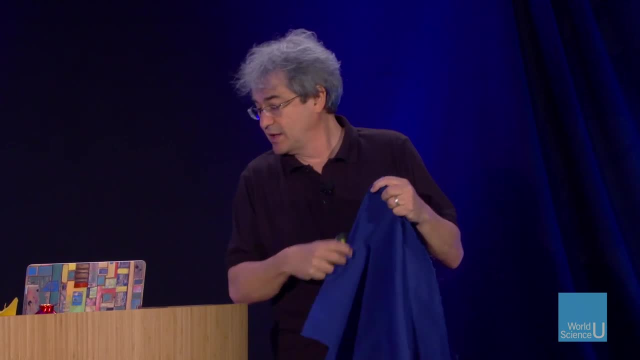 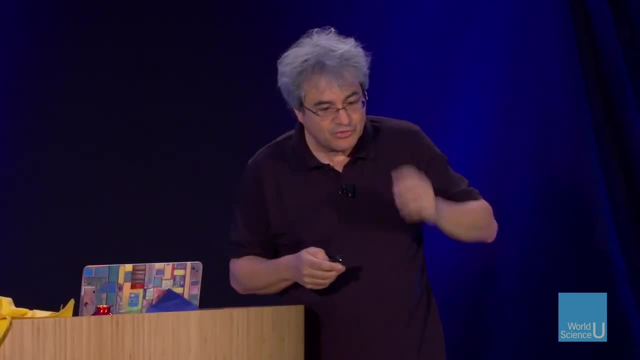 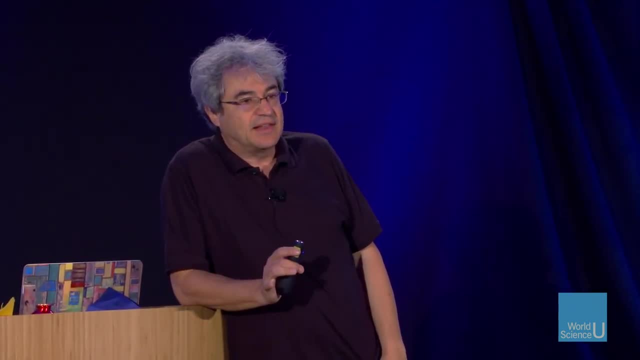 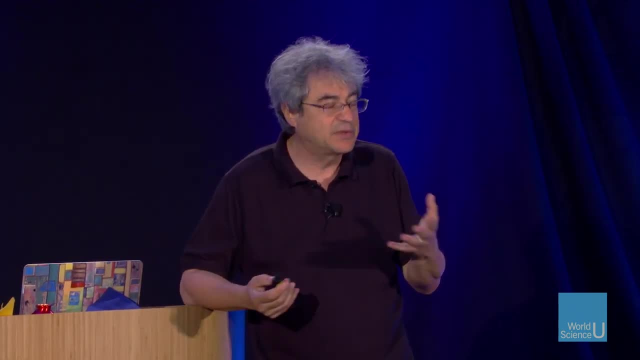 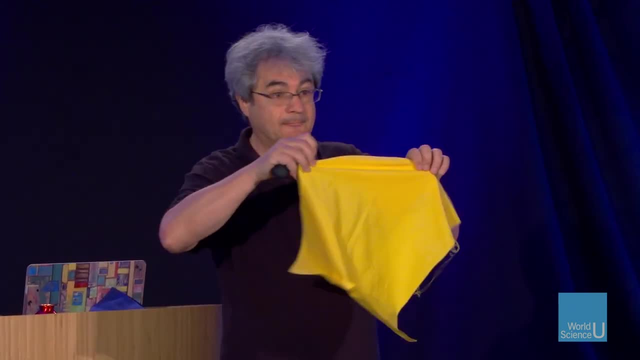 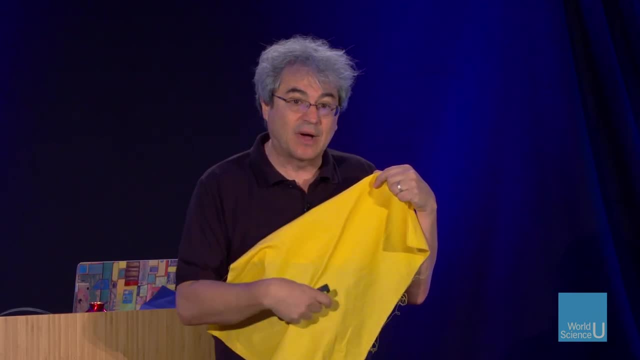 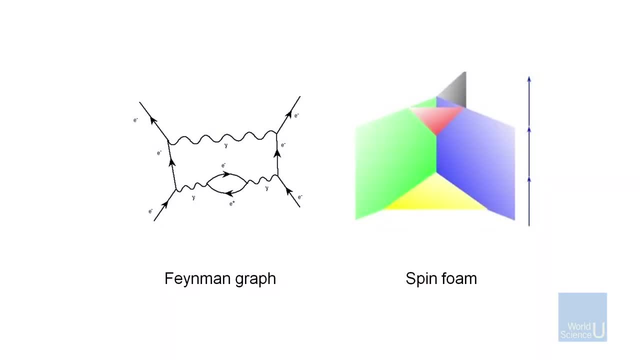 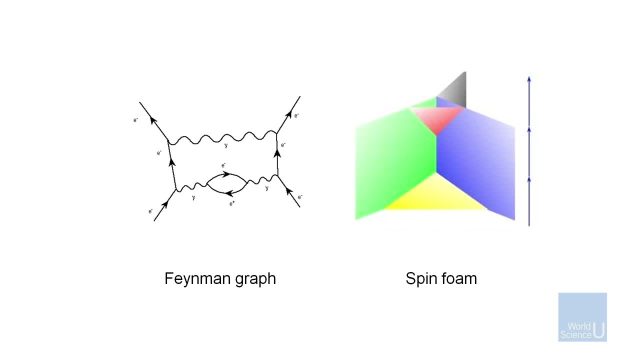 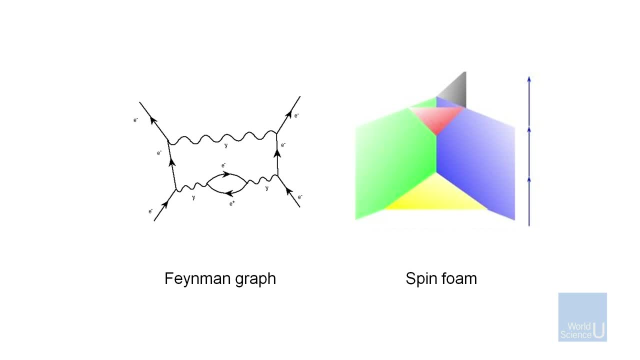 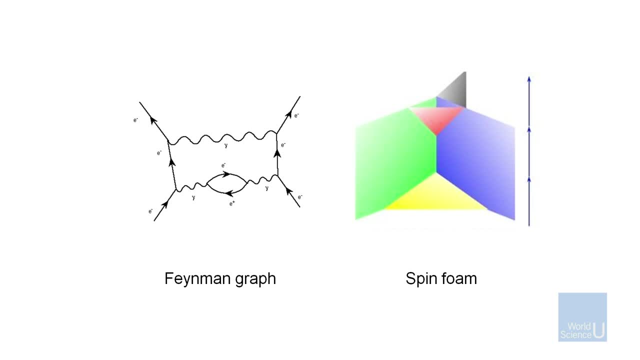 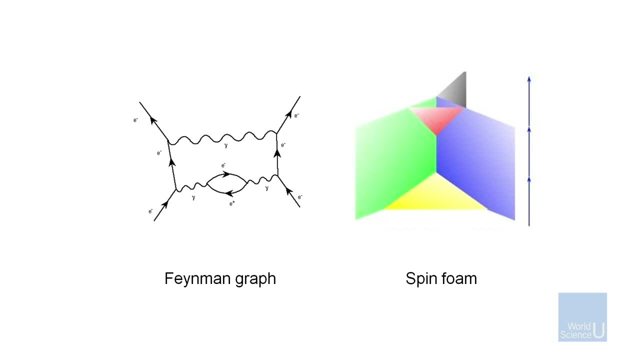 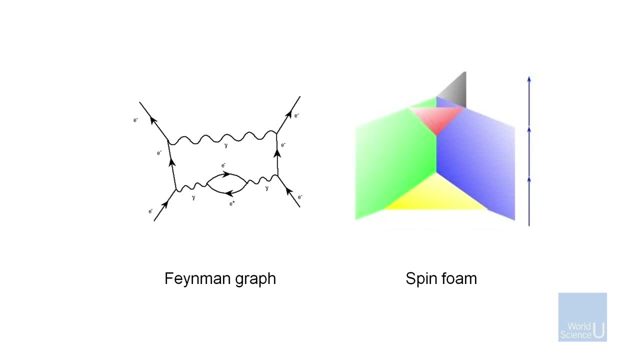 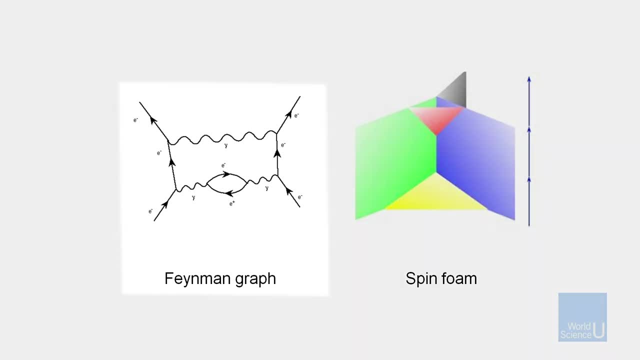 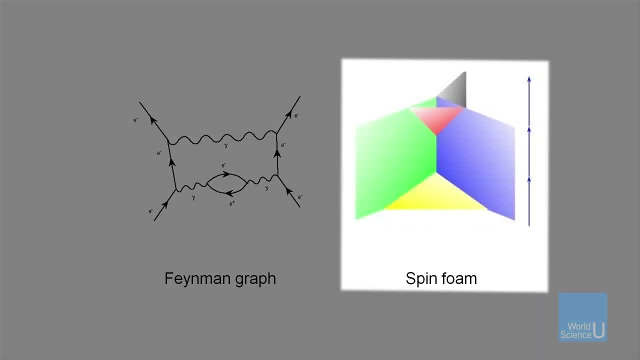 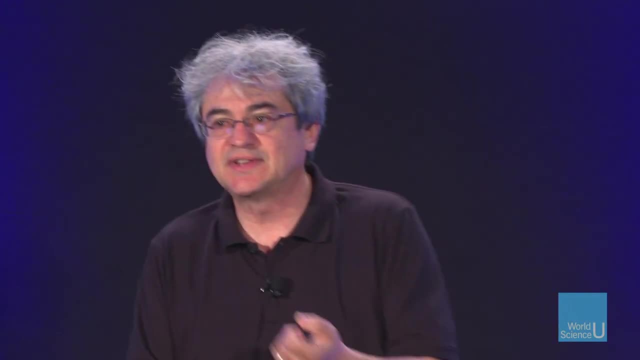 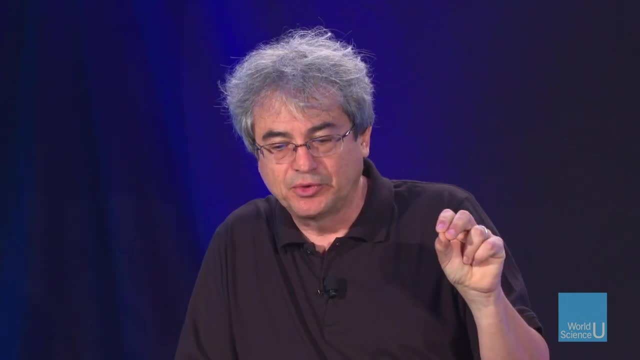 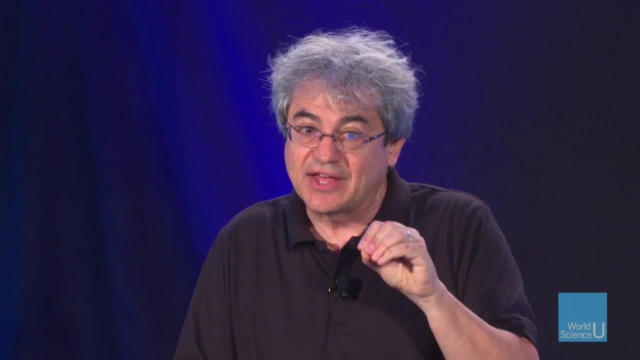 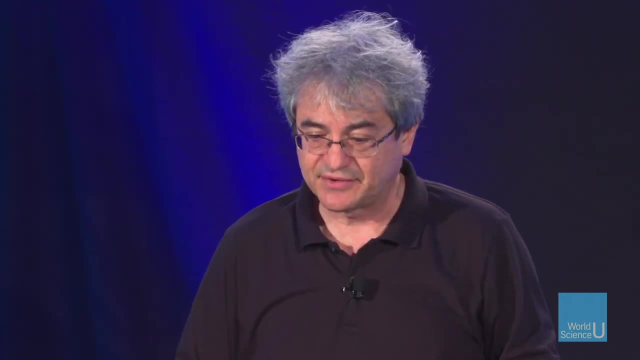 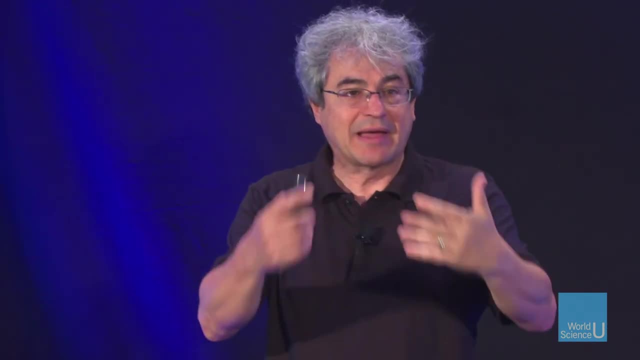 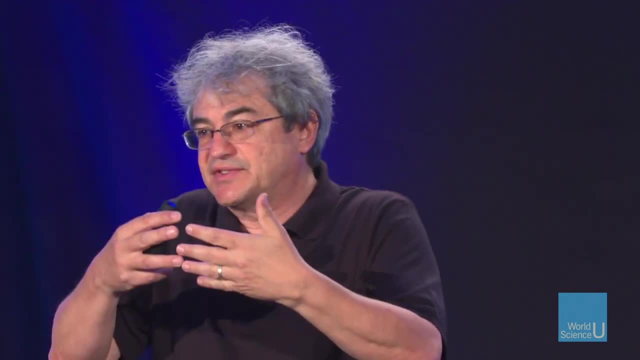 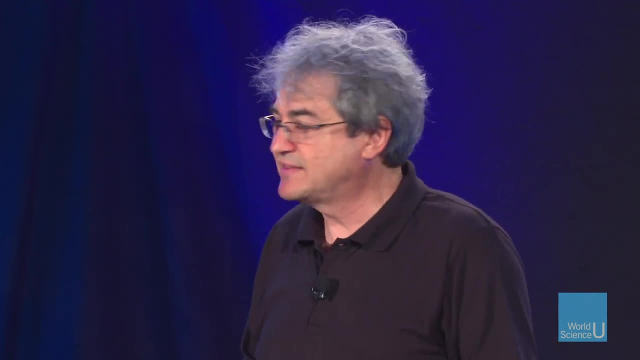 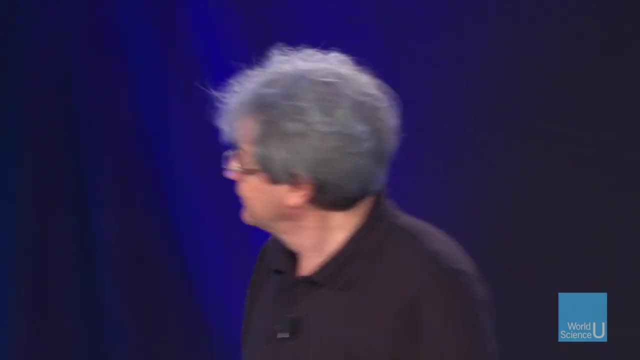 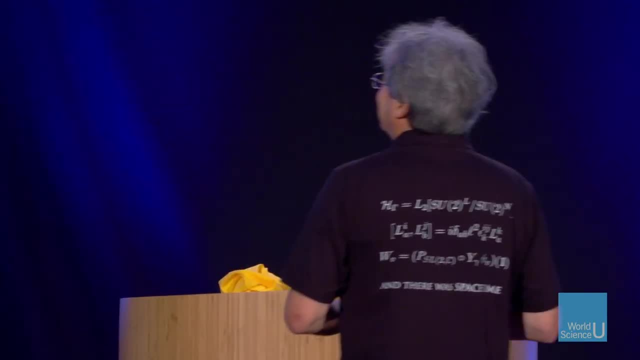 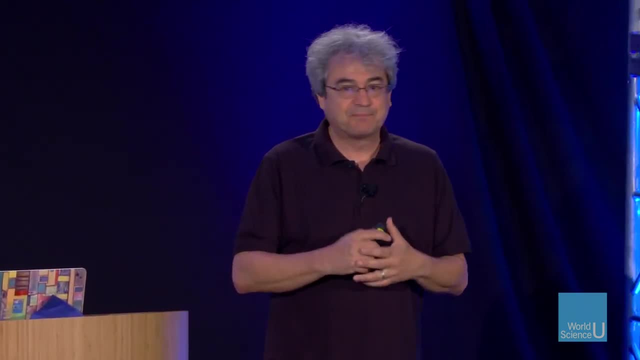 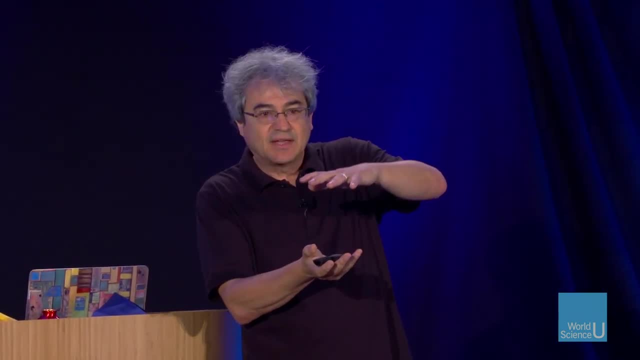 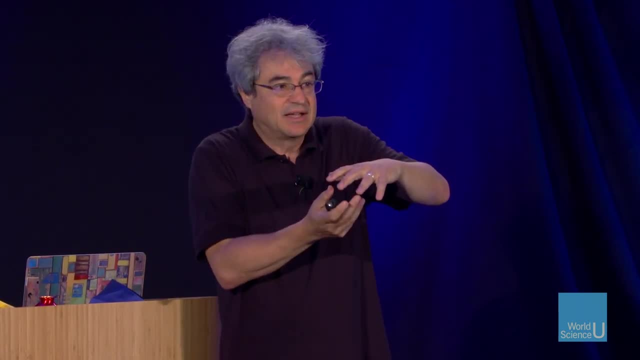 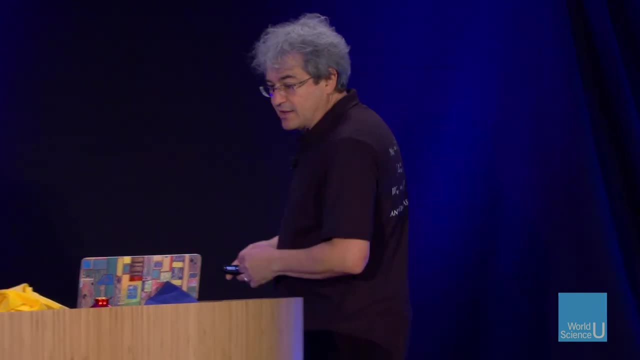 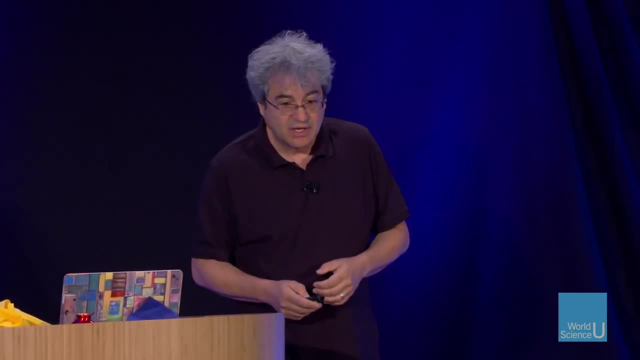 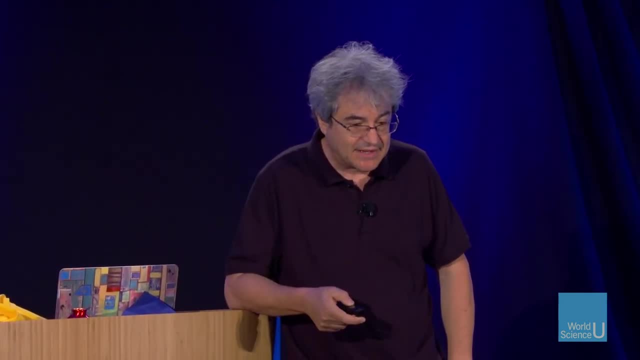 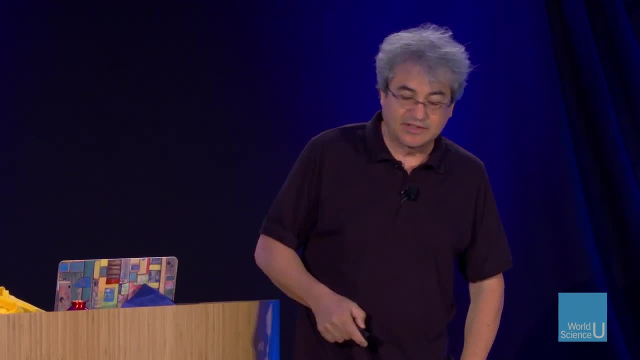 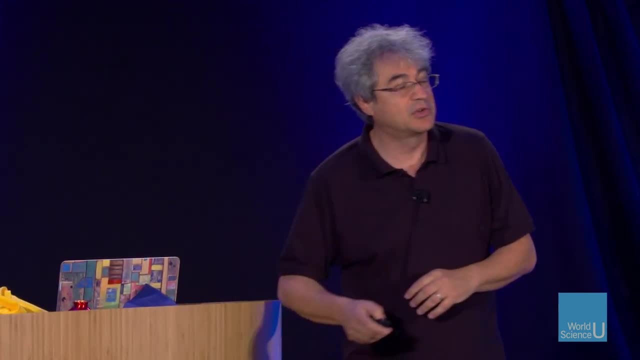 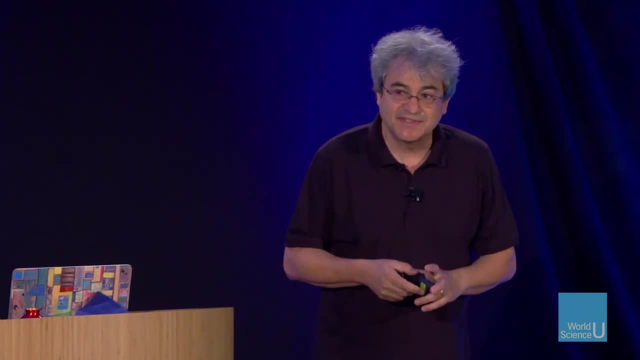 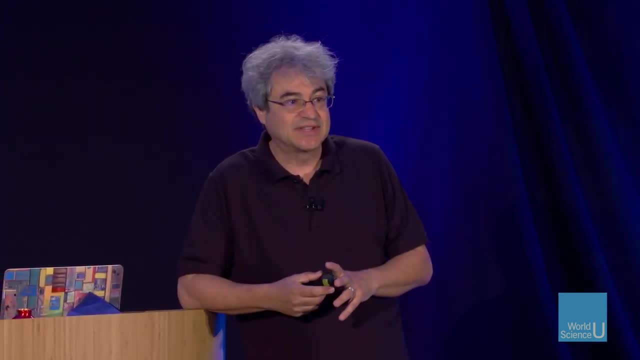 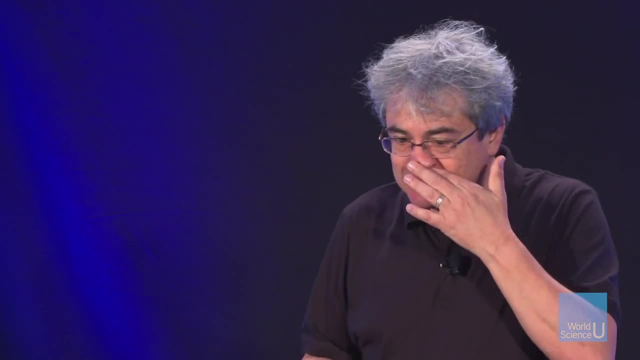 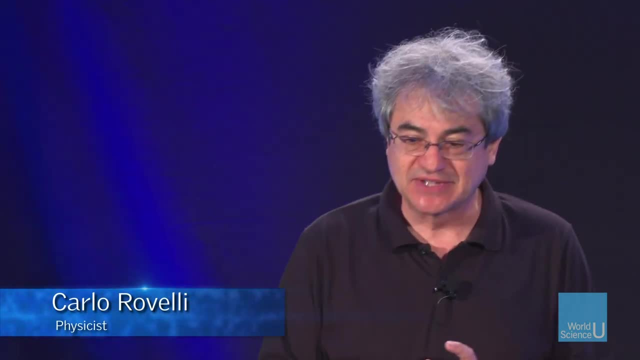 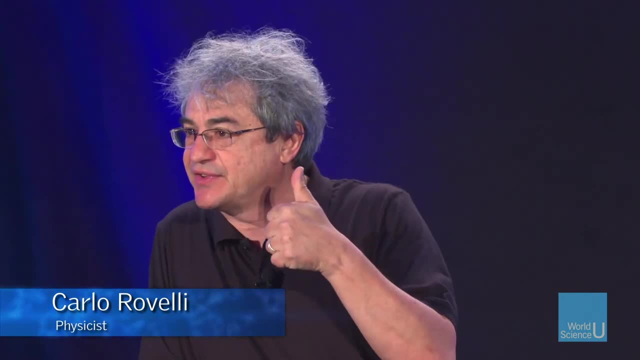 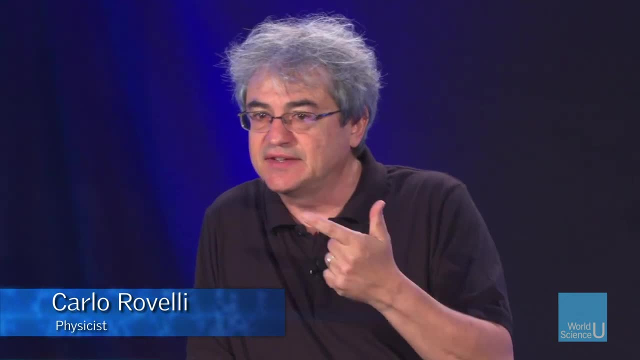 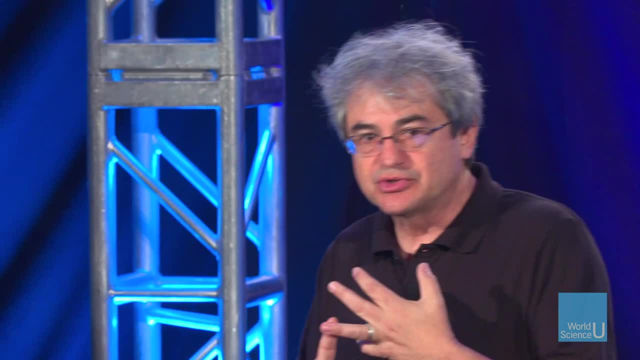 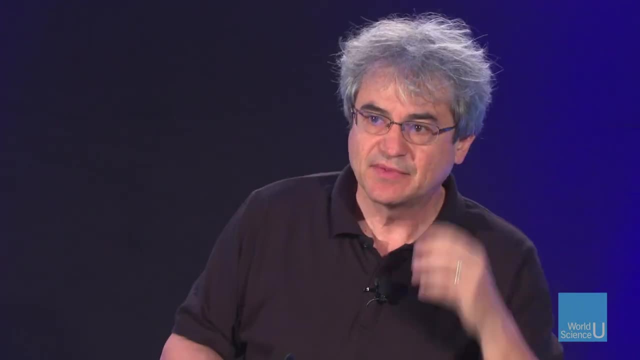 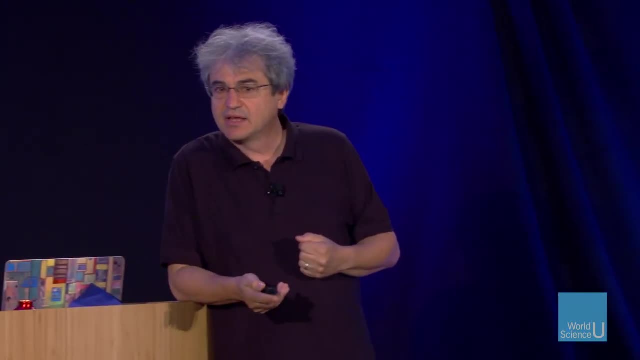 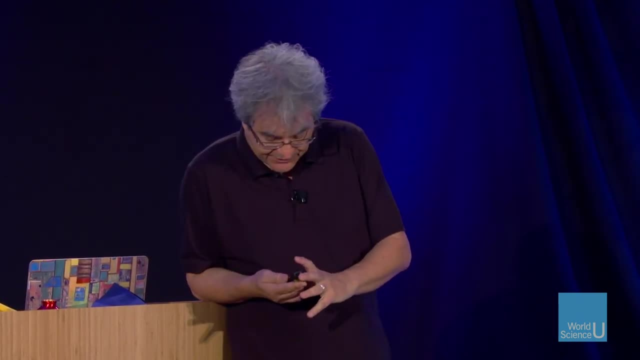 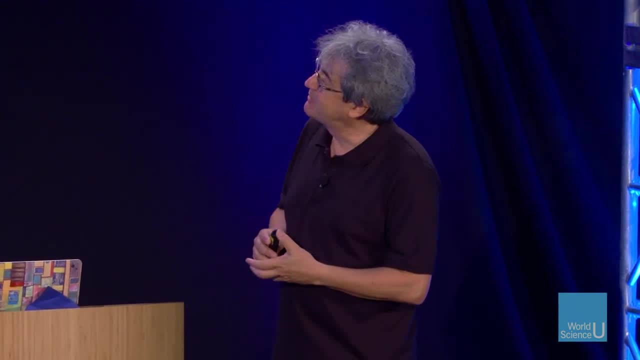 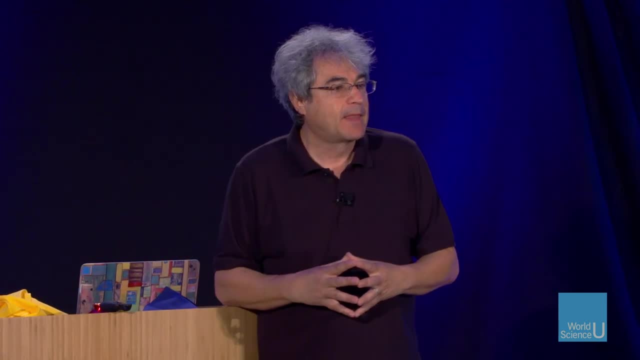 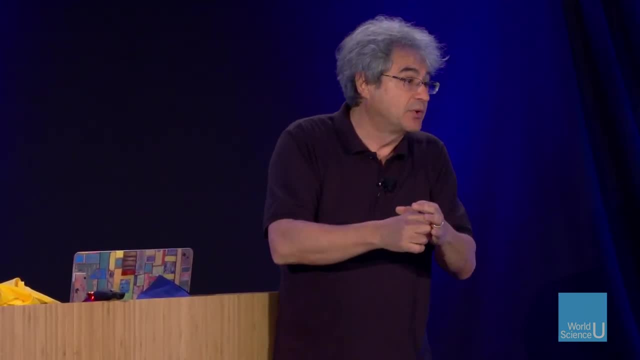 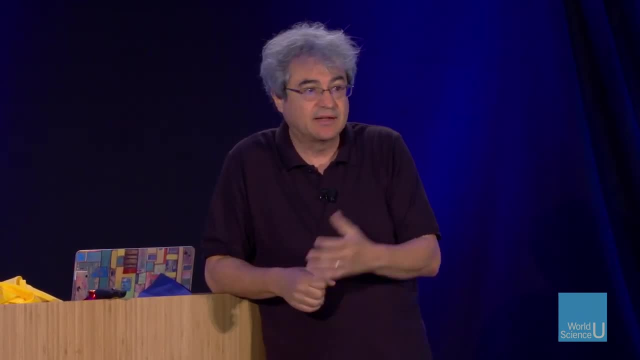 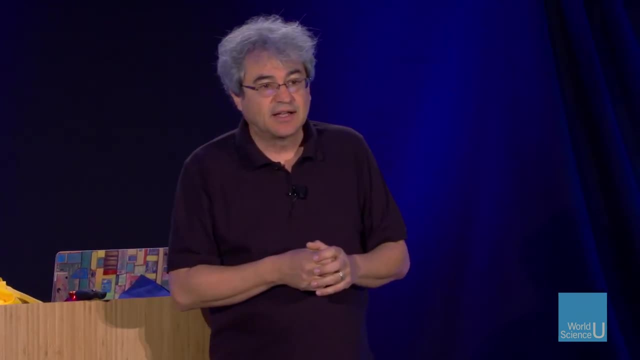 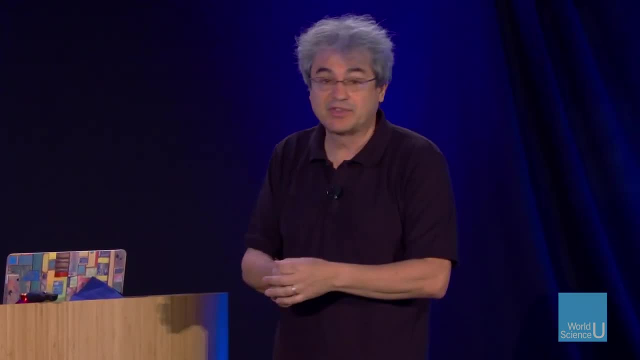 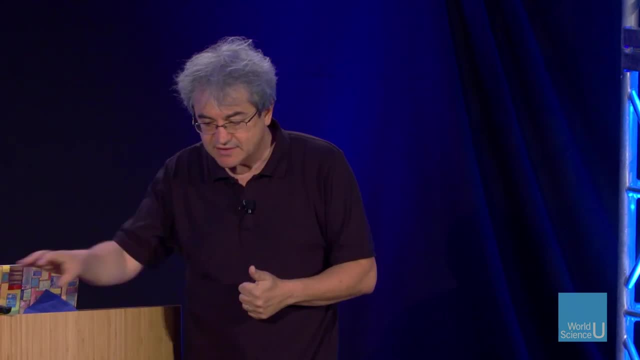 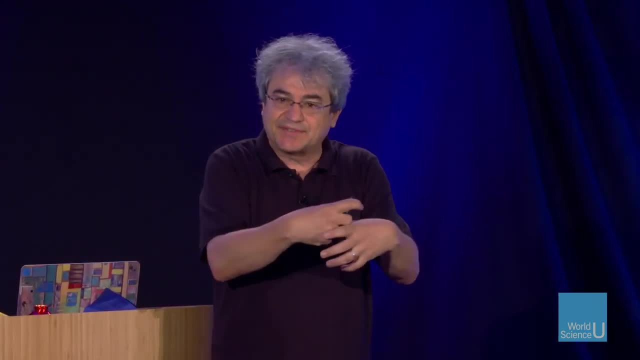 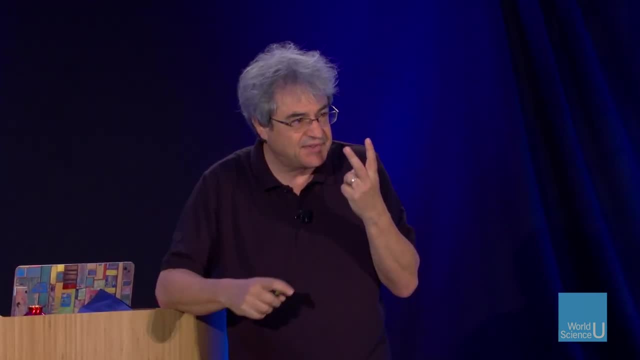 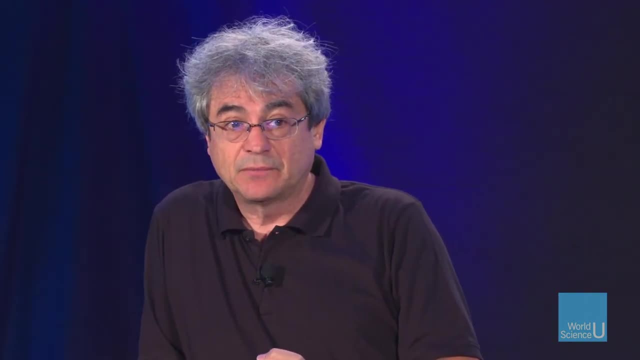 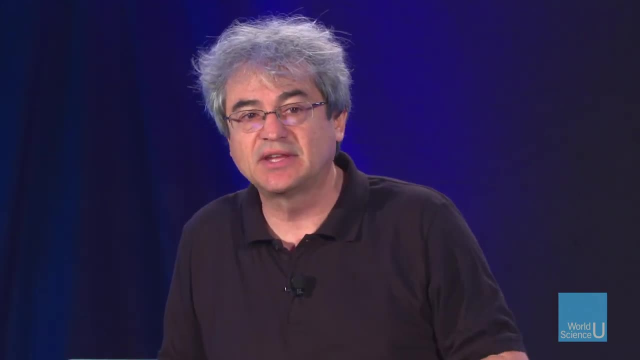 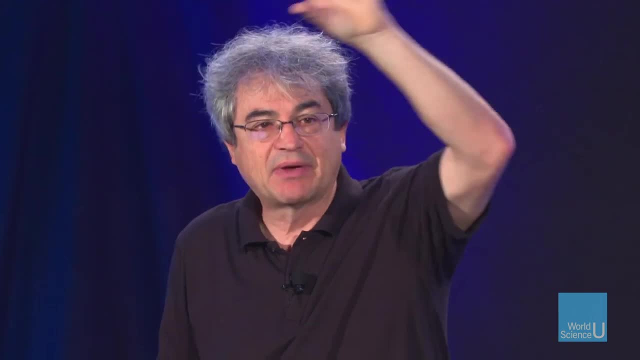 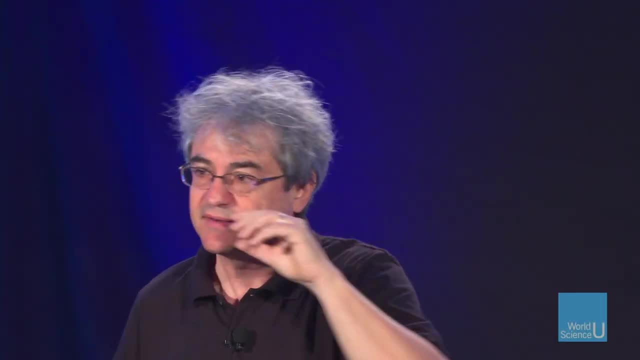 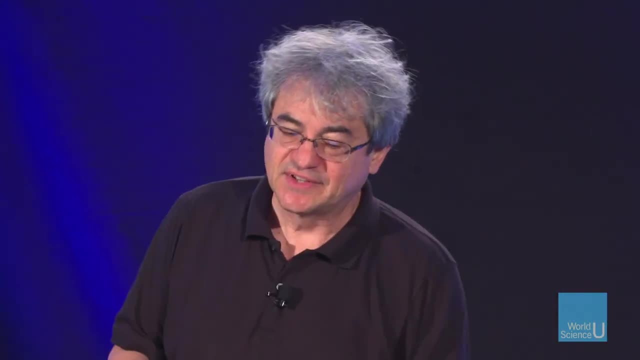 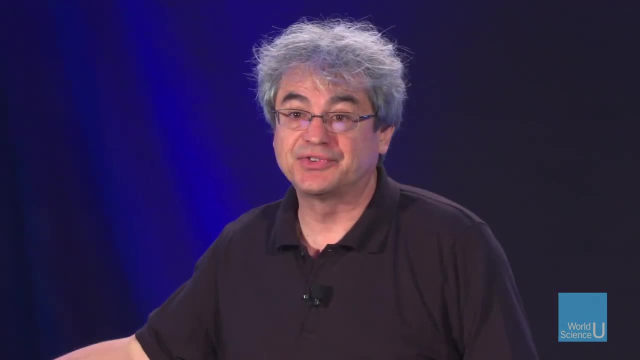 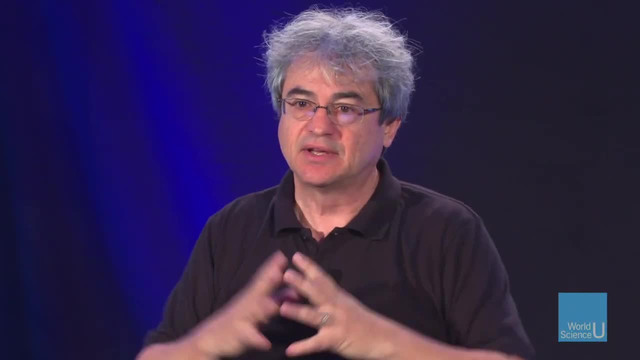 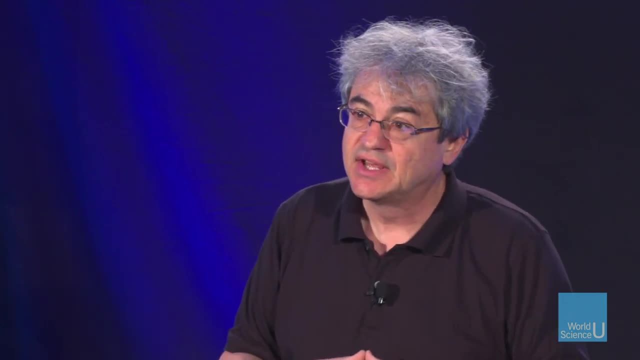 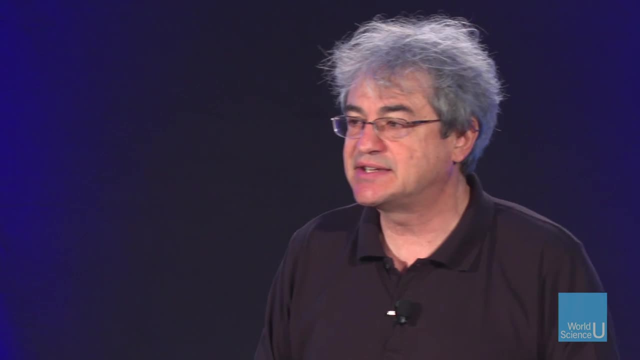 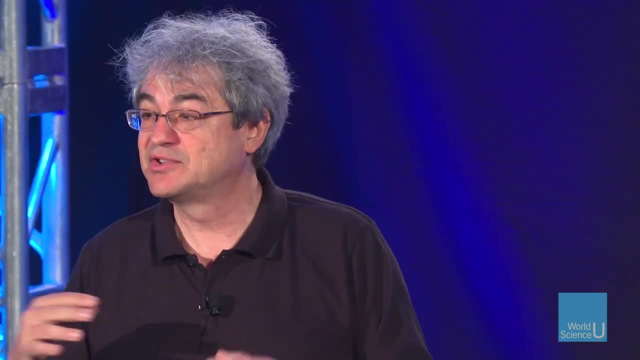 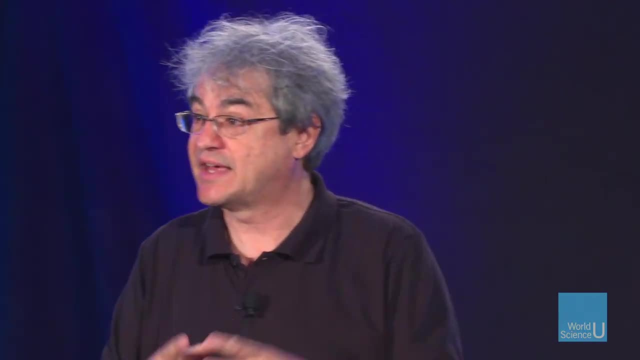 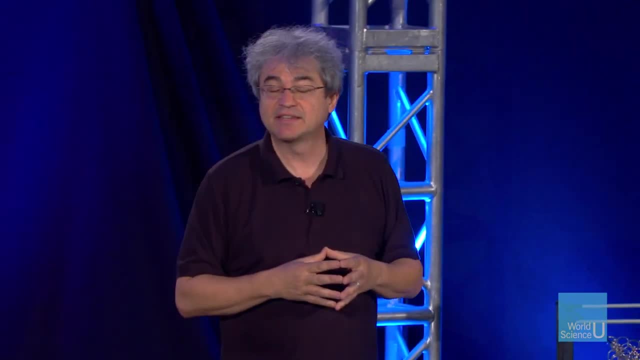 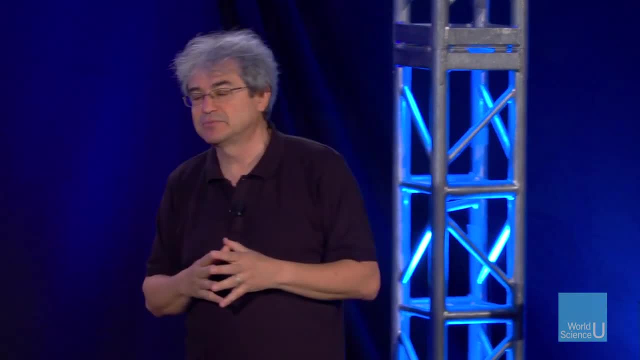 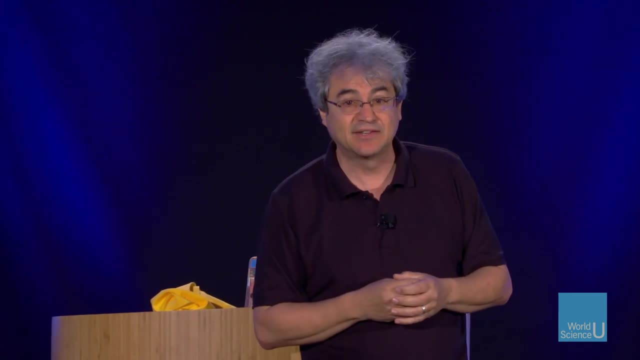 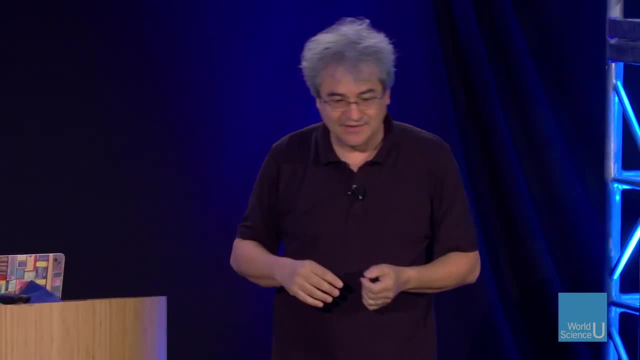 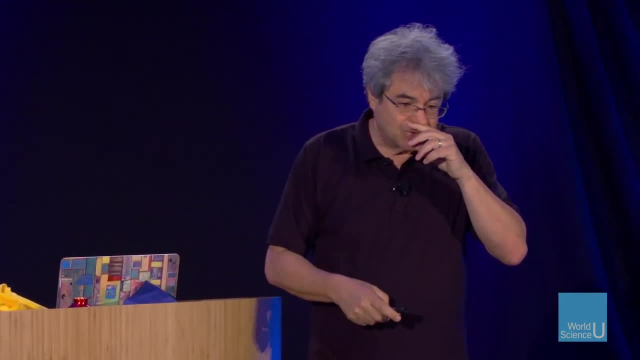 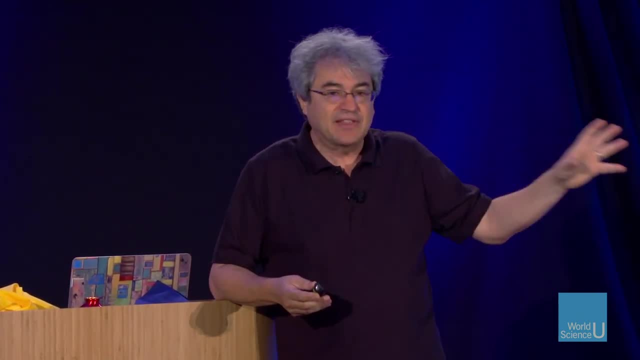 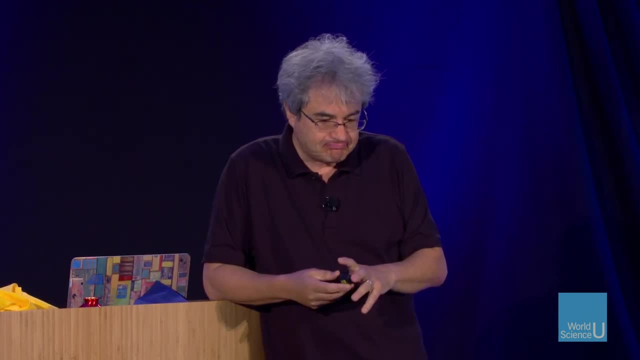 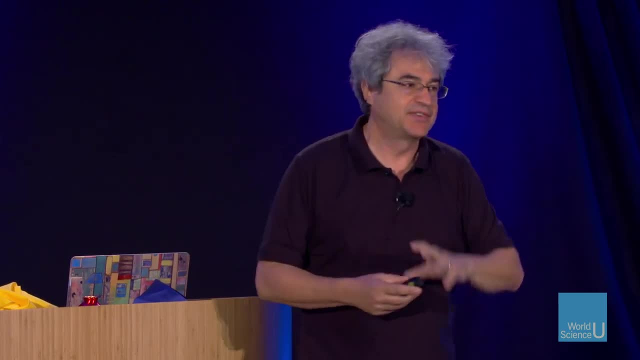 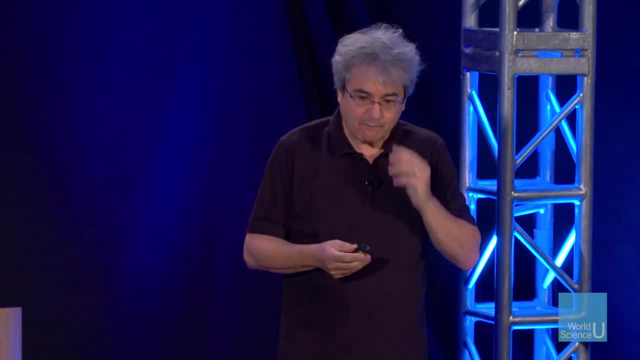 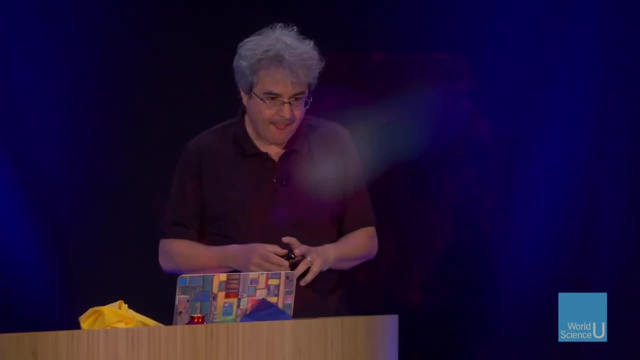 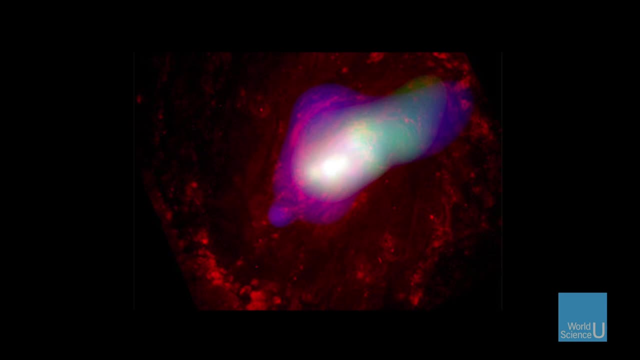 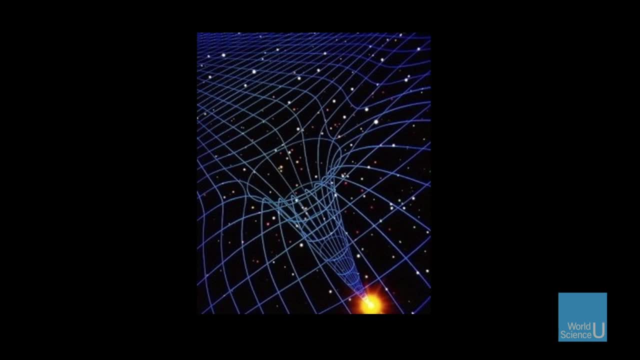 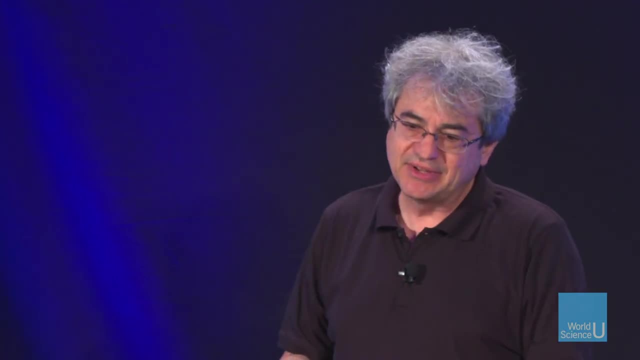 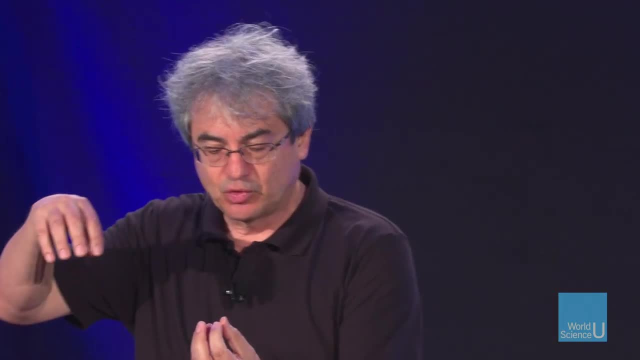 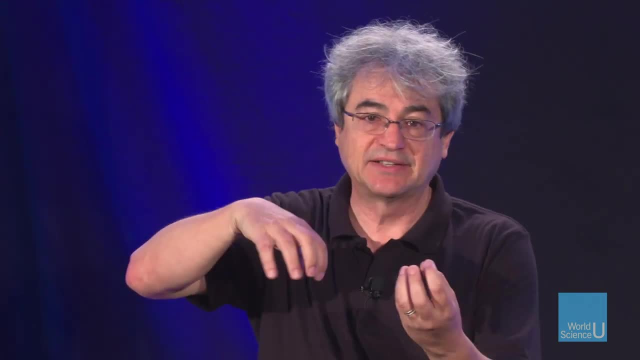 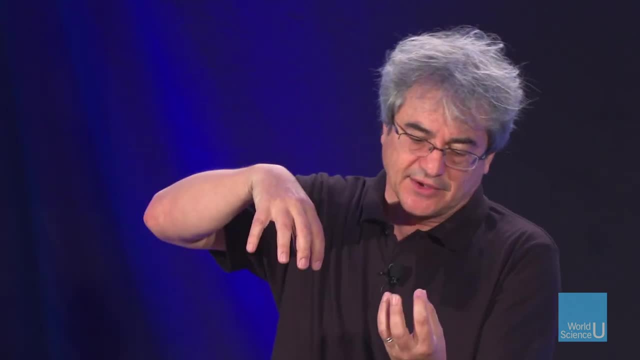 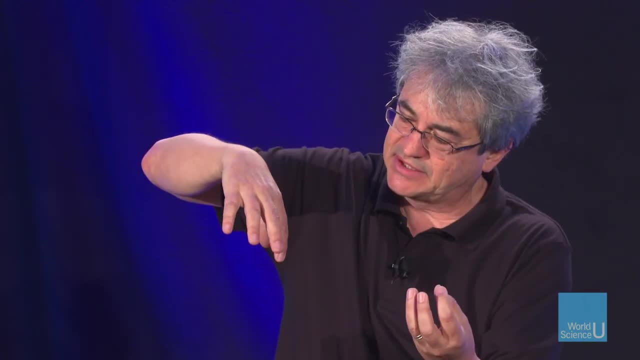 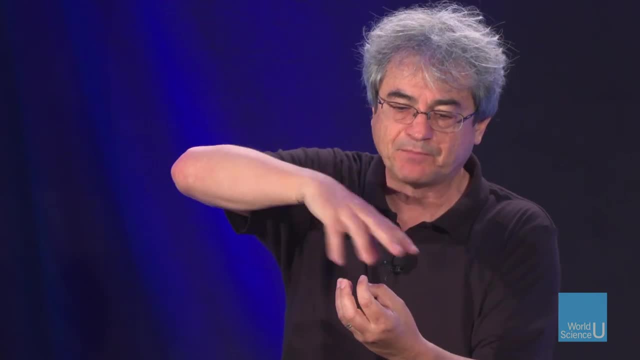 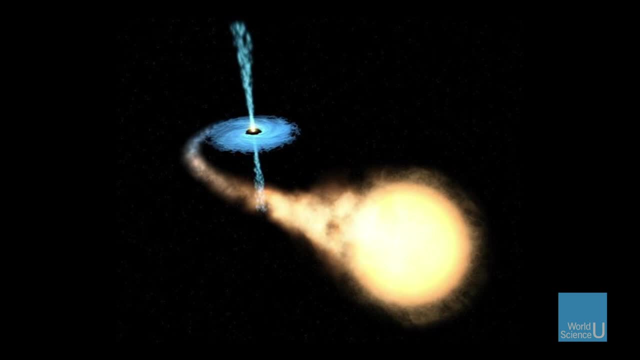 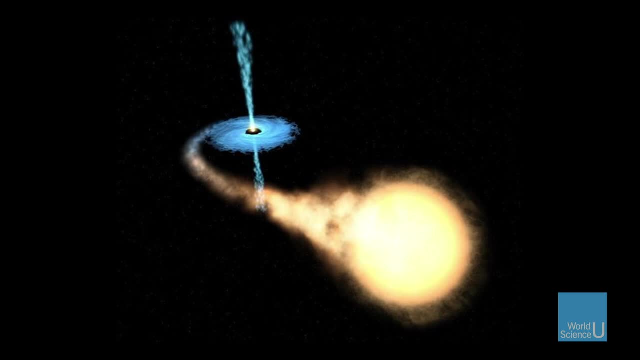 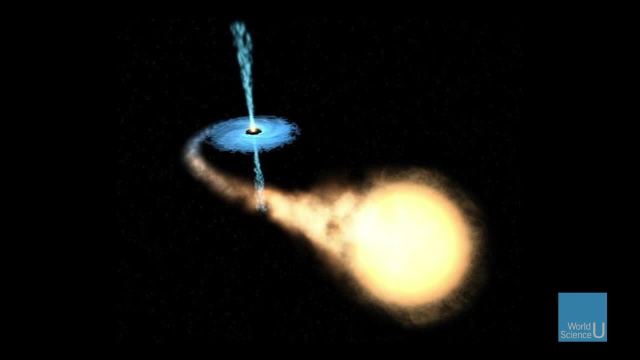 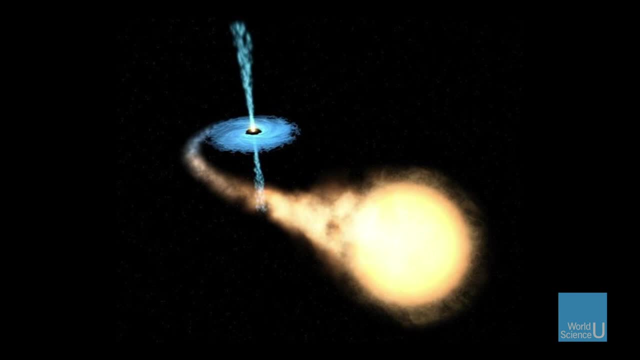 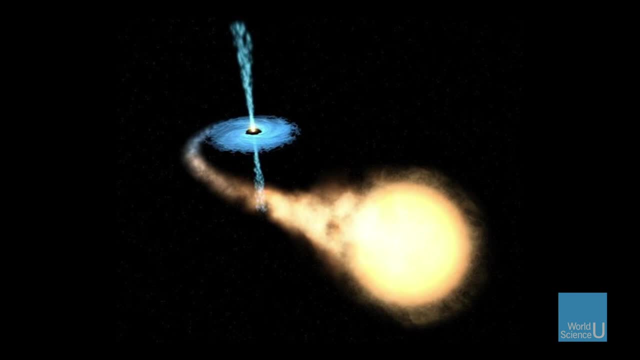 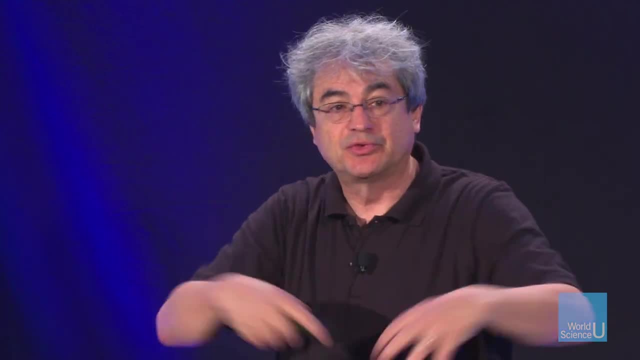 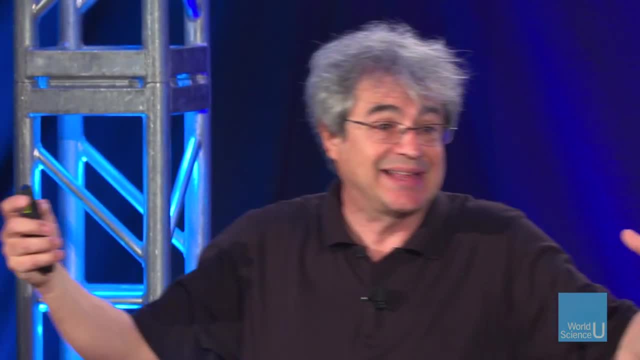 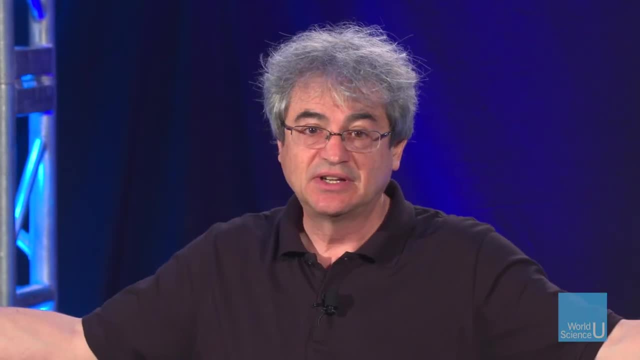 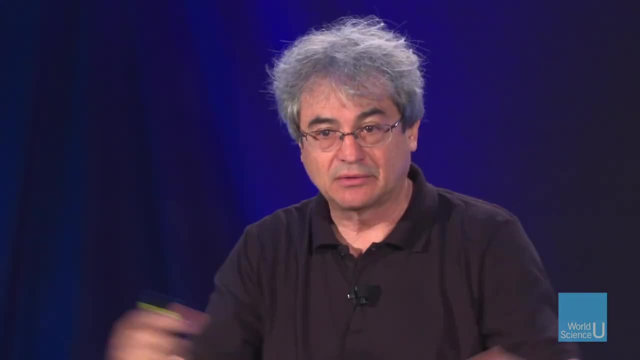 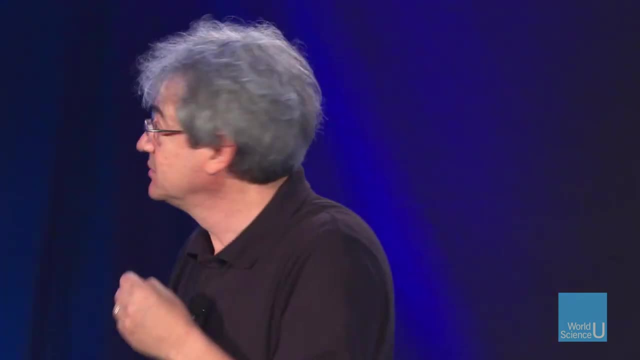 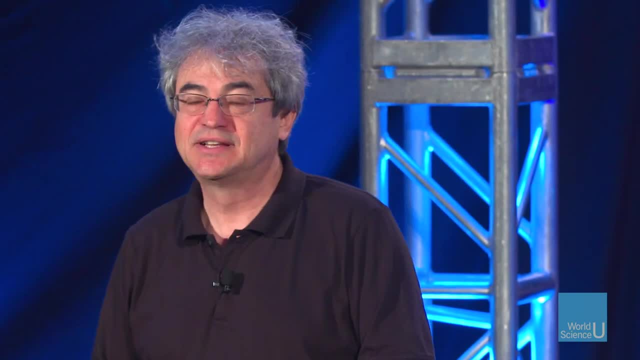 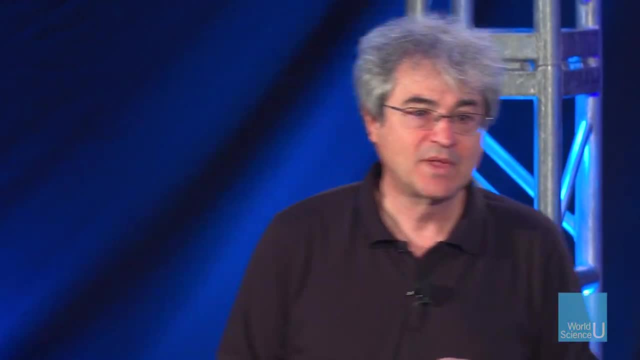 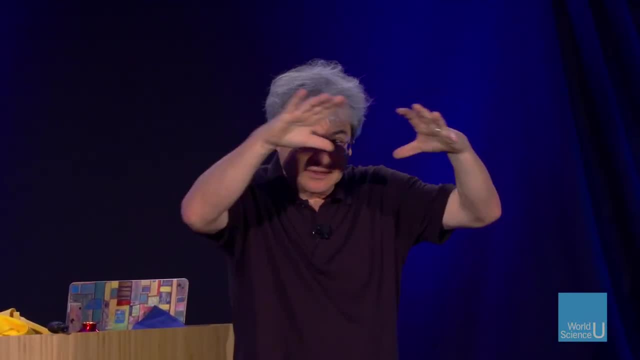 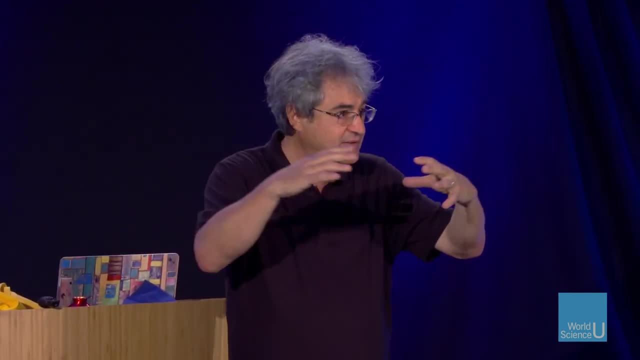 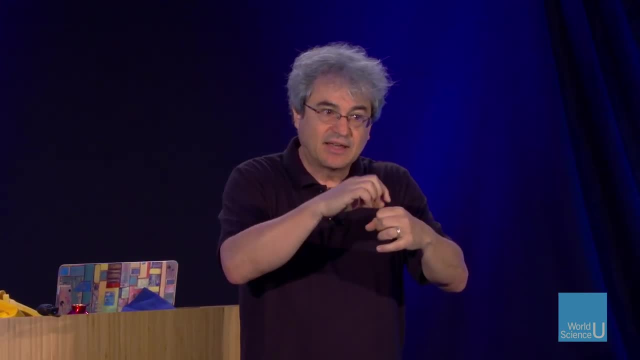 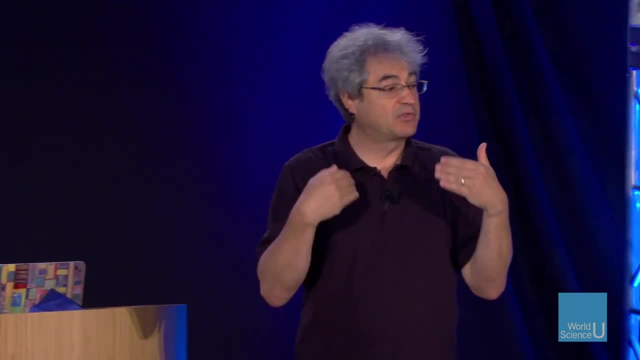 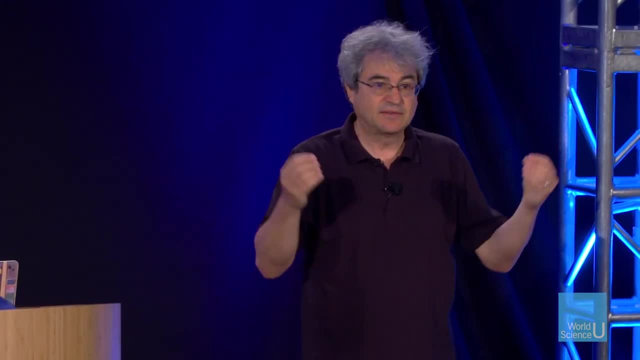 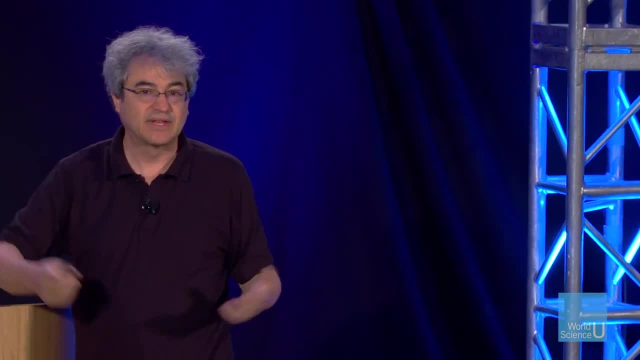 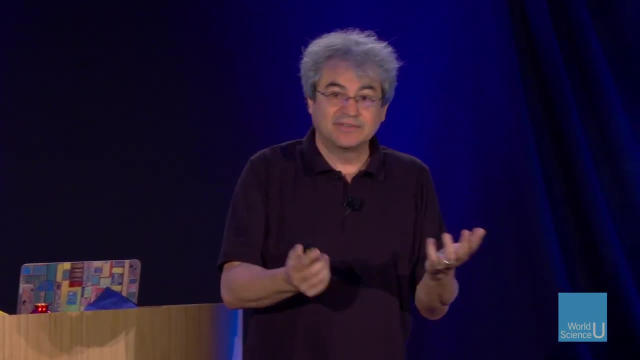 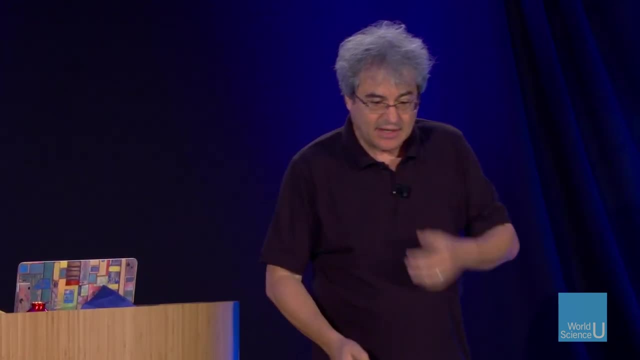 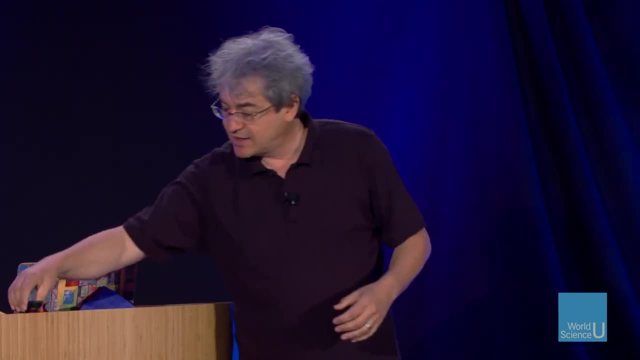 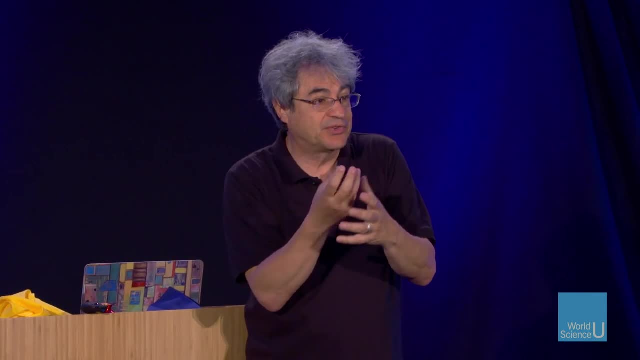 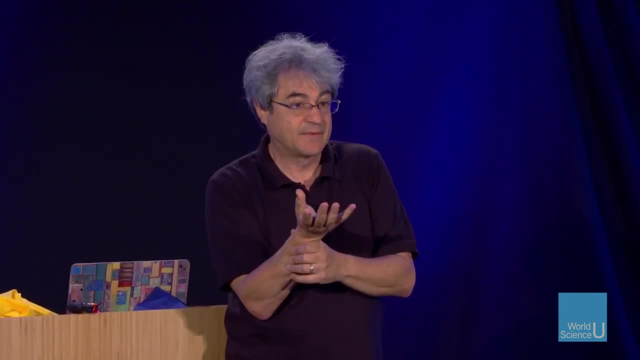 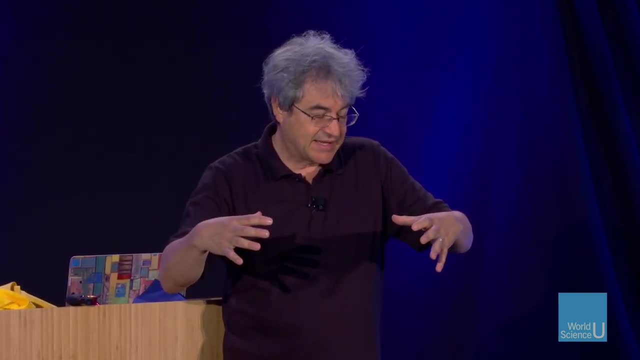 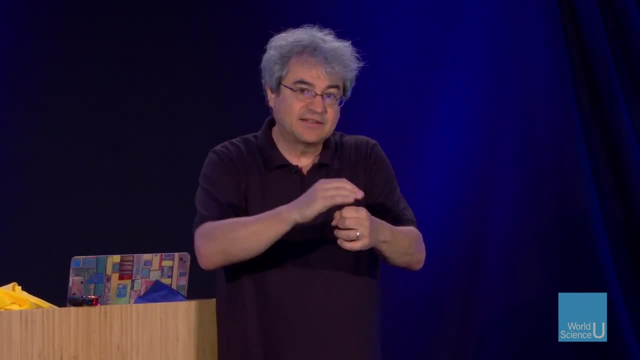 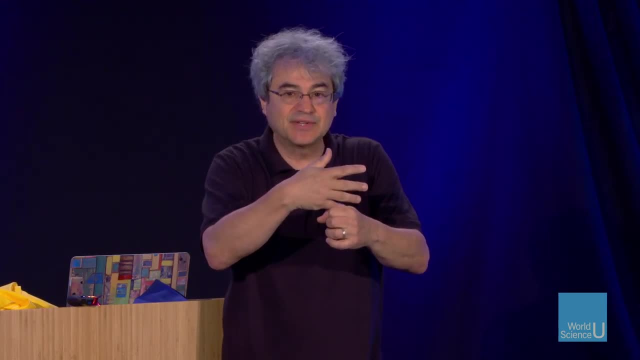 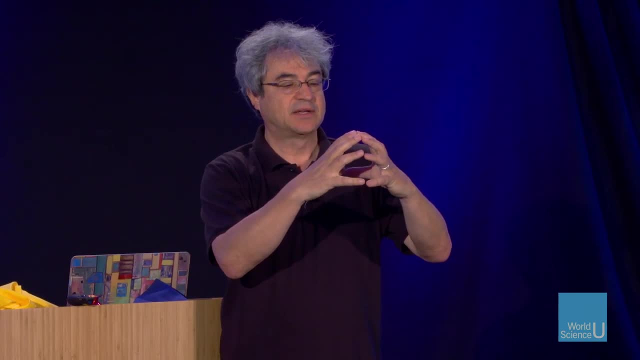 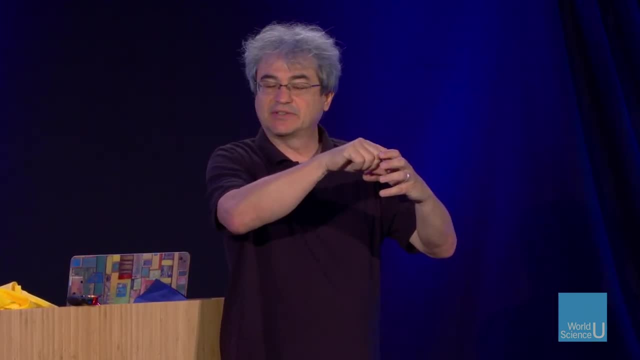 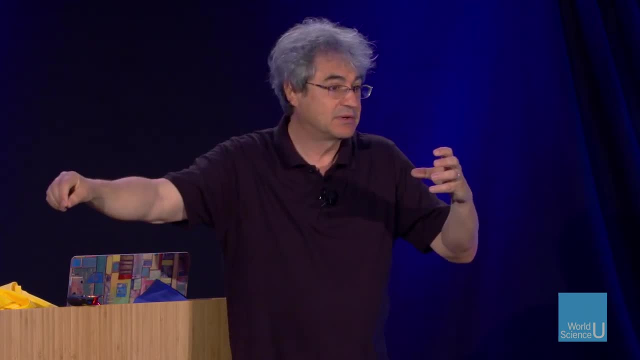 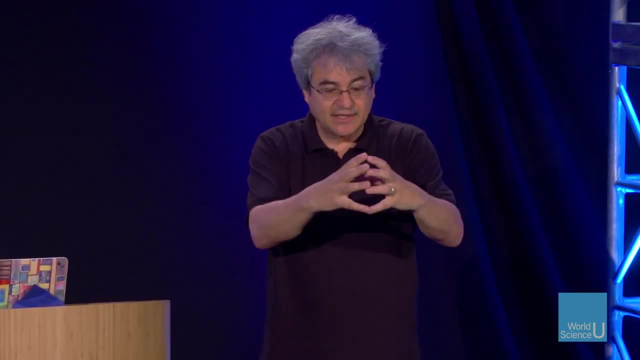 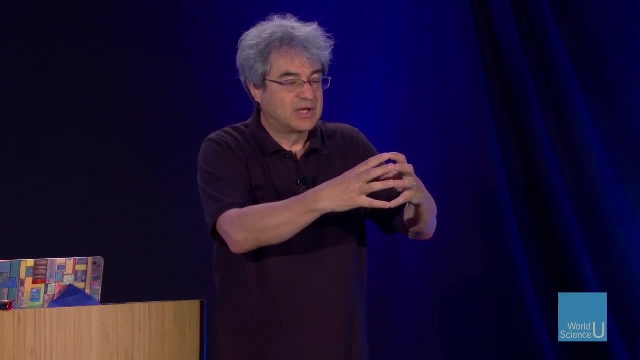 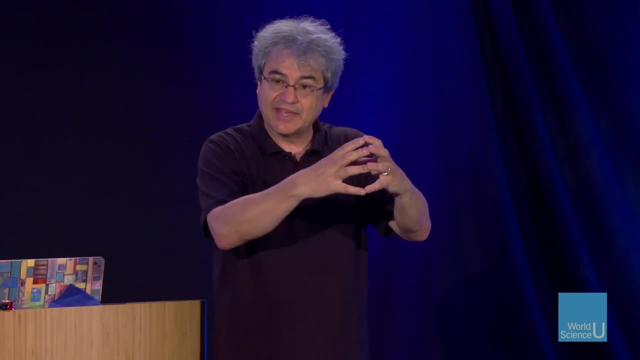 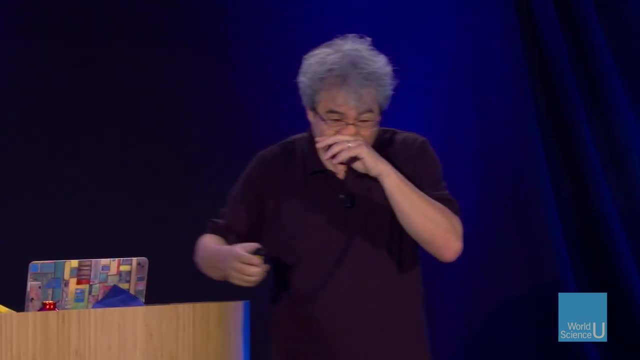 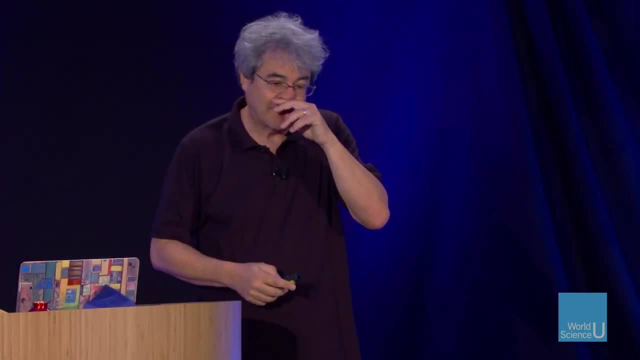 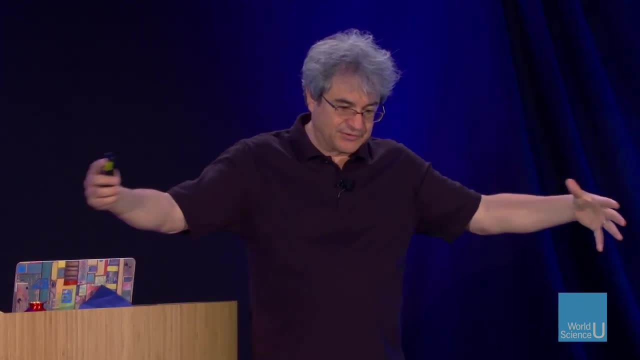 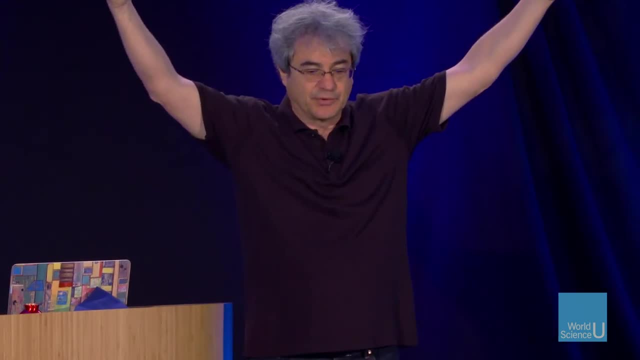 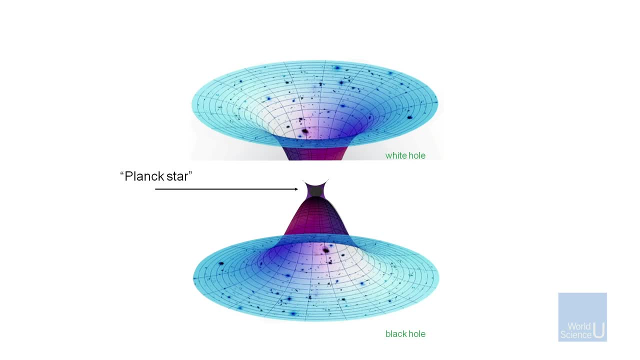 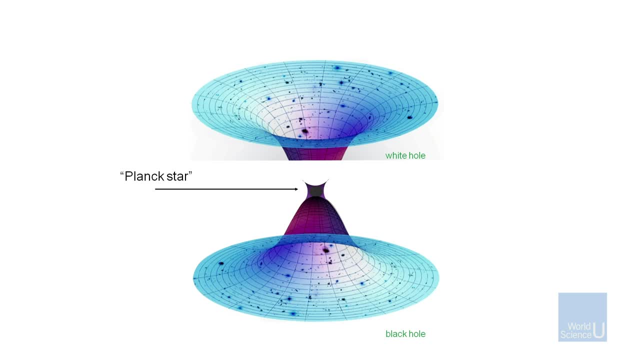 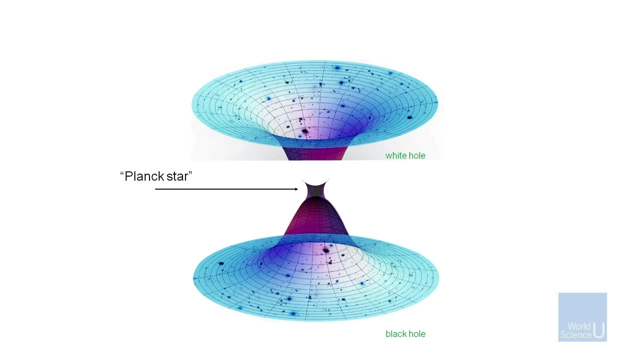 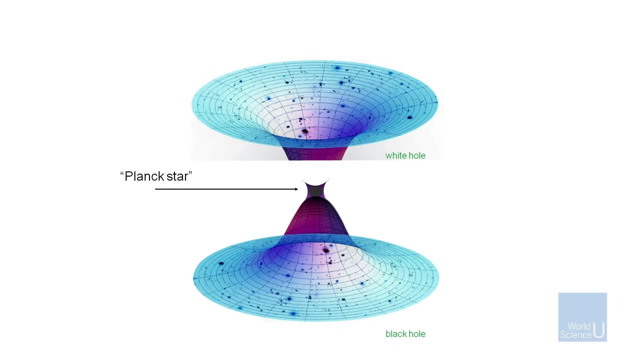 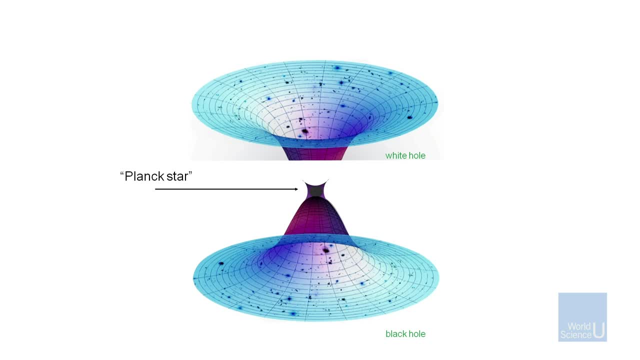 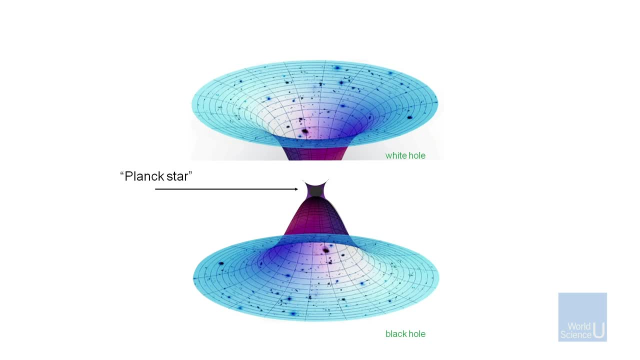 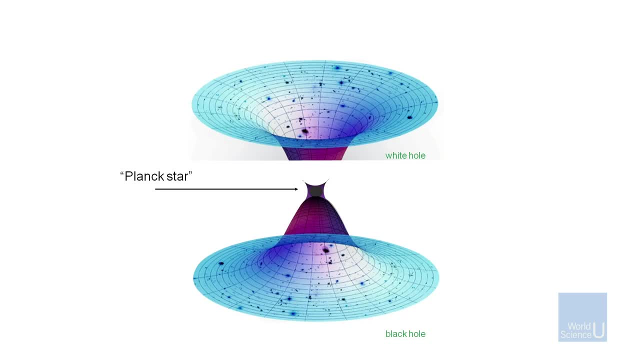 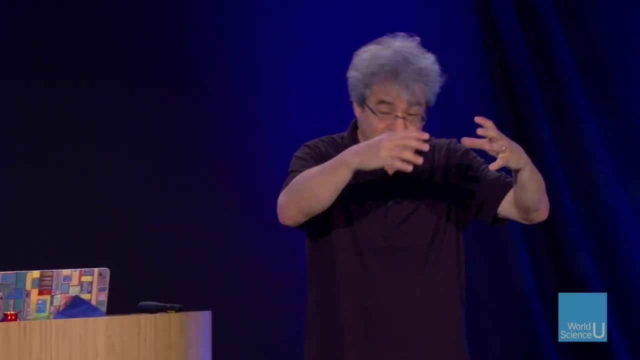 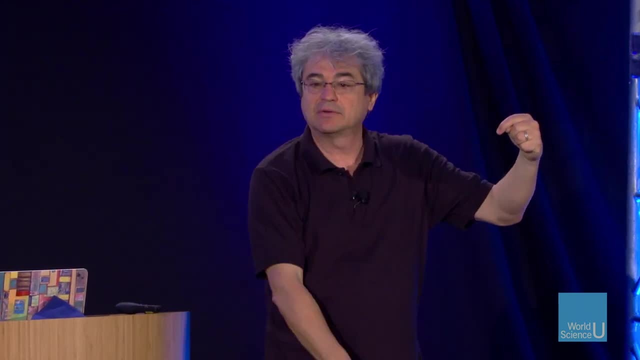 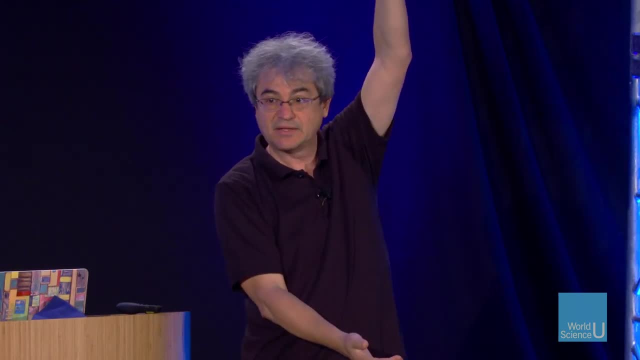 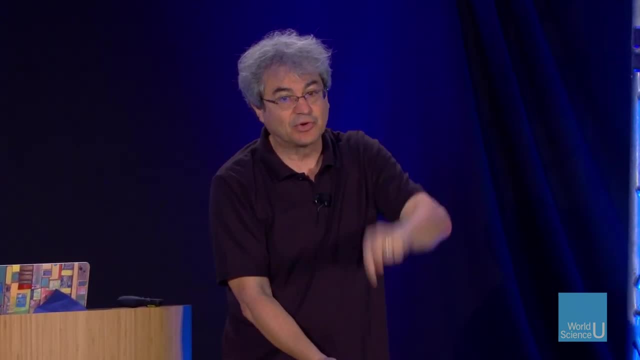 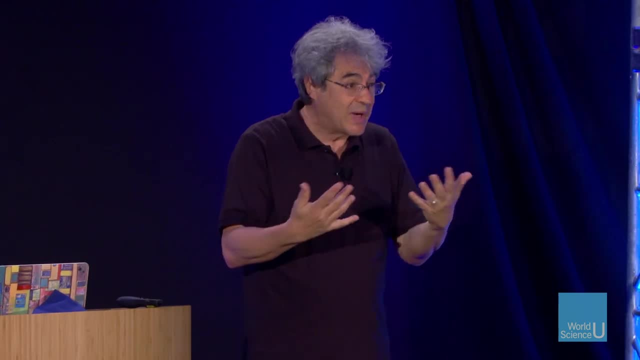 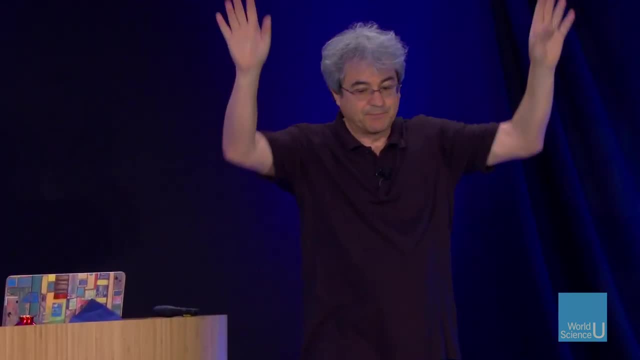 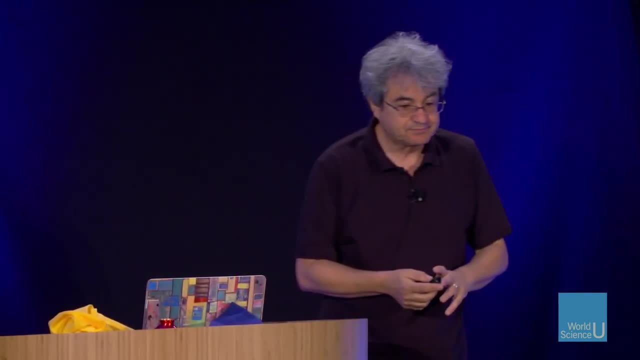 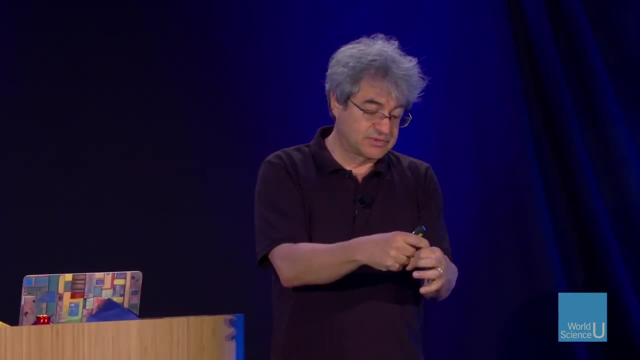 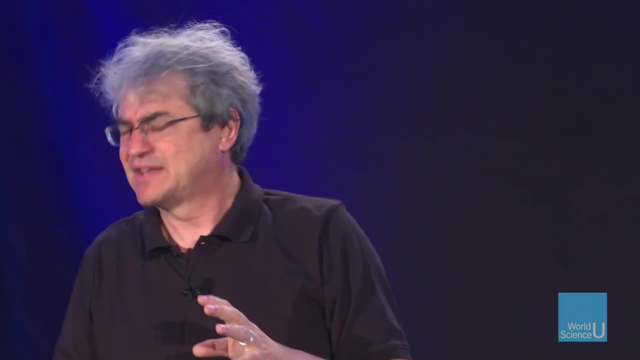 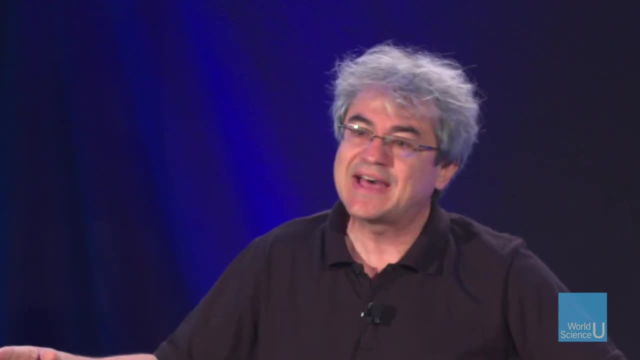 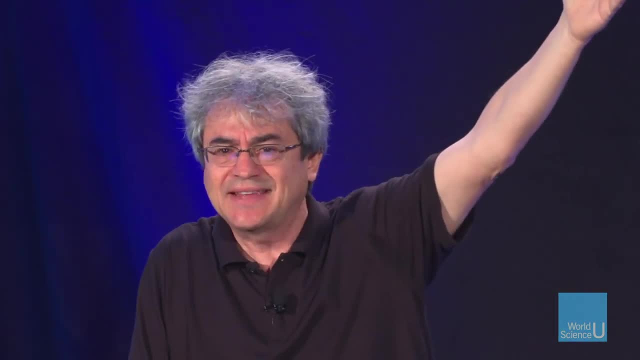 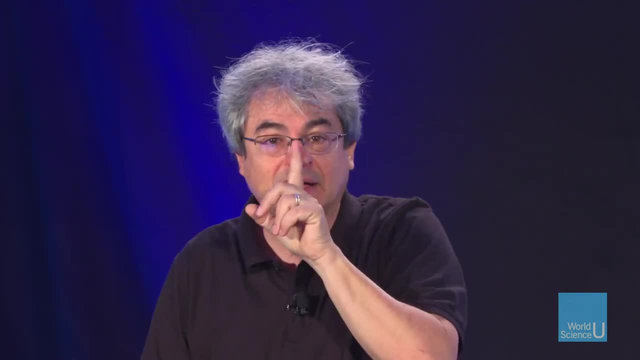 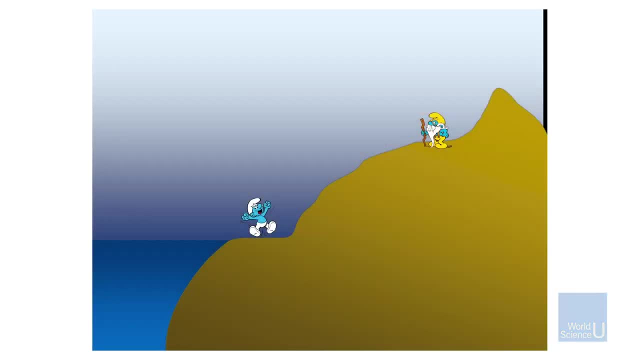 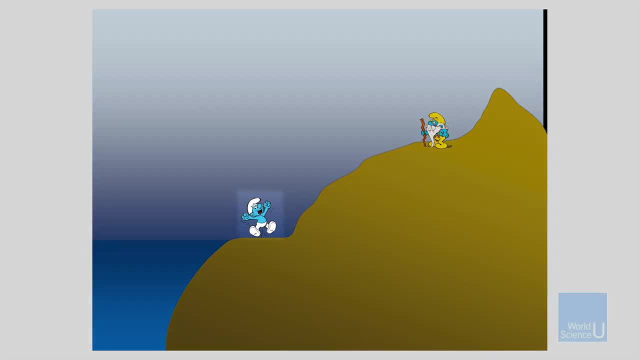 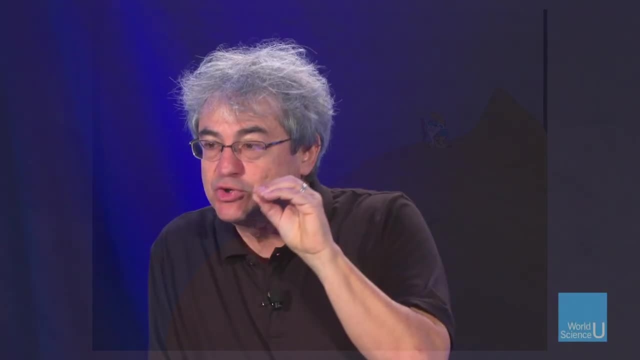 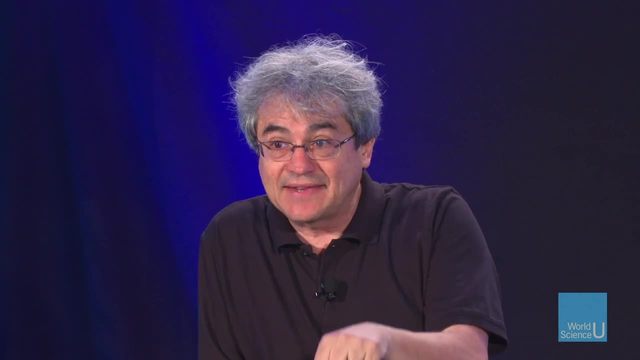 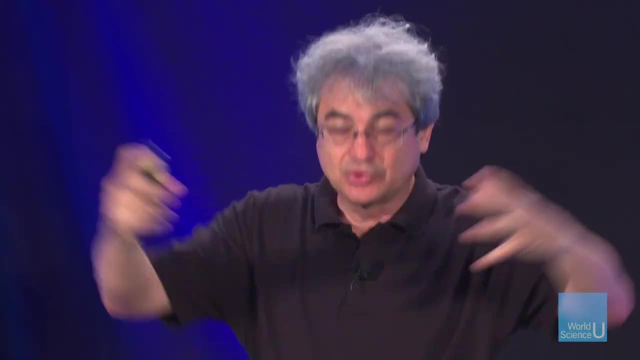 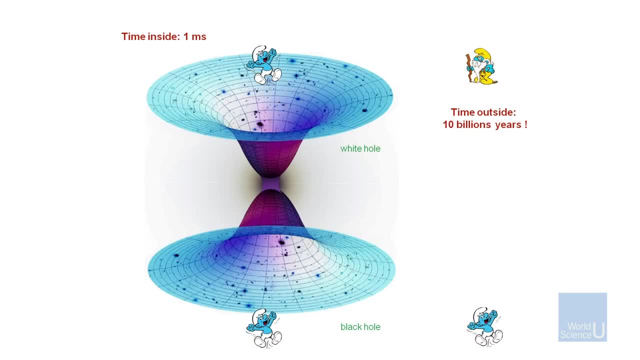 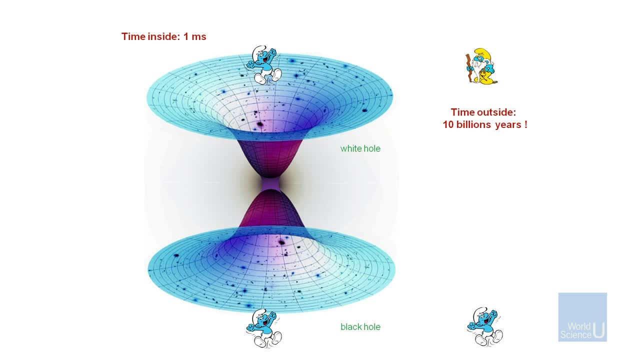 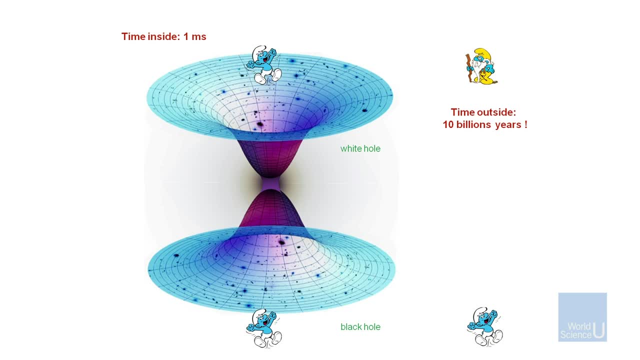 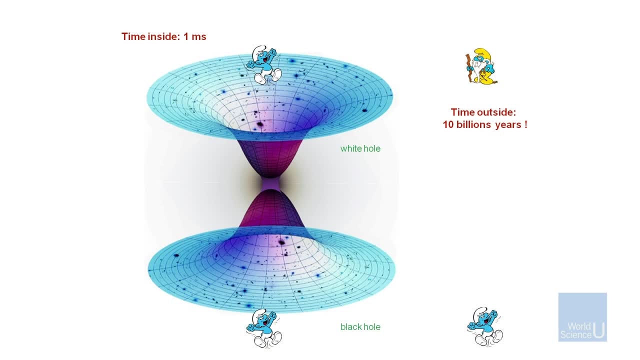 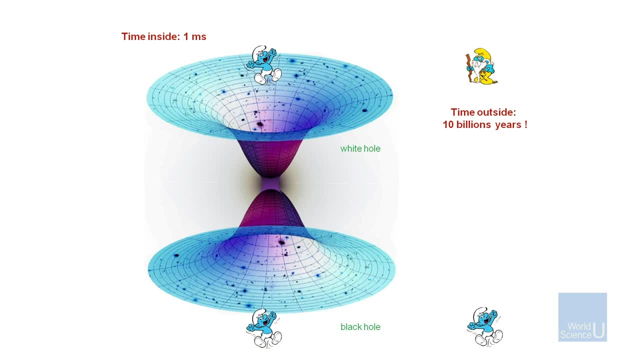 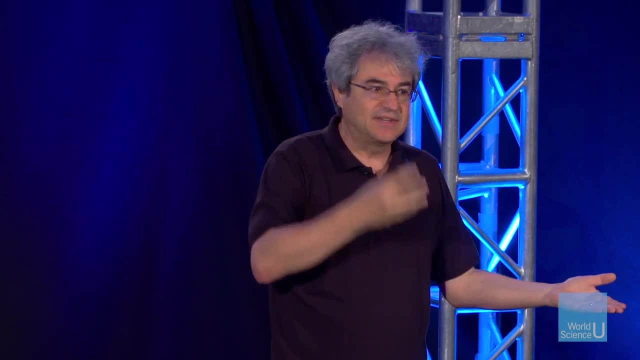 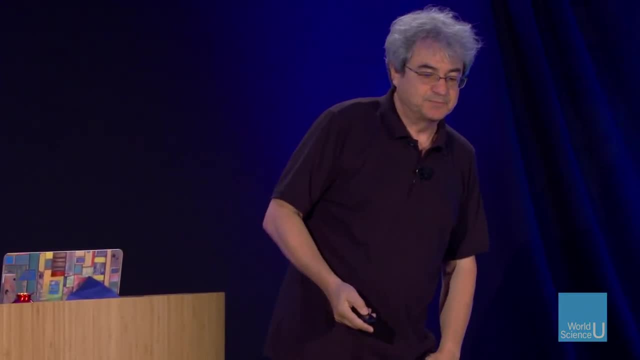 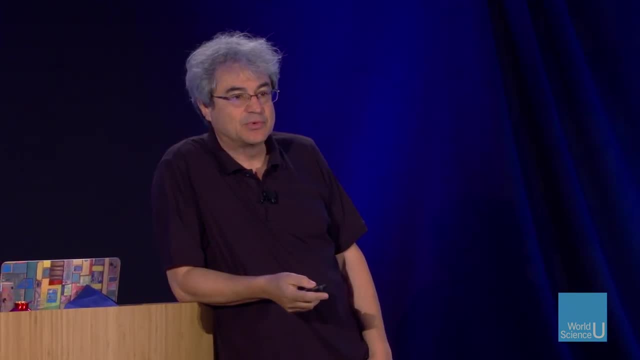 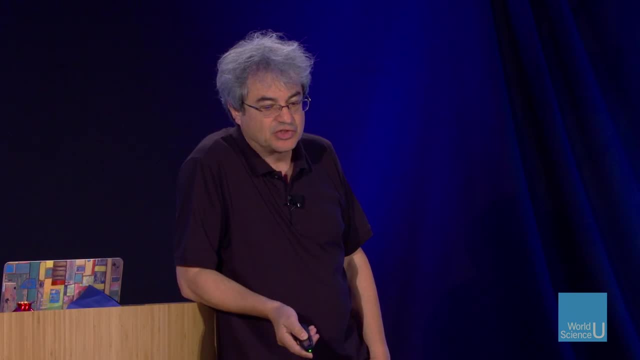 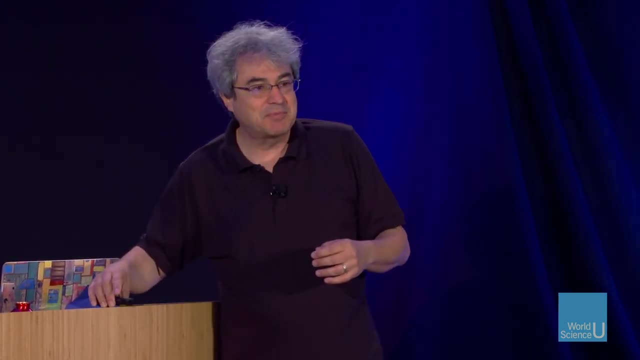 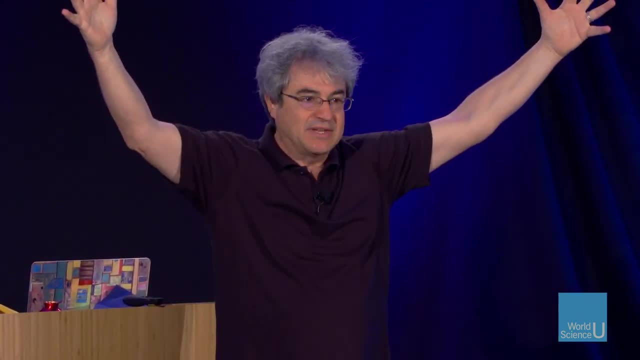 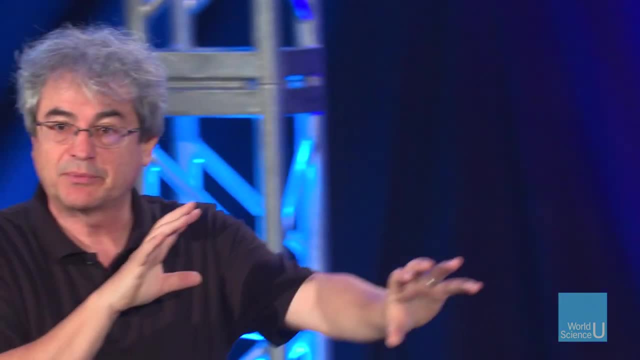 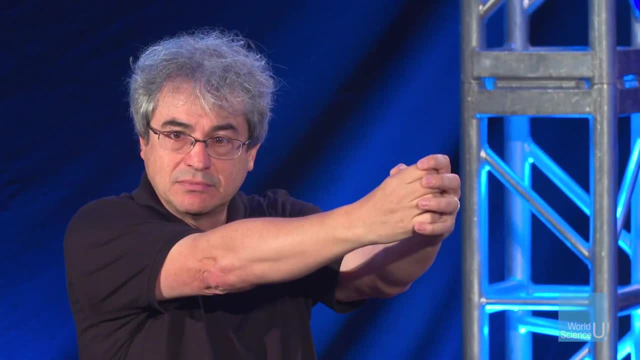 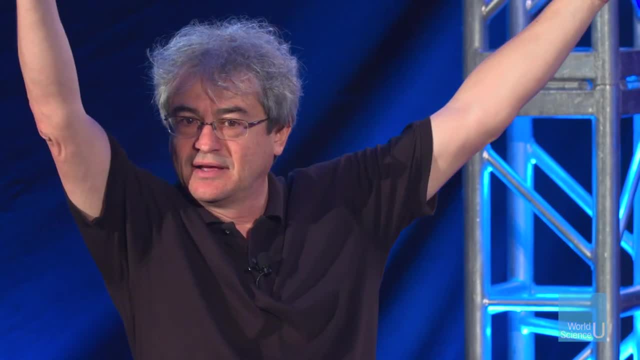 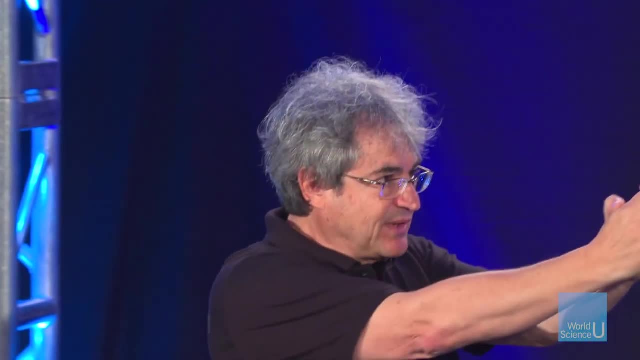 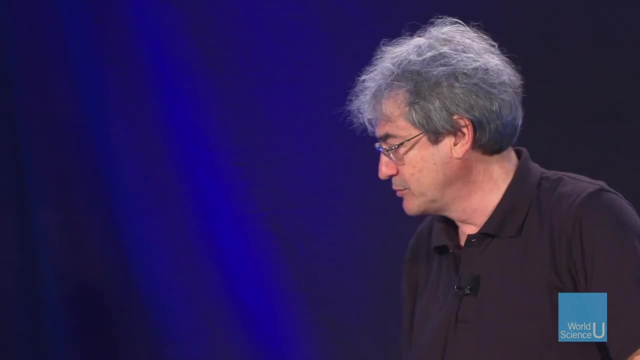 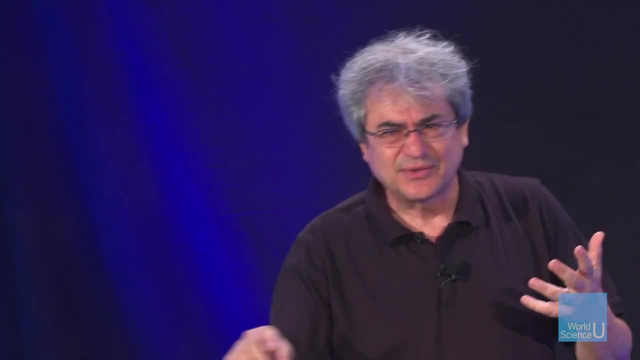 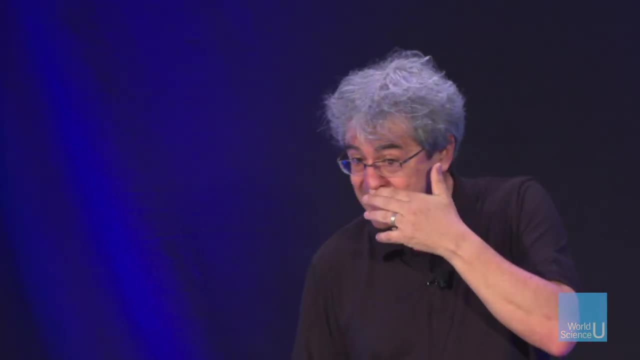 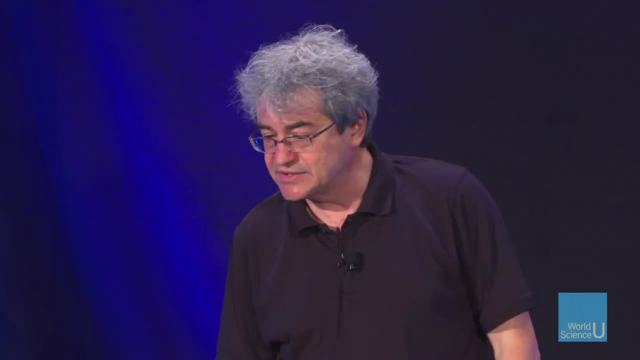 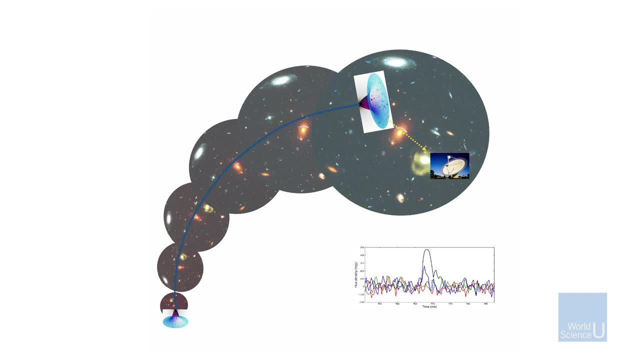 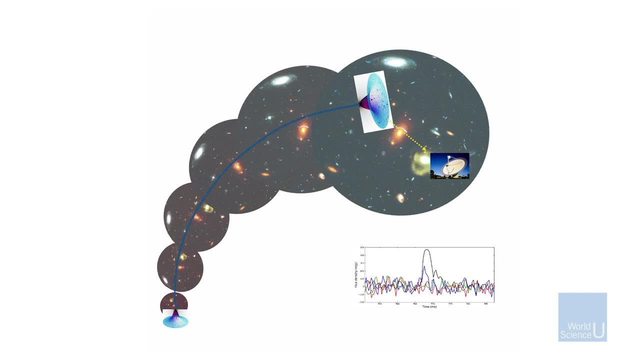 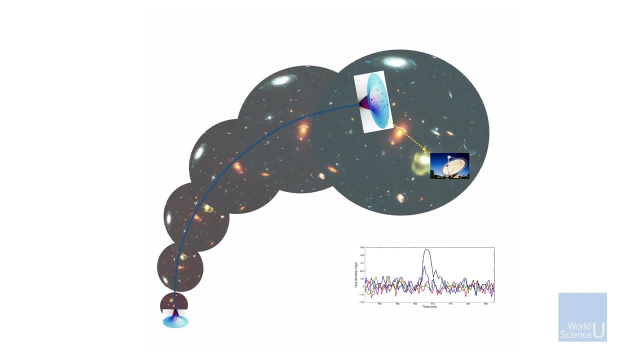 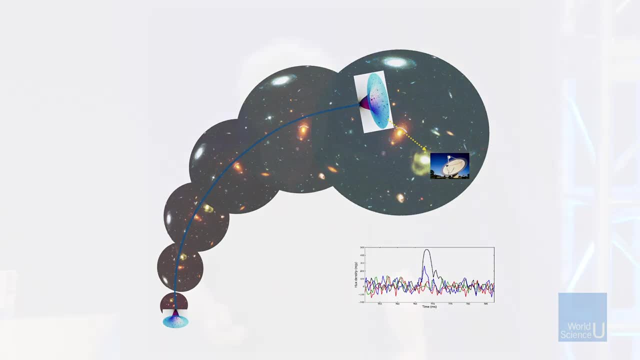 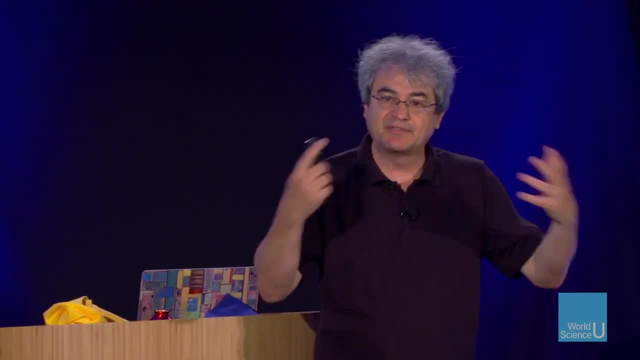 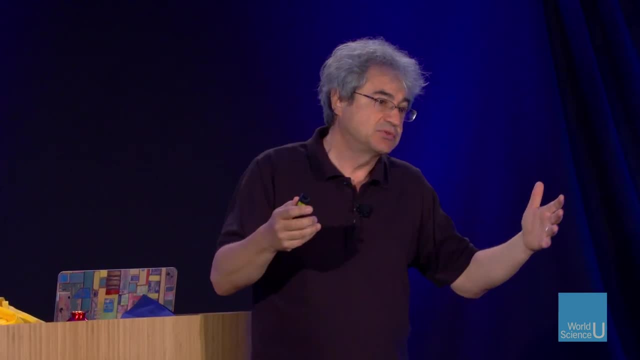 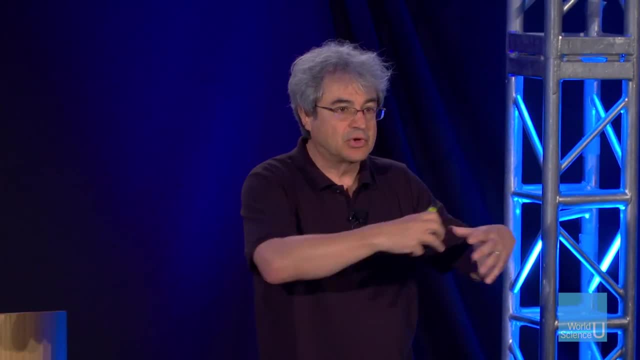 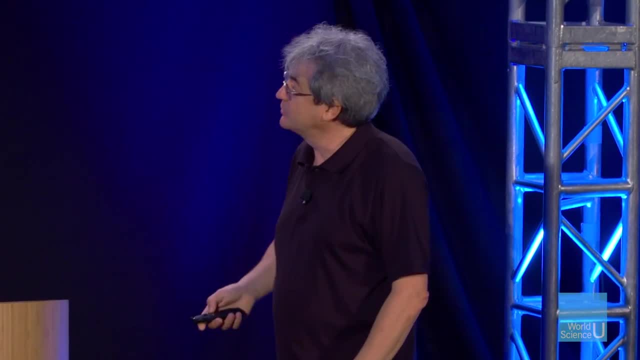 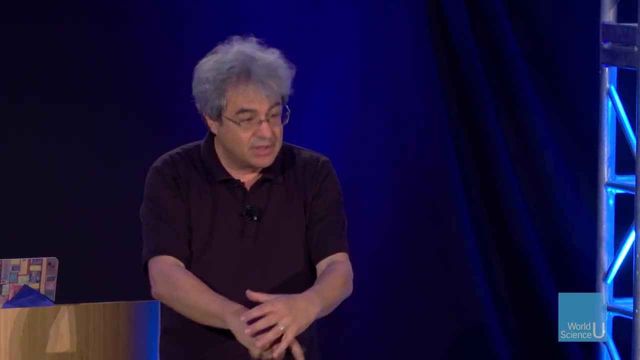 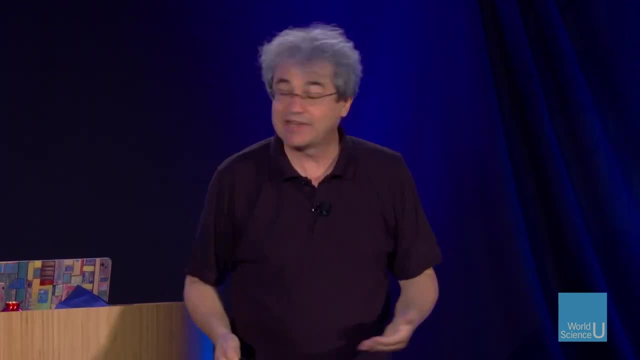 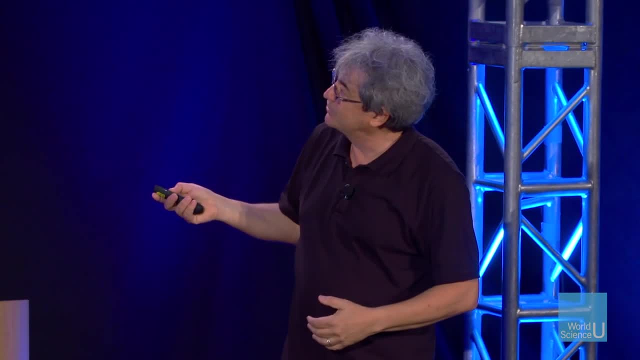 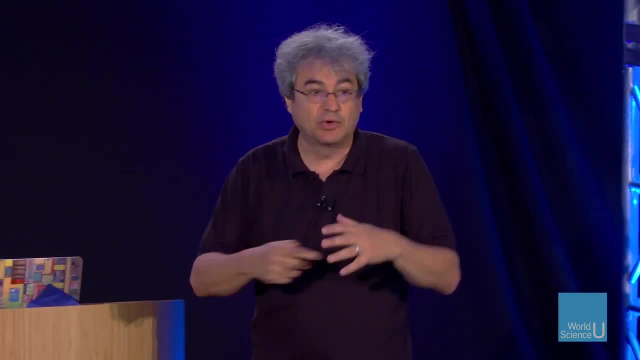 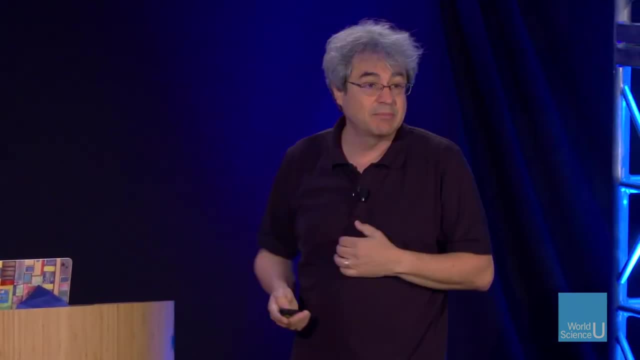 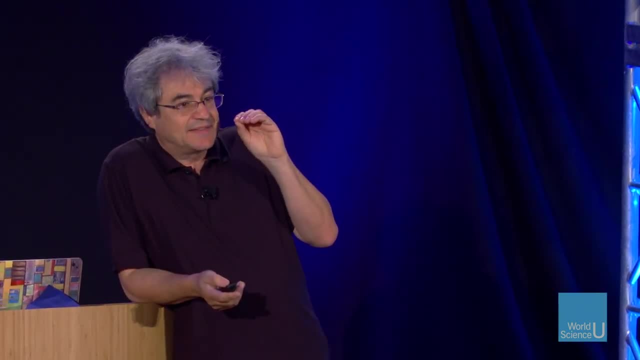 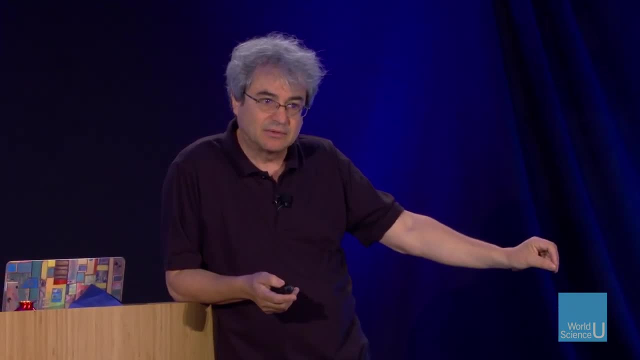 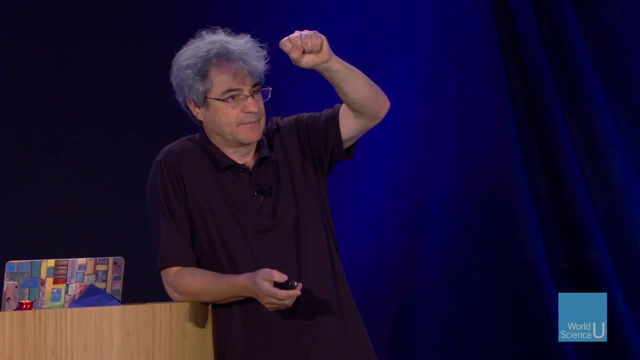 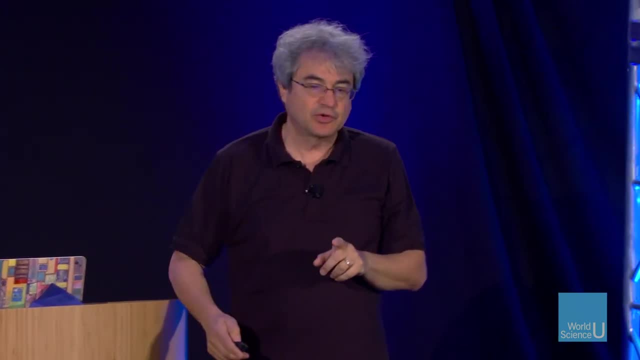 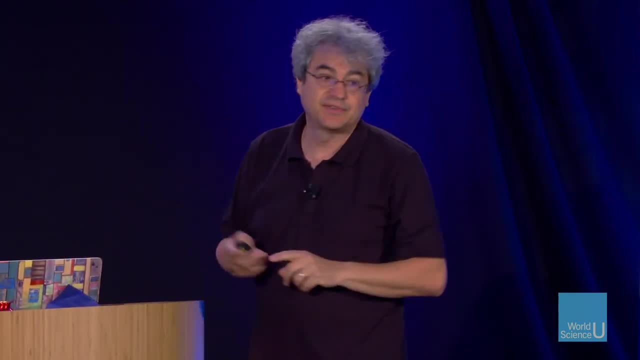 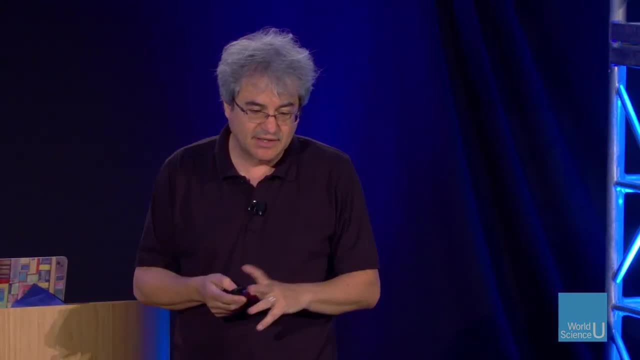 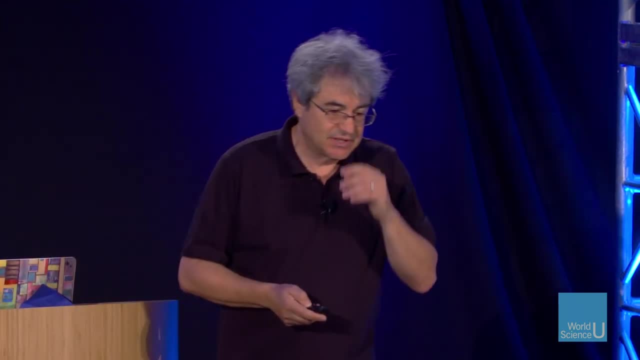 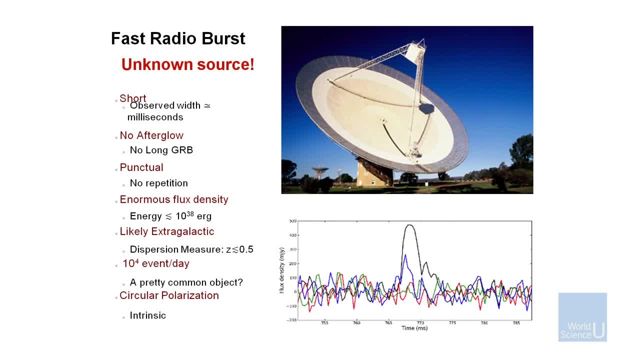 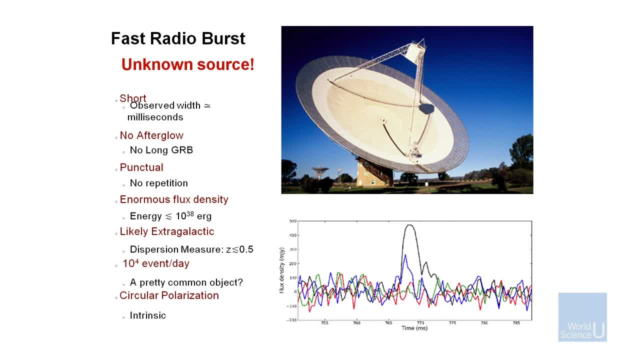 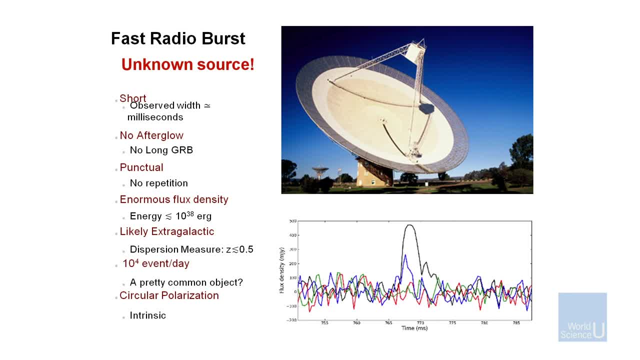 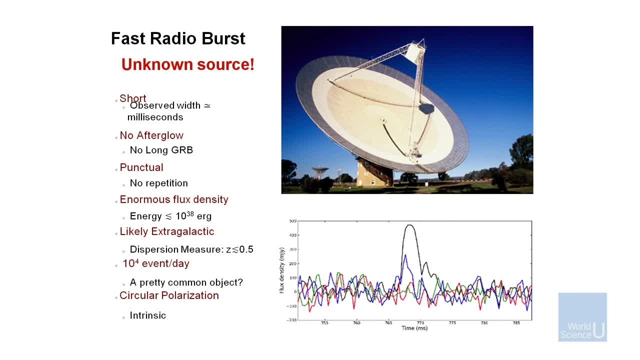 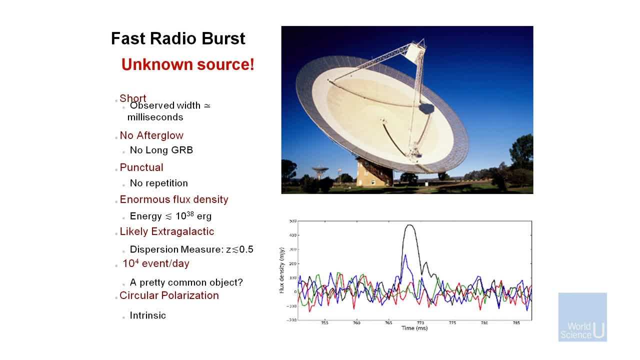 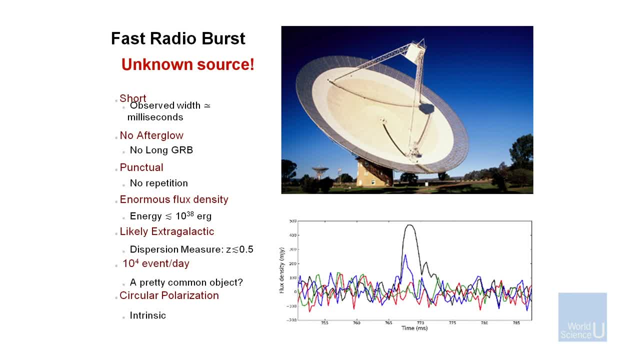 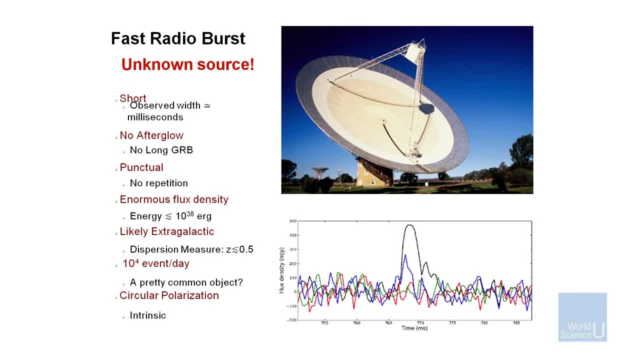 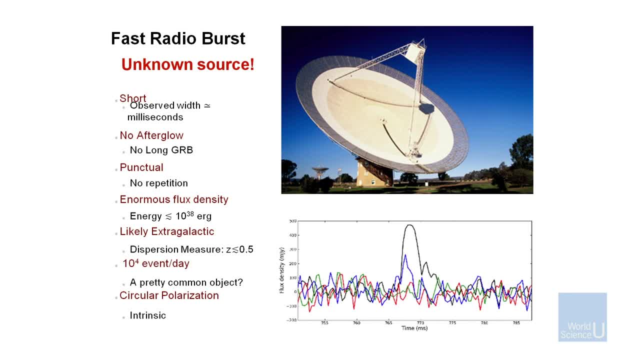 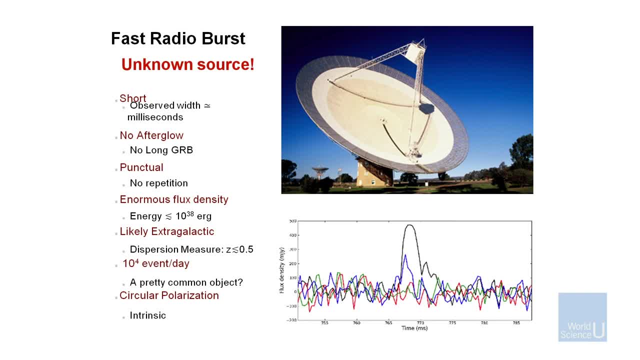 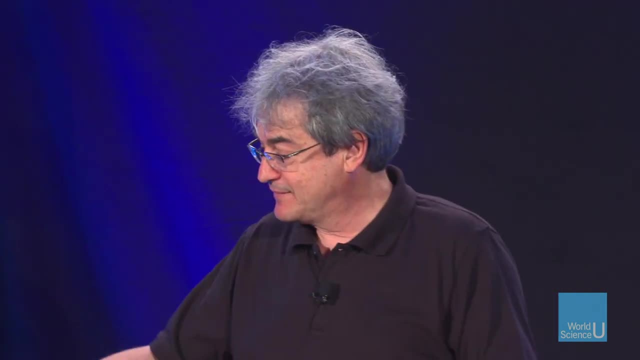 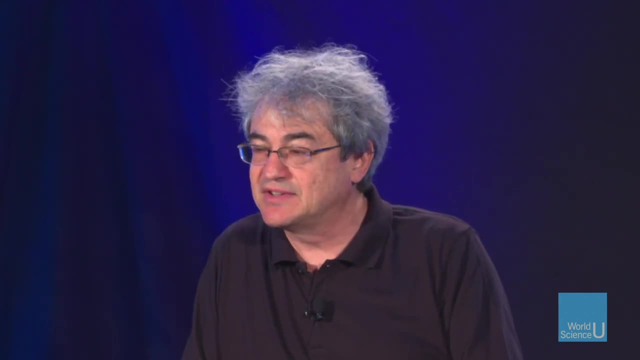 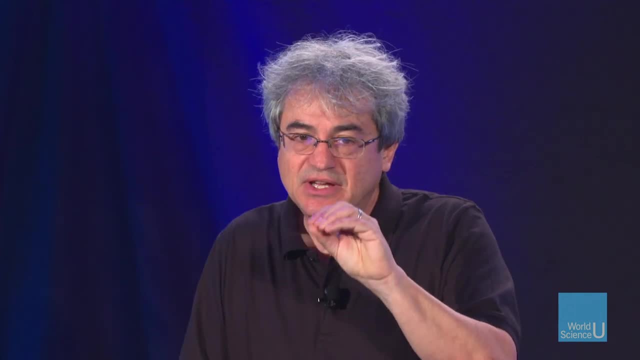 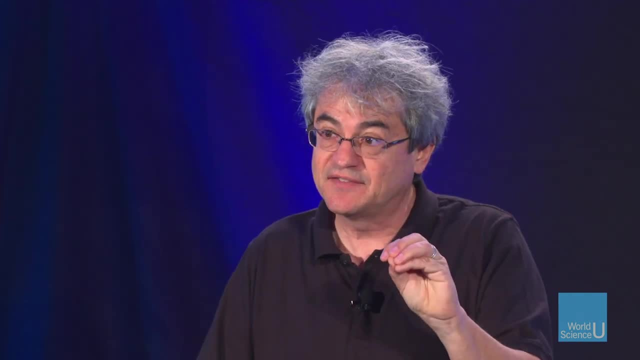 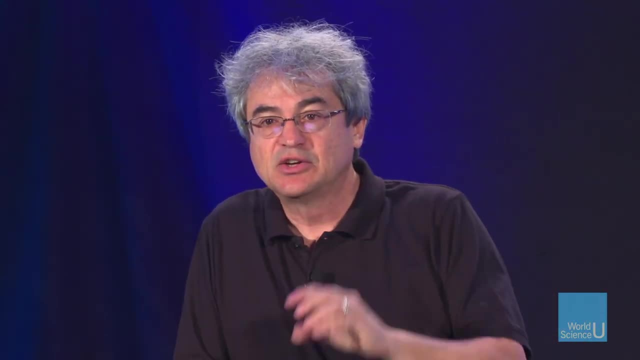 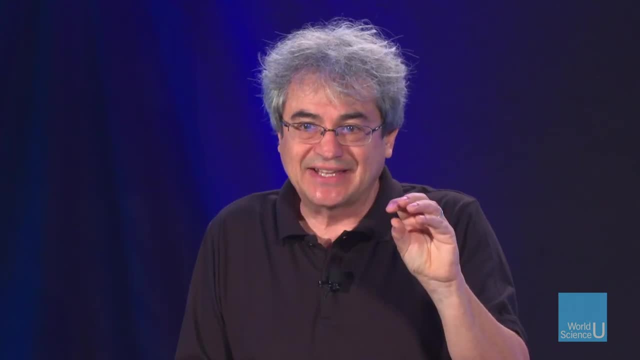 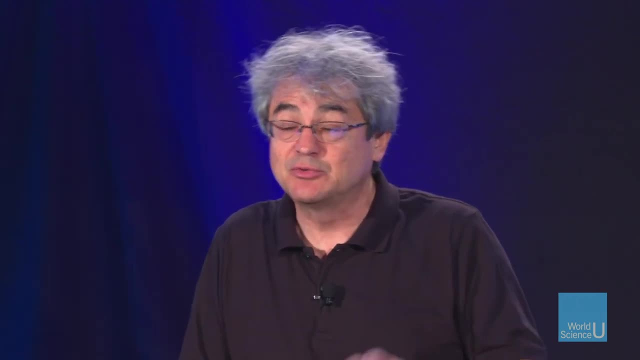 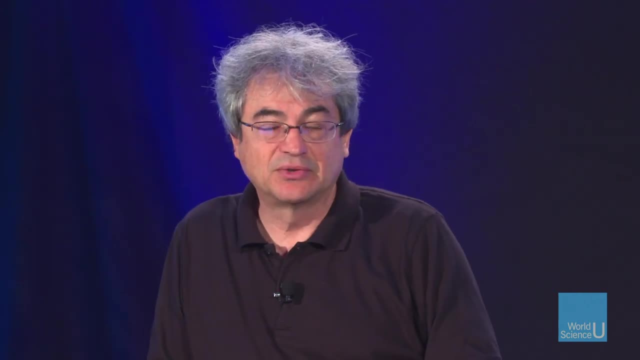 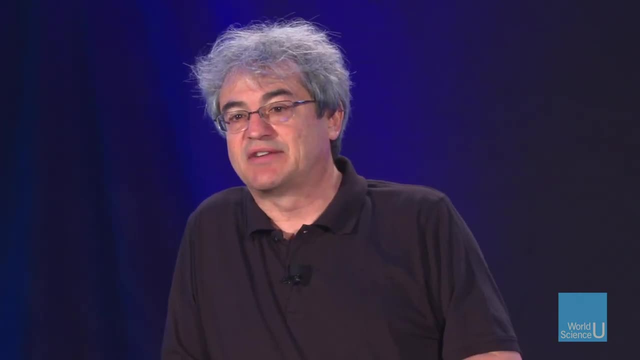 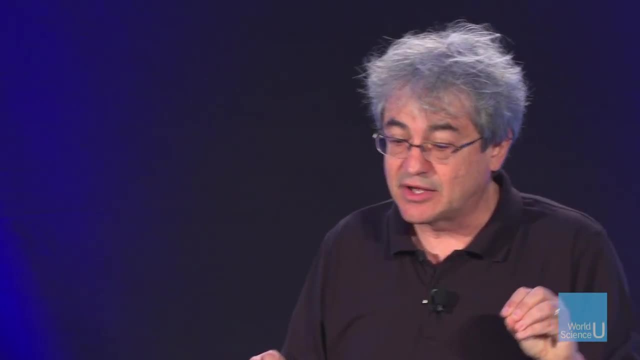 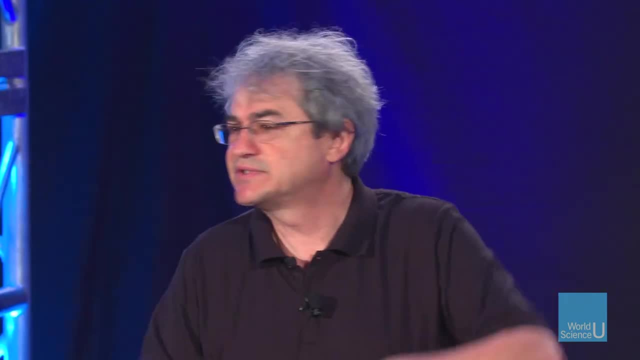 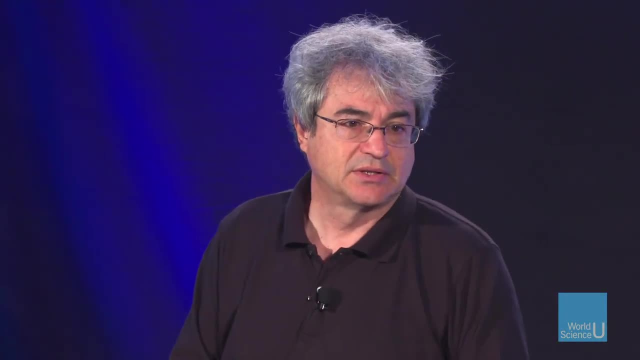 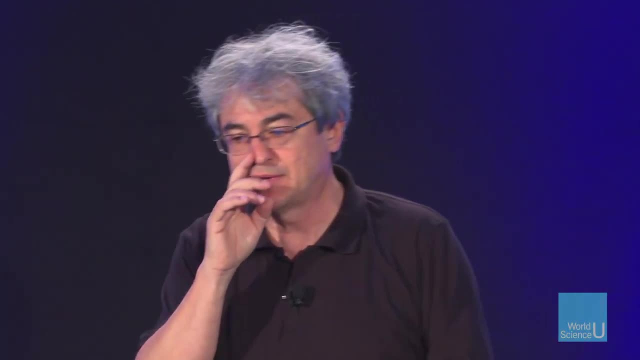 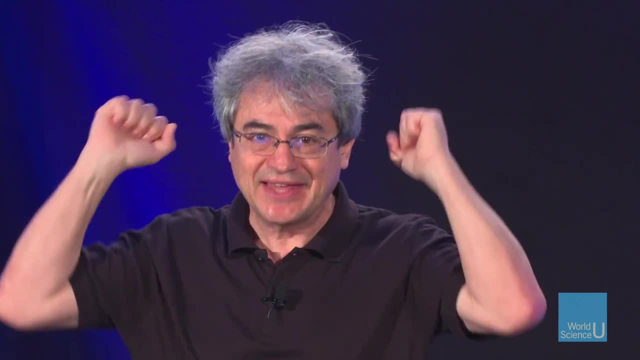 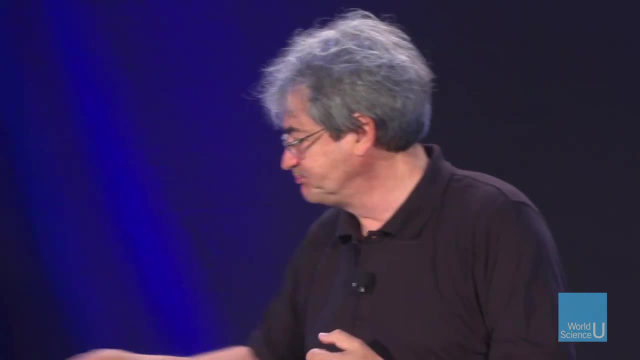 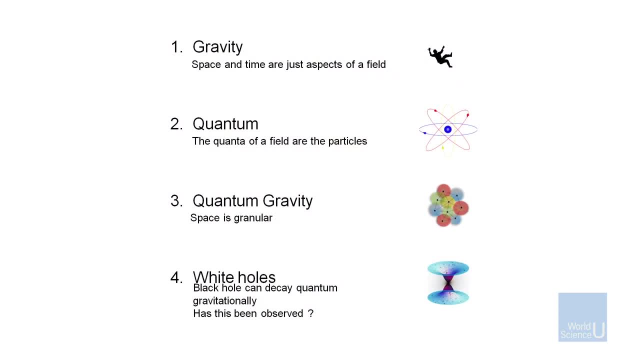 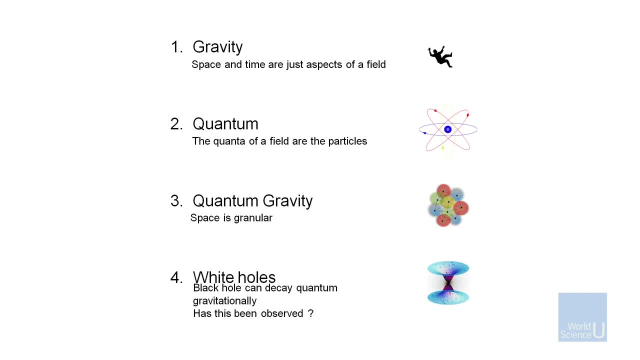 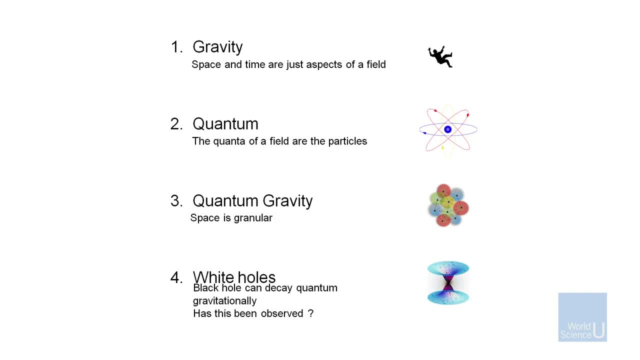 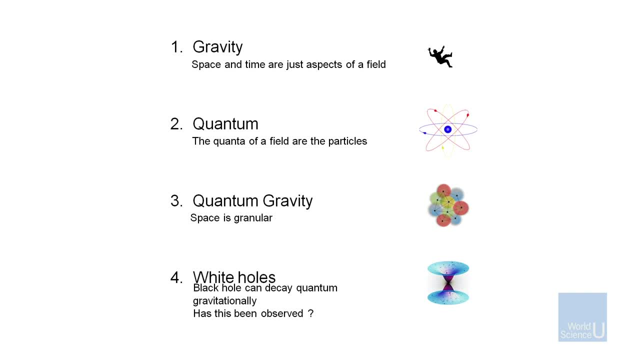 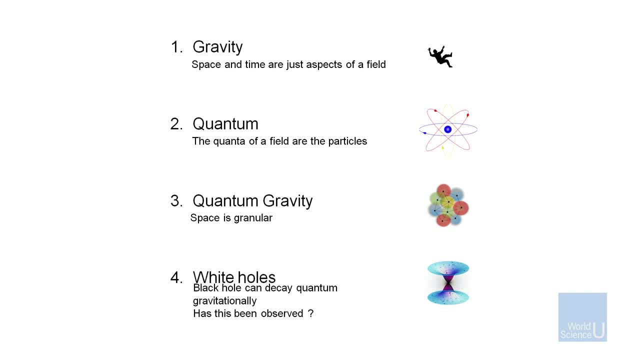 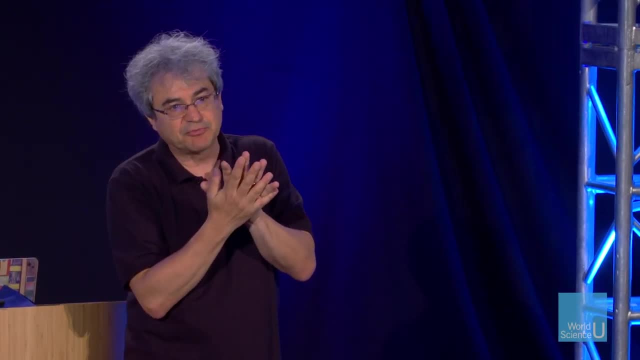 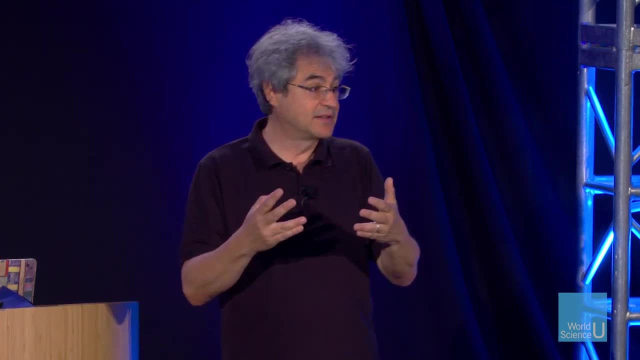 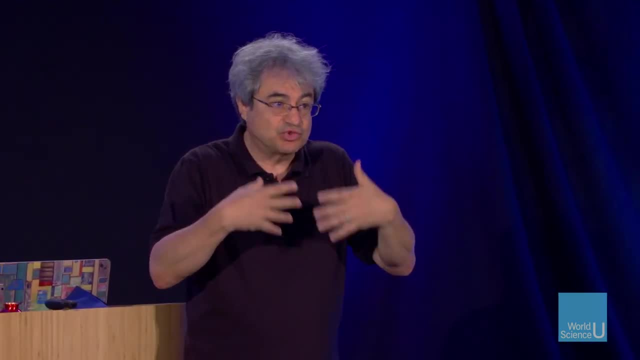 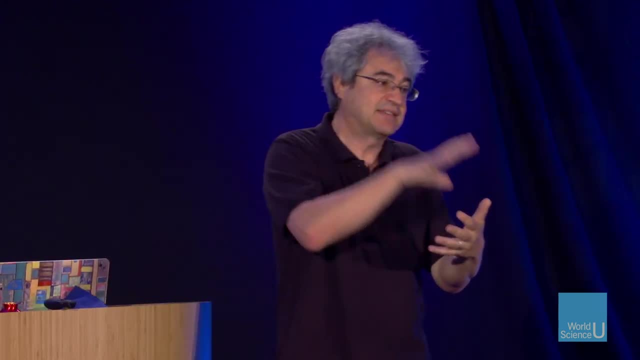 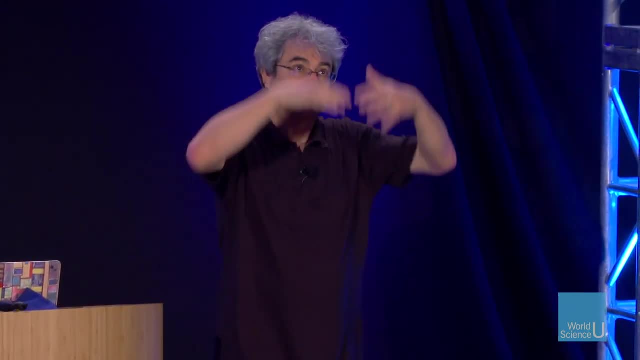 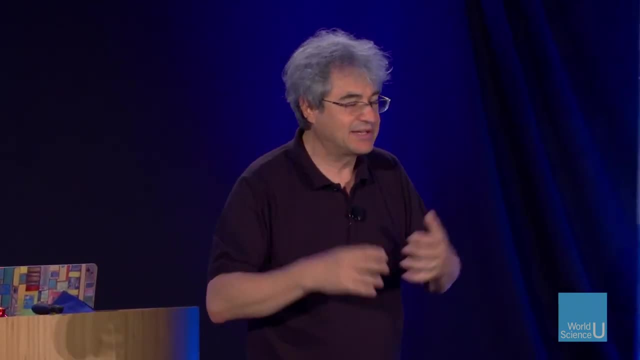 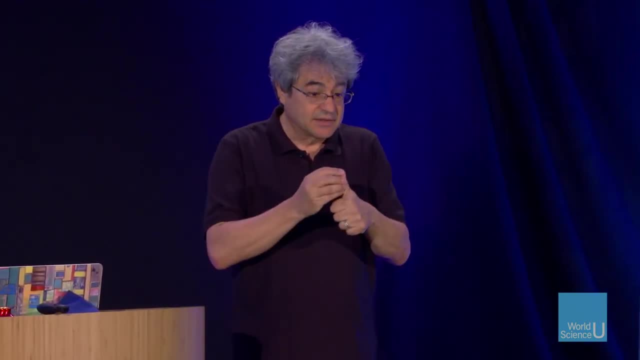 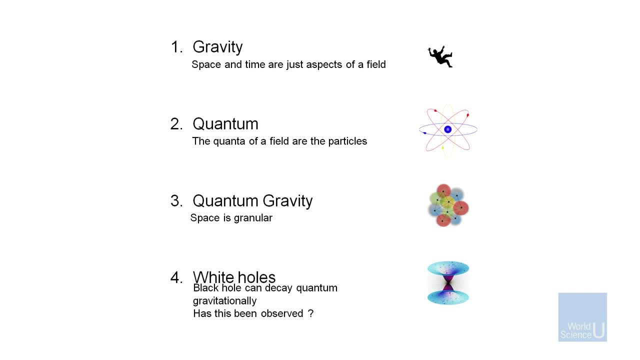 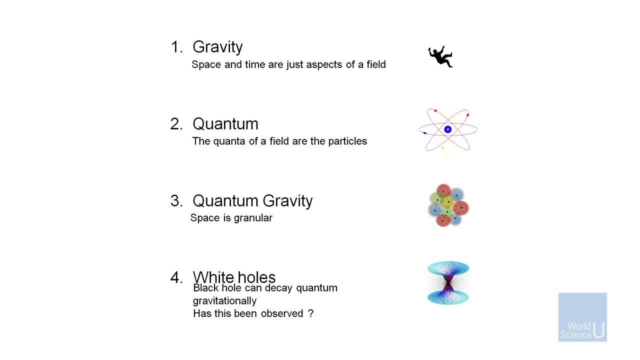 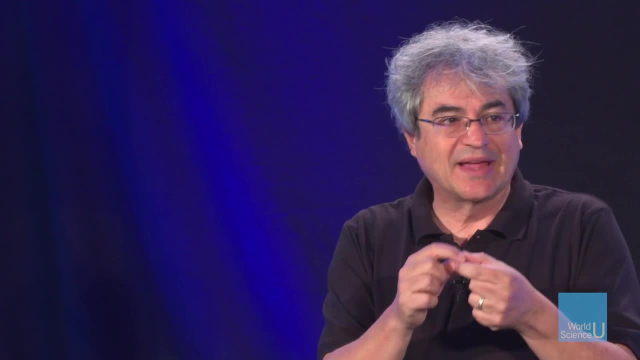 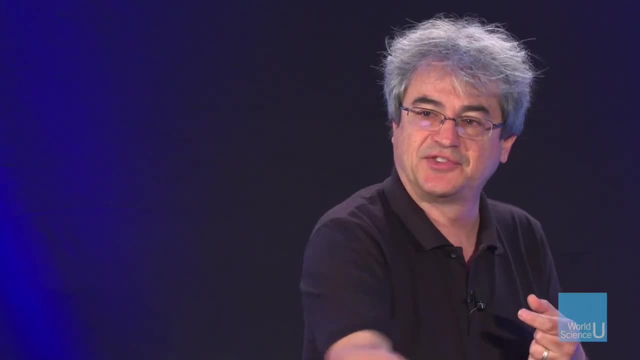 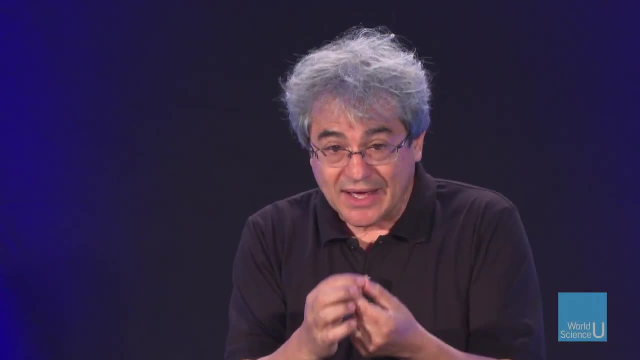 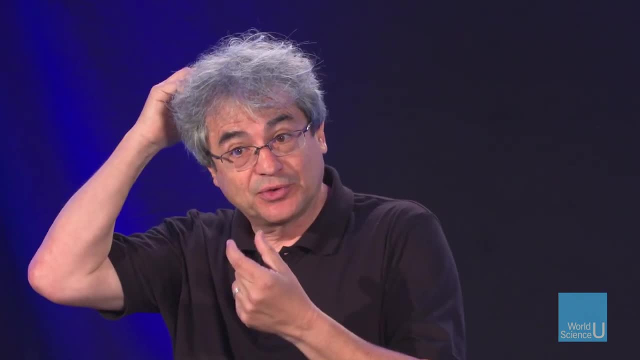 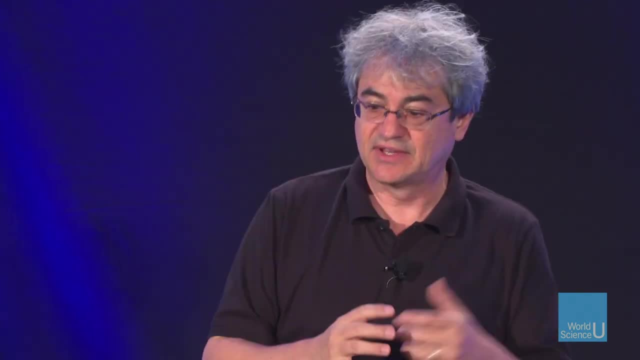 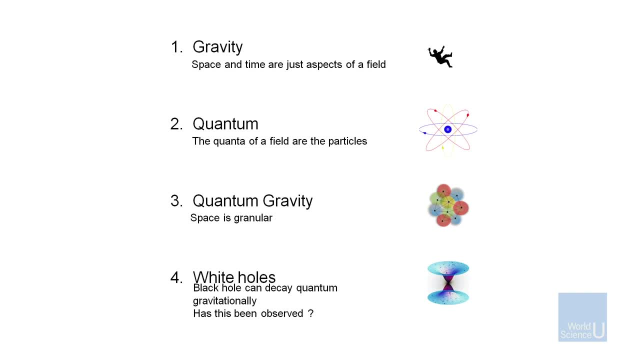 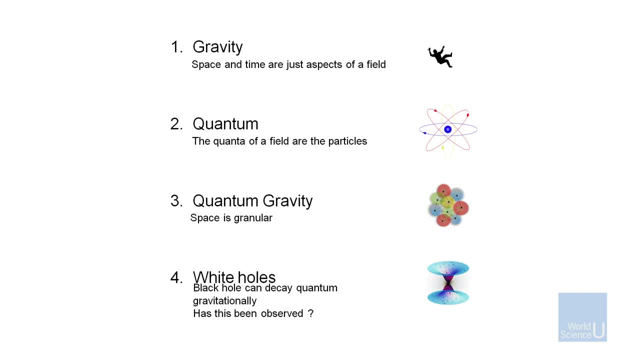 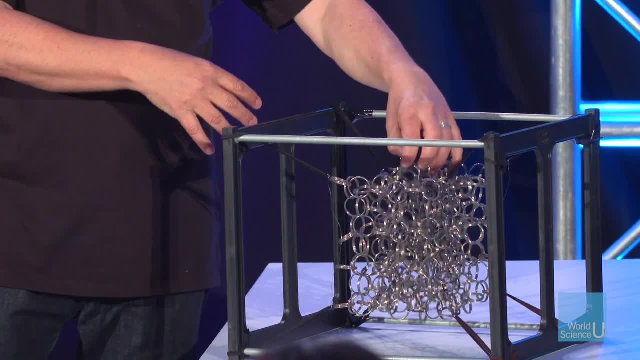 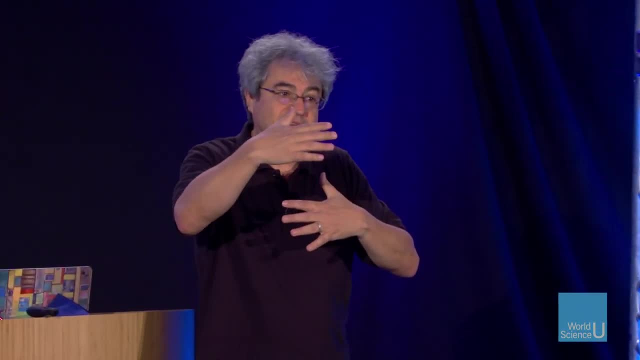 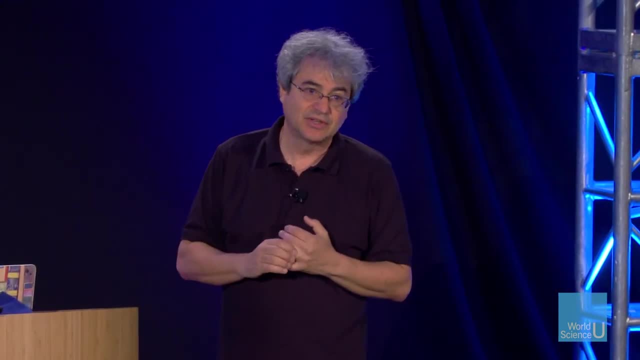 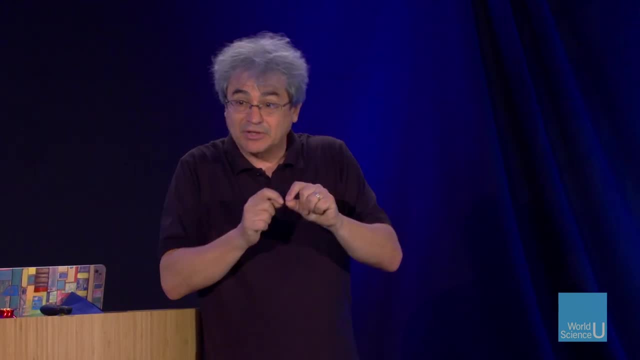 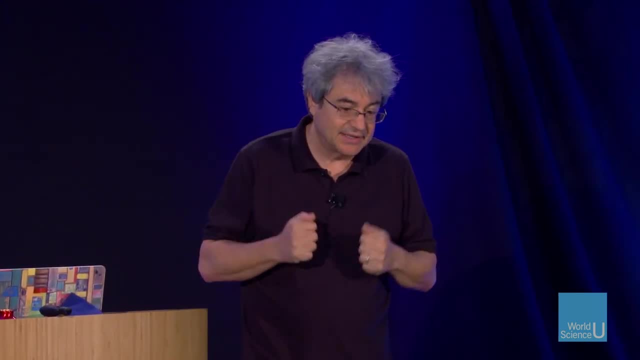 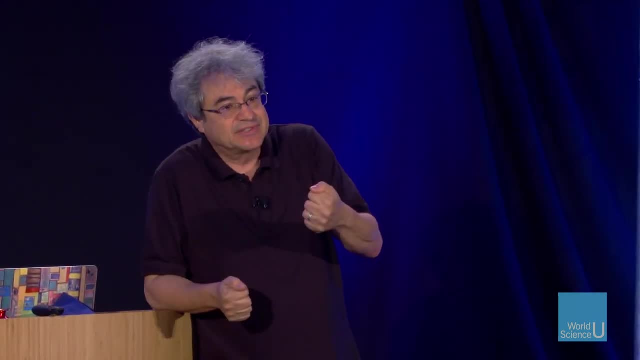 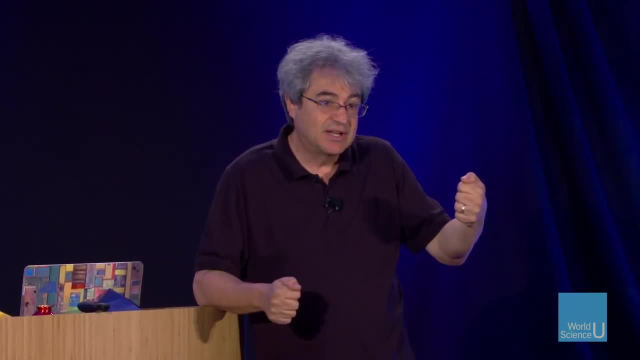 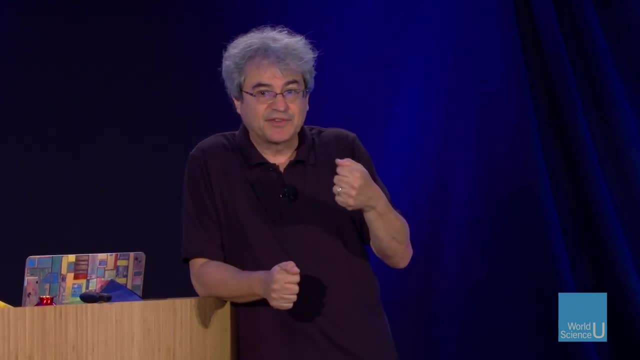 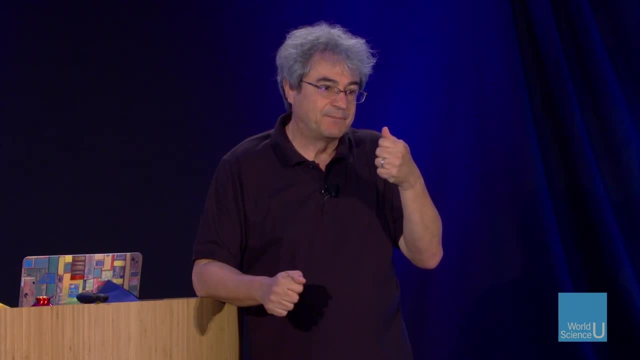 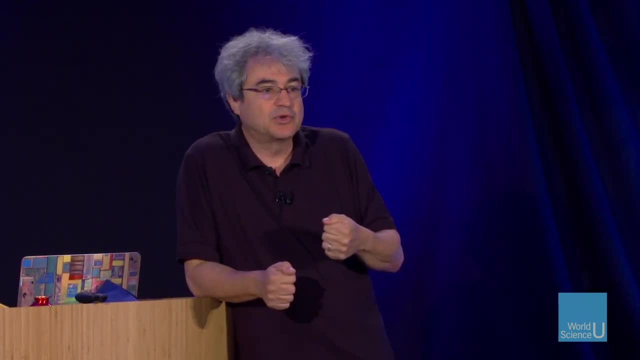 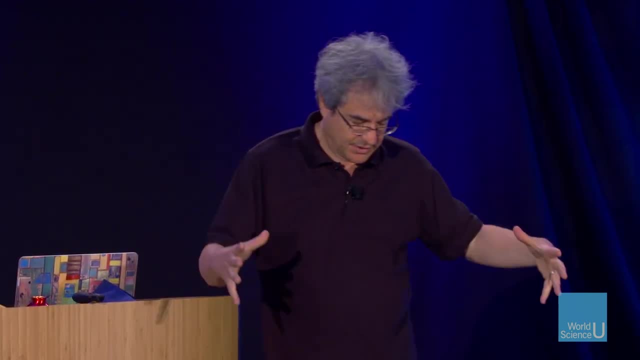 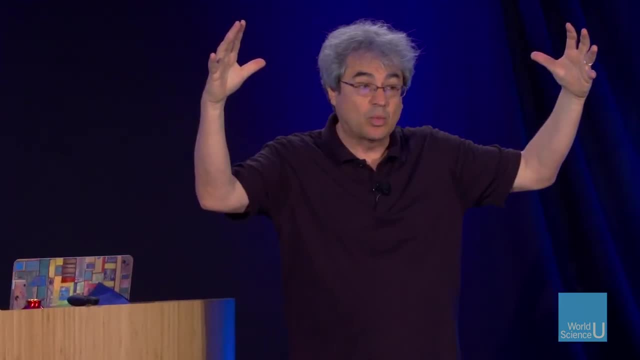 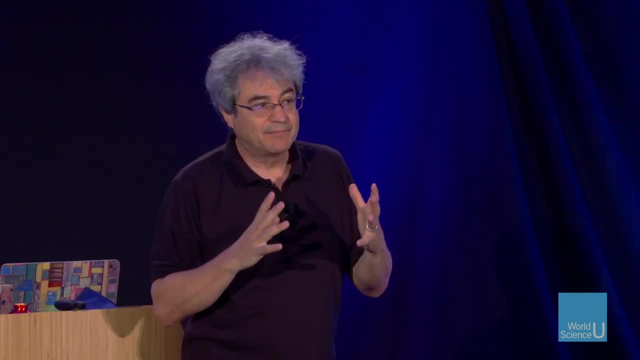 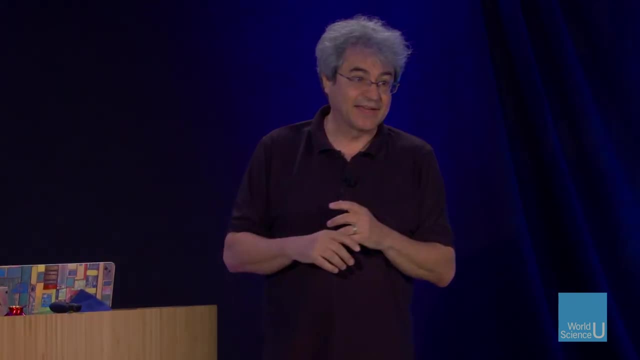 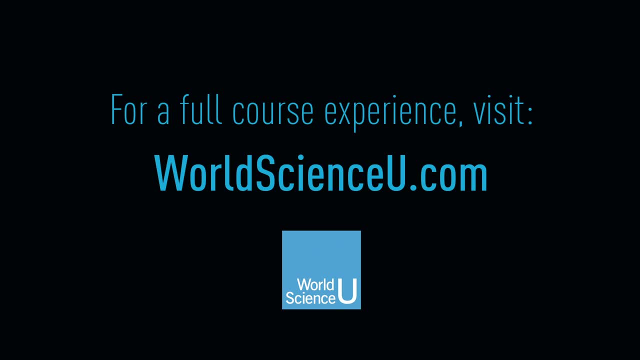